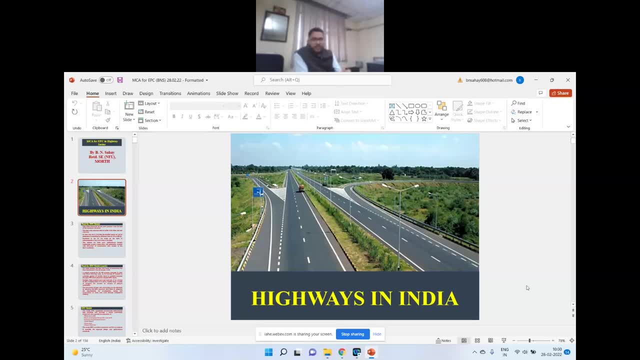 Now I would like to request our respected director, IHE Sanjeev Kumar sir, to address the participants. Sir, please Thank you. Thank you, Meena, and good morning everyone. First of all, I welcome all the participants on this very important calendar training program on contract management and dispute resolution. 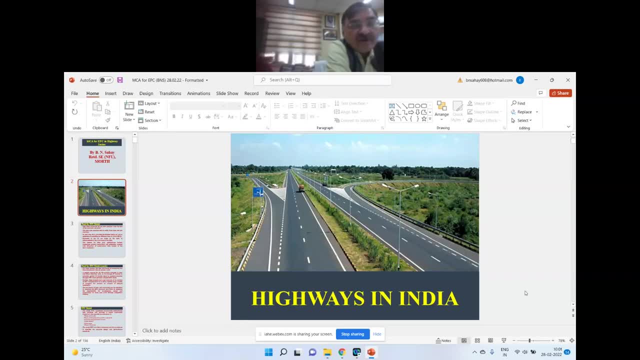 I also welcome Mr BN Sahai, who is recently retired. I know him very well from the Ministry of Road Transport and Highways. He shared with us his vast knowledge and experience in the very first session of this training program. During this training program, various aspects of contract management would be deliberated. 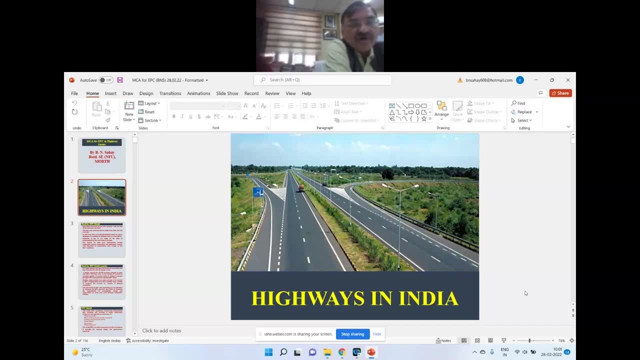 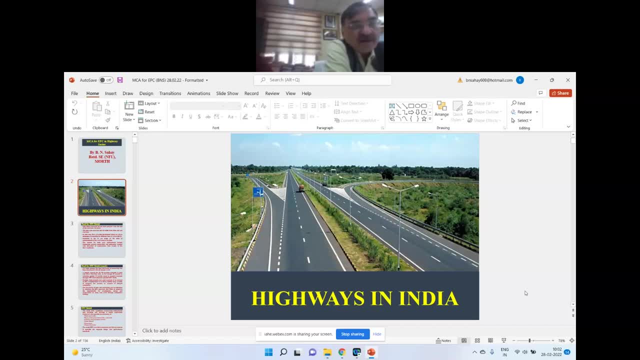 during this training program. uh contact management, to my understanding, is basically management of obligations in effective manner so that all the parties can efficiently utilize their time and resources. so we should be very particular about fulfilling our obligations and we have seen number of times uh dispute arises if we are not. 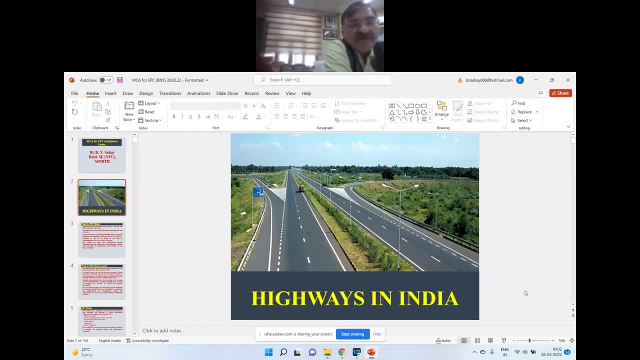 fulfilling our obligations, and it may leads to a huge loss in the form of fines, liquidated damages. Moreover, whatever benefits are to be accrued to the users, those are also affected. So I think we should be very particular to understand the nitty-gritty. 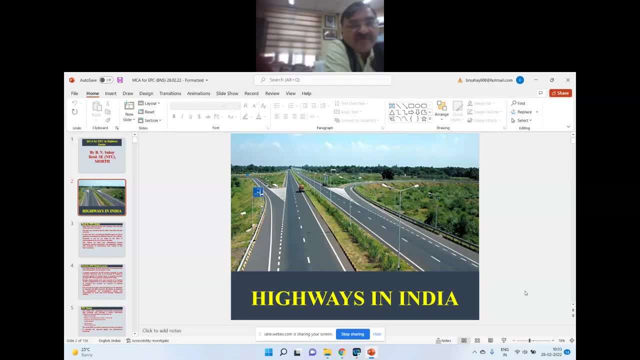 of the contract, contract management And whatever roles are there that should be fulfilled, and it should be fulfilled timely, because time is also very important and crucial. And another thing is we should regularly have a review meeting. If a contract is to be basically, effectively and efficiently to be dealt, I think we should have a regular 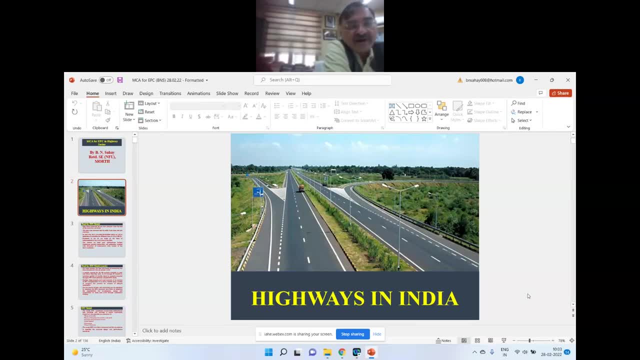 meeting and we should know where we are lacking And timely we should take the corrective measures. So I think all these aspects would be detailedly covered during this training program And I would request all the participants to actively interact with the faculties that have been engaged by IHE And whatever professional 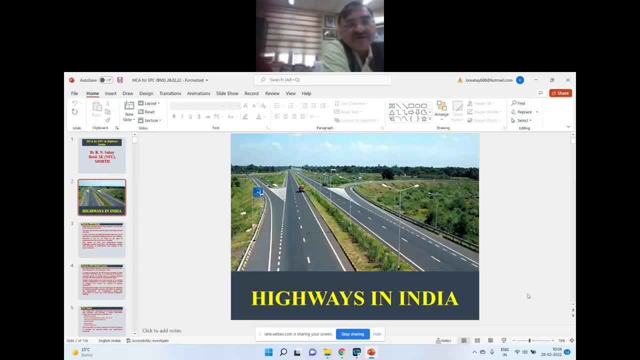 gaps are there or whatever doubts are there in your mind, it should be good, It should be clear and deliberated during this calendar training program And I hope with the upgraded knowledge that you will acquire during this training program, you will be in a better position to deal this subject matter in a efficient and effective. 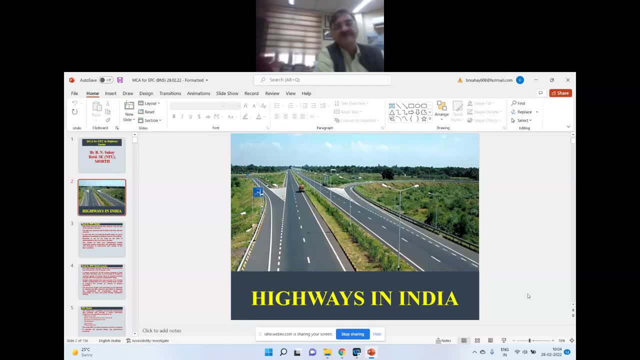 manner. So once again, I welcome you all and thank you very much, Dr R R. Thank you, Dr Eswar. thanks a lot, sir. thank you, sir. now i request today's distinguished faculty bn sahay sir to kindly enlighten on today's topic. sir, sir, please, sir, okay, thank you. 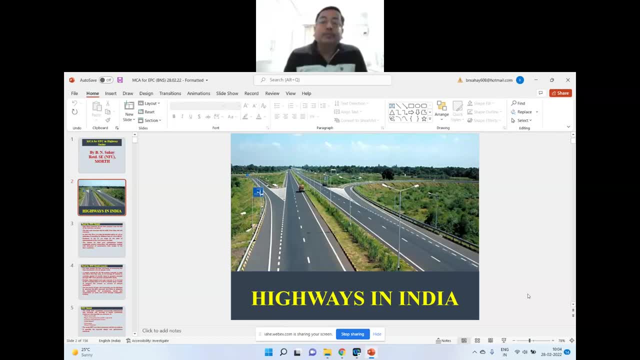 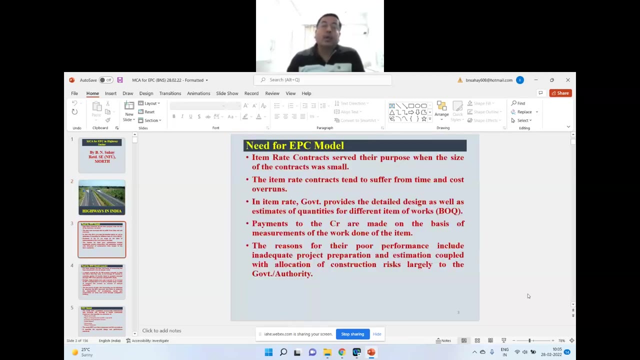 good morning everybody. this is bn sahay, recently retired from ministry of road transport and highway. today our topic is mca for epc in highway sector: why it is needed. why epc model is needed. actually, earlier we were having item rate contracts, and item rate contracts serve their purpose when the size of the contracts were. 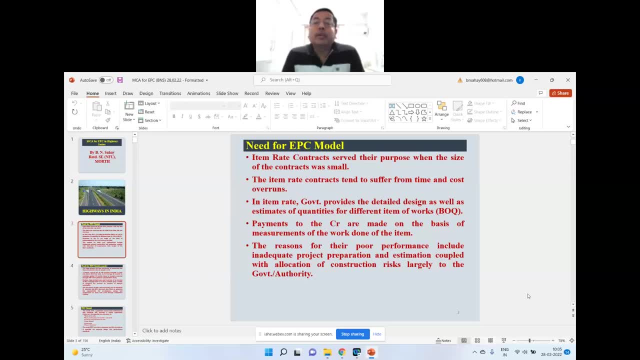 very small. the item rate contracts tend to suffer from time and cost overrun. this is why we switch over to this epc model. there are other things i am just reading out. in item rate, government provides the detailed design as well as estimate of quantity for different item offers. in case of item rate, you will have to prepare dpr. dpr is: 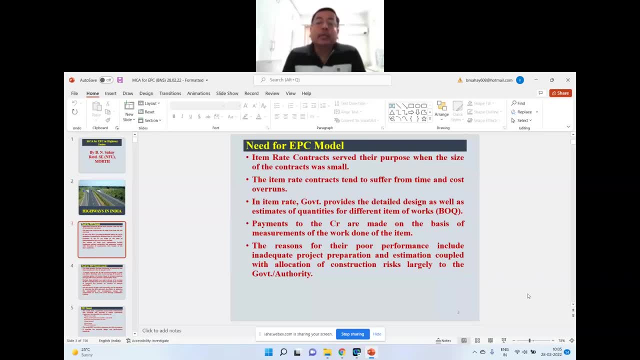 prepared by the authority and then based on the dpr estimates of quantities, that is, boq bill of quantities is prepared and on the basis of this boq tender is floated and the bidders, that is, contractors, bid their tender on the basis of rates and on the basis of lowest rate, we award the work. 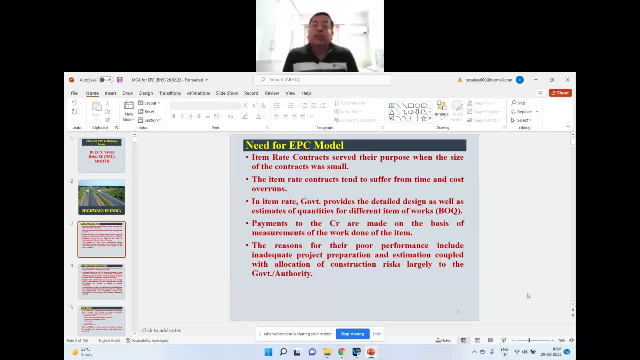 to the contractor. whoever is, l1 will be awarded the work. but design and all the things are done by design estimates, all the things are done by the authority, that is, government body. payment to the contractor are made on the basis of measurement of the work done of the item. 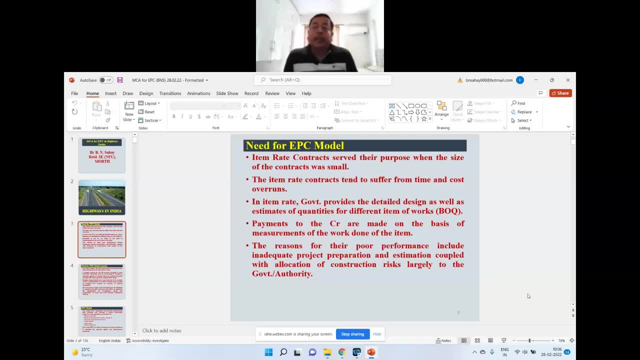 the reason for their poor performance in include inadequate project preparation and estimation coupled with allocation of construction risk largely to the government authority. suppose something wrong has happened. the contractor will tell you that it is your estimate, your design. it is faulty and this is why my structure has failed. so all the risk was with the government. 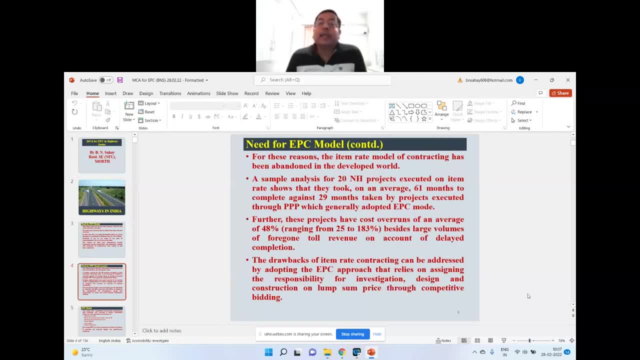 in case of item rate contract, all the data and availability for these examples and option of company a. for these reasons, i tell great model of contracting had been abandoned in the developed world. in the developed countries now this type of item rate contract are no more in. and home a sample analysis for 20 nscale how a. project wasn't done on item rates which so that they took on average 61 months to complete, against 29 months taken by project ETA through PP. the same project months to complete against 29 months in case of PPP, which generally adopted EPC mode. 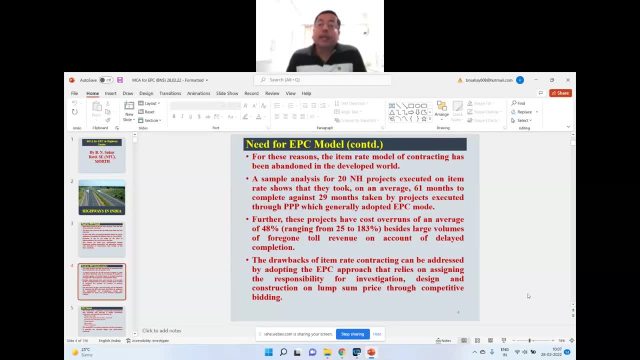 this model, which I am going to discuss Further. these projects have cost overrun of an average of 48%, ranging from 25% to 183%, Besides large volumes of foregone tall revenue on account of delayed companies. Suppose you are delaying your project work. 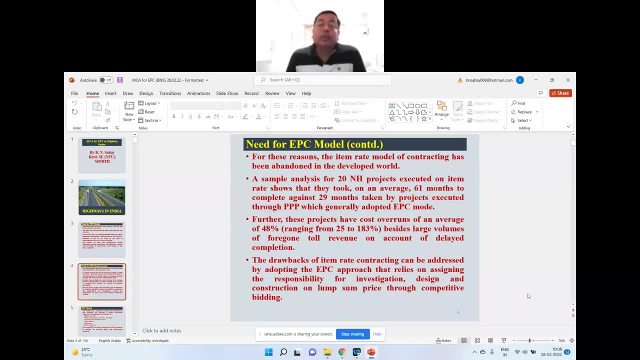 If you are not completing the same on time, you will lose tall revenue. and tall revenue is very much important because our financing model has the tall revenue and tall revenue is the only source from where it is financed. So in case of delay, the concessionaire will suffer and he will not get the benefit. and 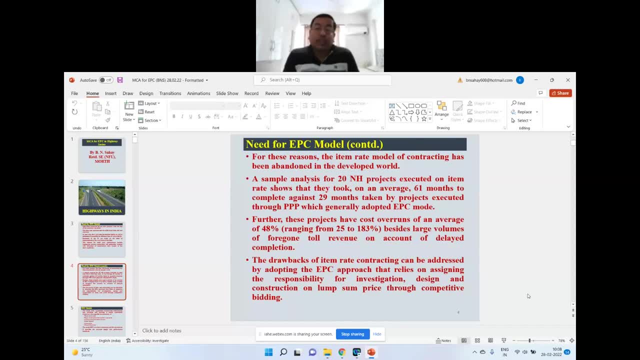 the profit which he has envisaged. The drawbacks of item rate contracting can be addressed by adopting the EPC approach that relies on assigning the responsibility for investigation, design and construction on lump sum price through competitive bidding. In this case, there is no fixed rate. 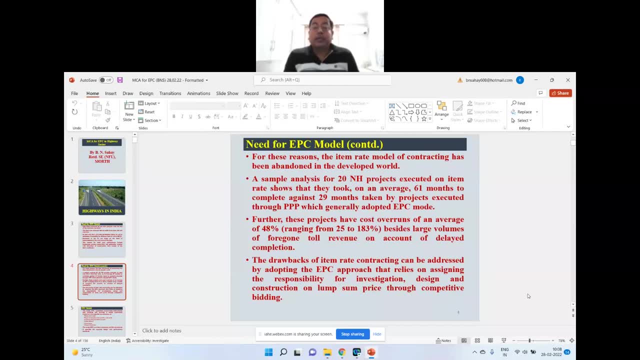 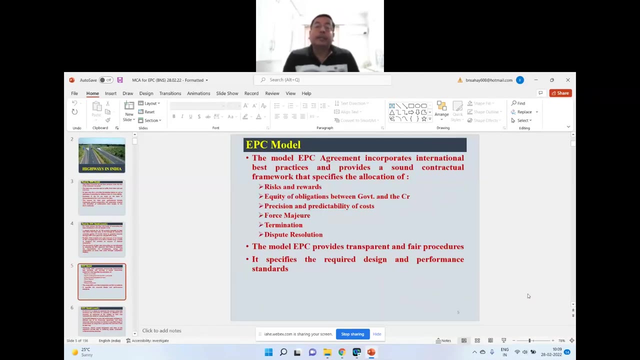 There is no BOQ Here. contractor has to design and on the basis of contractor's design a lump sum contract is agreed between the authorities And the contractor. the model EPC agreement incorporates international best practices and provides a sound contractual framework that specifies the location of risks and rewards. 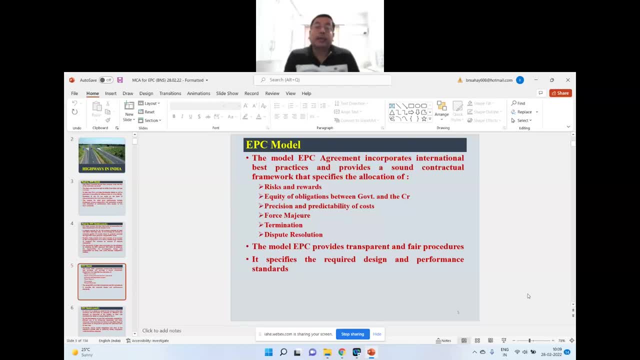 equity of obligations between government and the contractor, precision and predictability of costs. Force measure: Force measure is also very much important. Some of the things are beyond control of contractor as well as authority, And in that case force measure comes into this effect. 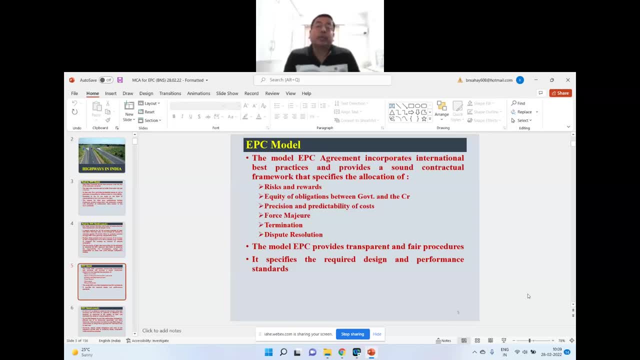 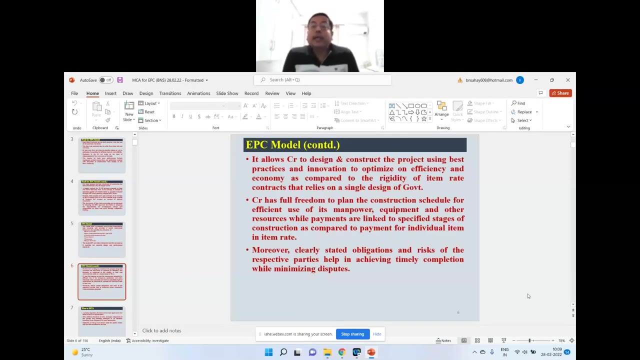 And for this we have made provision in this EPC contract Termination dispute resolution. The model EPC provides transparent and fair procedures. It specifies the required design and performance standards. It allows contractor to design and construct the project using best practices and innovation. 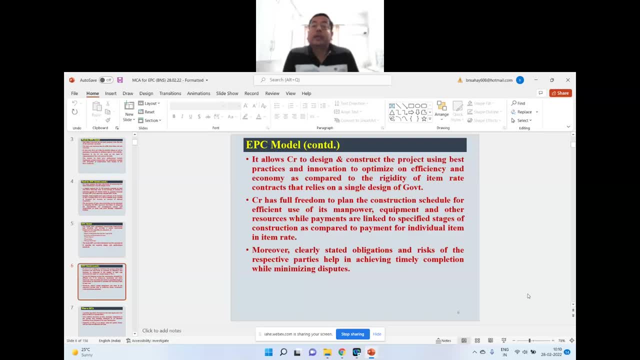 to optimize and efficiency and economy as compared to the validity of item. In case of items, Item rate. you have fixed all the things, So contractor is not having any liberty. But in this case, in this EPC model, contractor has to design, construct using best practices. 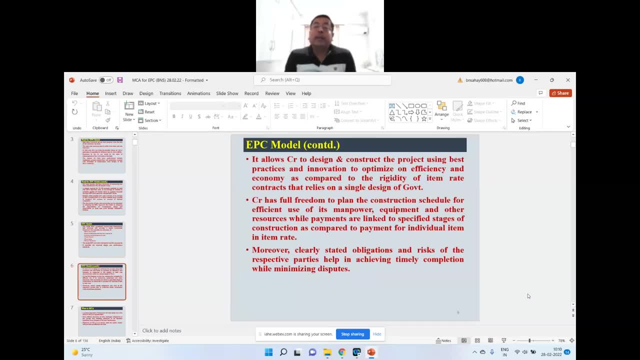 and he may optimize, he may economize the cost. So it is a very good practice that contractor has liberty to design at its own sweet will. He may adopt Indian standard. He may adopt Indian standard. He may adopt Indian standard. He may adopt American standard. 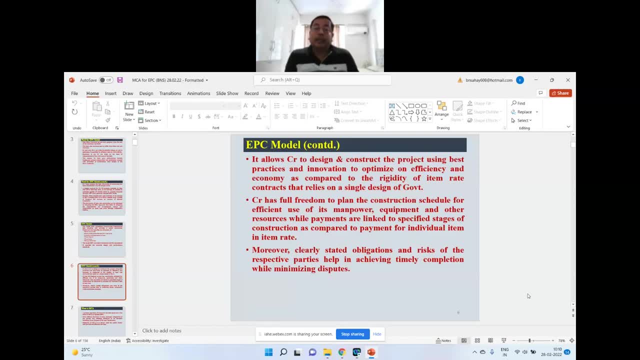 He may adopt European standard, He may adopt US standard, Korean standard, Japanese standard. Whatever he wants he can adopt And based on that, the work can be done by him And the design done by contractor will be approved by authority. engineer. 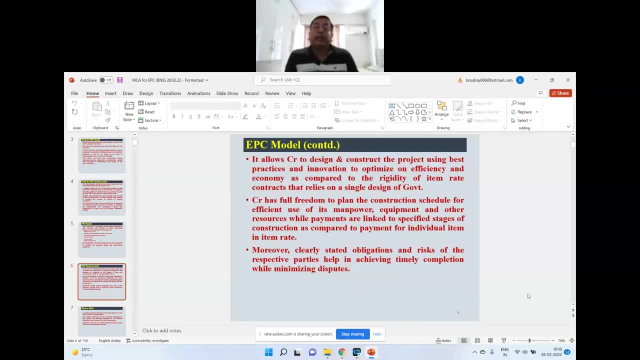 The contractor has full freedom to plan the construction schedule for efficient use of its manpower, equipment and other resources, while payments are linked to a specified amount of money, specified stages of construction, as compared to payments for individual item in item rate. In case of item rate, we measure the quantity Suppose in BOQ, it is 1000 cubic meter and its rate. 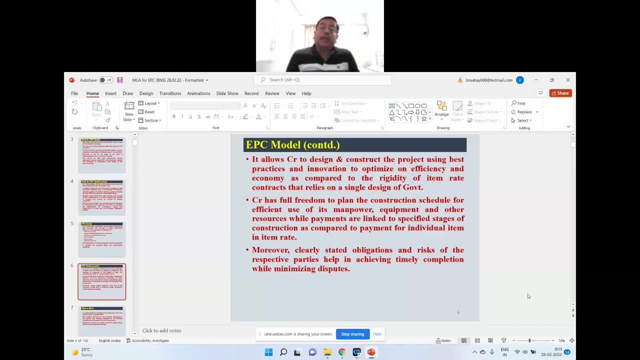 has been quoted by the contractor, and suppose the contractor has executed only 100 cubic meter, then we will pay at that rate by multiplying the 100 with the rate and he will get the payment. But in this case this is not the case. In this case we pay on the stages. Suppose he has. 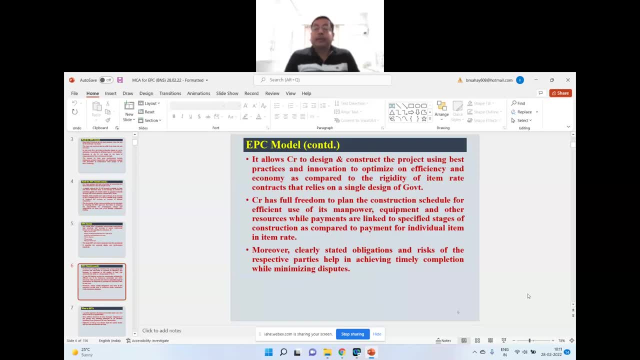 completed five kilometers of road, he will get payment. Everything is defined in terms of stages, not on the item rate. So, moreover, clearly stated obligations and risk of the respective parties help in achieving timely completion while minimizing dispute. Disputes are also minimized. 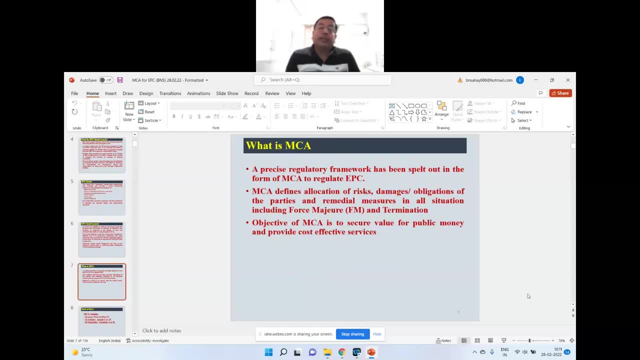 in this case, What is MCA? MCA is a precise regulatory framework and it has been spilt out in the form of MCA to regulate EPC. MCA defines allocations of risk, speak Rebound, incl. May say Disputes and. 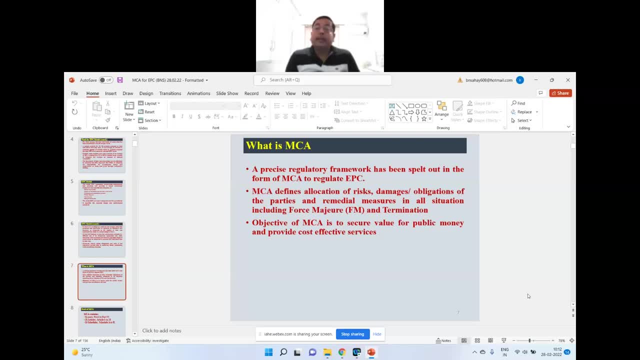 damasitness, obligations of the parties and remedial measures in all situations, including force measure and termination. MCA deals with all types of risks, damage, grav 아이り Fall, complide of whims and afflictions in various areas, and it is defined joining catering. 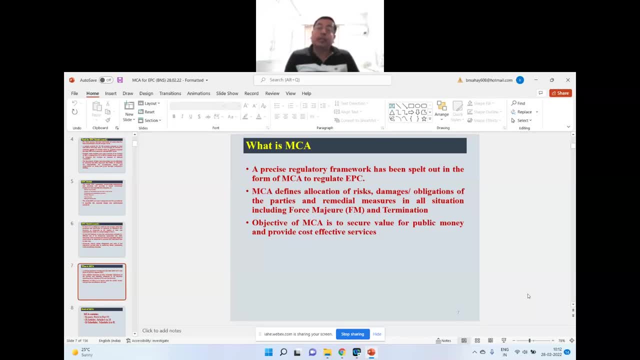 damages, obligations and remedial measures in all situations, including force measure and termination. All the cases have been taken care of and all the things have been incorporated in this EPC model of contract. So it is a very good quality of contract and it is very useful. 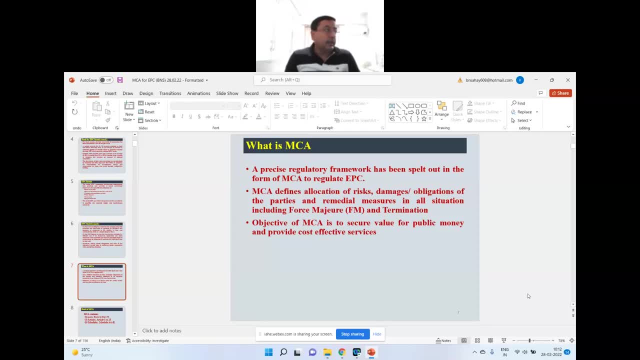 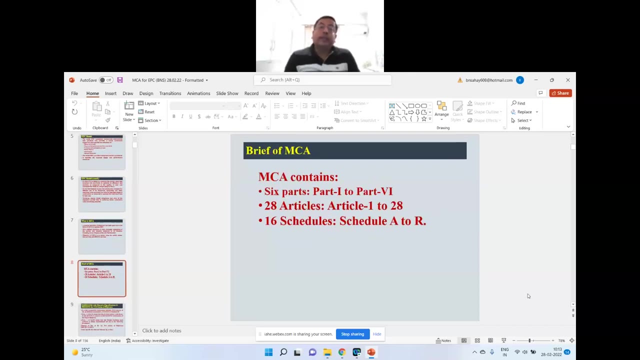 We have been using it for the last- I think, about 10-12 years and it is working in a very nice manner. Objective of MCA is to secure value for public money and provide cost-effective services. This MCA contains six parts, part 1 to part 6, 28 articles, article 1 to 28,. 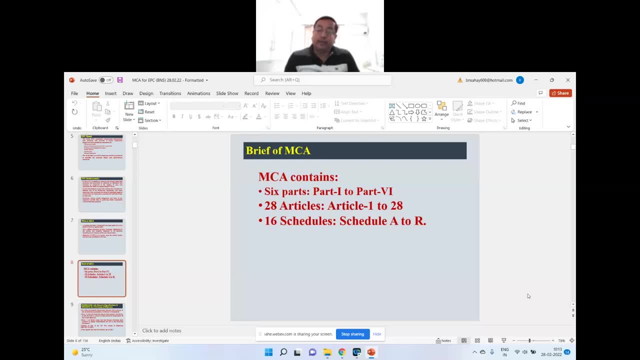 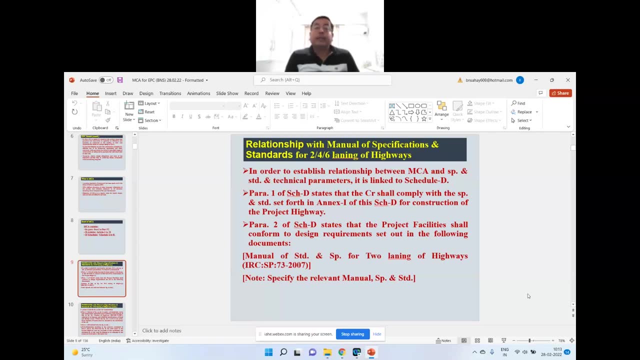 and 16 schedules, schedule A to R. Now, relationship between manual of specification and standard for 2,, 4, 6 lending of high wage. How there is a relationship between manual of specification and a standard for For 2,, 4, 6 lending of the project high wage. In order to establish relationship between 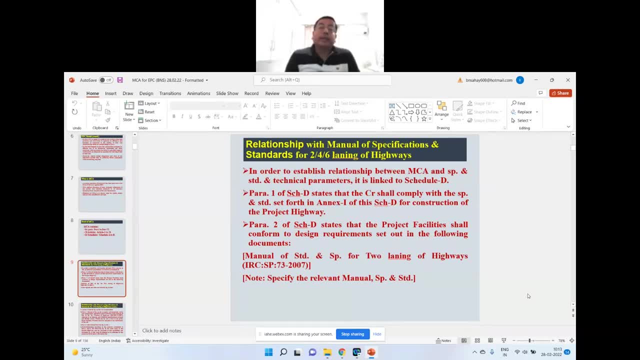 MCA and specification and standard and technical parameters. it is linked to Schedule D. Schedule D is the specification and a standard, as well as deviation in the specification and standard. Suppose you are not having enough land to achieve a radius of 400 meters, which is required. 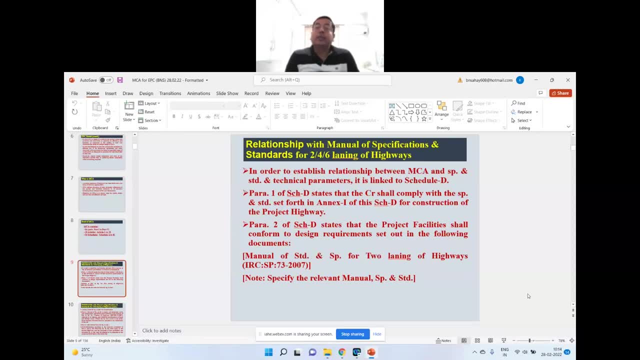 for design a speed of 100 kWh, Then you will have to restrict it in Schedule D and deviation will be pointed out that here the radius of curvature will be only 300 meters instead of 400. that then this is the Schedule D. Schedule D is the specification and a standard, including 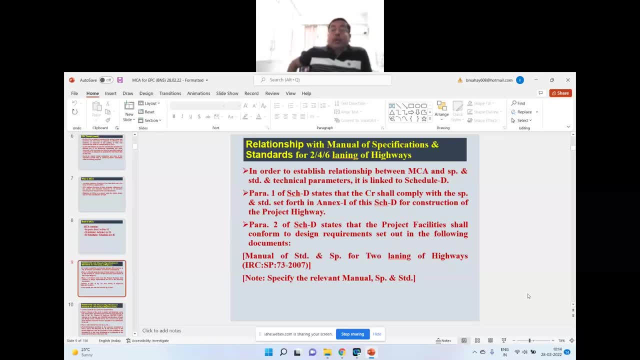 deviations. All the deviations are to be pointed out in Schedule D so that contractor have clear vision that these are the deviations which are allowed in the Design of Speed. Now, if you have developed only 1 speed for the operation of 2,, 4, 6 lending operations, 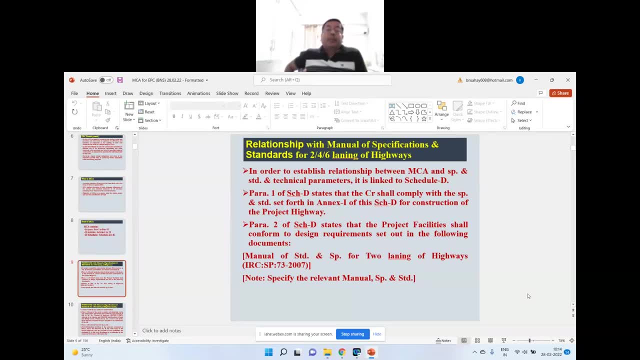 this contract, Para 1 of Schedule D states that the contractor shall comply with the specification and standard set forth in Annex 1 of this Schedule D for construction of the project highway, And Para 2 of Schedule D states that the project facilitated. Para 1 states the: 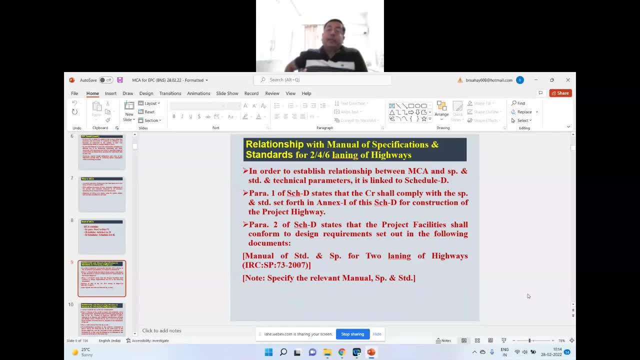 contractor to comply with the specification and standard, and the specification and standard has been set forth in Annex 1 of the Schedule D for construction of project highway, And Para 2 of Schedule D states that the project facilitated shall conform to design requirements set out in. 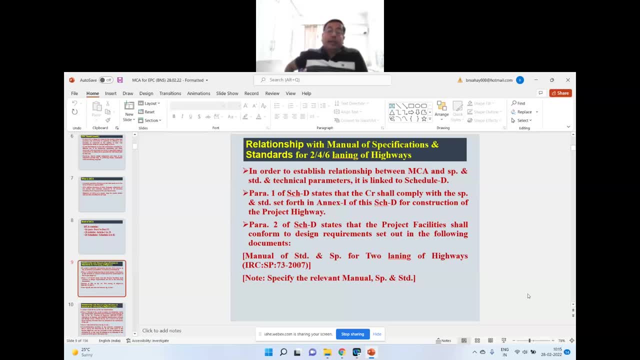 the following document: Now see in a square bracket we have given manual of a standard and a specification for two landing of highways. It is IRC SP 73 2007.. Now 2018 version has already in book, So you can write 2018.. This is the standard I have prepared my presentation based. 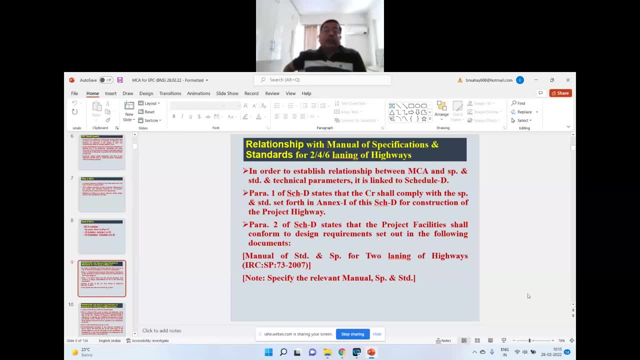 on the standard document, But now you have to change because it is IRC SP 73 2018. in case you want to implement two landing, In case you are going to implement four landing, then another manual will come. It will be IRC SP 84.. So, depending upon your work, 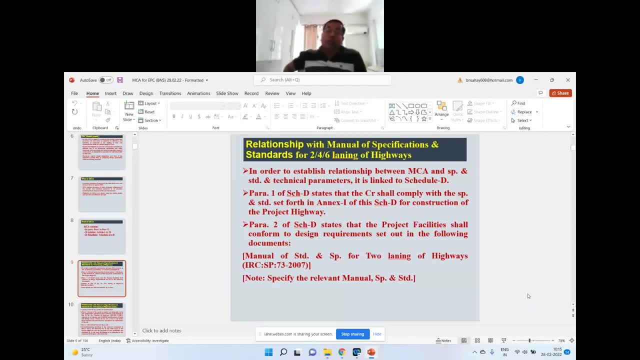 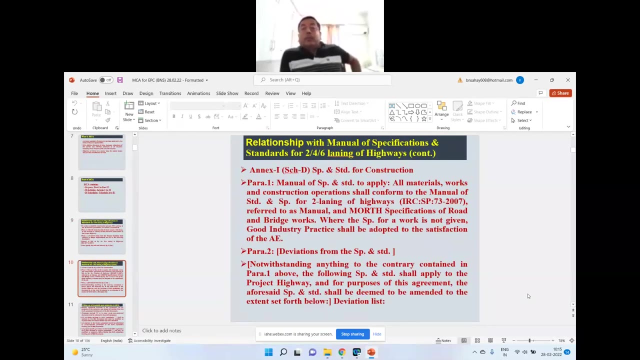 you have to define. this is a square bracket. You have to change it depending upon your suppose. your case is four landing or six landing, then manual will change here and contractor will follow this manual only. Annex 1 of Schedule D- specification and standard for construction. Para 1, manual of a specification and. 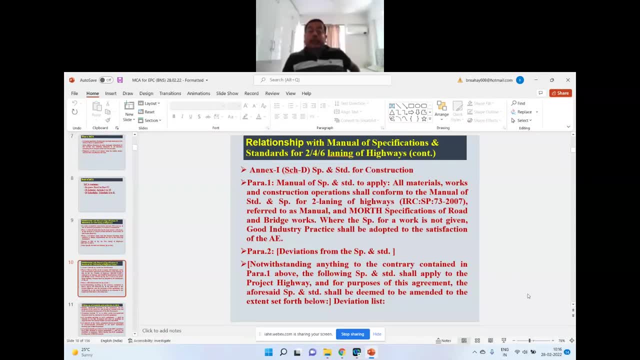 standard to apply. All materials, works and construction operations shall conform to the manual of a standard and a specification for two landing of highways, referred to as manual, and MORTH specification of road and bridge works. What is a MORTH specification for road and bridge works? It is orange book. You, you, popularly it is known as orange book. So 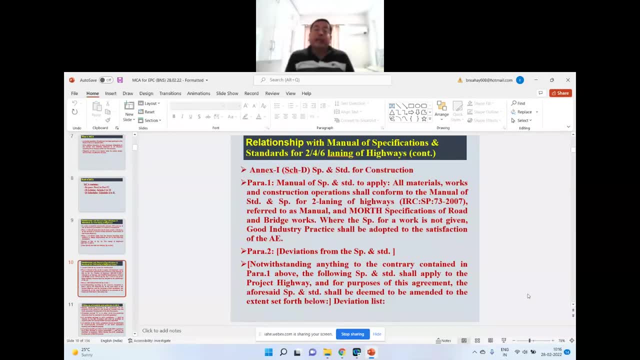 orange book and the manual. both are linked here and the contractor has to design and construct as per these manuals and specification and standard. only Where the specification for a work is not given, suppose some of the specification or any specification is not given in the manual or the 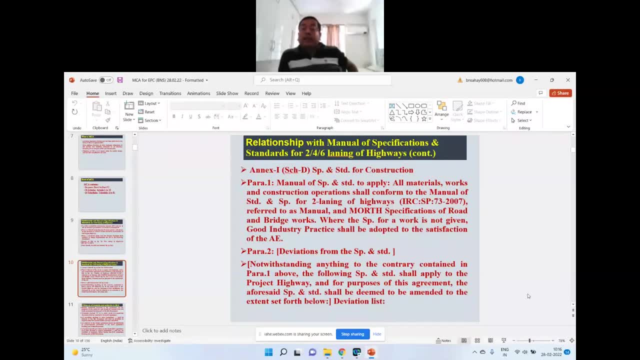 MORTH specification book. Then, in that case, what will be done? Good industry practice shall be adopted to the certification of road and bridge works. Good industry practice shall be adopted to the certification of road and bridge works. Good industry practice shall be adopted to the. 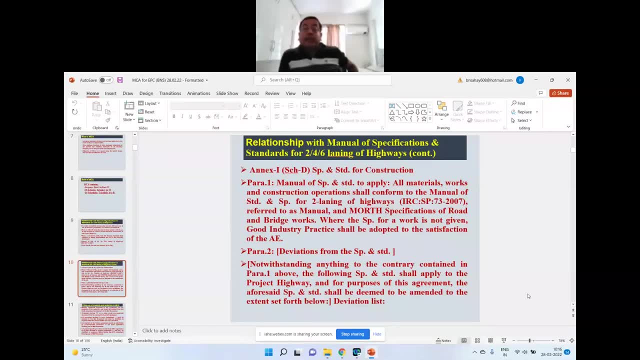 certification of road and bridge works. Good industry practices shall be adopted to the certification of the authority engineer. Please mind it that authority engineer is the most important person, most important authority in case of EPC agreement because it is a third party agreement with the client. 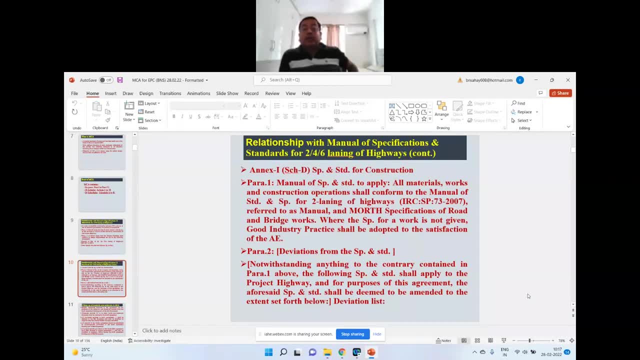 that is authority and he looks after our work And in case of some approval he may seek approval of the authority, but he is looking after our work. So authority without approval of authority, engineer contractor has to do nothing. Para 2: deviation from the specification and standard. Now in Para 2 we point out the 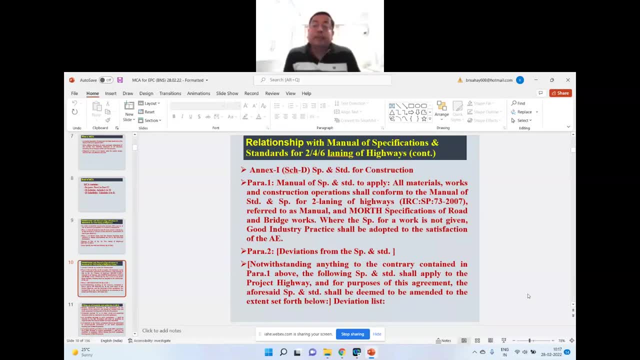 deviation. not withstanding anything to the contrary contained in Para 1 above, the following specifications and standards shall apply to the project highway and, for purposes of this agreement, the aforesaid specification and standards shall be deemed to be amended to the extent set forth below. Now deviation list You have to point out just for example. I already explained that suppose 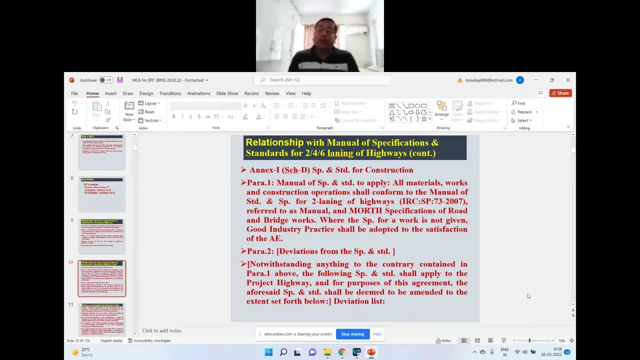 your radius of curvature. you are not having enough land? then you can restrict your radius of curvature from 400 meter to 300 meter. Similarly, a number of things can be deviated from the specification and standard, and all these things are to be listed below. 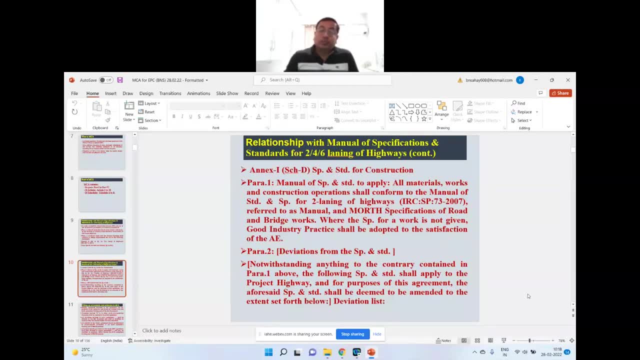 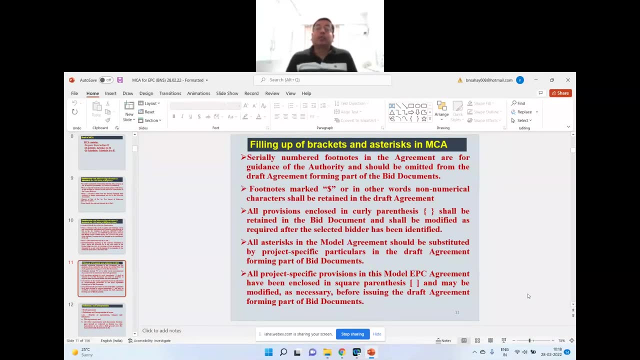 Until and unless you will list it, it will not be amended. Now what is the meaning of these numbered footnotes? or square bracket, curly bracket? this is explained here. Serially numbered footnotes in the agreement are for guidance of the authority and should be omitted from the draft. 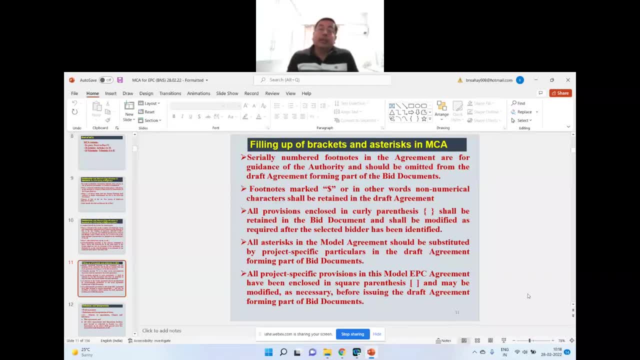 agreement forming part of the bid document. Suppose you will go through the MCA standard MCA, you will find 1, 2,, 3, 4- these type of things are written in footnotes. These are for your guidance. 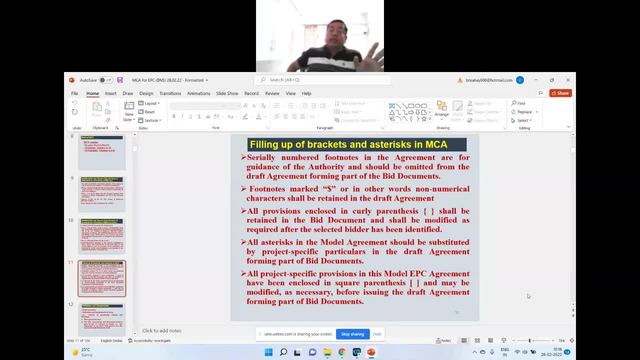 While you are going to float, you can delete it. omit it. Footnotes marked as dollar, or in other words, non numerical character, shall be retained in the draft agreement. These are to be retained. Whatever is written as dollar, marked as dollar two be retained. All provisions. 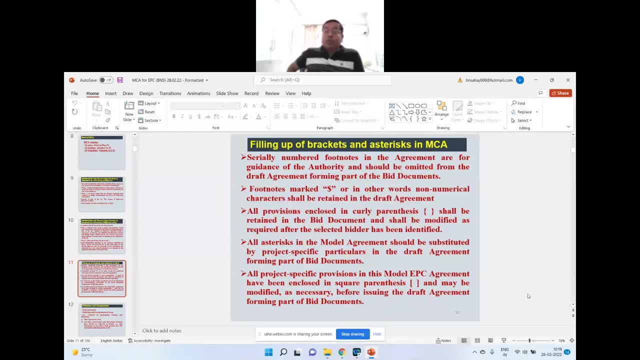 include in curly parenthesis I have shown on the screen. The curly parenthesis will be retained in the bid document and shall be modified as required after the selected bidder has been selected. bidder has been identified. you will. while floating your RFP, you have to include DCA also. DCA is also floated. 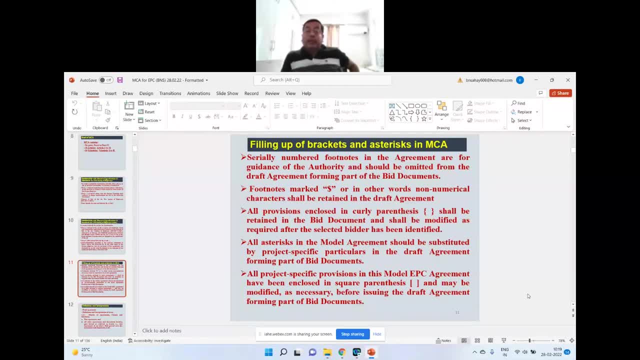 In that DCA. this curly parenthesis will remain there. but when the bid will be finalized and you have got a selected bidder, all the parameters will be filled up here. Before signing the agreement you will have to fill up in the curly parenthesis for the 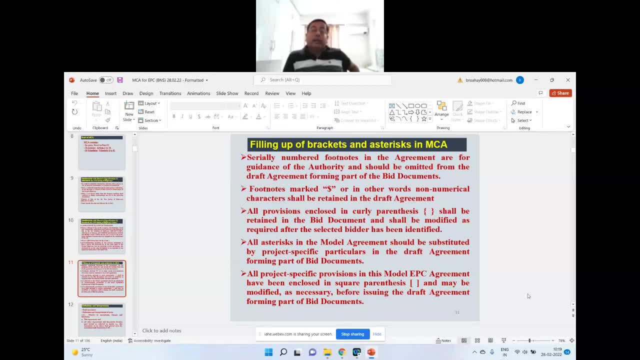 details of the selected bidder. All asterisks, that is star marks, in the model agreement should be substituted by project as specific particulars. Project as specific particulars are given with star marks in the draft agreement form part of bid document, So you have to modify it from this NH, from kilometer this, to this of this NH. 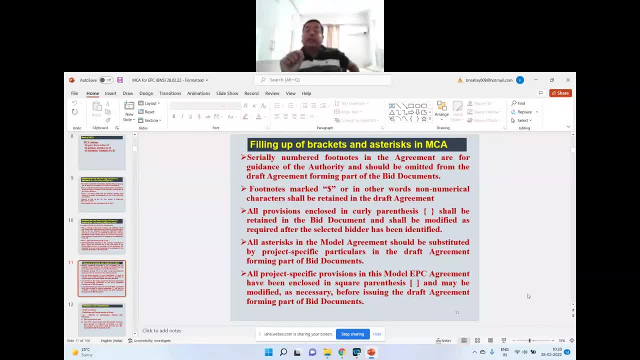 All the things are given in a star. Now you have to fill That is it: NH 25 and from kilometer 135.123 to 185.546.. So this has to be filled. These are all asterisks, that is, star marks, and you have to fill up. 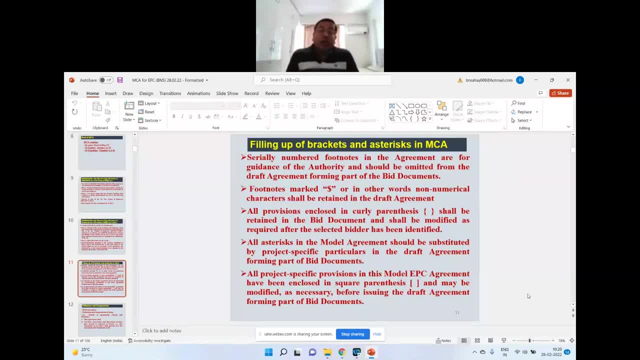 It is: project as specific particulars. All project as specific provisions in the model EPC agreement have been enclosed in a square bracket and may be modified as necessary. Now, project as specific provisions have been filled. These provisions have to be filled in a square bracket and may be modified as necessary. before. 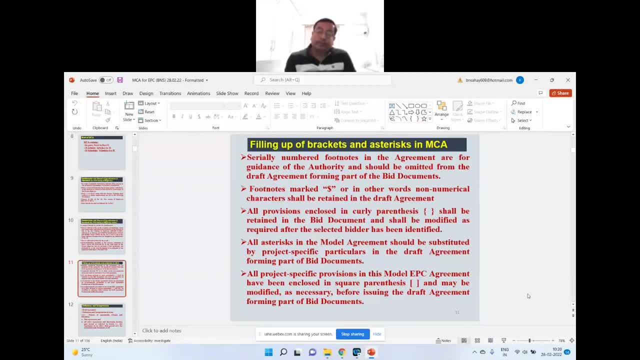 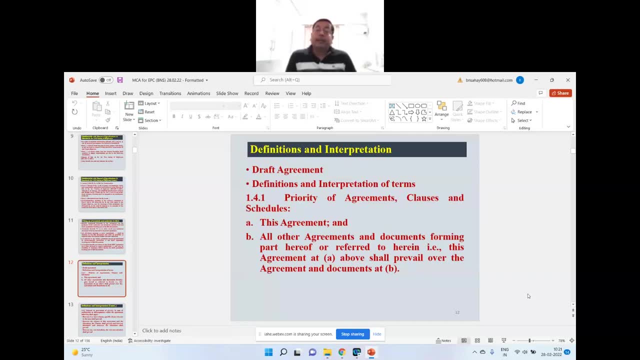 issuing draft agreement forming part of bid agreement. Now coming to definitions and interpretation. Draft agreement, Definition and interpretation of terms, Priority of agreement, Clauses and schedules. This agreement and all: A is this agreement and B is all other agreement and documents forming part of bid agreement. 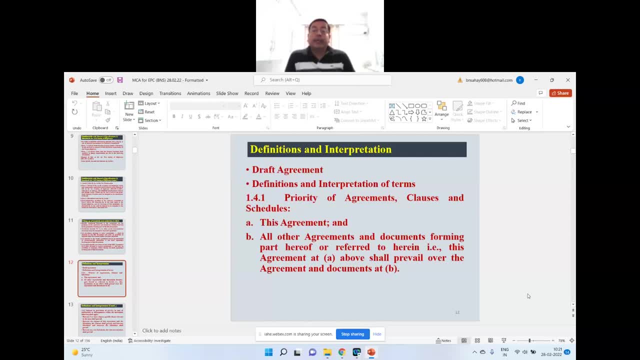 Hereof or referred to herein, that is, this agreement at A, That is, the agreement above, shall prevail over the agreement and documents at B. All other agreements which are forming part of this agreement will not prevail. This agreement will prevail over the B. All the things in A will prevail over items in 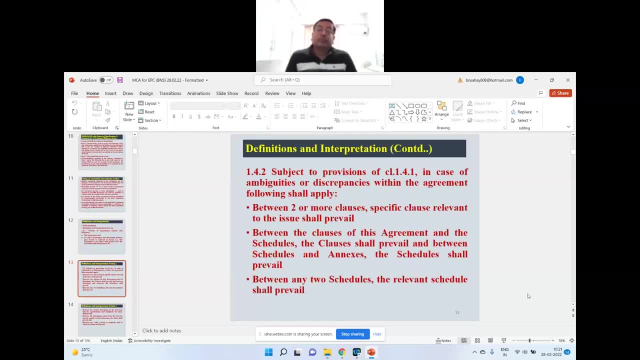 B. Definition and interpretation continued subject to provision of clause 1.14.13.. In case of ambiguities or discrepancies within the agreement, following shall apply: Between two or more clauses, a specific clause relevant to this issue shall prevail. Suppose you are having some ambiguity, that two clauses are having different meaning. 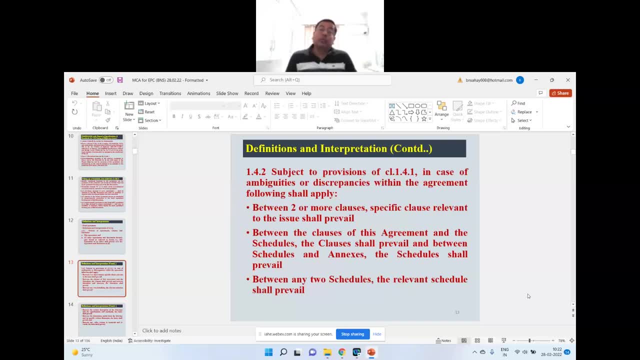 Then the specific clause which is relevant to the issue shall prevail. Between the clauses of this agreement and the schedule- Suppose there is some confusion between the agreement and the schedule, Then agreement will prevail over schedule. The clauses shall prevail, and between schedules and annexure, schedule shall prevail. 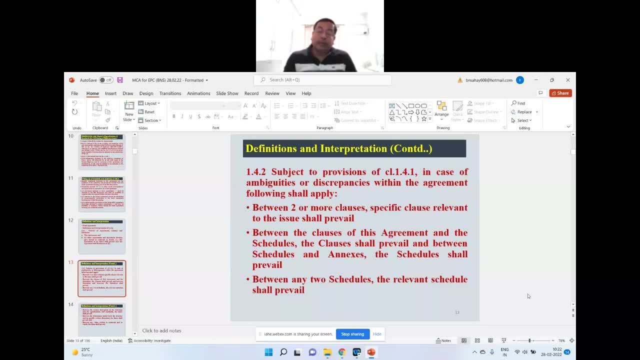 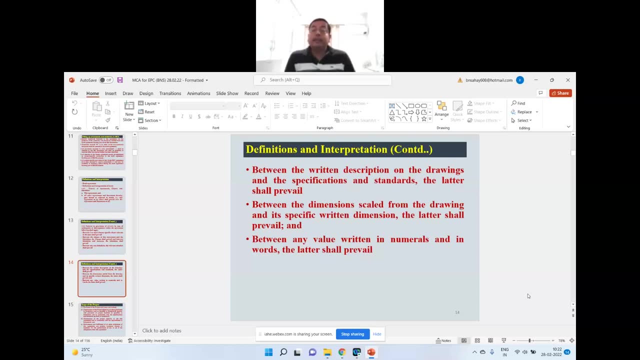 Between any two schedules, the relevant schedule shall prevail. Between the written description on the drawings and the specification and standards, the latter shall prevail. That is, standards and specification will prevail over written description. Between the dimensions scaled from the drawings and its specific written dimension, the latter shall prevail. 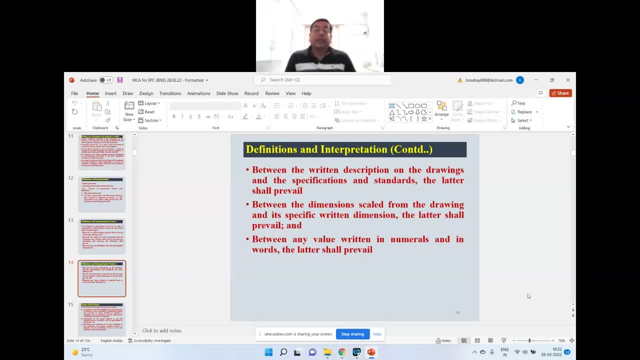 That is, a specific written dimension shall prevail. Between any value written in numerals and in words, the latter shall prevail, That is, those written in words will prevail over those written in numerals. These are the priority of document. This needs to be defined in order to have clarity in case of dispute with the contractor. 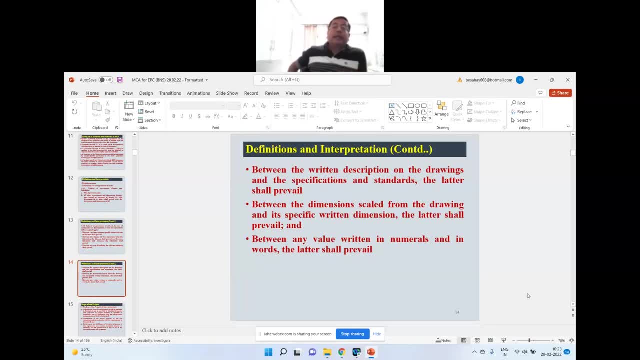 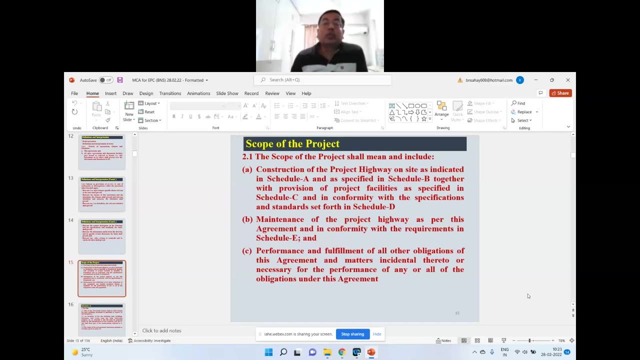 This will be very much Helpful, because everything is well defined and even arbitrator or court will also tell you that this has been written. So agreement will prevail over schedules. So everything is clarified here. Now, coming to the scope of the project. You have to define the scope of the project. 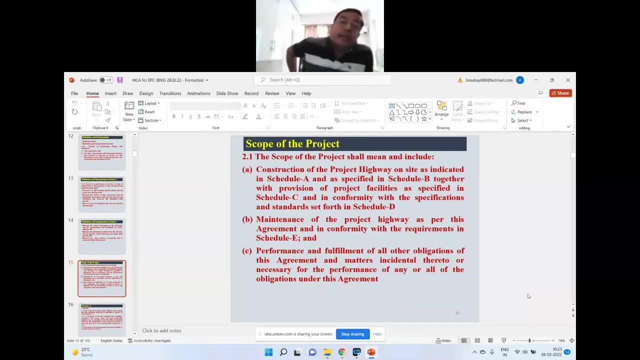 It is very much important because your contractor must understand what he has to do, and whatever he has to do must be mentioned in the scope of the project, must be mentioned in the scope of the project. The scope of the project shall mean and include construction of the project highway on site as indicated in Schedule A and as specified in Schedule B, together with provision of project facility as specified in Schedule C and in conformity with the specification in the standard set forth in Schedule D. 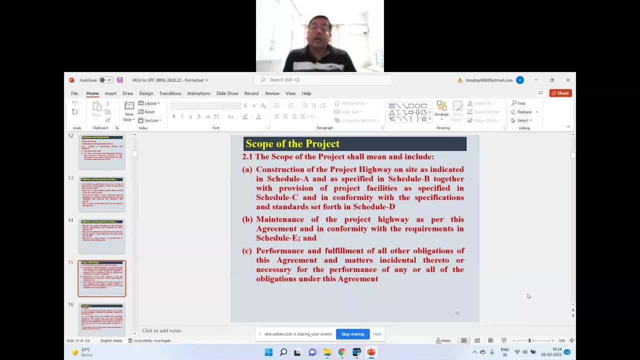 Here understand that this is very much important. How a scope has been defined: construction of the project highway on site. What is site is indicated in Schedule A. You will go to Schedule A. you will find that it is single lane road. Its carriageway width is this, its land available is this And what you have to do. 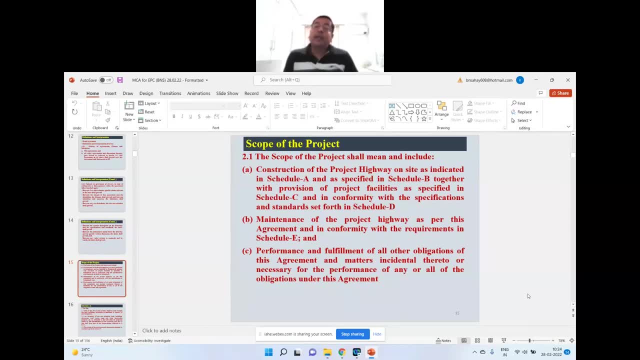 what the contractor has to do is defined in Schedule B. What are the modifications? Suppose a single lane road is there and it has to be converted into four lane. Then in Schedule B it is mentioned that the road has to be widened into four lane. Similarly, suppose ten structures. 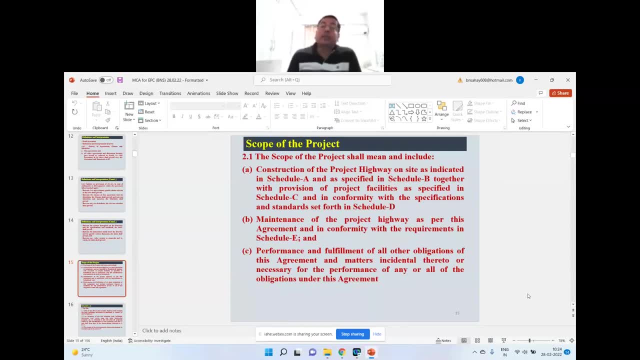 are to be retained or only widened and ten new structures are to be constructed. All these things need to be well defined in Schedule B, with tables, so that contractor must have clarity. So Schedule B defines the quantum of work for the highway. What is to be done? Four lanes needs. 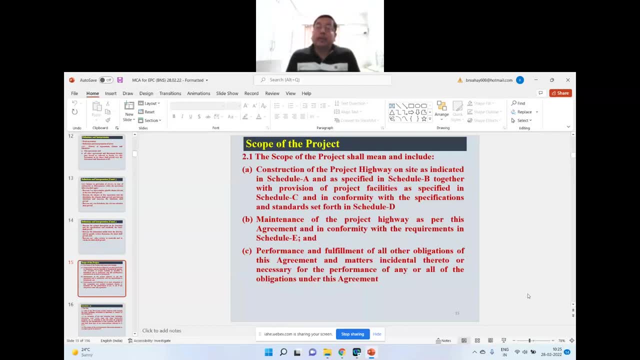 to be done. Ten new structures is to be done. Ten new structure needs to be done. Ten space structure needs to be done. Ten new structure needs to be done. Ten new city structures must be done. Ten structure means a bzw. a fully staffer is required for each one. The right way. 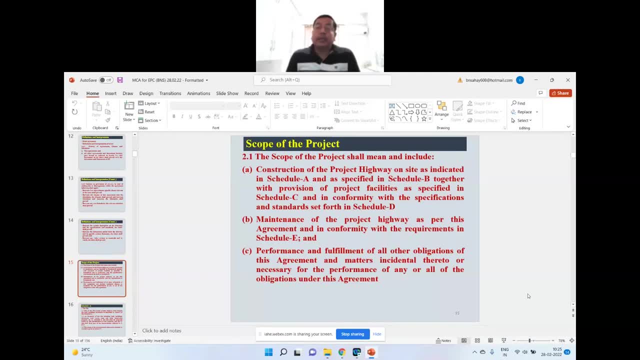 are to be widened, two ROV has to be constructed. everything is to be written in Schedule B. Now Schedule C: project facilities: Project facilities. I will come to Schedule C later, but Schedule C are project facilities: tall plaza, highway, medical, airports. there are. 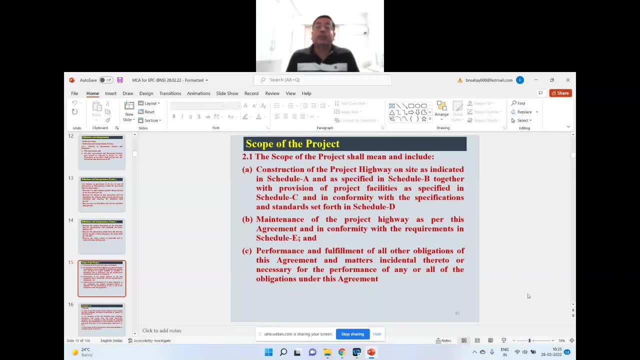 many things, all the things, all type of facilities come under Schedule C And in the last, in conformity with the specification and standard set forth in Schedule D. I have already dealt that. Schedule D is the specification and standard and their manual of specification and standard. 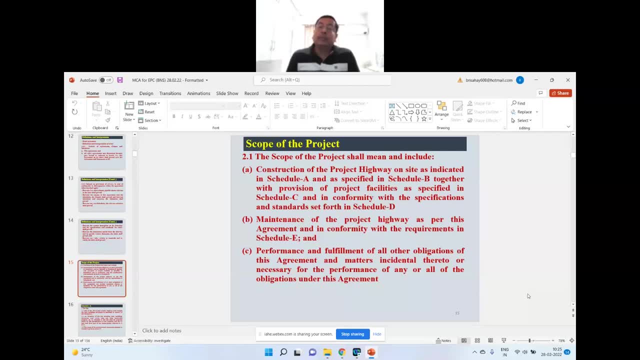 has already been included, linked along with MORTH specification for standard highway and bridge board. So all the things, including deviations, are mentioned in Schedule D and contractor has clarity that he has to follow the standard. So these specifications and standard and these deviations, all these things are defined in 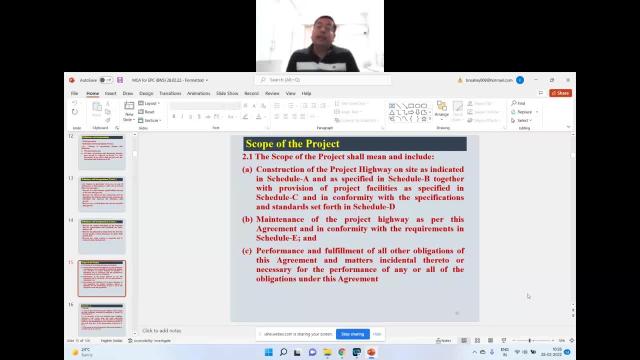 Schedule D. So this part A is very much important- that construction of the project highway on site, as indicated in Schedule A and as specified in Schedule B, together with provision of project facilities as specified in Schedule C and in conformity with the specifications and standards set forth in Schedule D. 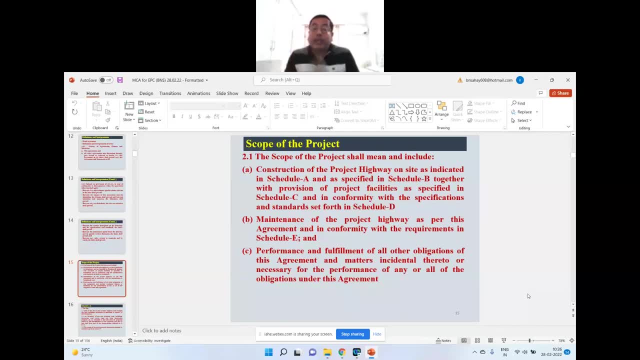 Now, second B point is construction Maintenance of the project highway. how maintenance of the project highway will be done: Maintenance of the project highway as per this agreement and in conformity with the requirement in Schedule E. In Schedule E we have already defined what type of maintenance has to be. 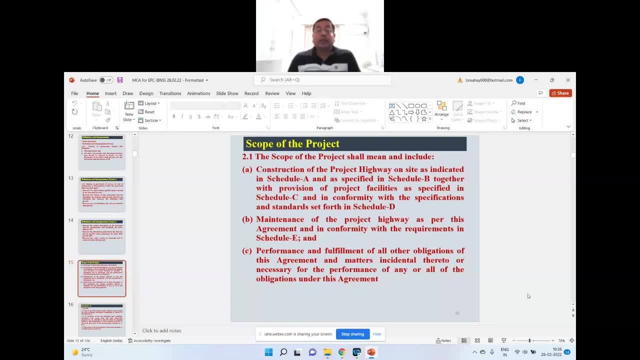 done in what time? Timeline is also defined in Schedule E, and so all the things are linked. Now construction will be done in part A, everything is written, and in B, maintenance will be done by the contractor in conformity with the requirement of Schedule E. 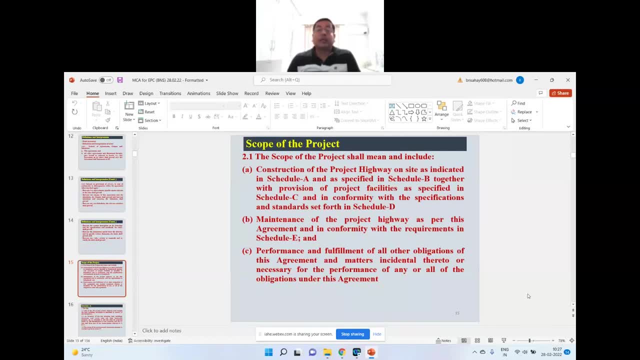 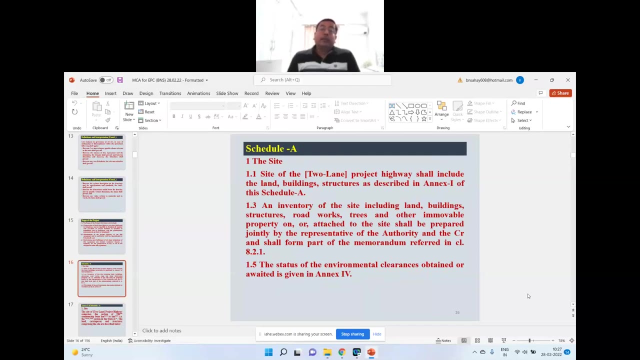 And C. C is performance and fulfillment of all other obligations of this agreement and matters incidental thereto or necessary for the performance of any or all of the obligations under this agreement. Now, what is Schedule A? The site, As I already explained, site of the two-lane, suppose your project highway is two-lane with 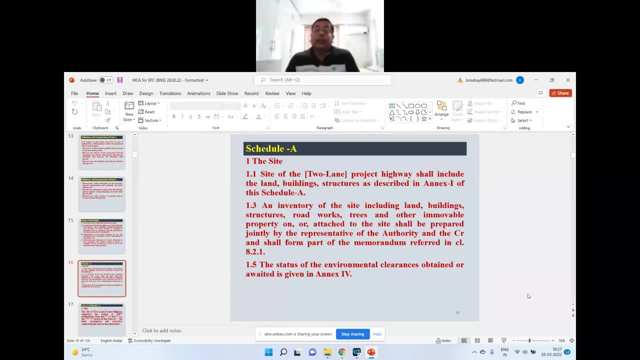 pep soldier, then site of the project. you will have to fill up here two-lane or four-lane or six-lane. However, in the case you have to now, I have mentioned in our square bracket two-lane. 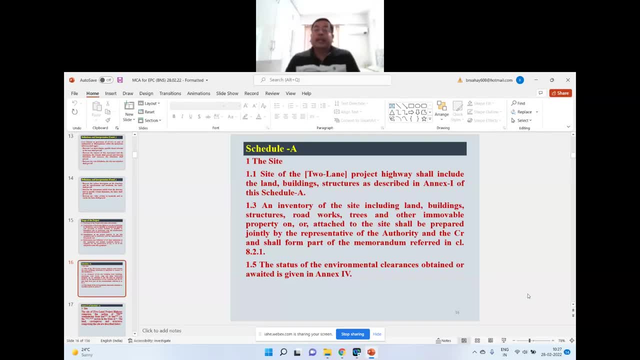 it means the contractor has to construct the road. two-lane Site of the project highway shall include the land building structures as described in Annexer 1 of this Schedule A, An inventory of the site including land buildings structures. 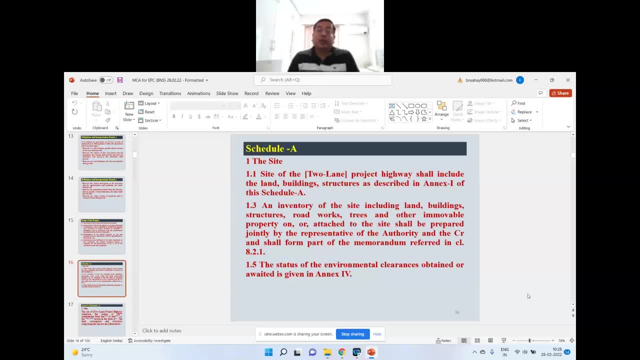 roadworks, trees and other immovable property on or attached to the site shall be prepared jointly by the representative contractor, The representative of the authority and the contractor and self for part of memorandum referred in clause 8.2.. A memorandum is prepared based on joint survey, joint inspection of the site and the inventory. 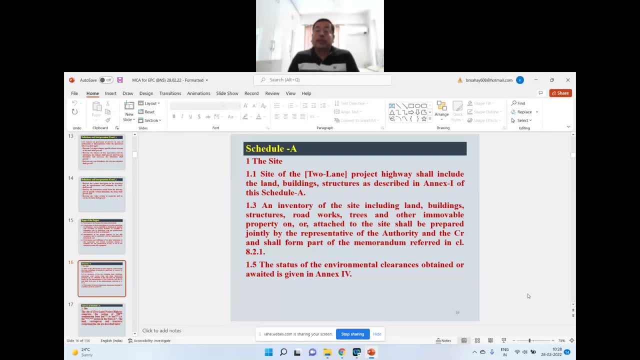 of site, including land, building structures, roadworks, trees and other immovable property which are at site, will be prepared. So it is a joint survey And this will form part of memorandum mentioned in clause 8.2.1.. 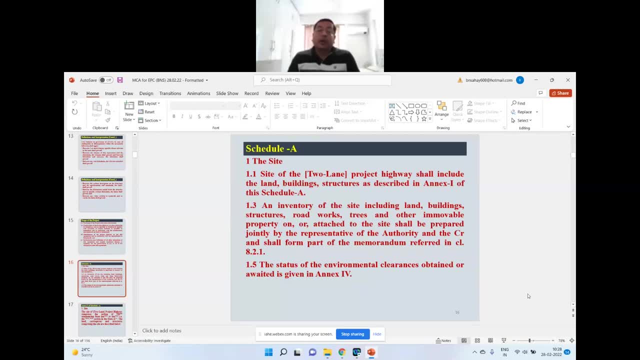 The status of the environmental clearance obtained or awaited is given in Annexer 4.. In Annexer 4, you have to define that out of the 100 kilometer we have already obtained environmental clearance in 90 kilometer and 10 kilometer will be given within 60 days. 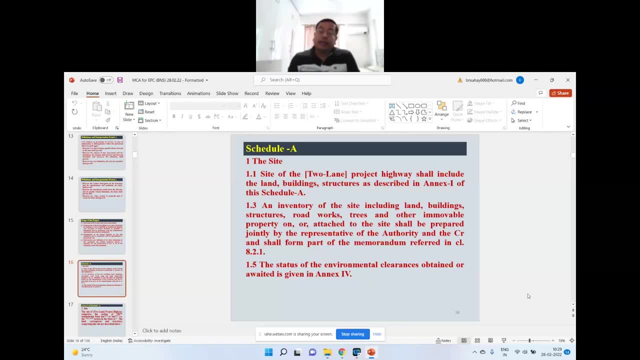 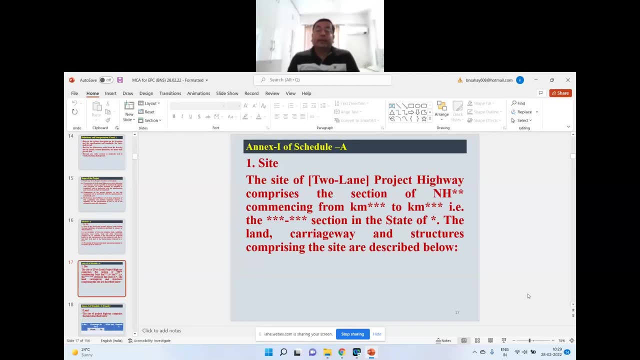 of appointed date. So everything has to be retained in Annexer 4 regarding environmental clearance. Thank you, Thank you, sir. Now site Pardon. The site of the two-lane project highway comprises the section of national highway. You have to mention national highway. 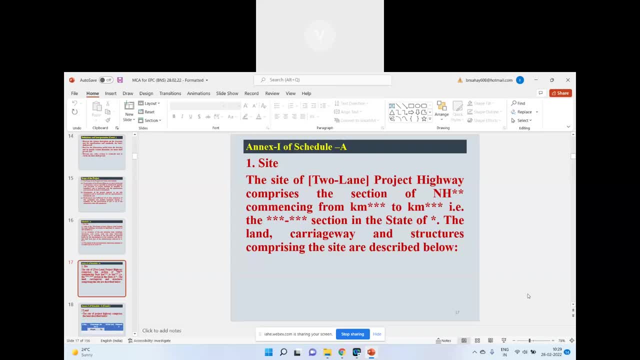 Suppose it is NH 25,, you will have to mention NH 25,, commencing from this kilometer to this kilometer. All star marks are to be filled by you before floating this agreement along with RFP. That is this much section. 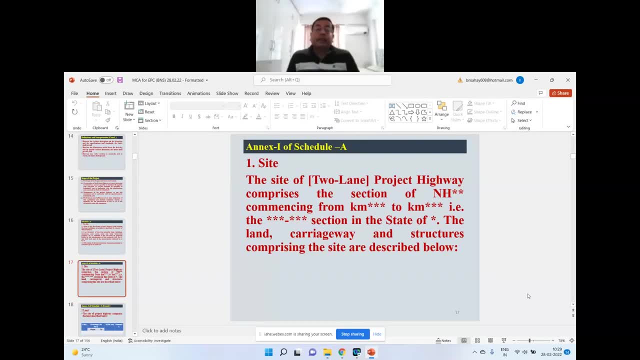 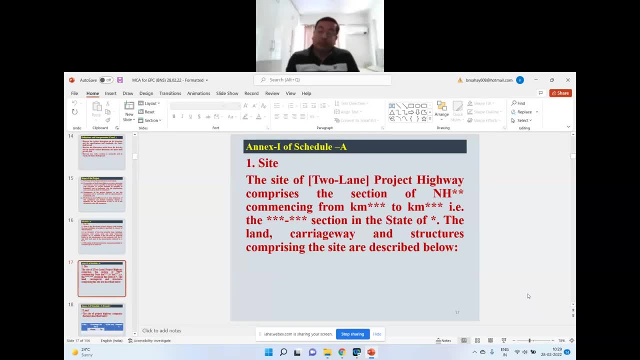 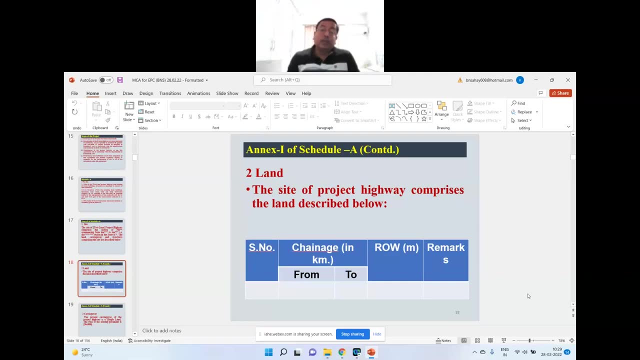 The land, carriageway and restructures comprising the site are described below. The site of the project highway comprising the land described below. Serial number: change in km from this change to this change ROW level you will have to mention. 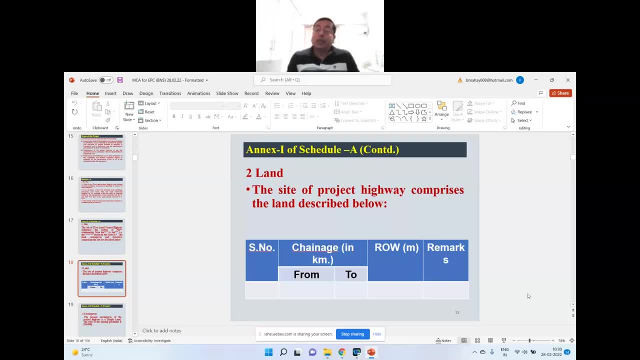 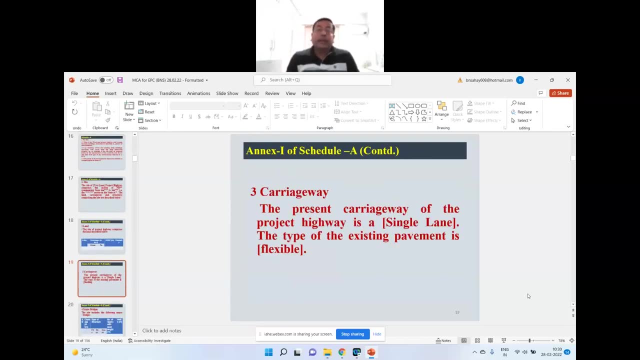 Here 18 m, here 22 m, all the things And along with remarks. In case you are having any remarks, you will fill up here. Carriageway: The present carriageway of the project highway is a single lane. 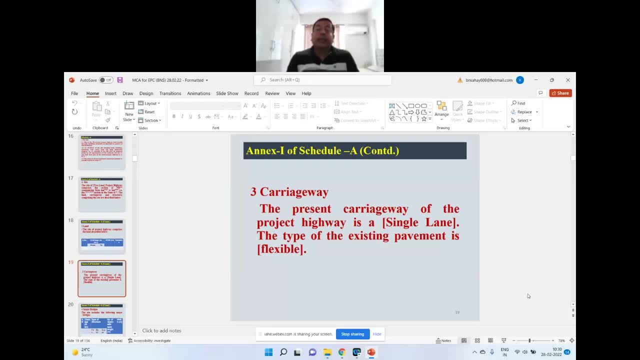 Suppose your project highway is presently single lane and it has to be converted into two lanes, Then here- single lane- you will have to mention. The type of the existing pavement is also to be mentioned. Suppose the existing pavement is rigid pavement. you will have to fill up here: rigid. 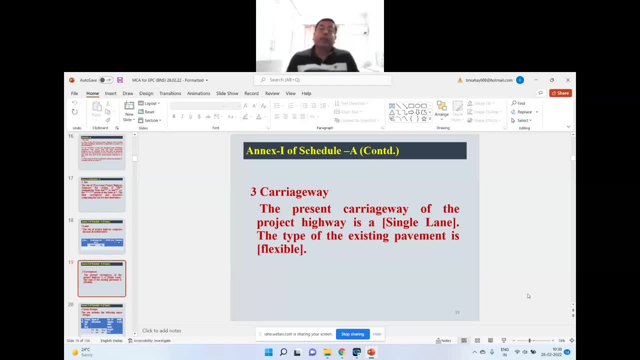 Instead of flexible, which I have Filled up. so in case of flexible, you will have to fill up flexible. in case of rigid, you will have to fill up rigid pavement. Similarly, we will have to define major bridges. The site includes the following major bridges: 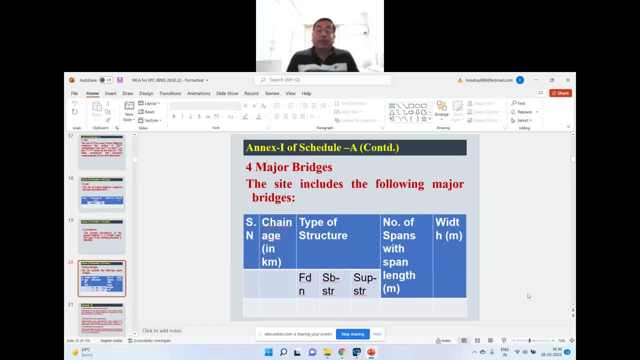 Serial number change. type of structure: foundation, sub structure, superstructure. number of spans with a span length. Suppose your bridge is having four span of 30 m each. then you will have to mention here: and width. What is the width of the bridge? 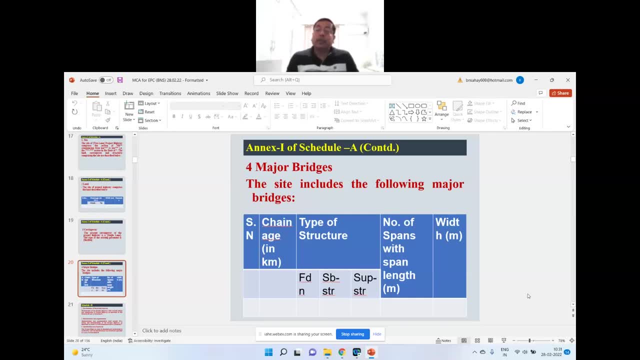 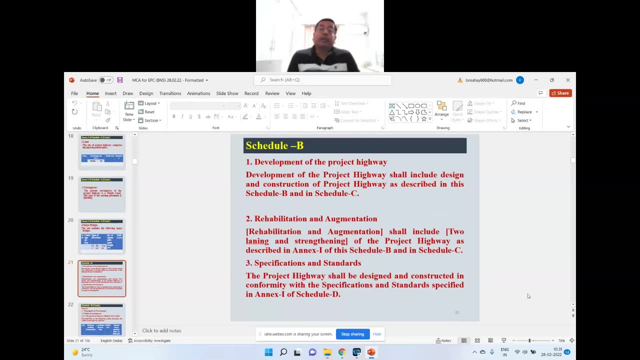 Suppose it is 14 m, then you will have to mention here 14 m. Now schedule B: Development of the project highway- Development of the project highways that include design and construction of project highway as described in this schedule B and Schedule C. 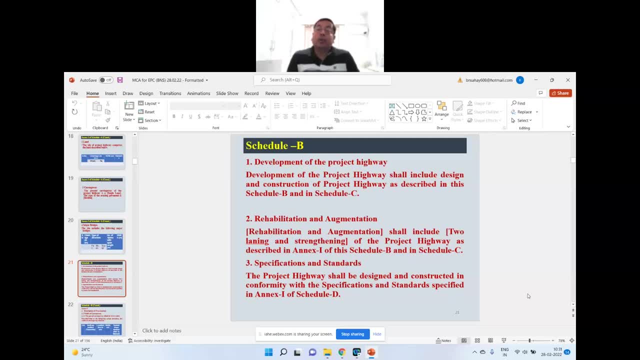 I have already explained that whatever you have to got done from the contractor has to be mentioned in Schedule B and Schedule C, Because Schedule B Is the modification required in the existing highway and Schedule C is the project facility. So you have to very carefully define each and every item in Schedule B and Schedule C. 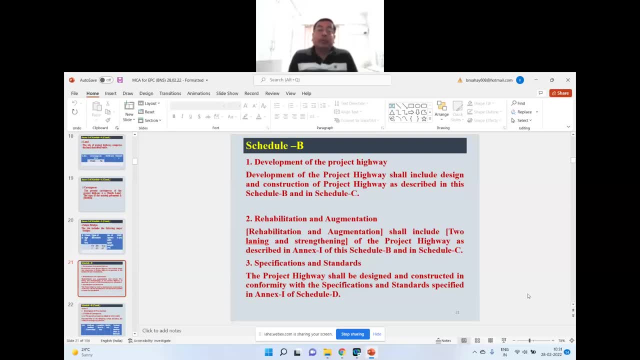 Now suppose some rehabilitation and augmentation is also to be done, then that has also to be defined. Rehabilitation and augmentation shall include two: learning and strengthening of the project highway, as described in Annex R1 of the Schedule B and Schedule C Now coming to Establishment. 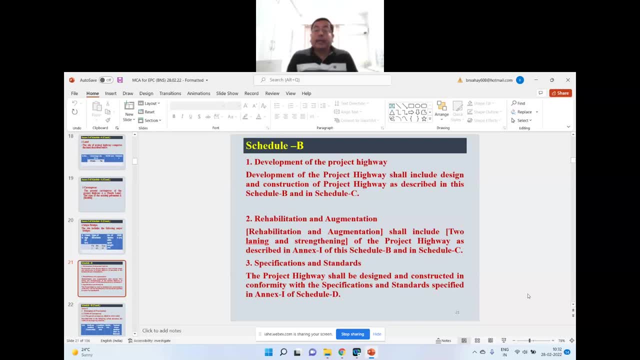 Specification and Standards. The project highway shall be designed and constructed in conformity with the specification and standard specified in Annex R1 of Schedule D. We are just linking it that they have to follow Annex R1 of Schedule D and in Annex R1 of Schedule D. 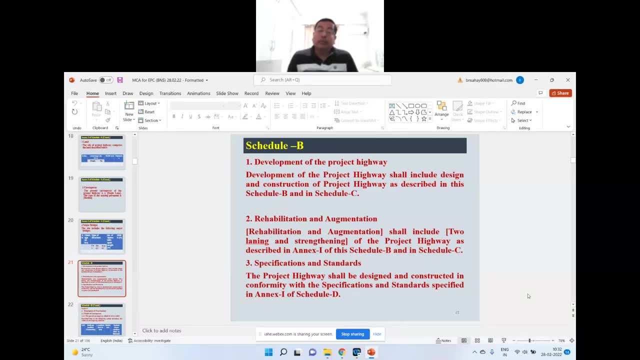 What you have written. You have written manual, Manual of two-lanning, four-lanning or six-lanning, whatever it is, And the What you have to do Now: description of two-lanning or four-lanning, whatever the case may be. 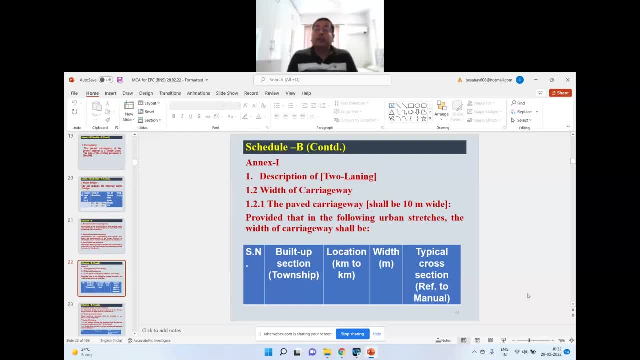 Without carriageway, the paved carriageway shall be 10 meters. In case of two-lanning with paved soldier, we are having 10 meter wide paved carriageway, Provided that in the following R1 stages Suppose in a span of 100 kilometer length. 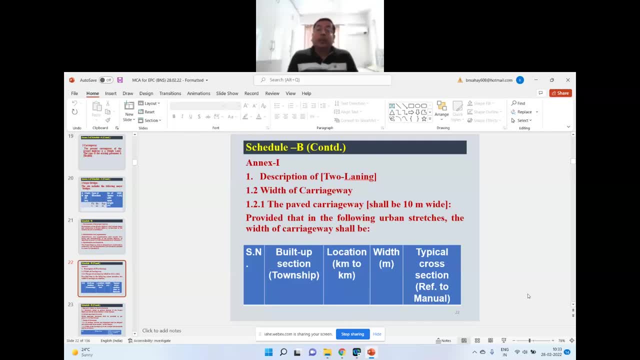 There may be five townships And in that township you may not have much space. Then you have to build some other type of typical cross-section. So these are defined here: Serial number, built-up section, township, location, from kilometer this to this, and width. 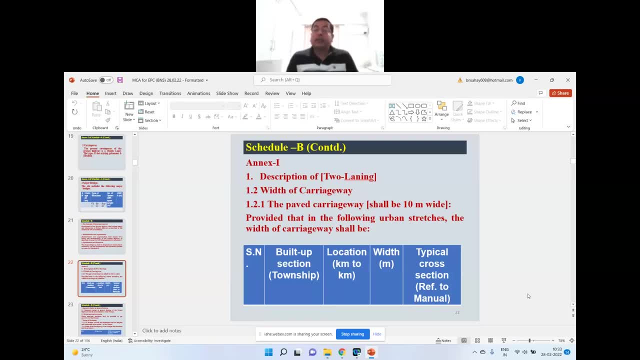 What is the width of the road and typical cross-section referred to manual. Which type of typical cross-section is to be adopted as per the manual You have just to Mention? Suppose 7.3.2 of the manual means a typical cross-section mentioned in 7.3.2 will be followed. 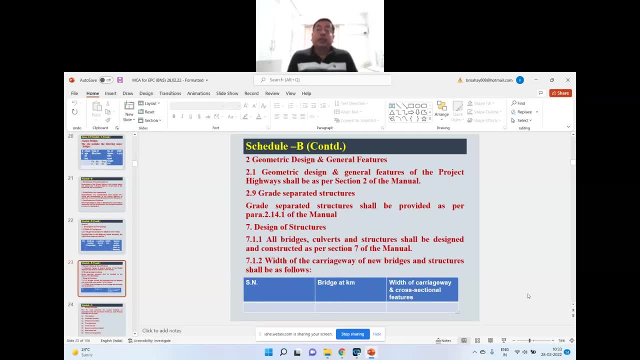 Geometric design and general features. Geometric design and general features of the project highway shall be as per section two of the manual. Now for geometric design and general features. contractor will follow section two of the manual, Manual of two-lanning or four-lanning, whatever your case may be. 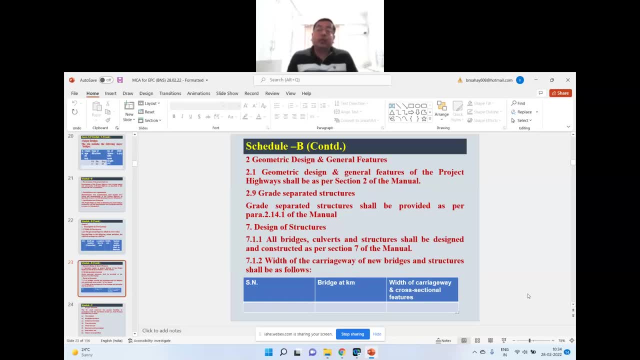 Great separator structure. Great separator structure shall be provided as per para 2.14.1 of the manual. He has to follow this manual. Even clause has been mentioned that as per this clause only they have to design Design of a structure. 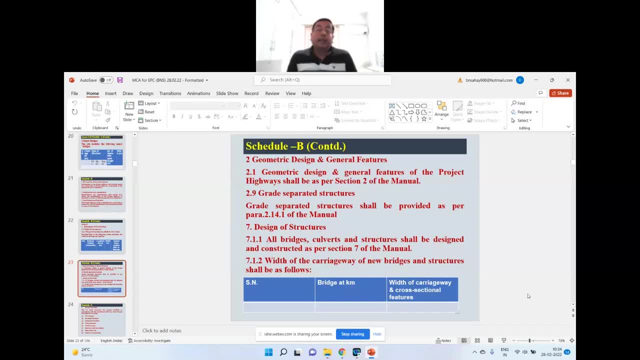 All bridges, culverts and structures shall be designed and constructed as per section seven of the manual. In case of bridges, culverts and structure, he will design, as per section seven of the manual, Width of the carriageway of new bridges. 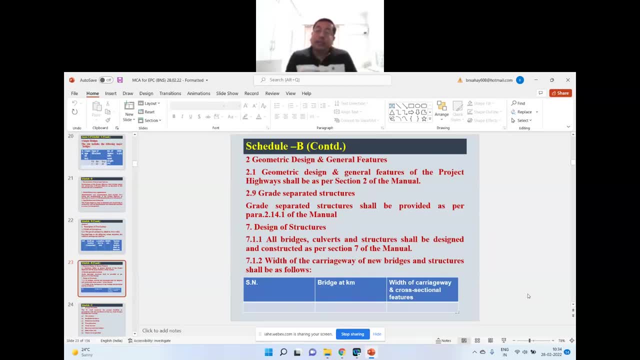 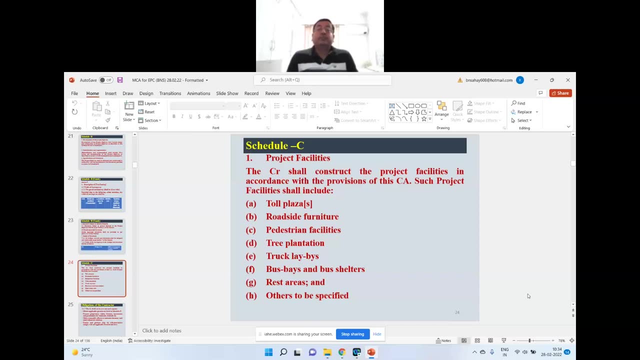 Structure shall be as follows. Here you will have to define this table: Serial number, bridge at kilometre width of carriageway and cross-section features. Now coming to Schedule C, project facilities. The contractor shall construct the project facilities in accordance with provisions of this CA. 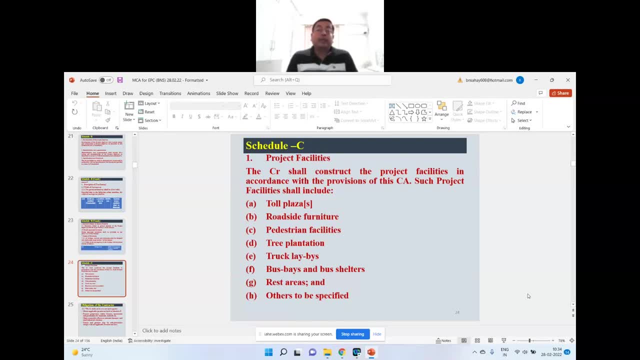 Such project facilities shall include first tall plaza or tall plazas. Suppose your highway is long and it may be 120 kilometre. In that case you must be having two or three tall plazas. In that case, you must be having two or three tall plazas. 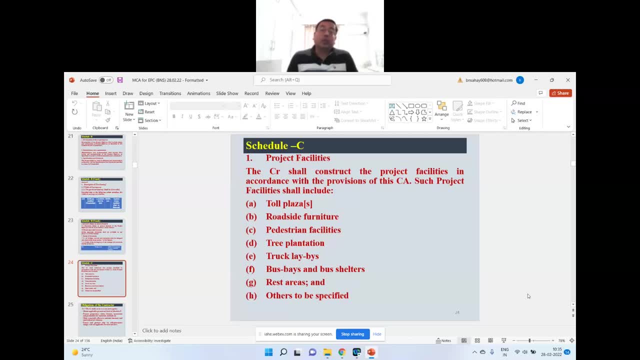 In that case you must be having two or three tall plazas, So you will have to mention location of tall plazas. Roadside furniture: which type of roadside furniture you want? delinators, cat's-eye, whatever. you want roadside furniture, it is mentioned. 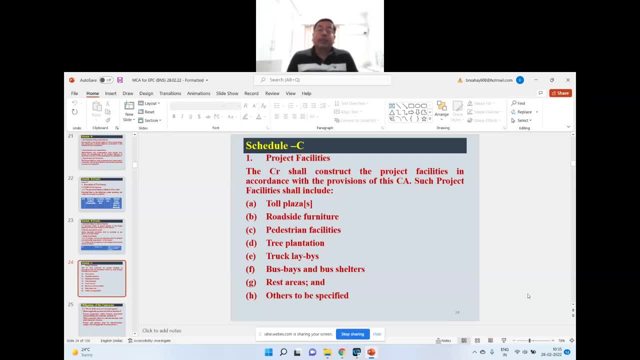 Prestigeant facilities. what type of prestigeant facilities? Suppose you want footpath, then everything will be defined in the Schedule C. Tree plantation: you want tree plantation along the highway After the soldiers, Truck lay-by, bus bays and bus shelters, rest areas and others you can specify. 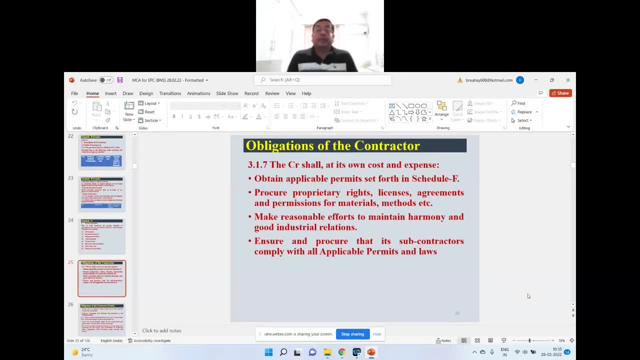 The contractor shall, at its own cost and expense, obtain applicable permit. He has to obtain applicable permit at its own cost. authority will not bear any cost, And what type of permits he is required is mentioned in Schedule F. In Schedule F all the permits are well defined. 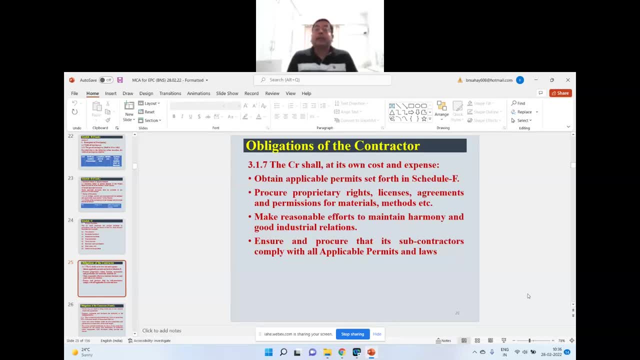 So contractor know that he has to obtain following permits which is mentioned in Schedule F: Procure proprietary rights, licenses, agreements and permissions for materials, methods etc. He will also procure these things, Make reasonable effort to maintain harmony and good industrial relation. 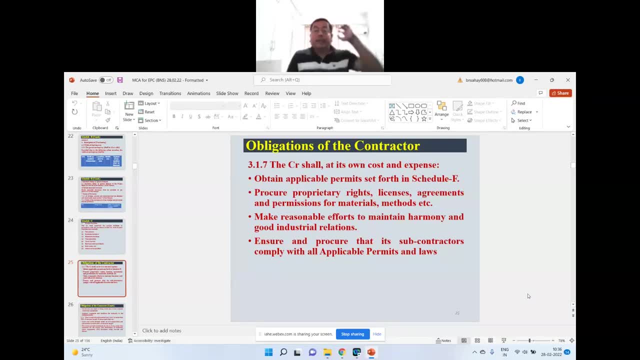 He will maintain a very good industrial relation and harmony at site, Ensure and procure that the subcontractors comply with all applicable permits and laws. It is also to be ensured by the contractor subcontractor that its subcontractor will comply with all applicable permits and lodge Otherwise. 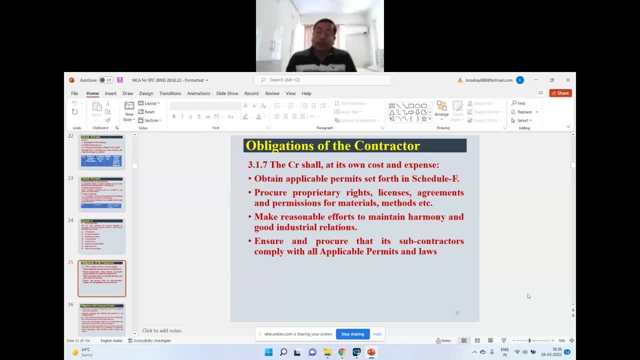 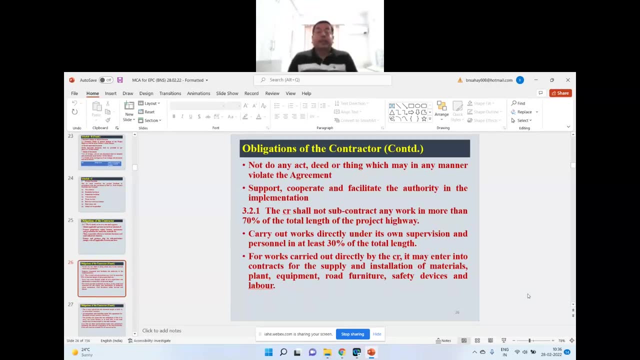 it will have a dispute with other departments. So this is mentioned in this agreement. Whatever you want to incorporate or whatever you want to get done, you must mention here, because until, as you will mention here, contractor has no obligation to do this. So everything should be mentioned. 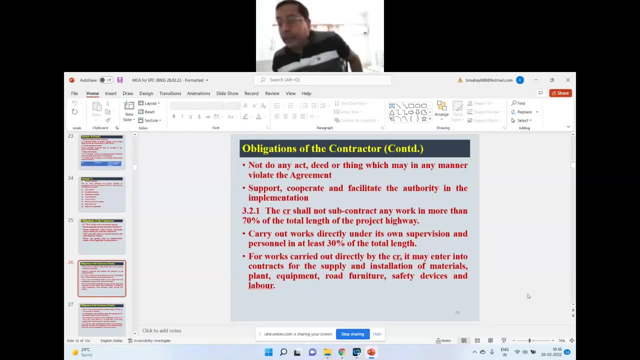 clearly in this agreement. While drafting this, your agreement for a project, you must go through each and every clause and may amend and get approval of the competent authority and then float it Now. obligation of the contractor not do any act, deed or things which may in any manner. 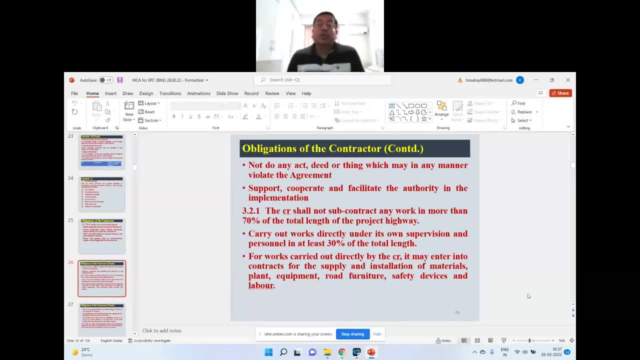 violate this agreement, Support, cooperate and facilitate the authority in the implementation. He will support, cooperate and facilitate the authority in implementation. Now coming to clause 3.2.1,. the contractor shall not subcontract any work in more than 70% of total length of the. 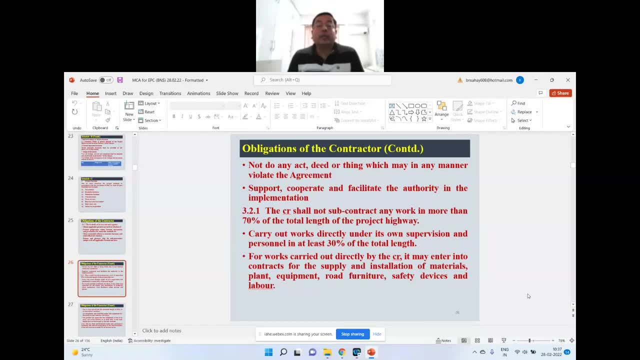 project. It means 30% of the work had to be executed by the contractor itself and he can sublet 70%, Carry out work directly under its own supervision and personally in at least 30% of the total length. For works carried out directly by the contractor it may enter into contracts for the supply. 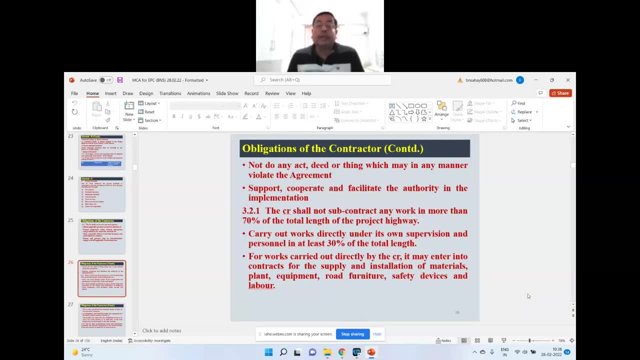 Suppose in this 30%, 30% had to be done by the contractor itself and 70% can be sublet. But for 30% he may enter into contracts for supply and installation of materials, plants, equipment, road furniture, safety devices and labor. So he is allowed to obtain these things under a contract. 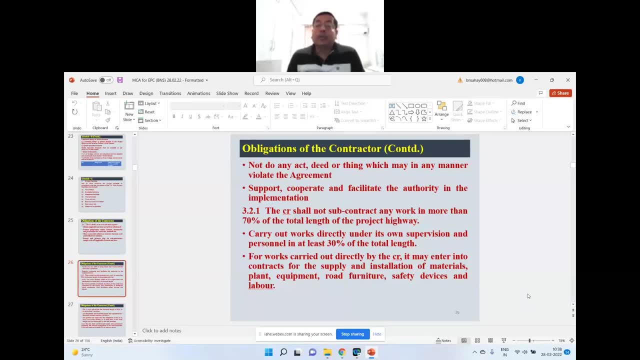 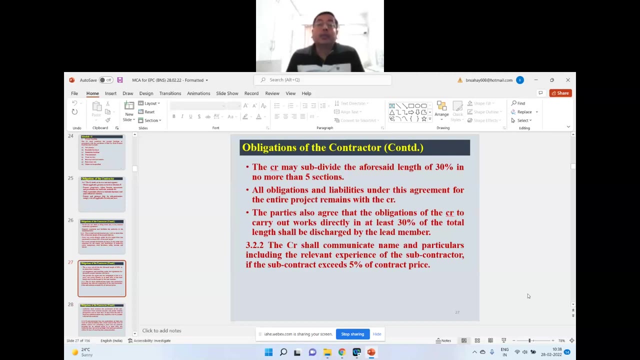 like supply and installation, plant equipment, road furniture. They may enter into an agreement with another subcontractor for these things within their 30% work. The contractor may subdivide the forced length of 30% in no more than five sections. Now, this 30% length is not to be bifurcated in more than five sections All. 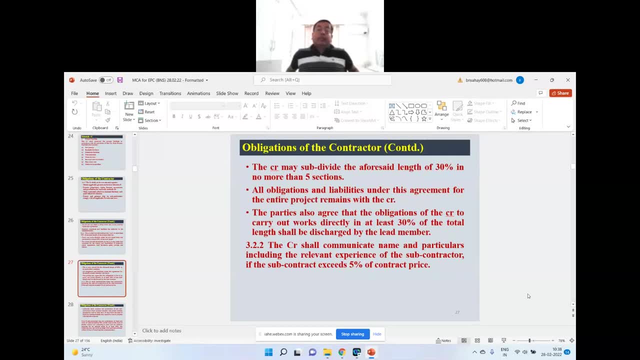 obligations and liability under this agreement for the entire project remains with the contractor, All obligations and liability, even though he has awarded the work to subcontractor. but all the obligations and liabilities lie with the main contractor. He is accountable. Suppose something wrong happens, we will not try to subcontractor, We will ask the contractor to get it done. 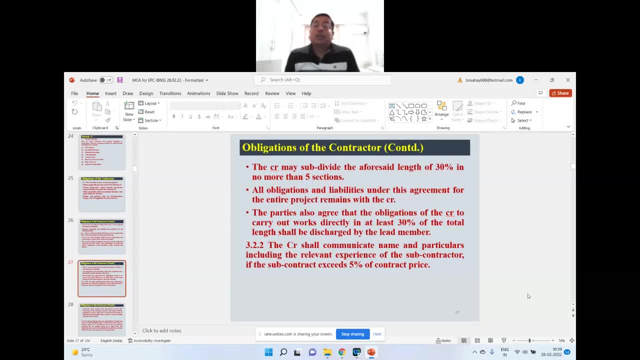 modify it. The parties also agree that the obligation of the contractor to carry out works directly in at least 30% of total length shall be discharged by the lead member. Here it is also mentioned. suppose your work has been awarded to a contractor which is in JV Joint Venture. 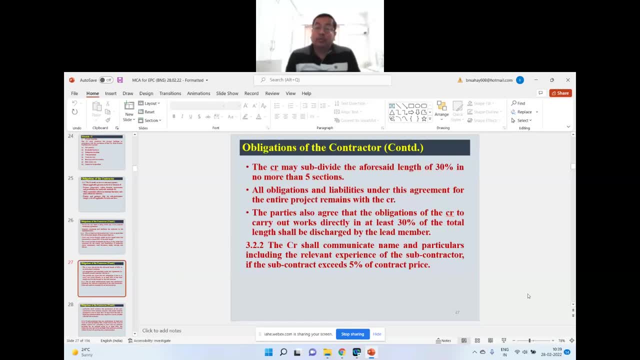 In that case, this 30% quantum of the work, 30% length of the work, will be done by the lead member only, not by the other member. The contractor shall communicate name and particulars, including the relevant experience, of the subcontractor. 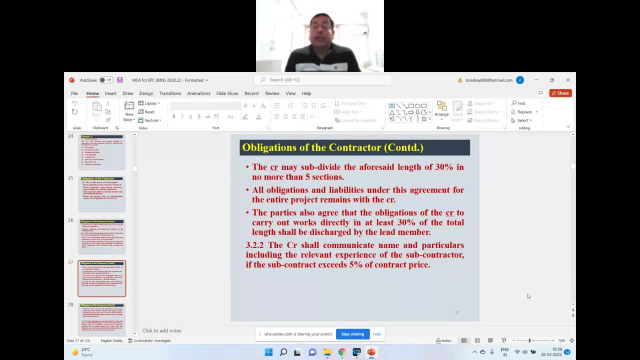 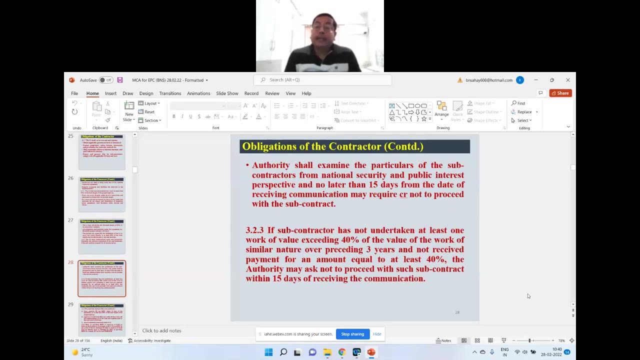 If the subcontract exceeds 5% of contract price. In case of subcontract exceeding 5%, he will have to mention name and particulars and relevant experience of the subcontractor to the authority. Authority shall examine the particulars of the subcontractors from national security and public interest perspective. 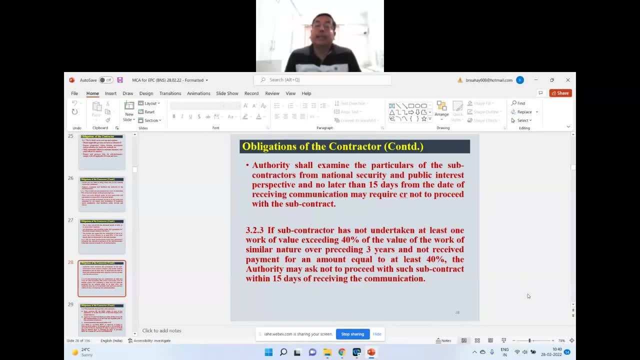 And no later than 15 days from the date of receiving communication may require contractor not to proceed with the subcontract. Suppose Contractor furnished you the details of the subcontractor and you examined it. Suppose the contractor is from other country. You don't want to engage those country personal from those country. 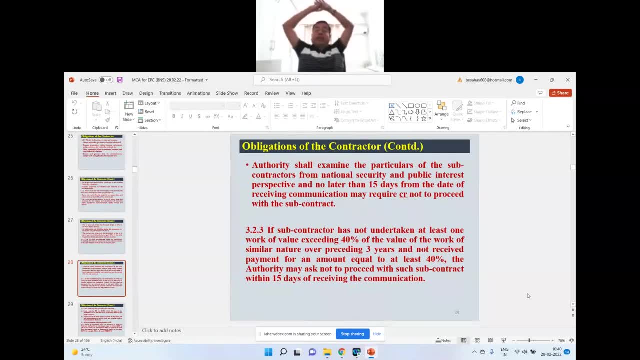 In that case you can deny And suppose the subcontractor is not having the requisite experience. In that case also you have to communicate that not to proceed with the subcontractor, But no later than 15 days If subcontractor has not undertaken at least one work of value exceeding 40% of the value of work of similar nature over preceding three years. 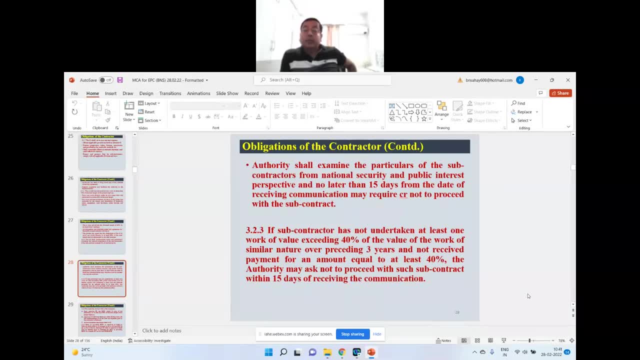 If he has not executed a work of value exceeding 40% of the value of the work which he has been assigned of similar nature over preceding three years and not received payment for an amount equal to at least 40%, the authority may ask not to proceed. 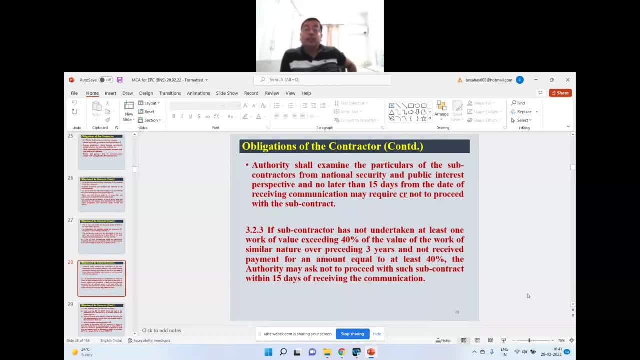 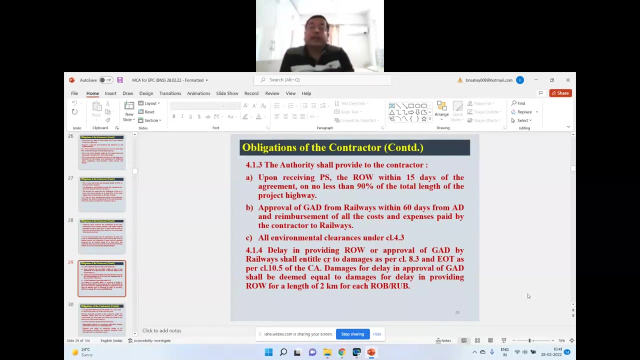 In that case subcontractor is not eligible And you may write that this subcontractor cannot be allowed. But you have to define the only thing: within 15 days of receiving the communication from the contractor, The authority shall provide to the contractor upon receiving performance security. 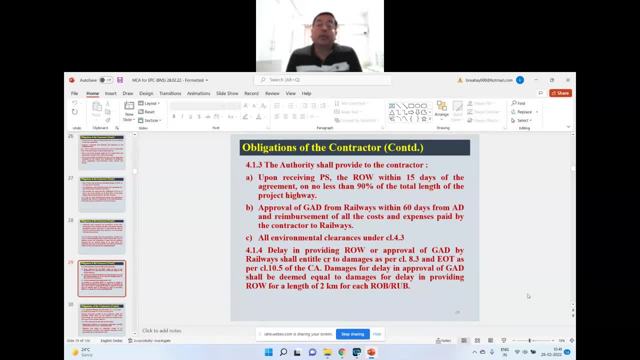 the Right-of-Way within 15 days of the agreement On no less 9 percent or total and appropriate events. an agreement On no less 9 percent or total and appropriate events. highway: Please mind it, You have to furnish 90% of the total. Suppose your highway is 100 kilometer. 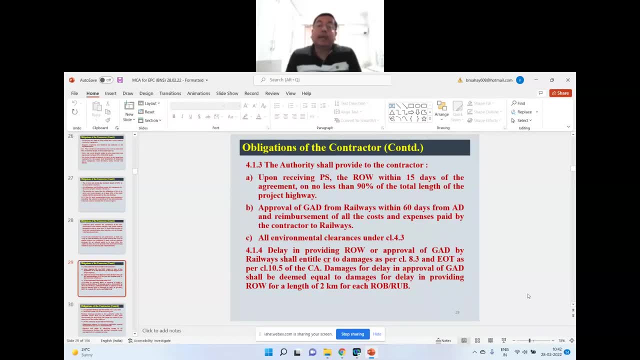 you have to provide 90 kilometer length of the project highway after receiving performance security within 15 days. So you must also be very much alert while awarding the work Approval of GAD from railway within 60 days from the appointed date. The approval of GAD. 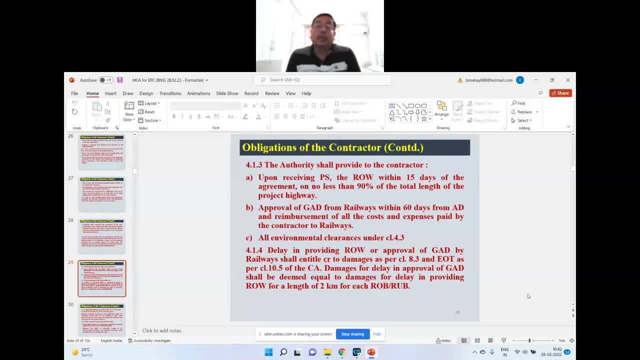 from railway is your job and you have to provide it to the contractor within 60 days from the appointed date, and you will also reimburse all costs and expenses paid by the contractor to railway. Initially, the contractor will pay all the fees of the railway and later on, after- within 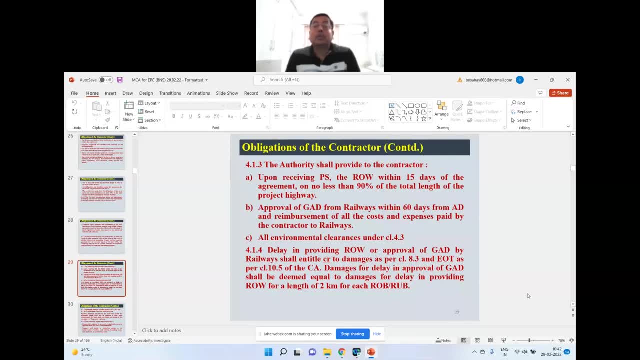 60 days from the appointed date. you will reimburse all the costs and expenses done by the contractor for railway. Any query? Okay, Now all environmental clearances under 4.3. You will also have to get environmental clearance from the concerned authority so that you provide unencumbered land to 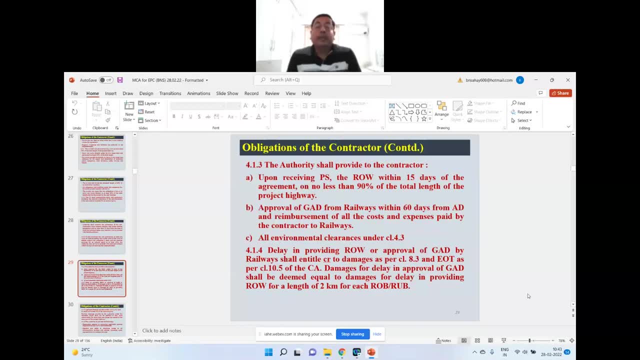 contractor for the construction of work. Delay in providing right-of-way or approval of GAD by railway shall entitle contractor to damage 8.25% or damage as per clause 8.30%, and EOT as per clause 10.8% of the CA. 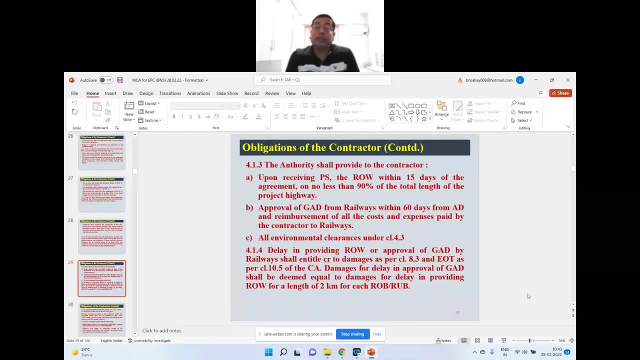 Mind it. if you are delaying in providing ROW or approval of GAD, the contractors shall be entitled to damages as per clause: damages for delay in providing right of way for a length of 2 kilometer for each ROV. What will be the quantum of damages for a ROV equivalent to 2 kilometer of? 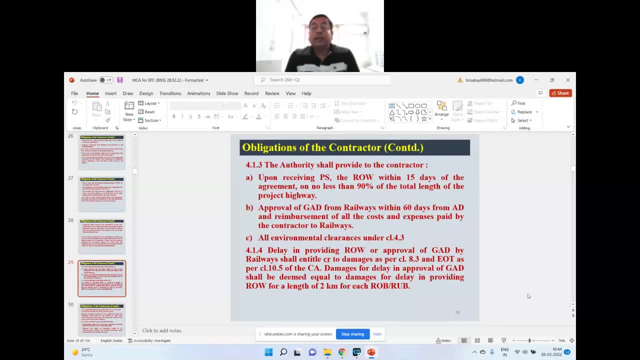 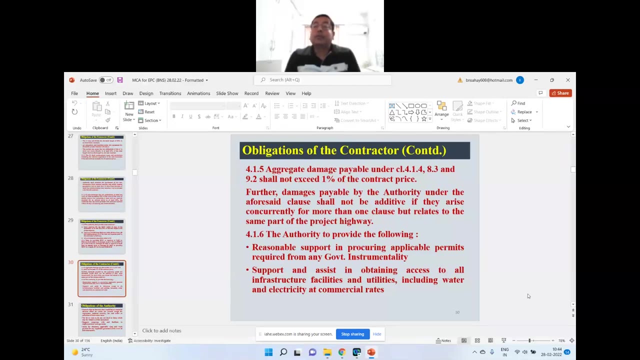 road length. In case you are unable to provide approval of GAD of a ROV, you will have to pay damage for 2 kilometer length of the highway. Now it is also defined: aggregate damages payable under clause 4.1.4,, 8.3 and 9.2 shall not. 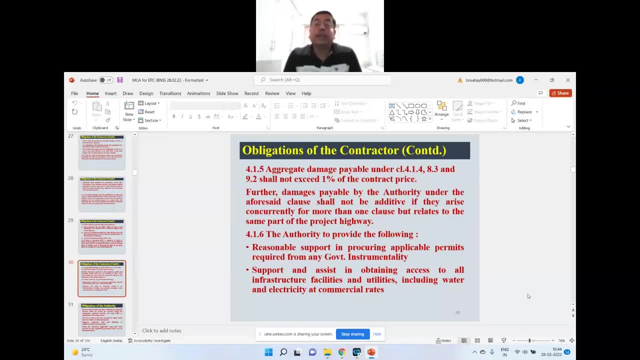 exceed 1% of the contract price. It is also to be very clearly understood. suppose your contract is of 500 crore, you have not to pay more than 5 crore. That is only 1% in that total damages payable under the clause 4.1.4,, 8.3 and. 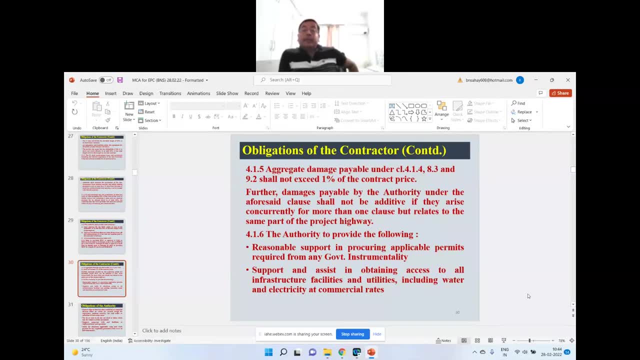 9.2.. For the damages payable by the 30 under this. under the above clauses shall not be additive if they arise concurrently for more than one clause but relate to the same part of the project highway, Suppose between kilometer 50 to 55. you are not. 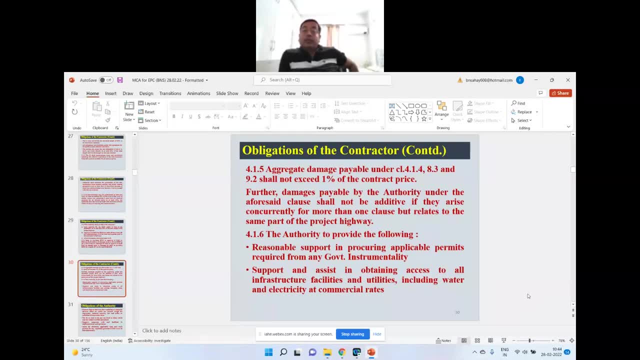 having clearance of GAD and environmental clearance for the same part of the project highway. you are having a number of things. then you will not have to pay damages for each of the things. If the same part of the project highway is there, then you will have to pay damage for. 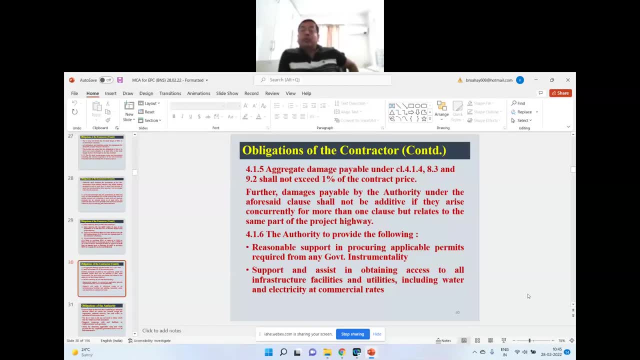 that part of the project highway for only one thing, not for the all the things separately. The authority had to provide the following: reasonable support in procuring applicable permits required from any government. instrumentality Support and assist in obtaining access to all infrastructure facilities and utilities, including water and electricity, at commercial rate, not at domestic. 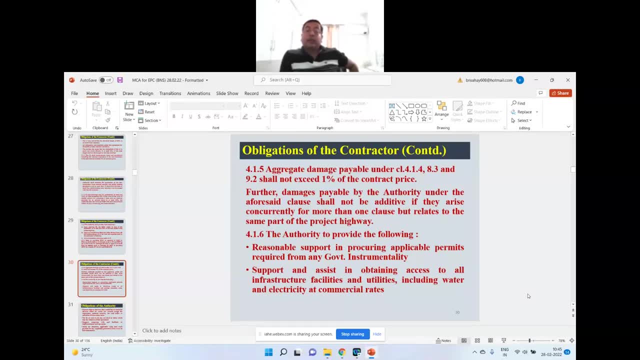 rate- commercial rate. You have to cooperate because he will procure permits but you will have to write to the concerned authority. Similarly, suppose he wants to get water connection, electricity connection at site, project site, then you will facilitate, but at commercial rate. He will get all the things at commercial rate from the concerned authority. 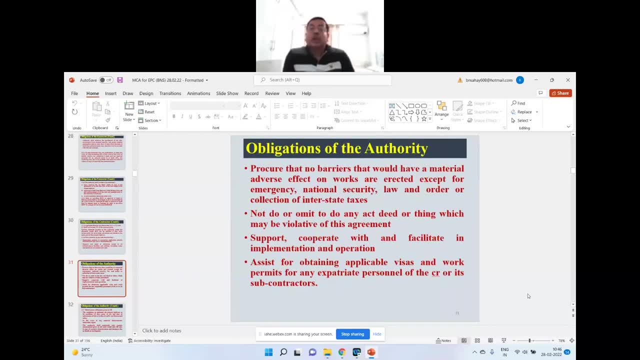 Department and you will cooperate. Obligation of the authority: Authority. please see, these are your obligations. You have to procure that no barrier that would be that would have a material adverse effect on works are rejected, except for emergency. Suppose some emergency is there then? 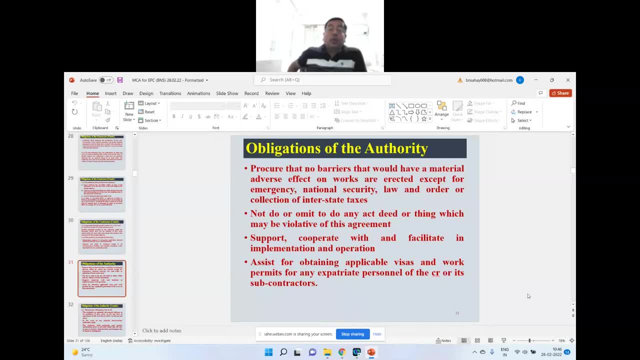 you have to reject national security law and order or collection of interstate taxes, Other responsibilities. You cannot adjustment any barrier. You have to insure it. You have not to do or omit to do any act, did or thing which may be violative of this agreement. 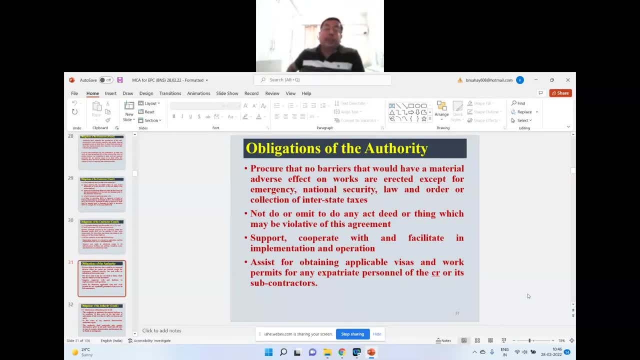 Third, support, cooperate with and facilitate in implementation and operation. you have to support, cooperate and facilitate in implementation and operation And assist for obtaining applicable Visya and work permits for any expertise person of the contractor or its subcontractor. the contractor is having subcontractor and he is expatriate. it means he is a foreign national. 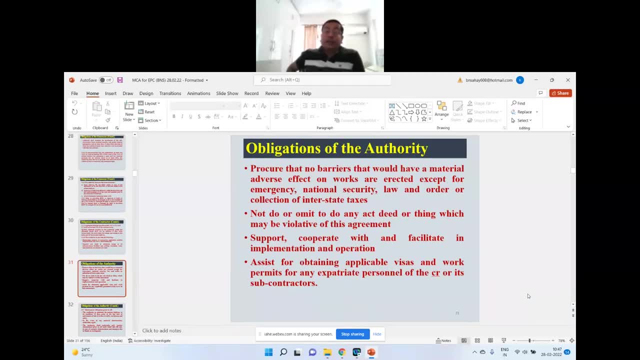 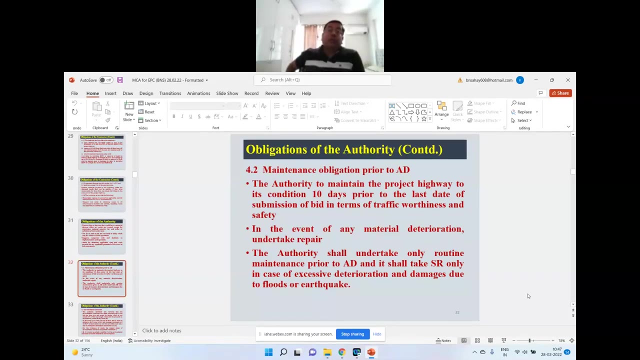 in that case he will require visa. you will have to procure that. so authority has this liability obligation, which has to be done, and you will procure visa for him. this is also very important clause: maintenance obligation prior to appointed date. please see that whatever you have written in the agreement must be very much clearly defined. 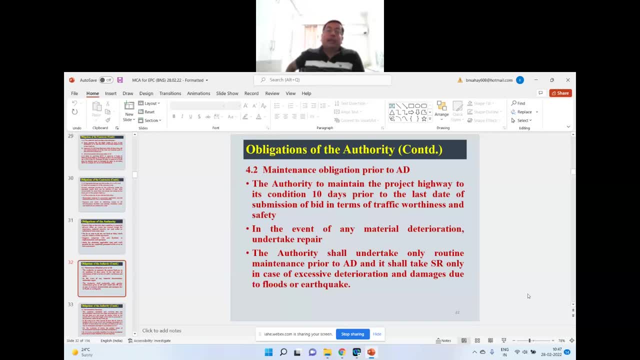 otherwise your project highway may suffer. so try to write each and everything in this agreement if you think it is essential, and so, before floating it, amend it, what wherever it is required, and then take approval of the competent authority and only then float the rfp and dca draft contract agreement. 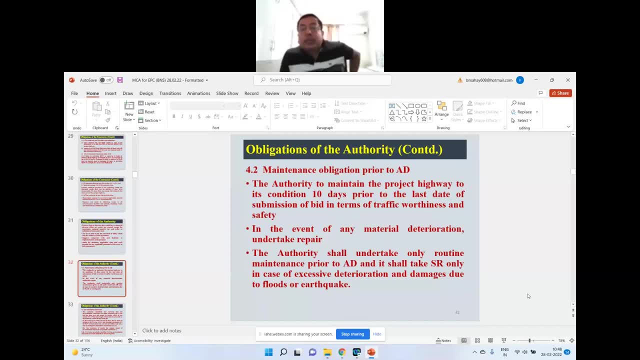 the authority to you to maintain the project highway. the authority has to maintain the project highway to its condition 10 days prior to the last date of submission of bid. in terms of traffic worthiness and safety, this is the obligation of authority. that authority will maintain the project highway. 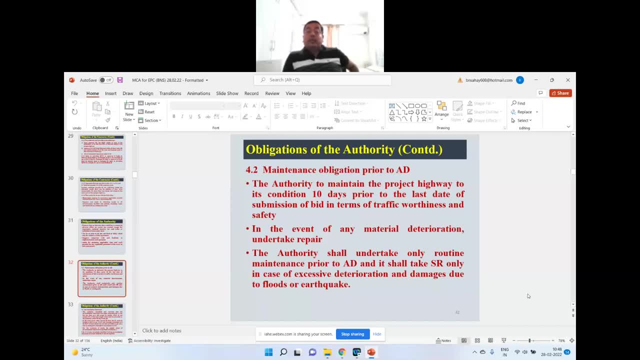 to what condition 10 days prior to the last date of submission of bid? in terms of traffic worthiness and safety in the, he will. the authority will not improve it but maintain it in traffic but in safe condition. in the event of any material deterioration, undertake repair, suppose. 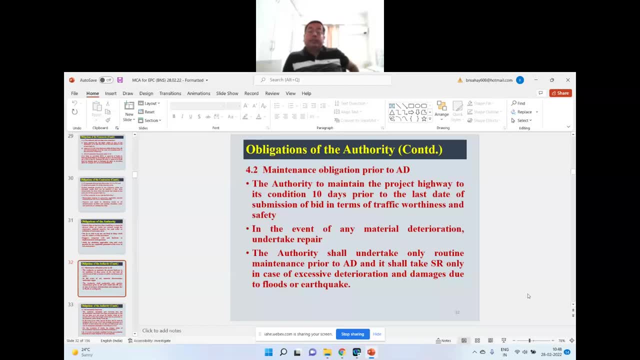 some portal portals have been developed. it will have to be filled up or suppose wearing cold hand deteriorated, it will have to be repaired. the 30 cell undertake only routine maintenance. it is also defined that a 30 cell will undertake only routine maintenance prior to a point, a date, and it shall. 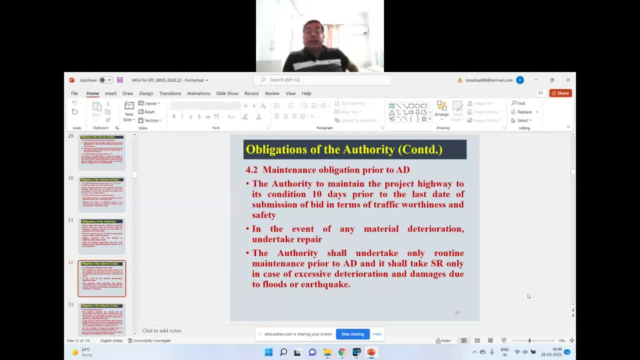 take a special repair only in case of excessive deterioration, only in case of excessive deterioration and damages due to flood or earthquake. Suppose some earthquake has come or some flood has come and the road is washed away- In that case only a special repair will be done. Otherwise, 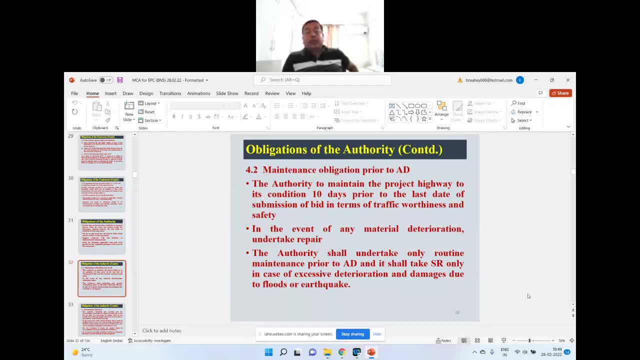 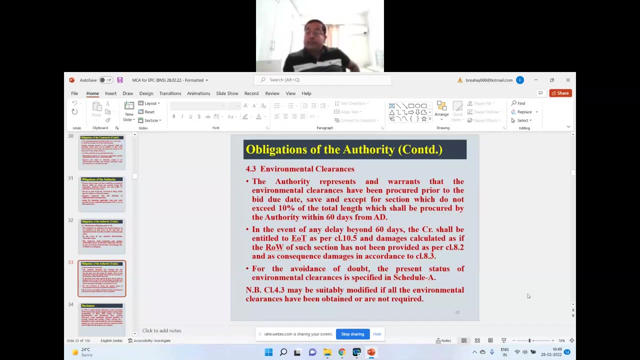 only routine maintenance will be done prior to a punctuality. This is also well defined in the agreement so that your contractor may not dispute these things with you. Environmental clearances: The authority represents an invariant that the environmental clearance have been procured prior to the B due date. save and accept for section which do not exceed 10% of total. 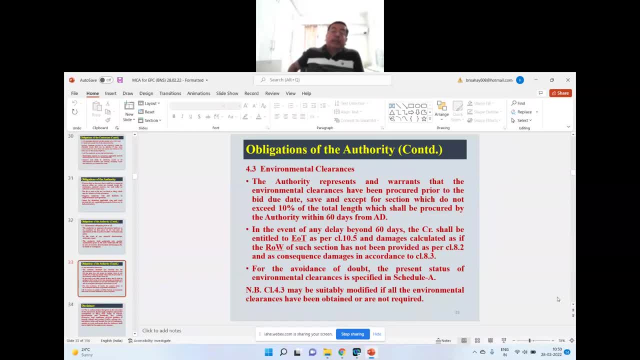 length, which shall be procured by the authority within 60 days from the appointed date. This is well defined: that environmental clearance for 90% has already been obtained and 10 percent will be procured, provided within 60 days from appointed date. 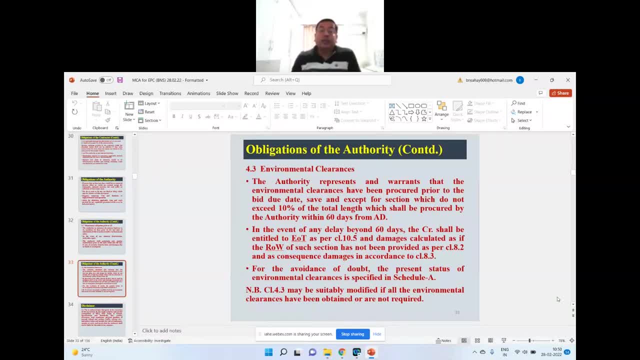 In any delay beyond 60 days, the character cell being entitled to extension of time as per clause 10.5, and damages calculated as if the ROW of such sections have not been provided, as per clause 8.2, and as consequences damages in accordance with clause 8.3.. 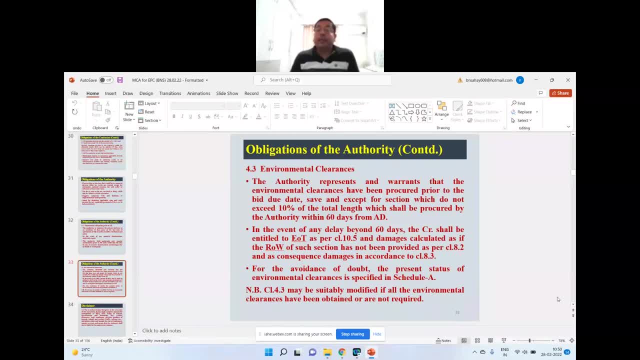 It means, in the event delay beyond 60 days, the character cell being entitled to EOT as per clause 10.5 and damages as per clause 8.3, as if you have not provided the requisite ROW. So please be careful while building the project: you must be well prepared at site also. and 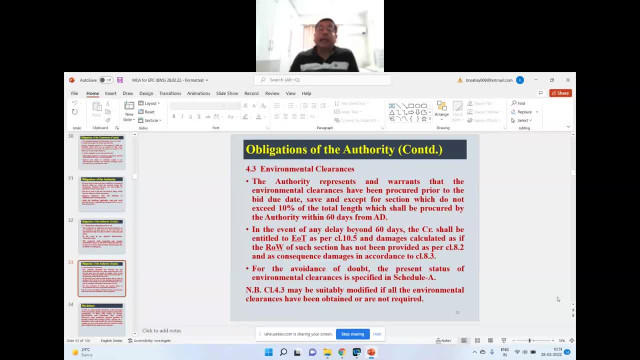 procure all the things. Otherwise you will have to pay damages At this rate, including time extension. For the avoidance of doubt, the present status of environmental clearances is specified in Schedule A. In Schedule A we have already defined status of environmental clearances. 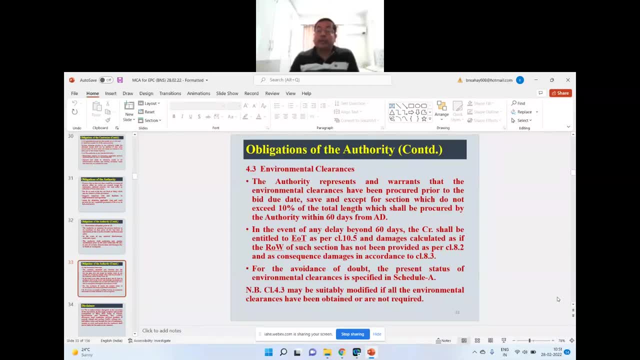 Whatever is the condition, whatever is the status of environmental clearances is already defined in annexure of the Schedule A. Clause 4.3 may be suitably modified If all the environmental clearances have been obtained or are not required. Suppose you need not any environmental clearances, then you will not have to write these things. 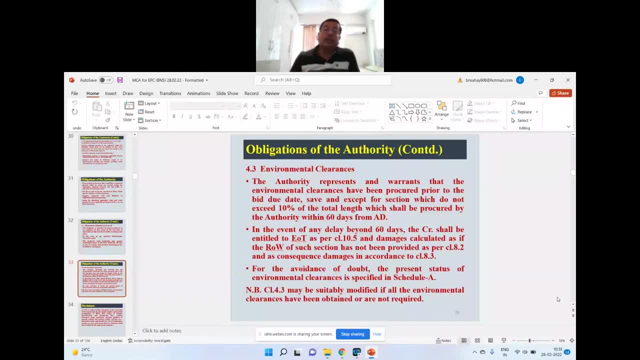 because you have already got all the things, So you can delete all these clauses. Depending upon the site condition, you can amend your MCF. please mind it. you go through it and carefully study each and every clause and, depending upon the site condition, you. 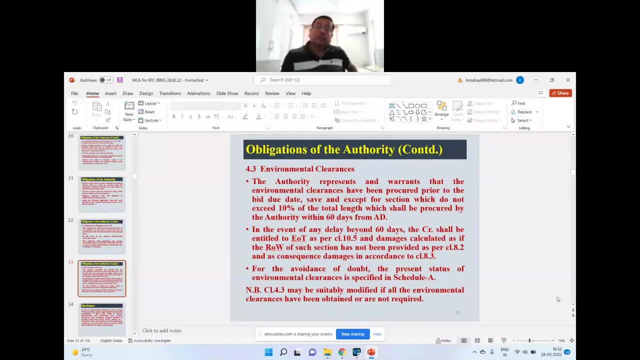 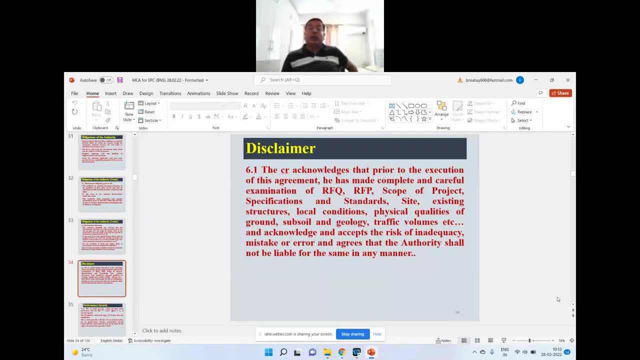 amend it before bidding. Okay, Now what is disclaimer In disclaimer? chapter authority wants to clarify that we are not responsible for anything. You must go through all the things and you acknowledge that, all the things you have seen, and we are not accountable for anything. 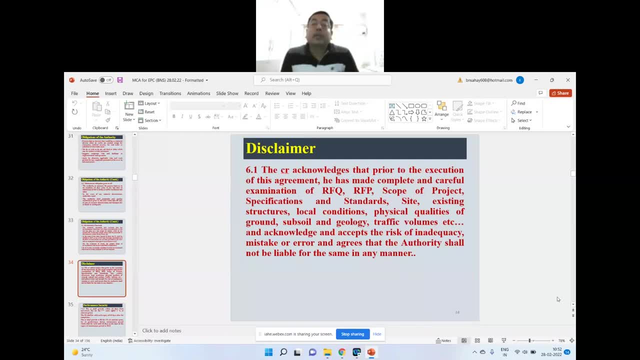 So it has been mentioned and written. The contractor acknowledges that, prior to the execution of this agreement, he has made complete and careful examination. Okay, So the contractor has made complete and careful examination of RFQ RFP. scope of the project. 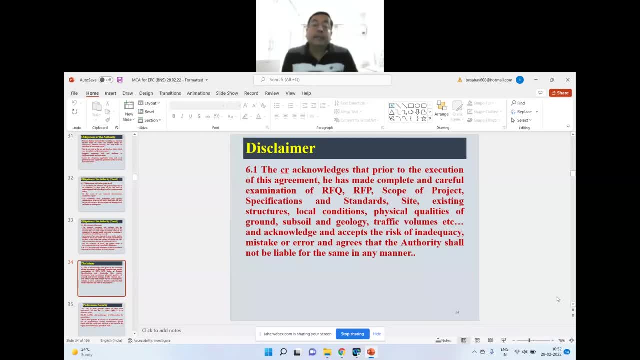 specification and standards, site, existing structures, local conditions, physical quality of ground, subsoil and geology. Suppose he will tell your soil is not good After signing the agreement and after your ground is not good, it is having expensive soil. 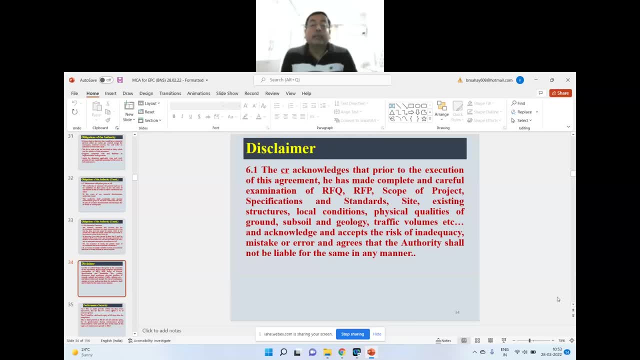 No, he cannot do so because we have already written the disclaimer that please go to the site And our things may be wrong. You examine the site, including its subsoil and geology, traffic volumes, and accept that the risk of inadequacy, mistake or error. 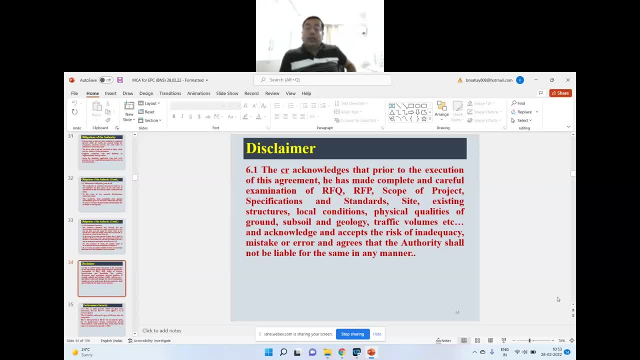 All the things are not. authority is not accountable for any of these things And contractor agreed that the authority shall not be liable for the same in any manner. Disclaimer chapter is very much important from the point of view That contractor cannot claim that this was wrong at site and I was not knowing the contractor. 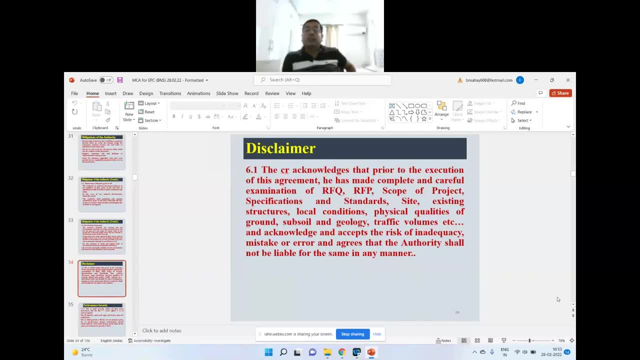 in this disclaimer chapter has been clearly mentioned that you go to the site, you acquaint yourself with the physical condition of the site and then you agree and our data may be inadequate, inaccurate or it may have error or mistake, So we are not accountable for this. 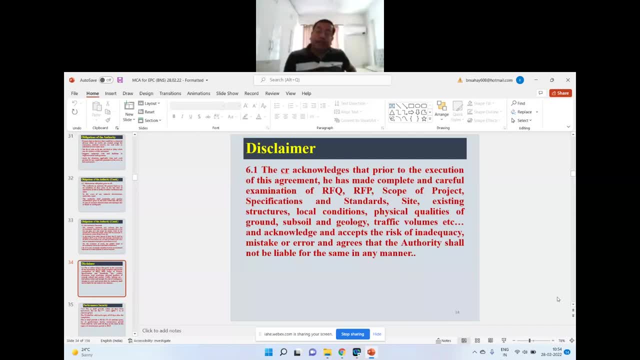 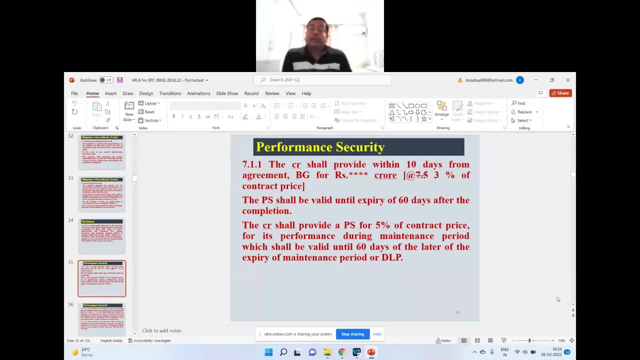 So contractor has been. The contractor has to sign this, So disclaimer has been given here. Now performance security: The contractor shall provide within 10 days from the agreement. Please see, they have to furnish performance security within 10 days of the agreement in. 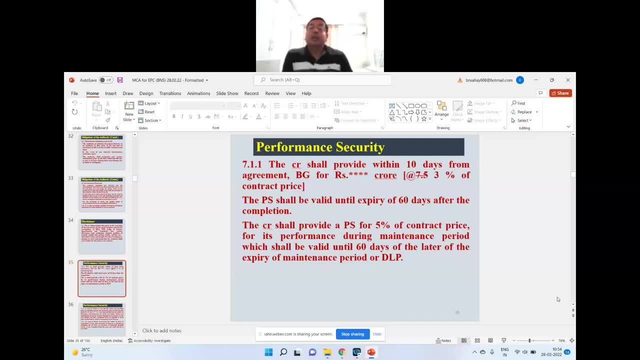 the form of bank guarantee for rupees at the rate of 3% of contract price. Earlier it was 7.5,, then it was 5, and now it is 3% of contract. This can be varied. This can be varied. 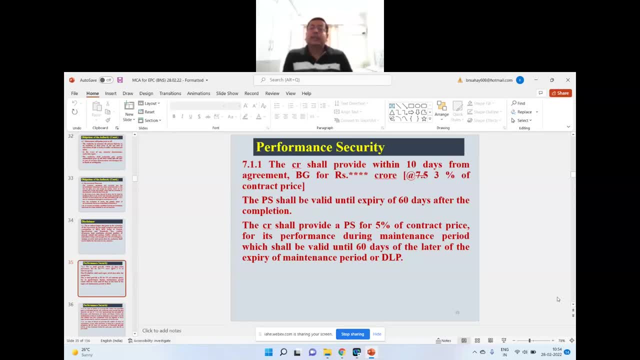 This can be varied Depending upon circulars issued by the authority from time to time. you have to see what is the quantum of performance security. accordingly, you can fill up here. The performance security shall be valid until expiry of 60 days after the completion. 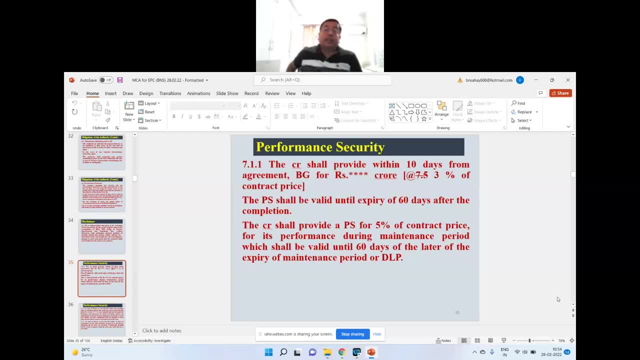 The performance security shall be valid 60 days after the completion. The contractor shall provide a performance security for 5% of contract price for its performance during the maintenance period. Okay, During maintenance period also, they will provide 5% of contract price, which shall: 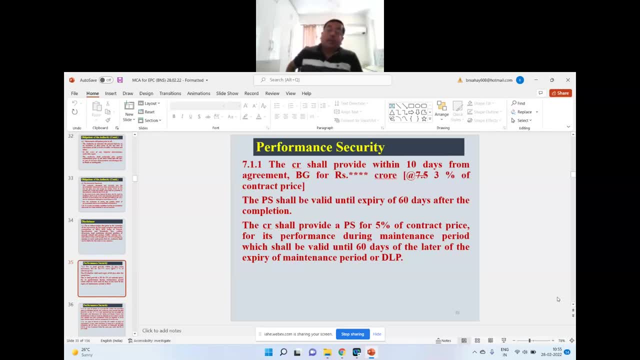 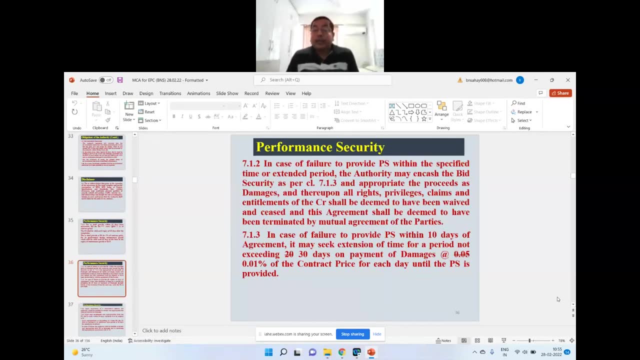 be valid until 60 days of the later of the expiry of maintenance period or DLP. DLP means defect liability period. In case of failure to provide performance security within the specified time or extended period, the authority may encash the bid security as per clause 7.1.3 and appropriate the proceeds. 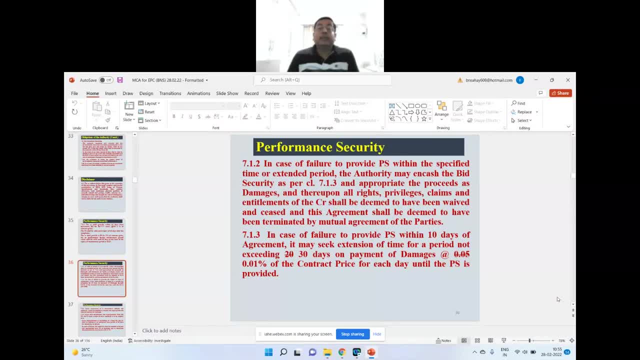 and damages. This has been mentioned that in case of failure to provide PAs performance security within a specified time, you may encash and proceed the damages and thereupon what will happen. All rights, privileges, claims and entitlements of the contractor shall be deemed to have. 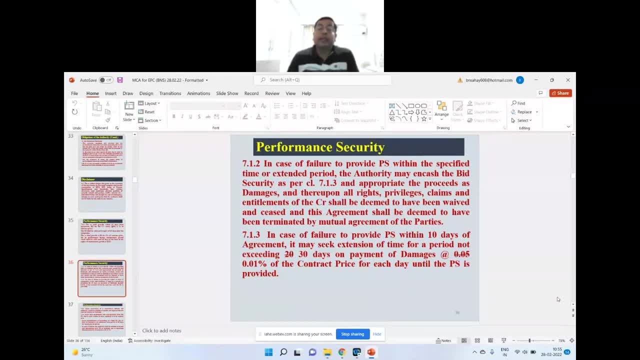 been waived and seized and this agreement shall be deemed to have been terminated by mutual agreement of the parties. You will encash And it will be assumed that it has been terminated by mutual agreement of both the parties, contractor and the authority. In case of failure to provide performance security within 10 days of agreement. in case: 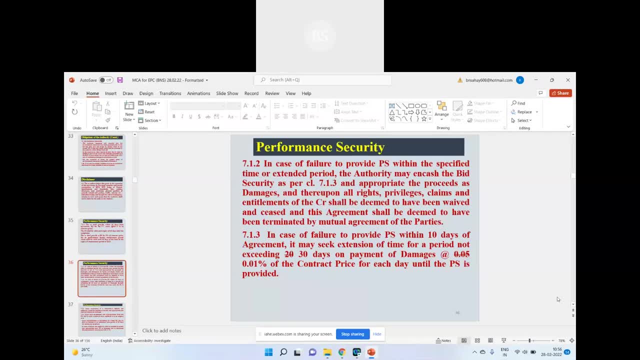 of failure to provide performance security within 10 days of agreement. it may seek extension of time for a period not exceeding. earlier it was 20 days, now it is 30 days. on payment of damages: Earlier the damages were at the rate of 0.05%. 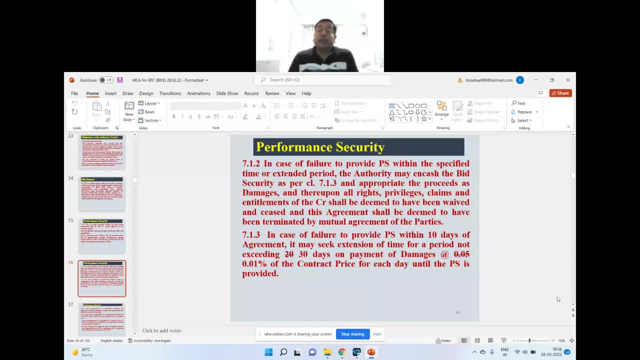 Now it is 0.05%, Now it is 0.05%, Now it is 0.05%. The impact was at the rate of 0.01% of the contract price for each day until the performance security is provided. Suppose contractor understands that he cannot provide within 10 days, then he will seek. 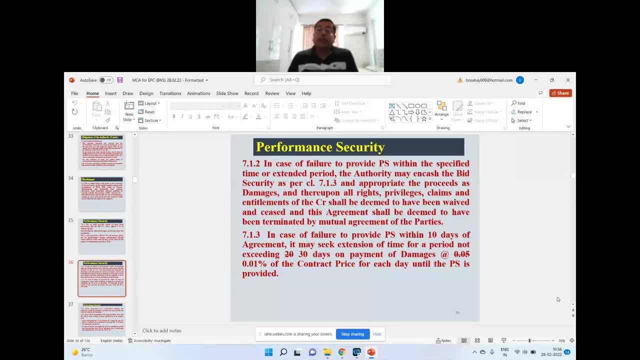 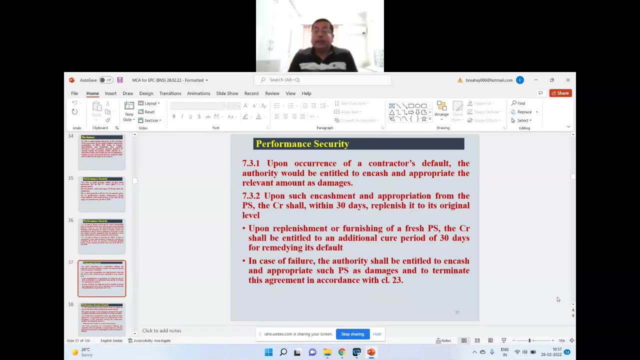 extension, but he will have to pay damages at the rate of 0.01% of the contract price for each day delay until the performance security is provided. Last question: what about PAs and PAs without their Guns? Please ask Upon occurrence of a contractor default. suppose some default has been done by the contractor. 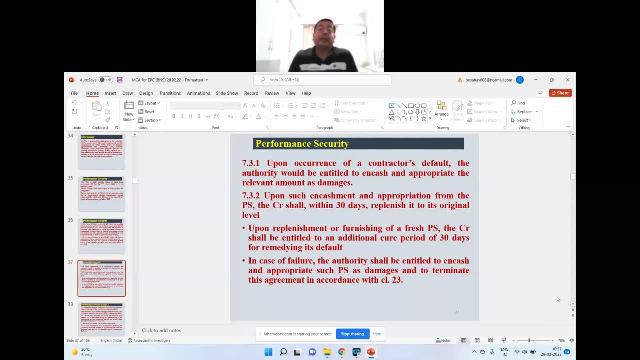 the authority would be entitled to encash and appropriate the relevant amount as measured. Suppose you are having a bank guarantee of 50 crore and suppose you want to encash 10 crore, then you are entitled as per this clause for his default, for the default of the contractor. And you can encash 10 crore out of the 50 crore performance security. Upon such encashment and appropriation from the performance security, the contractor shall within 30 days replenish it to its original level. Suppose: out of 50 crore you have already encashed 10 crore, so only 40 crore is remaining. 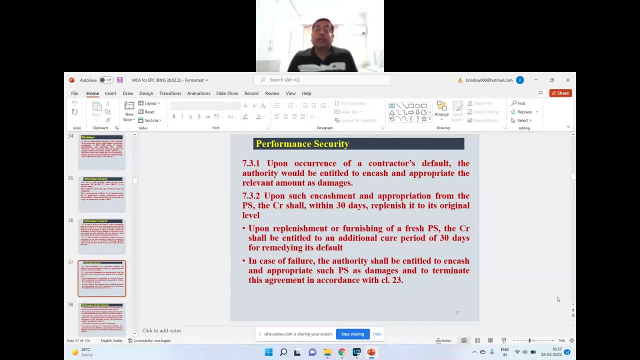 Now he will replenish it to its original level, that is, 50 crore. So he will provide a BD of 10 crore Immediately and not exceeding 30 days. Within 30 days he will provide a BD of 10 crore. Upon replenishment or furnishing of a fresh PS performance security, the contractor shall be entitled to an additional cure period of 30 days for remaining its defects. Suppose some defect has occurred and you have been encashed, then after replenishment of the performance security, 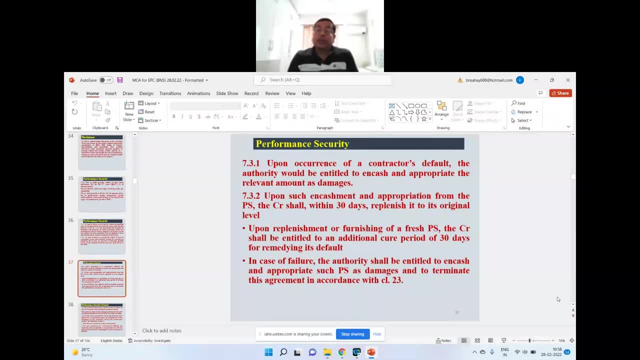 the contractor shall be entitled to an additional cure period of 30 days only, not more than that, for remaining its default. In case of failure, the authority shall be entitled to encash and appropriate such PS as damages and to terminate this agreement. 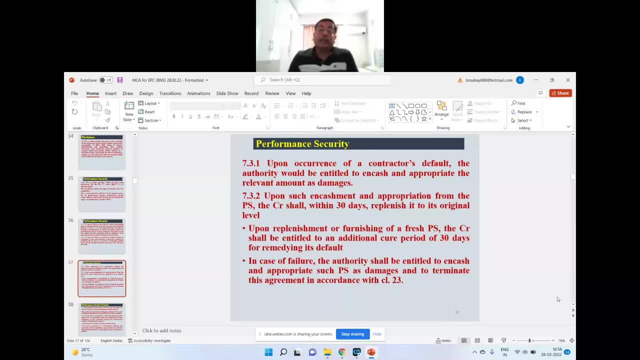 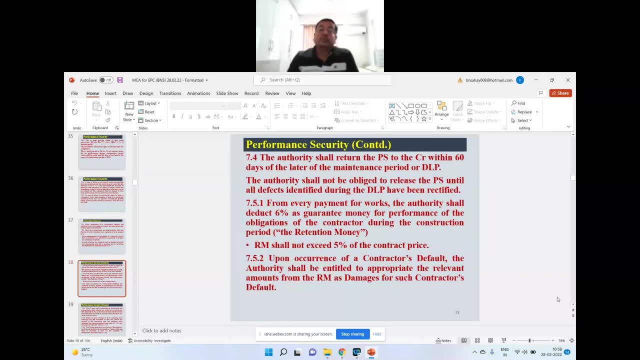 Suppose he is going beyond 30 days, then you can encash entire PS performance security as damages and terminate this agreement As per clause 23.. The authority shall return the performance security to the contractor within 60 days of or the later of the meeting. 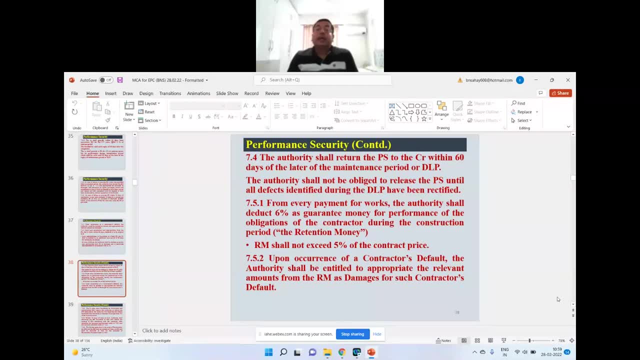 And then the contractor should issue the maintenance period of DLP. You will have to return the performance security to the contractor within 60 days of the latter of maintenance period or defect liabilities. The authorities shall not be obliged to release the performance security until all defects identified. 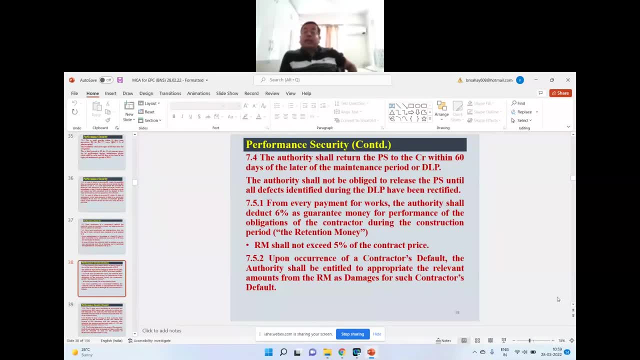 The factor shall not be obliged to release the performance. Please mind that. please see, this is being oh so clear. items. all the defects identified during the DLP period have been rectified. only then you will return the performance security. not before that, Suppose some work is left for which you have. 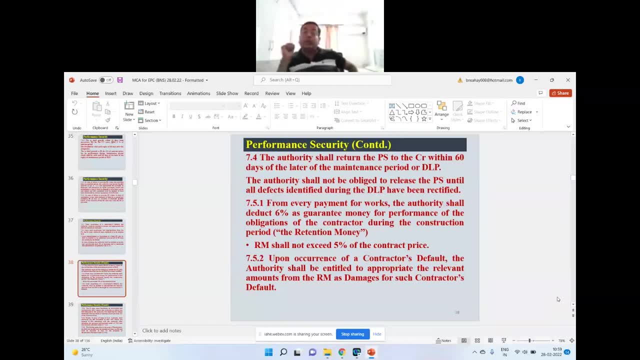 already pointed out the defect and the contractor has not remedied it, then you will not release the performance security. Performance security will be released only when all the defects identified during the DLP have been rectified. Now, from every payment for works, the 30 shall deduct 6%. 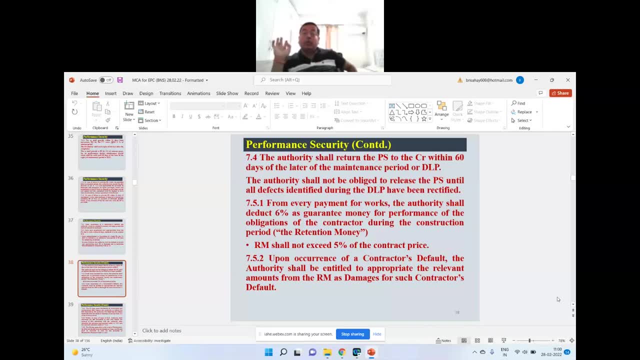 as guarantee money. In addition to performance security, you will also have to deduct 6% as guarantee money for performance of the obligation of the contractor during the construction period. This is known as retention money. This retention money shall not exceed 5% of the contractor From. 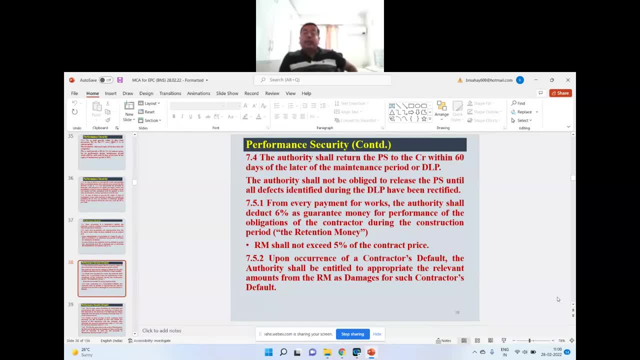 the every bill you will deduct 6% till it reached 5%. So this is also very much important- Upon occurrence of a contractor default- suppose some contractor default has occurred- the 30 shall be entitled to appropriate the relevant amount from the retention money as damages for such contractors default. So retention money has. 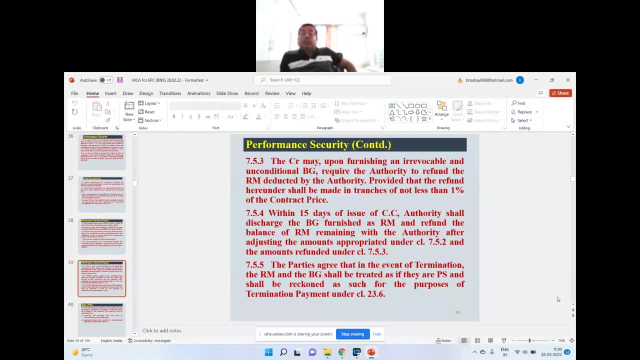 this purpose, The contractor may, upon furnishing an irrevocable and unconditional BG bank guarantee, difficulty requires the authority to refund the retention money deducted by the authority. The contractor may ask you that please refund my retention money and I am providing you the BG. 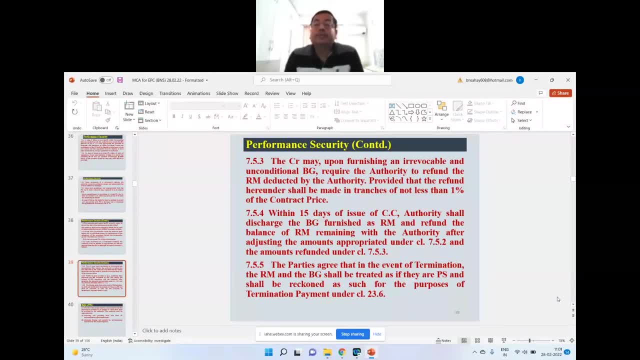 irrevocable and unconditional BG. In that case you can refund it after obtaining BG, provided that the refund shall be made in tranches of not less than 1% of the contract price. Whenever you will refund it, it, it will be not less than one percent, but Viduiiver Refinal ambush for processing fee. 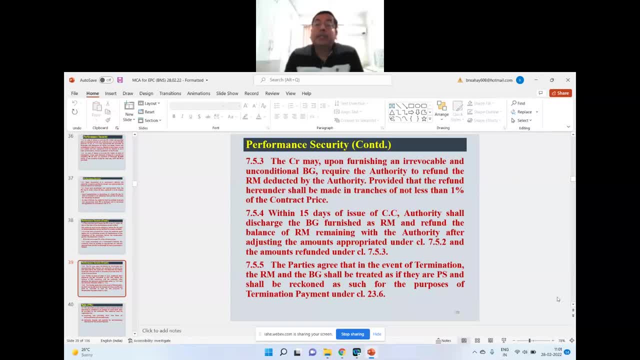 this is an weeds hopper of a way of revocable and unconditional BG. Theándala difficult to recover activities. percent of the contract price. He will provide BG for 5 percent, then you will refund 5 percent. He will return, submit BG for 3 percent, then you will. 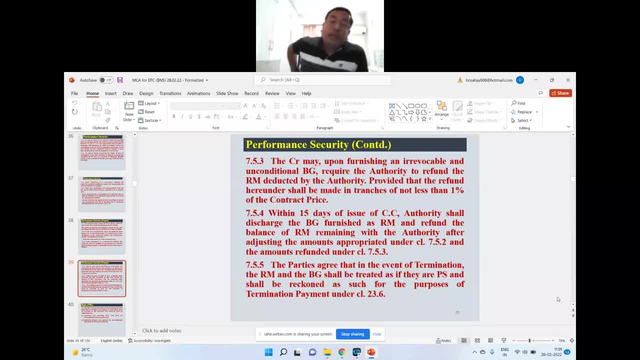 refund only 3 percent. Within 15 days of issue of completion certificate, authority shall discharge the BG furnished as retention money and refund the balance of retention money remaining with the authority. Within 15 days of issue of completion, authority shall discharge the BG furnished as retention money and. 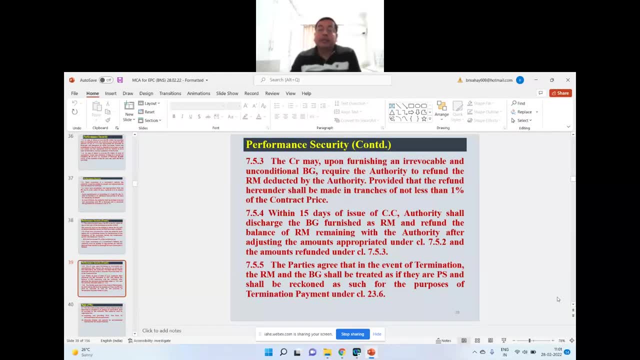 refund the balance of RM remaining, with the authority After adjusting the amount appropriated under clause 7.. Suppose something is damages are to be deducted, then you deduct and refund the retention money or the BG furnished for the retention money. The party is agreed that in the event of termination the 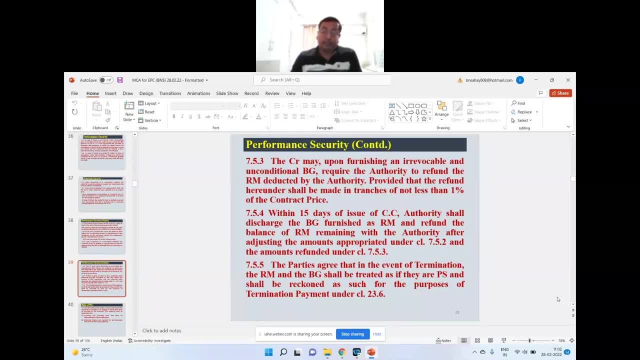 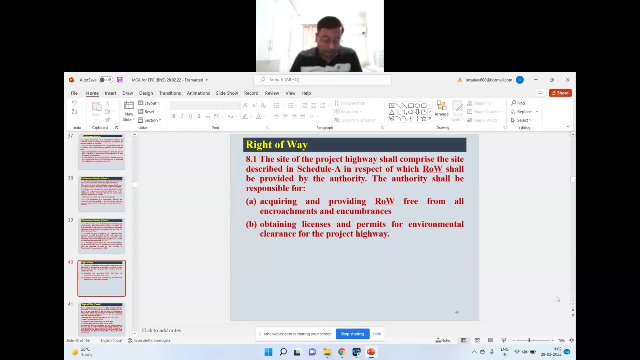 retention money and the BG shall be treated as performance security and shall be reckoned as such for the purpose of termination payment under clause. In that case you will treat it as performance security and may encash appropriate amount out of this Right of way. ROW, The site of the project IBSR, comprise the 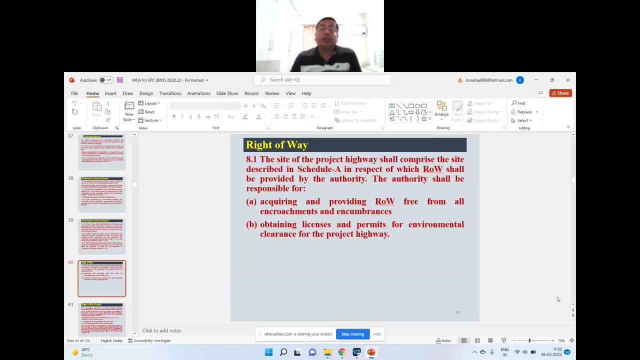 site described in Schedule A, in respect of which ROW shall be provided by the 30. The 30 shall be responsible for acquiring and providing ROW, free from all encroachment and incumbencies. This is your main duty, main responsibility that you have to. 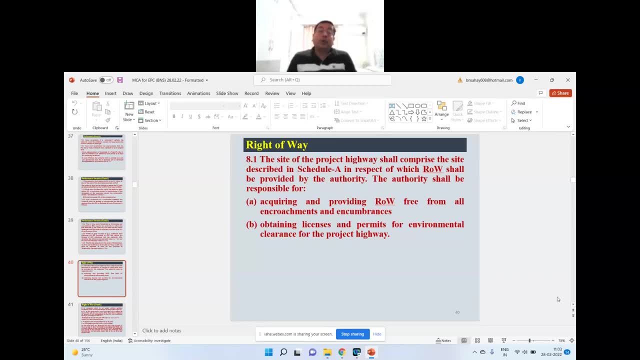 acquire and provide ROW free from all encroachments and incumbencies to the contractor. So it is a very important part on your authority side and you have to take all the necessary steps so that you may avoid- and you you may avoid- you may not pay any damages for this- be obtaining licenses and permits for 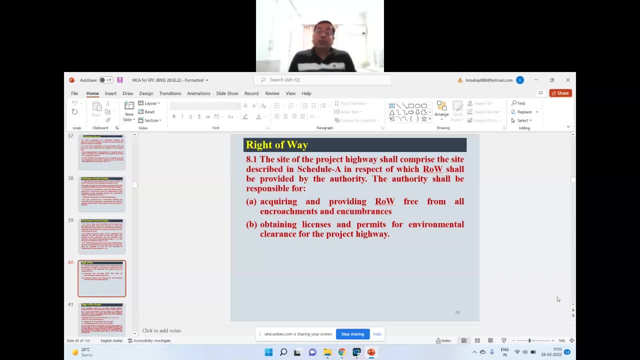 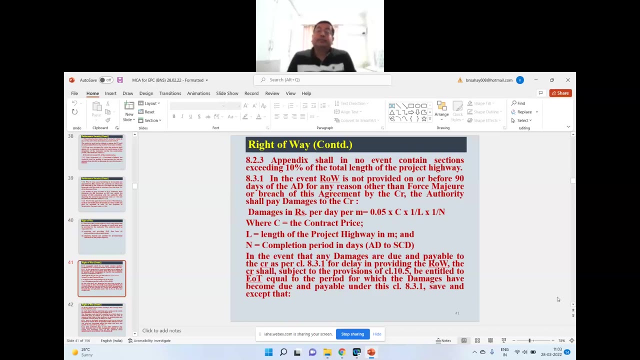 environmental clearance for the project having. you also need to have license and permits for environmental clearance from the concern department for the project. having this is also your obligations. now, what is appendix when contractor and the authority representative visit the site and prepare an appendix? what are not available? those which is those which are available, is not mentioned in the 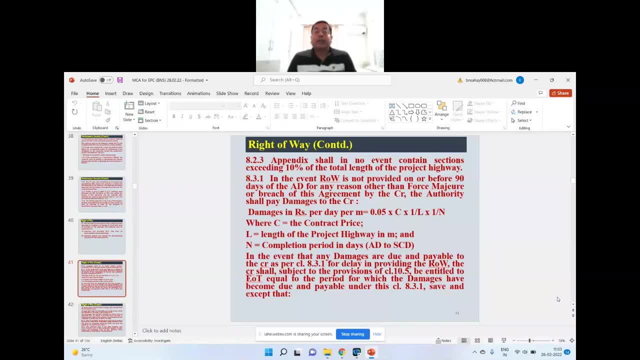 appendix. appendix contain only those parts of the land right of way which has not been made available to the contractor and it should not exceed 10% of total length of the project. having suppose your highways having 100 kilometer, the appendix should not contain more than 10 kilometers of total. 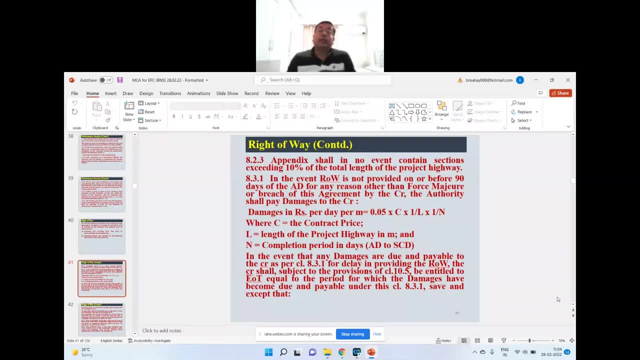 length of the project having so so. so, provided on or before 90 days from the appointed, you are having a relaxation of 90 days after signing of the agreement. appointed date after appointed, you will get 90 days to provide the right of way and for any reason other than force. 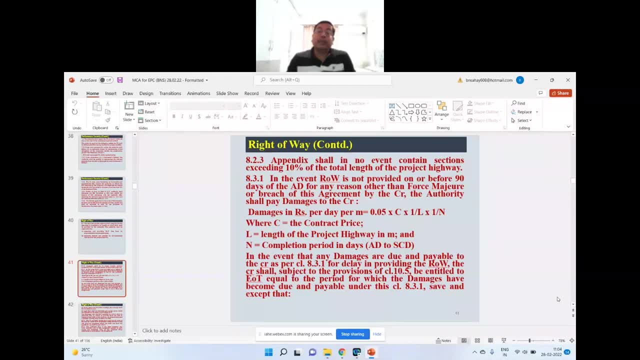 measure or bridge of this agreement by the contractor, the authority shall pay damages to the contractor. what is the quantum of damages? this is formulated here: damages in rupees per day per meter is equal to 0.05 into c, into 1 by l, into 1 by n. c is the contract price, l is the length of the project having meter. 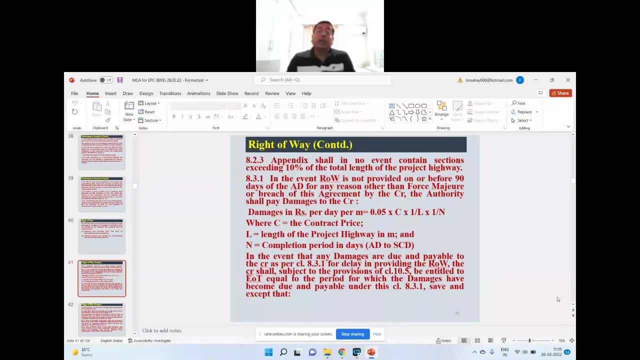 not in kilometer. l is the length of the project having meter because you are driving. damages in rupees per day per meter and 1 by n. completion period in days- not here in days- from appointed date to schedule completion date in the event that any damages are due and payable to the 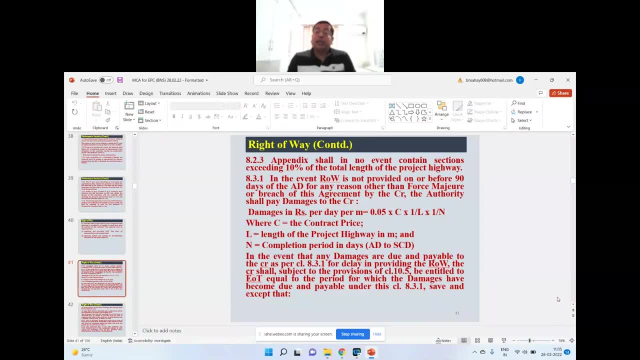 contractor as per clause 8.3.1, or delay in providing the right of way, the contractor shall, subject to the provision of clause 20.5, be entitled to eot equal to the period for which damages have become due and payable. you have not only to pay damages, you have to pay time, you have also to provide. time extension for that part of the road as per the clause 10.5. so be careful. in case of failure to provide right-of-way you will have to pay damages and time extension also target contract. you have to make the reason that if you do not have enough, no delay is. 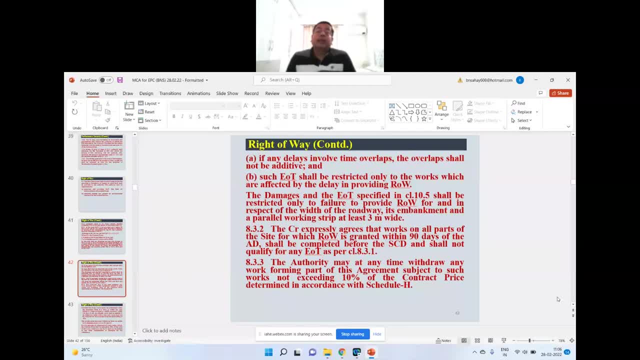 there any delay will be. the delay related to the ileover or 맛이 will be denied in. in case of calculation, if any delay involve time overlap, the overlap shall not be adding in. in case of delay involve time overlap, the overlap shall not be relative. such eot shall be. restricted only to the works which are affected by the delay providing our order. the dimension and the eote specified enclosed and place can be restricted only to failure to provide row for and in respect of the width of the roadway due to termination or Criminal Amendment Clause. 9.なて perseptiveケملیaki дов مع�生. 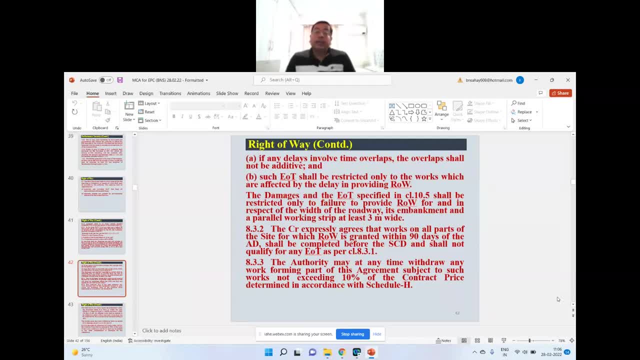 for and in respect of the width of the roadway, its embankment and a parallel working strip of at least 3 m. Suppose your right-of-way is 45 m. you have not to pay damages for all the things. If you are providing working front and a 3 m parallel strip, you have not to. 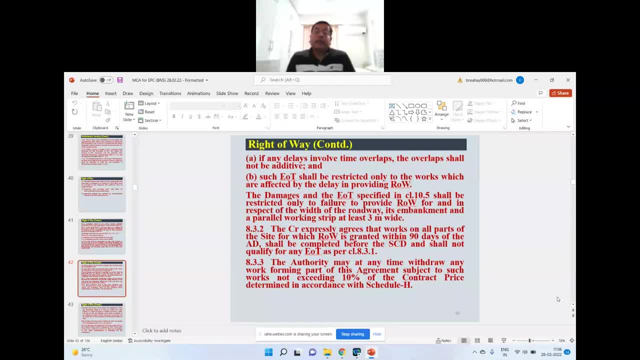 pay damages. This has been defined here. The contractor expressly agrees that works on all parts of the site for which ROW is granted within 90 days of the appointed date shall be completed before the schedule completion date and shall not qualify for any extension of time as per clause 8.3.1.. Is this clear? Contractor acknowledges that all parts of 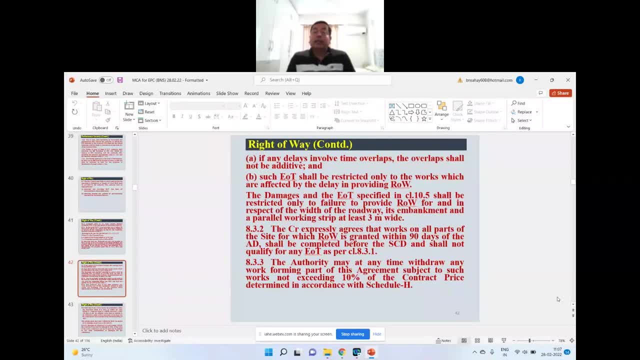 the road, including those which have been granted within 90 days of the appointed date, shall be completed before the schedule completion date and shall not qualify for any extension of time as per clause 8.3.1.. The authority may at any time withdraw any work forming. 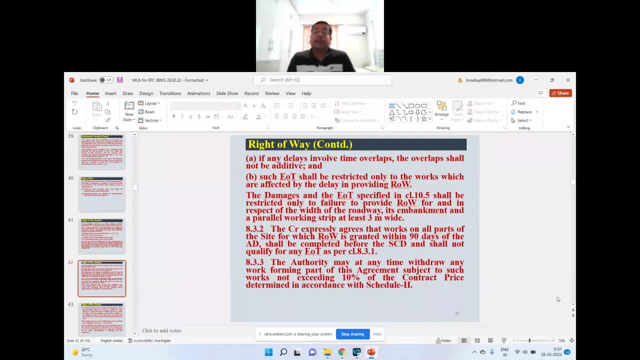 part of this agreement. See. this is also an overriding power of the authority that the authority may at any time withdraw any work forming part of this agreement, subject to such work not exceeding 10% of the contract price. Suppose the contract price is 500 crore. 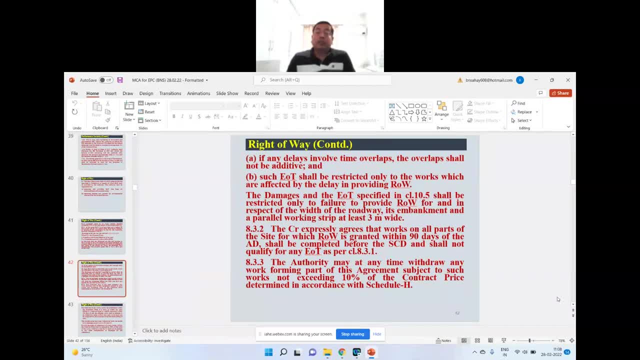 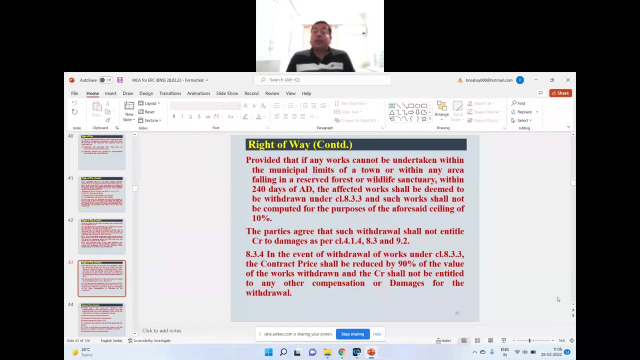 authority can withdraw work up to the quantum of 50 crore in accordance with the, and this will be determined in accordance with the schedule age, provided that if any work cannot be undertaken within the municipal limit of a town or within any area falling in reserve forest or wildlife sanctuary within 240. 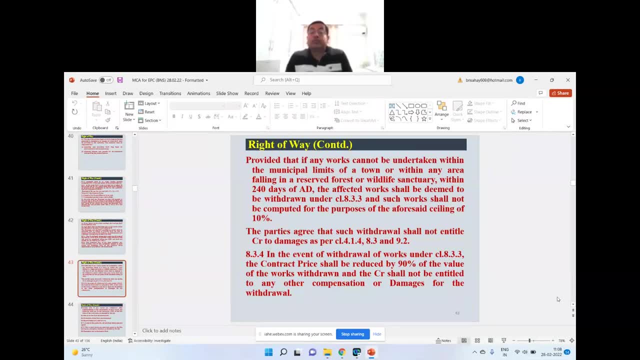 days of a punted date, the affected works shall be deemed to be withdrawn. the affected work shall be deemed to be withdrawn under project 1, 3, 1, 3 and such work shall not be computed for the purpose of their faucet ceiling often pattern. this 10% I defined in the Claude, but in case in some miss по limit. 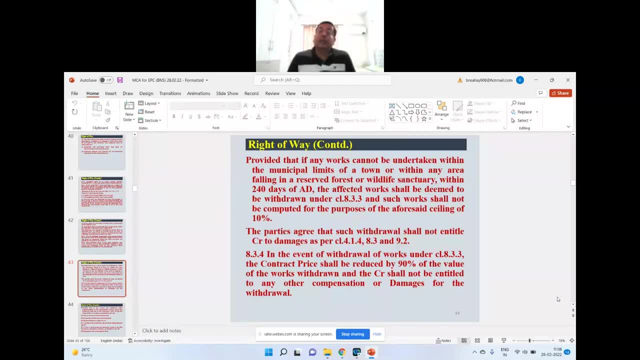 municipality is objecting that he will not allow, then in that case a 30 can withdraw it within 240 days of a punton ate and for this a 30 will not have to. but this will not be completed underมา wildlife sanctuary or municipality cases. this will not be counted. This is clearly. 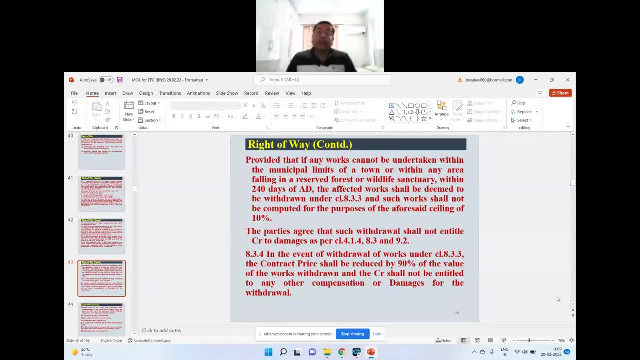 defined. The parties agreed that such withdrawal shall not entitle contractor to damages as per clause 4.1.4,, 8.3 and 9.2.. In the case of, or in the event of withdrawal of works under clause 8.3.3,, the contract price shall be reduced by 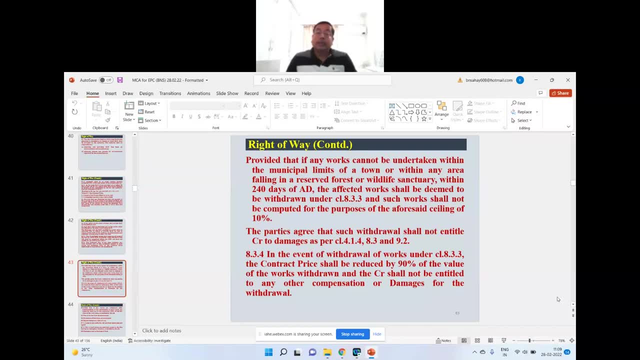 90% of the value of work withdrawn and contractor shall not be entitled to any other compensation or damages for withdrawal. In the case of in the event of withdrawal of work under clause 8.3,, he will get 90% The contract price shall. 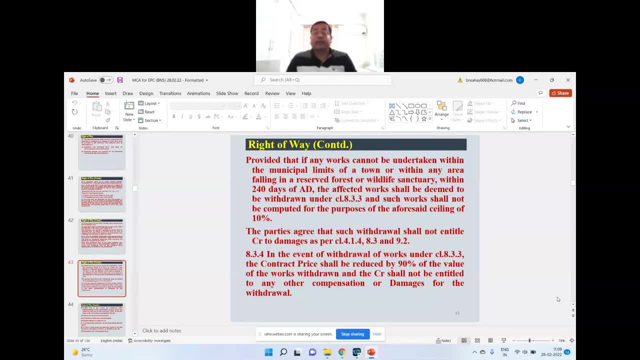 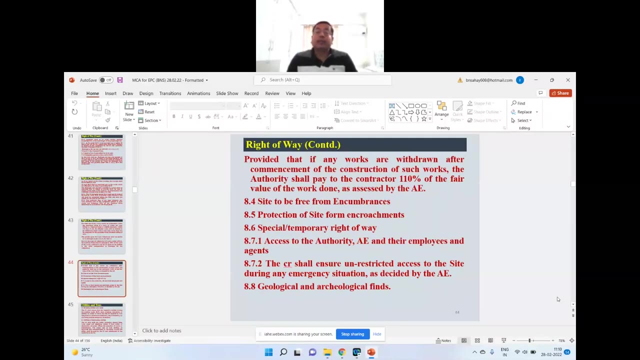 be reduced by 90%. That is 10% he will get and that is the compensation or damages and he will not get anything other than this. Provided further that if any works are withdrawn after commencement of the construction of such works, the 30 shall pay to the contractor 110% of the fair. 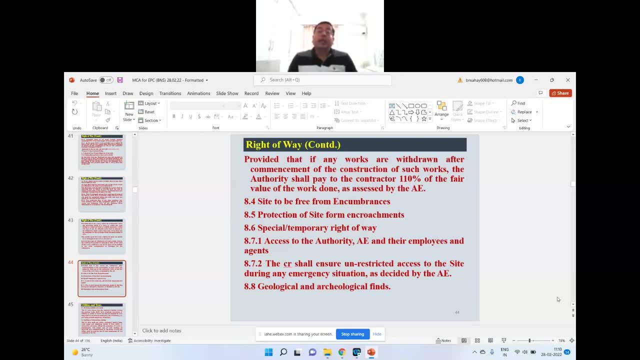 value of the work done as assessed by AE. Suppose wildlife sanctuary falls under your stretch and you have started work and now MOEF warned you not to work, Then in that case, if contractor has done some work, you will have to pay 110% of the fair value of the work done as assessed by the authority. 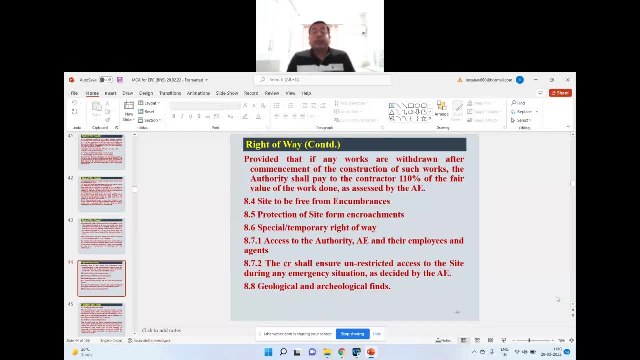 engineer Site should be free from incumbency. So you have to take all the steps that it is incumbency free, Protection of site from encroachments. You have to provide ROW free of encroachments and contractor is also required to keep it encroachment free. In case of any problem he will intimate it. to the authority. That's why you have to pay 110% of the fair value of the work done. Provided further that some encroachment is going to be happen or encroachments have happened and authority will clear it- A special temporary write-off way Suppose. 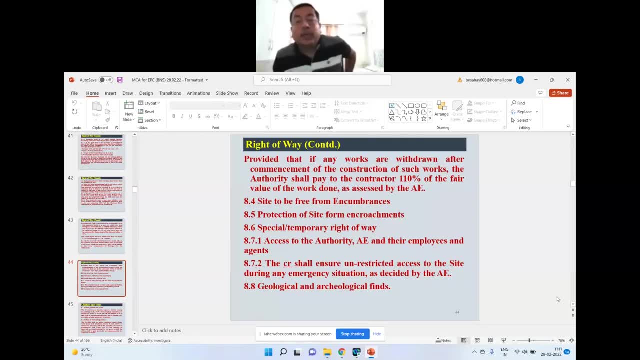 contractor wants to install GSB plant, WM plant or HMP, In that case he will require write-off way. This type of write-off way is known as a special or temporary. This type of a special, temporary write-off way has to be procured by the 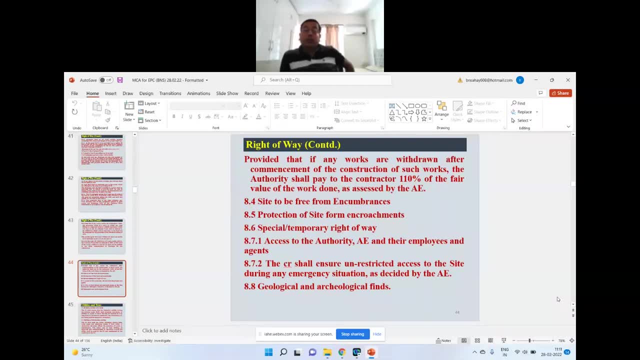 contractor on its own, at its own cost, and authority will clear it And authority will not provide. 8.7.1. Access to the authority AE and their employees and agents. All the contractor will give free access to the authority authority engineer and their employees and agents. Now, 8.7.2. The. 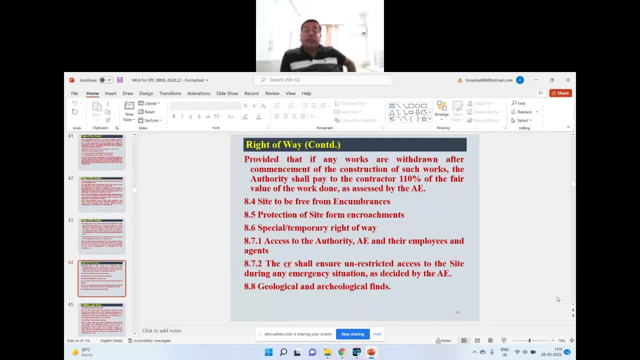 contractor shall ensure unrestricted access to the site during any emergency situation as decided by the authority engineer. This has to be ensured by the contractor that access to the site should be available for authority or authority engineer and in case of emergency, he can visit any any part of the site. 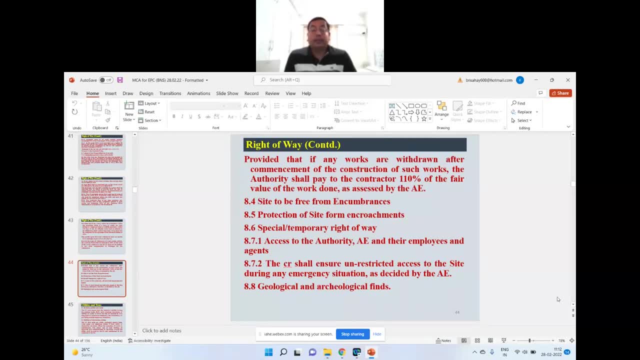 Geological and archaeological finds. What is this? Suppose you have entered into an agreement and work is going on after appointed date and later on it is found that some geological things suppose coal mines are there. Coal is beneath your road and mining department pointed out. in that case you will have to divert the road. 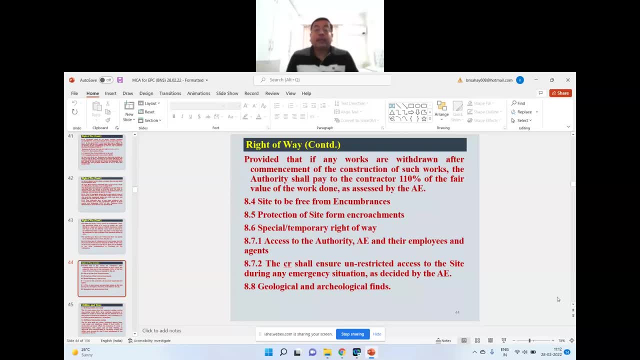 So contractor has not been granted right for mining. He cannot coal mine because he has been given contract only for construction of food. So in case of geological or archaeological finds, contractor has to back it, the site, by Short-term developer. If he doesn't. 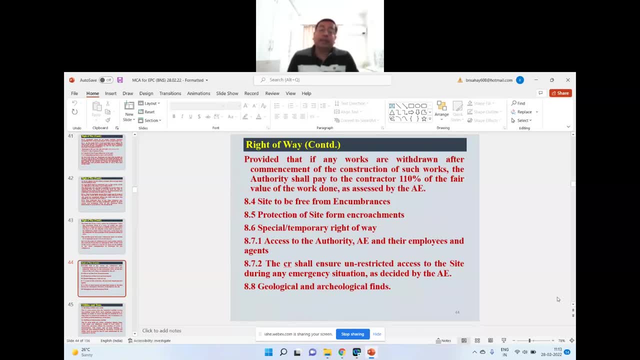 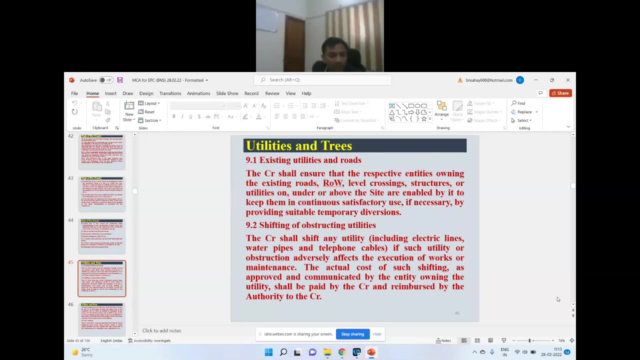 back at the site and for that he may get compensation, but he cannot mine it, he cannot do anything on the geological and archaeological site. excuse me, sir, yes, sir, i have a doubt sometimes. what happens that when we are omitting any scope, then we are giving 110 percent of that scope? we have this copy, so sometimes it's change of this covered under. 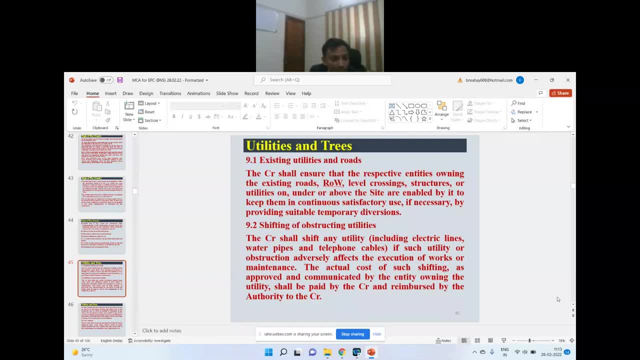 change of scope. like that we have omitted any scope and in place of that we are providing any other scope for working. like we have a disc of the five meter carriageway and providing seven meter carriageway. that case also, we have to give 110 percent or not, sir? your question is in case. 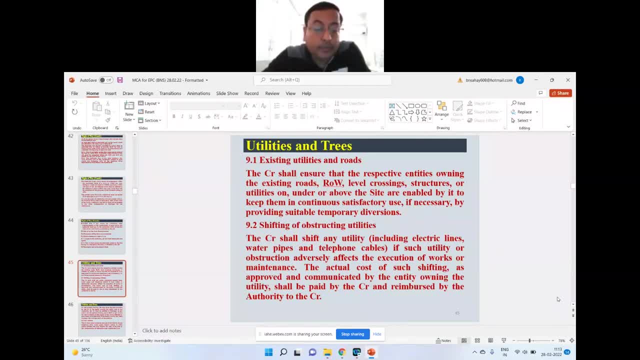 of geological finds, you have to divert, oh, sir. and in the case of any change of scope, sir, yes, sir, whatever scope we are descoping, in every case we have to pay 110 percent, sir, no, in case you can withdraw 10 percent of the 10 percent of the length you can withdraw, it will retain the agreement. 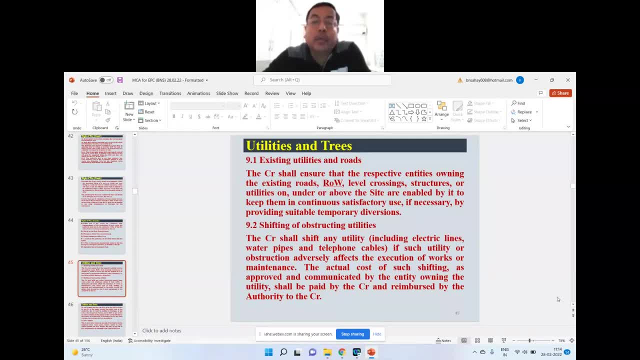 but this will not include mentally limits and wildlife sanctuary. and in that 10 percent also he will get 90 percent. should not change. yes, if he can withdraw, they should gift the Jest property percent. 90 percent will be. it means he will get the 10 percent, so he is not going to lose. but 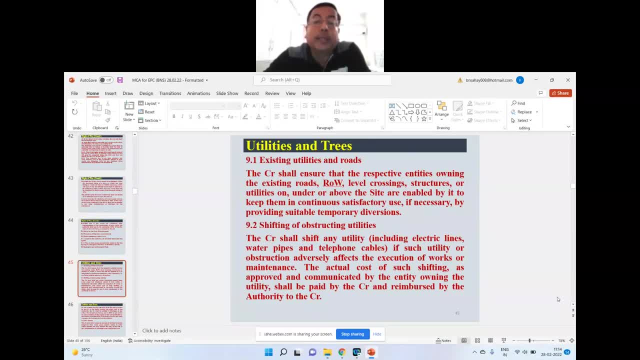 this is the final compensation. no other things will be allowed by the authority. this is the case and in case in case it is worked. it has worked something in wildlife portion and on latter date you have to not to work, then you will give 110 percent of the work. suppose a culvert has been. 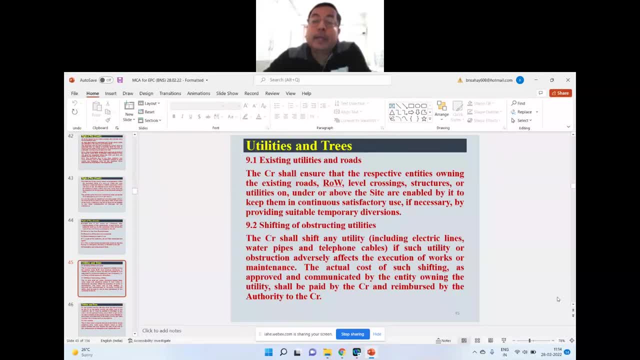 constructed by him in the portion which has been restricted by wildlife, then the cost of the culvert multiplied by 110 percent will be paid to the contractor. talk about any area which doesn't cover under wildlife sanctuary. if you talk about in a normal area, like in our case, there was a 10 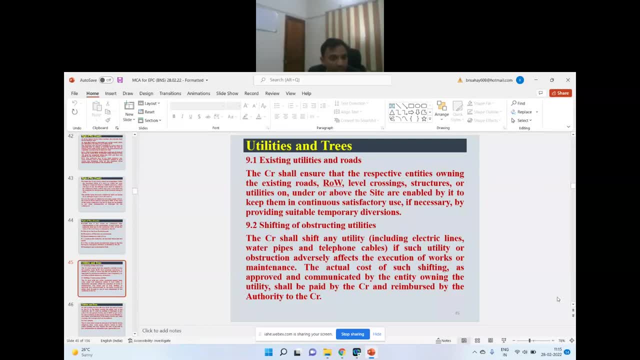 bus base was under the scope of contractor okay constructed eight bus base and for two bus base we were unable to provide the land, sir. okay, we have to discover 90 percent of value or 100 percent of value. 90 percent of that, sir, but in in our case we are providing in in place of bus base, another. 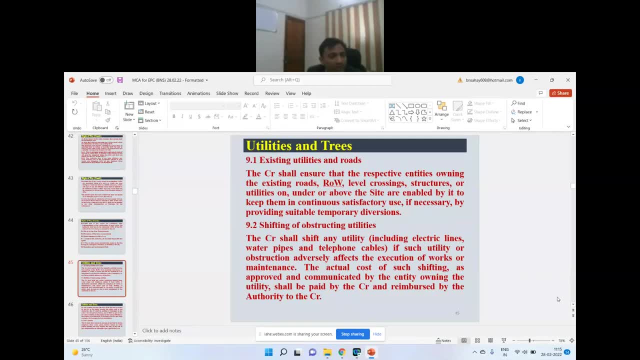 positive change of scope also we were providing. sir, it depends upon you. suppose your contractor agreed and he has given some undertaking or some affidavit, then you cannot deduct in, otherwise you will have to pay because it is your fault. two bus base cannot be constructed by the contractor. 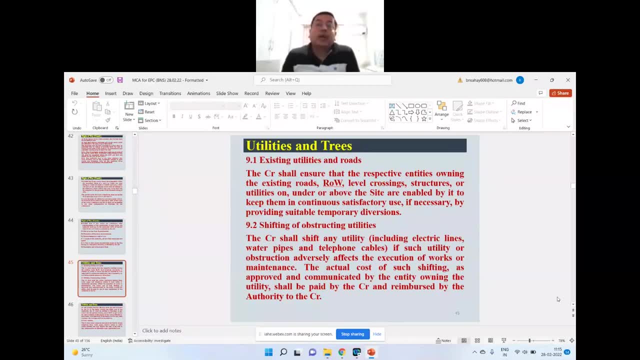 because you have not provided the requisite land. yes, sir, now he is entitled as per this segment, but if you can get him agreed that you don't charge instead of this, i will provide this, this one he may agree. so this is the agreement. but there are something beyond agreement you can do, and in many 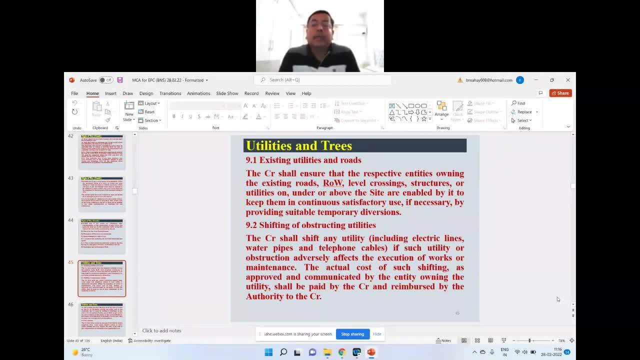 cases, contractor agree with you and then you can make the agreement and then you have to pay for it. you will have to pay because it is your fault. two bus base cannot be constructed by the contractor because may not deduct. it depends upon situation, site situation. you can handle it okay, sir. okay, thank you. 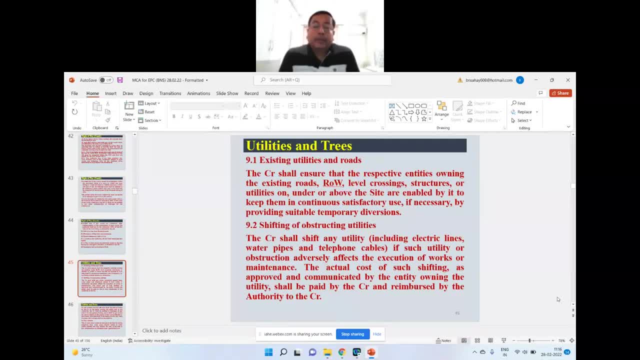 excuse me, sir. okay, 40 break, 15 sir, 15 minutes, 40 break. yes, sir, it means we will 11: 30 sir, 11, 30.. yes, sir, we will resume the session at 11: 30 sir. okay, thank you. thank you, sir. 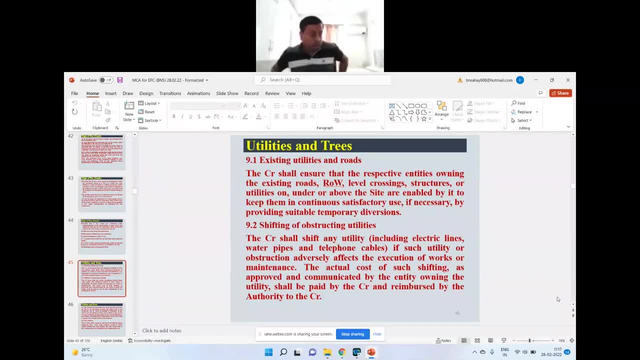 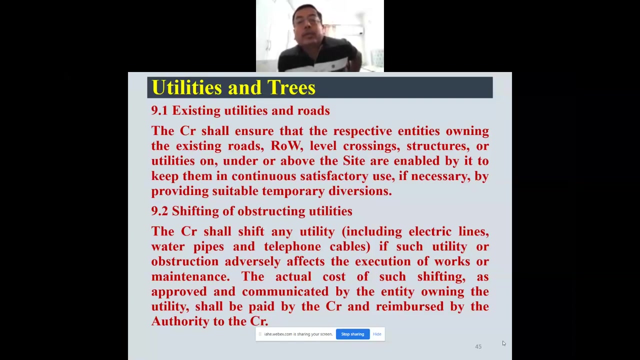 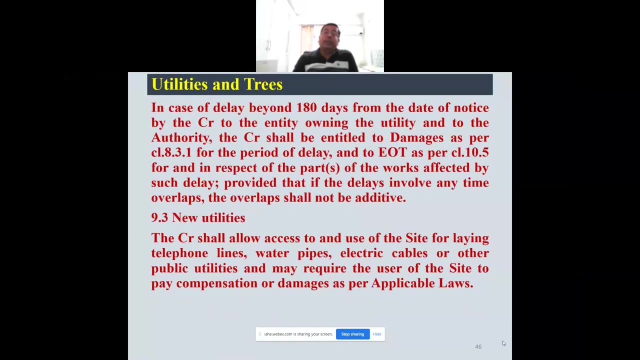 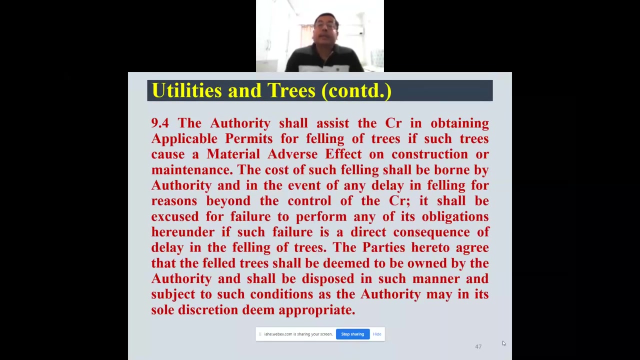 so so This is mentioned, otherwise your contractor will not allow any cable or water pipeline, then then it will be a problem for the area. the authorities shall assist the contractor in obtaining applicable permits for failing of trees if such trees call a material adverse effect on construction or maintenance. 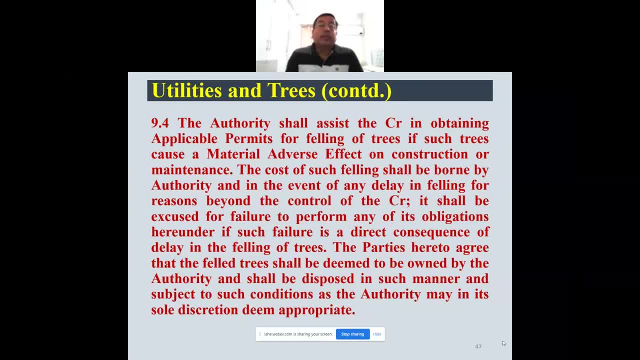 the cost of such failing shall be borne by the authority, and in the event of any delay in failing for reason beyond the control of the contractor, it shall be assumed for failure to perform any of its obligations here under if such failure is a direct consequence of delay in the failing of trees. so you have to. 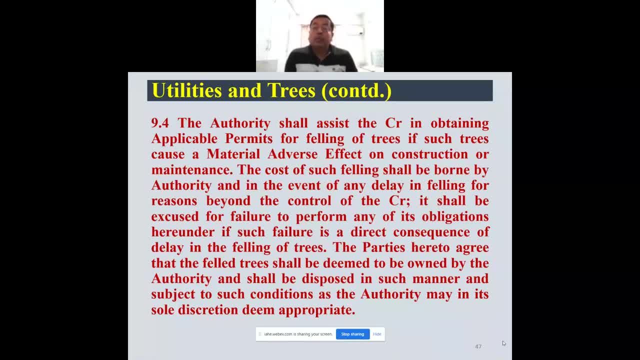 facilitate contractor for failing of trees and you have to reimburse the amount which is incurred by the contractor. the parties agree that the failed trees shall be deemed to be owned by the authority. the trees will be. owner of the trees will be authority and shall be disposed of in such a manner and subject to such. 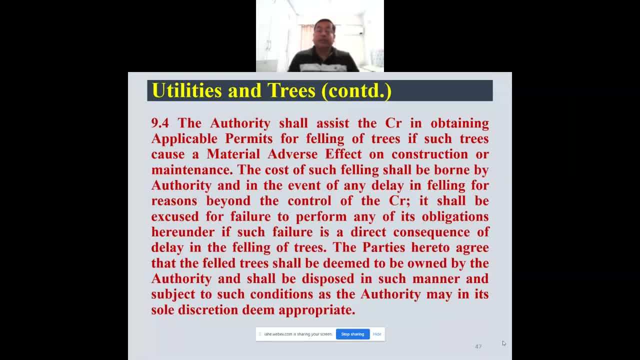 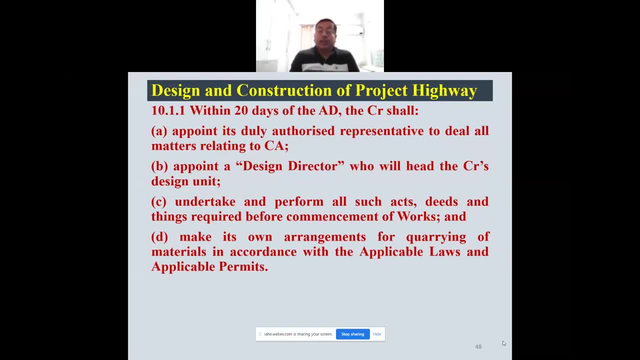 condition, as the authority may need sole discretion, deem appropriate. now coming to design and construction of project highway: within 20 days of the appointed date, the contractor shall appoint its duly authorized representative to deal all matters relating to the contract agreement. now suppose you have entered into an agreement and appointed date has been achieved. the contractor has to do. 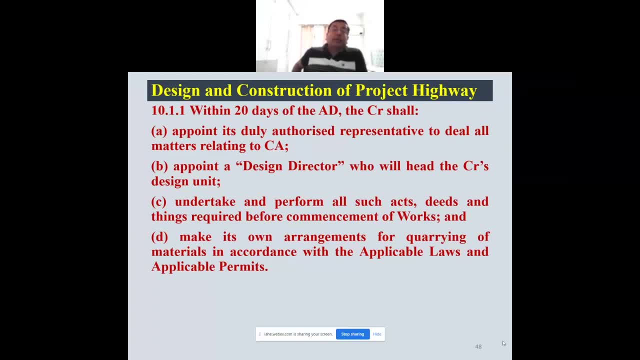 following things immediately within 20 days: first, appointed duly authorized representative to deal all matter relating to contract agreement. he has to point out, he has to mention that he is my authorized signatorett oxide representative. Second, appoint a design director who will head the contractor's design. 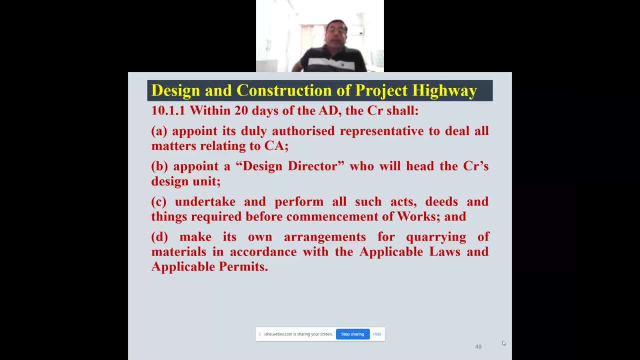 unit Third: undertake and perform all such acts, deeds and things required before commencement of works and make its own arrangement for querying of materials in accordance with the applicable law and applicable permits. So these are defined. that querying of materials is not the subject of. 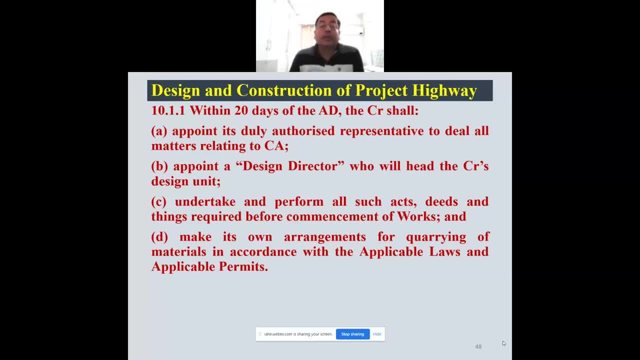 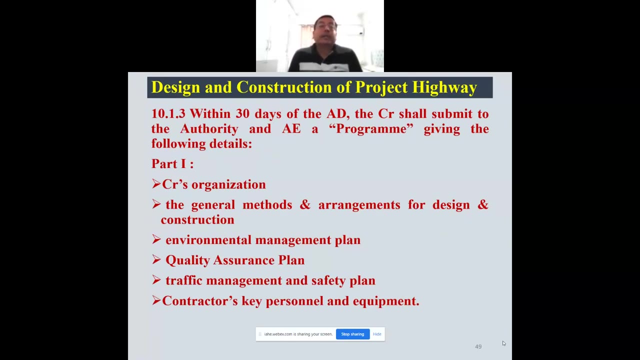 authority. it is the subject of contractor and he has to do as per applicable laws and applicable permits. Now, within 30 days of the appointed date, the contractor shall submit to the authority and authority engineer a program giving the following details: Now, within 30 days: 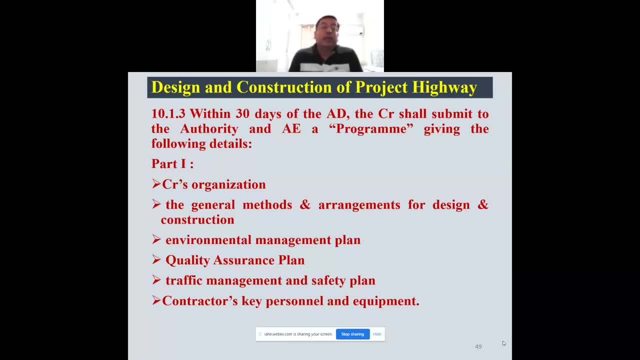 of appointed date contractor has to submit following First part one. Part one is contractors orders. Part two: contractors orders. Part three: contractors orders. Part four: contractors orders. He will show that he is my CMD, he is our board of director, he is some person. So all the. 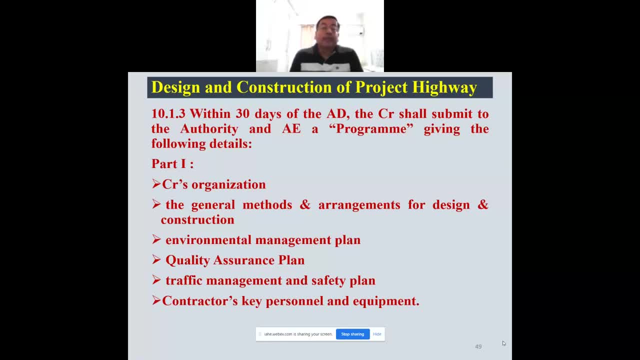 organization chart will be shown by the contractor in part one. The second is general methods and arrangement for design and construction. General methods and arrangements for design and construction will have to be given. Third is environmental management plan. He will also mention environmental management plan. Then he will also mention environmental management plan. Then he will also. 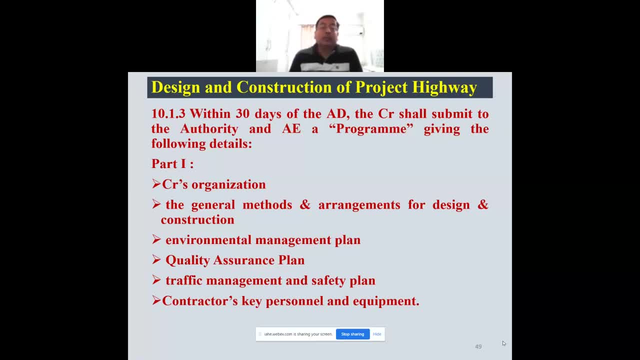 mention quality assurance plan. What is the measures which he is going to take? So these all things are mentioned in quality assurance plan. Next is traffic management safety plan. He has to take all the safety measures during construction, including traffic management, because you are 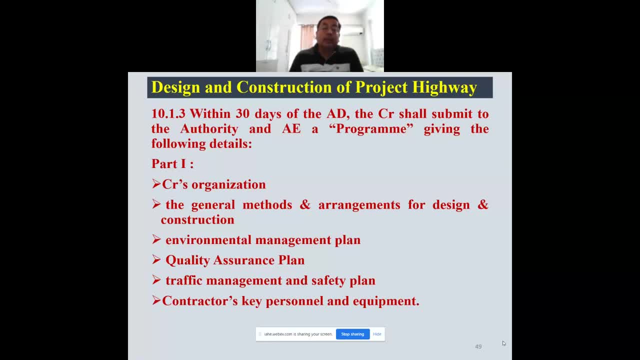 dealing a national highway and traffic has to be regulated. So traffic management is also very much important and contractor will regulate traffic and manage the traffic. So traffic management safety plan is to be done by the contractor. So he will also mention environmental management plan. 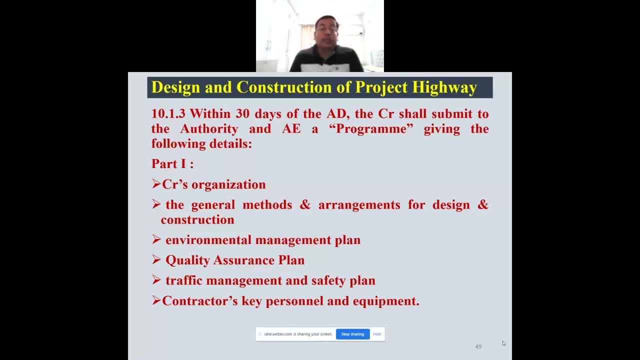 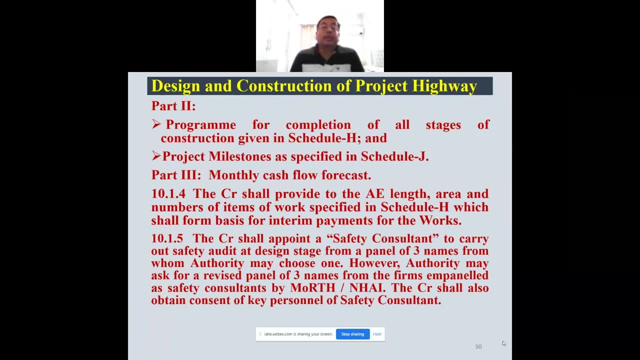 So traffic management safety plan is to be done by the contractor. Contractor's key personal and equipment is also to be mentioned by the contractor. Part two In part two: program for completion of all stages of construction given in schedule H In part two of the program he will mention completion of 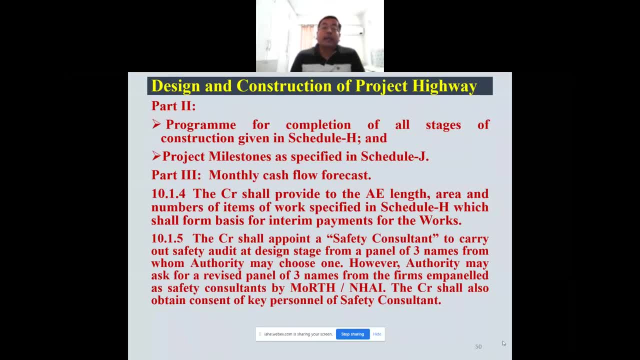 all stages of construction in schedule H and project milestones as specified in schedule J In part three. monthly cash flow forecast will also be mentioned. So he will also mention financial statements within schedule H. This part of contract has to be mentioned before he invests money under a schedule a. This part can also be mentioned. This is also known. 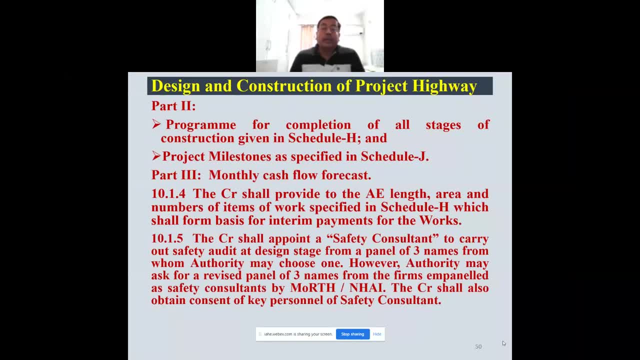 as S-curve. What is the quota of money he will invest it each quarter or each month will be mentioned The contractor. the contractor has to provide to the 30 linear length, area and number of item of items of work as specified in schedule H, which shall form basis for. 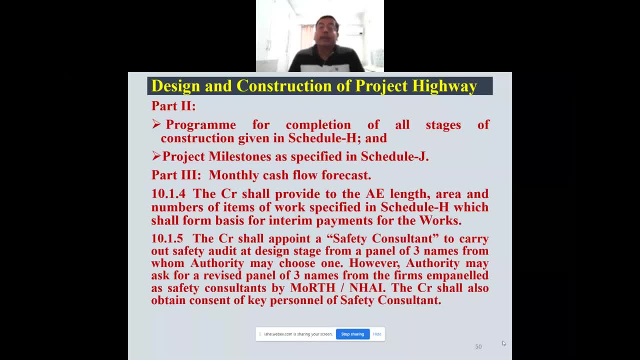 intrain payments for the works S-curve. Also to provide to the AE a 13-year length, area and number of item of works specified in Schedule H. Schedule H: what is Schedule H? In Schedule H, quantum of each and every component of work has been defined with its percentage. 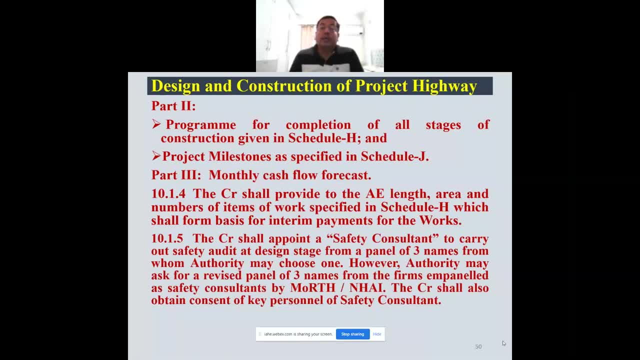 And this cell form basis for interim payment for the works. So contractor has to provide this also. The contractors have appointed a safety consultant, Now safety consultant. It is very much important to carry out safety audit at design stage from a panel of three names from whom authority may choose one. 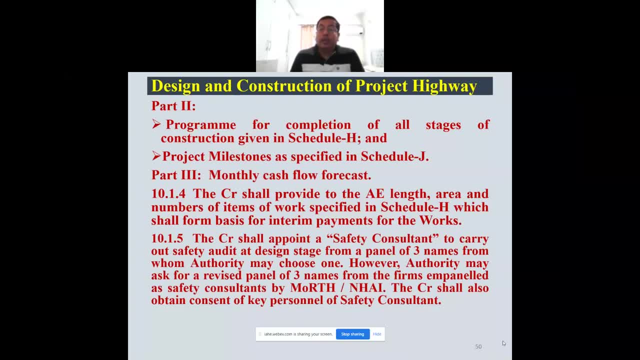 The contractor will send you a proposal of three company three safety consultant out of which you have to choose one. However, authority may ask for a revised panel of three names from the firms in panel as a safety consultant by MORTH or NHEI. 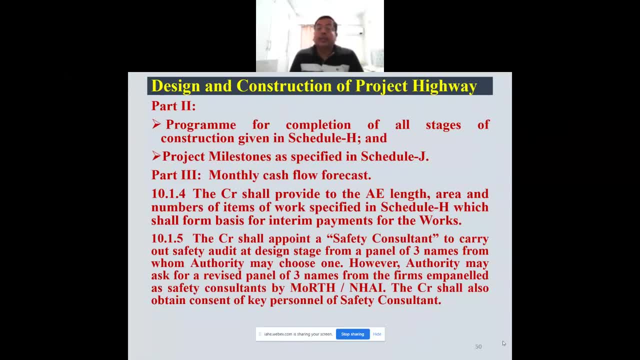 You may ask for another three Suppose. Suppose the three names of the companies you don't want to engage as a safety consultant. you may ask the contractor to furnish three names. The contractors have also obtained consent of key personnel of safety consultant. The contractor will also have to obtain consent of authority for key personnel of the safety consultant. 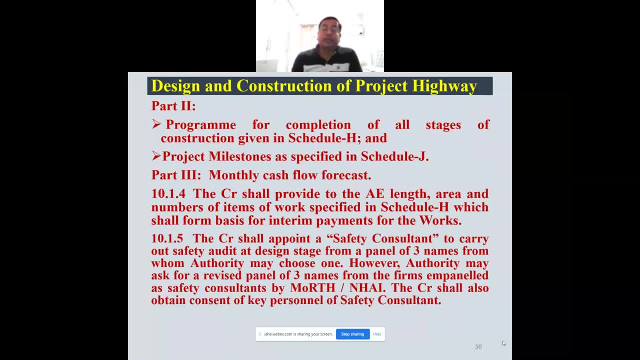 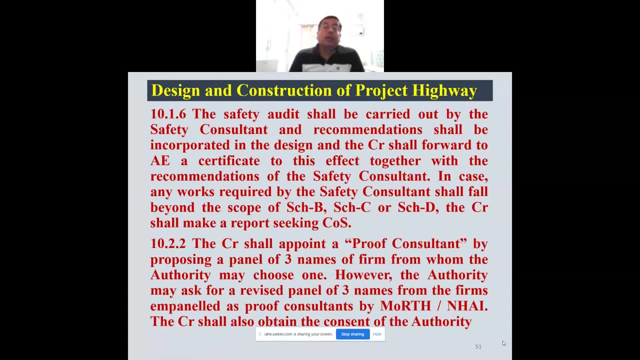 He will mention that these are the safety consultant personnel. Please give approval and you will have to communicate the approval. The safety audit shall be carried out by the safety consultant. The safety audit shall be carried out by the safety consultant. The safety audit shall be carried out by the safety consultant and recommendations shall be incorporated in the design and the contractor shall forward to a authority needed a certificate with this effect, together with the recommendation of the safety consultant. 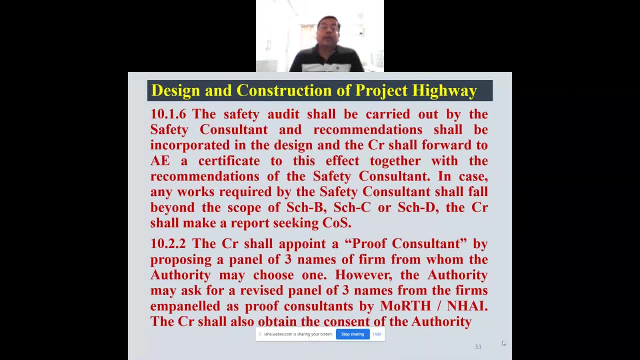 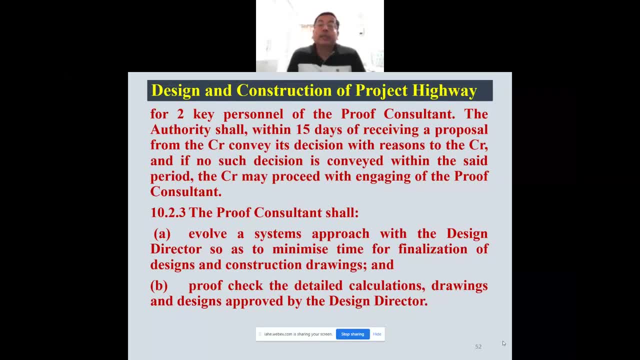 The safety audit shall be carried out by the safety consultant and recommendations shall forward to a authority needed a certificate, together with the recommendation of the safety consultant decision with regard to the contractor and if no such decision is conveyed within the said period, the contractor may proceed with engaging of the proof consultant. 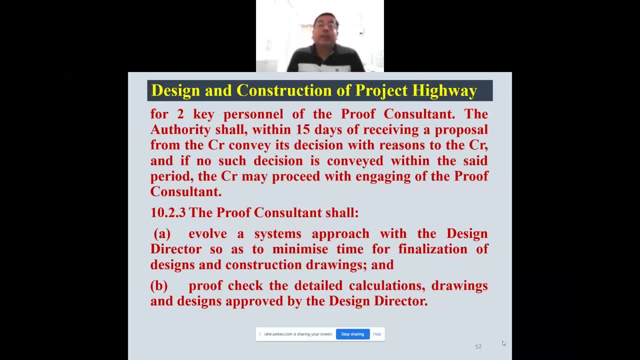 You have to finalize the proof consultant within 15 days. If you are failing, he may engage the proof consultant. The proof consultant shall evolve a system approach. What proof consultant will do First? evolve a system approach with the design director, Design director. who is design director? Design director is heading the design team of the 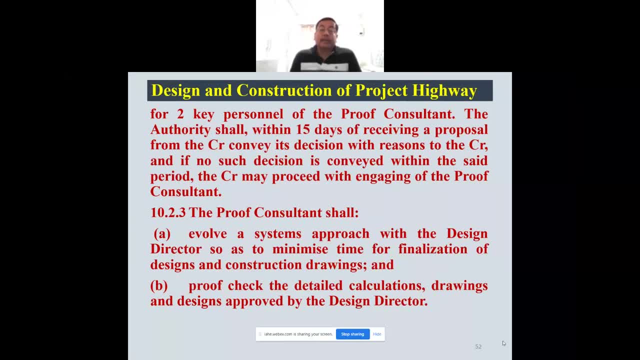 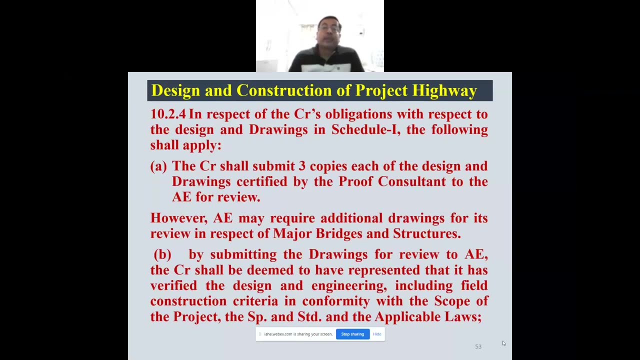 contractor so as to minimize time for finalization of design and construction drawings. And second, the proof consultant will proof check the detailed calculations, drawings and designs approved by the design director In respect of the contractor's obligation, with request, to with respect to the design. 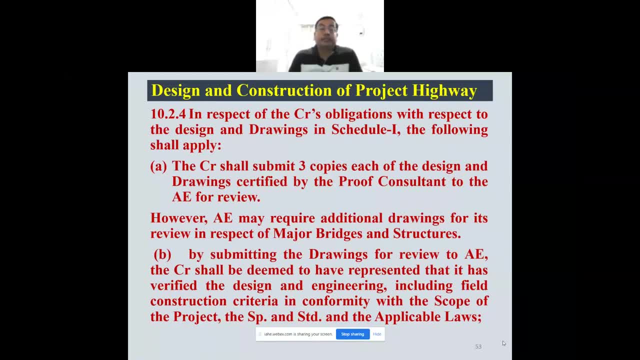 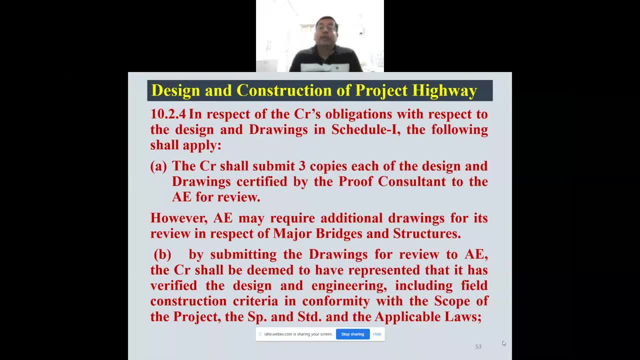 the same to proof consultant and proof consultant will check it and it will be certified by proof consultant to the authority engineer for review. However, authority engineer may require additional drawings in re for its review. in respect of major business structure, Suppose authority engineer has gone through the design, he may seek additional drawings for review, especially in case 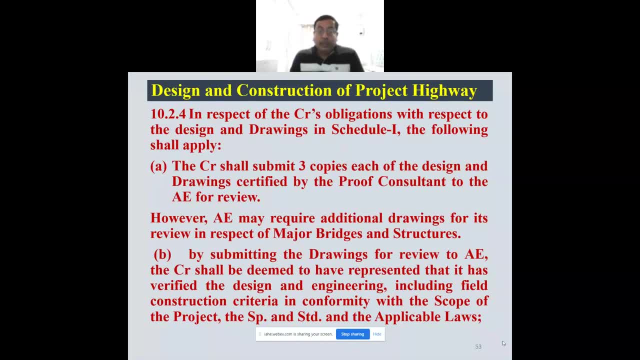 of major bridge structures. By submitting the drawings for review to the authority engineer, the contractor shall be deemed to have represented that it has verified the design and engineering, including field construction criteria, in conformity with the scope of the project, the specification standard and the applicable law. Once the contractor has submitted the drawing for 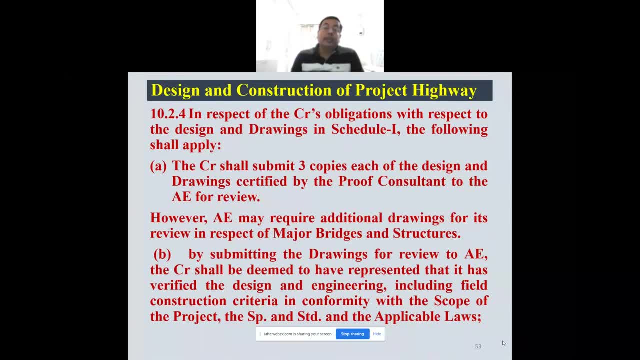 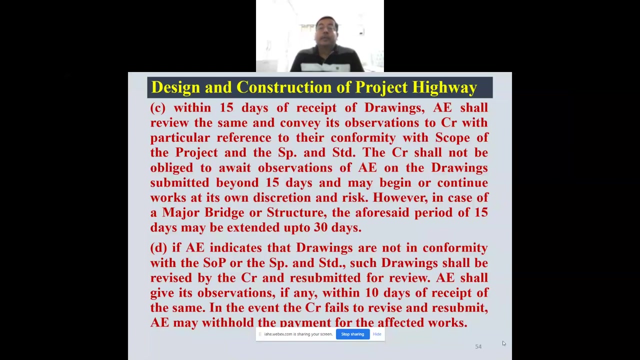 review to the authority engineer, it will be assumed it will be deemed that the contractor have represented, that it has verified the design and engineering, including field construction criteria and in conformity with the scope of the project, specification, standard and applicable law. Now, within 15 days of receipt of drawings, the authority engineer shall review the same. 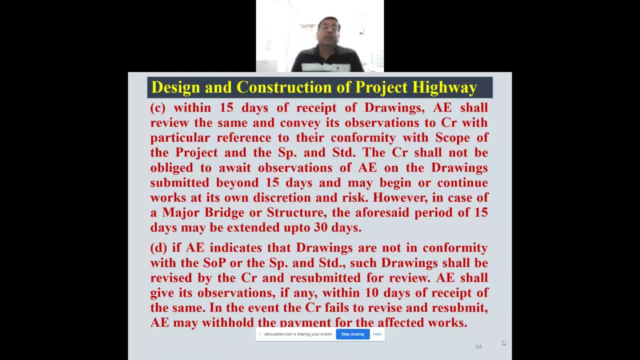 and convey its observation to the contractor, with particular reference to their conformity with the scope of the project and the specification standard. He will review and then he will send its observation or approve it. The contractor shall not be obliged to await observations of AE on the drawing. 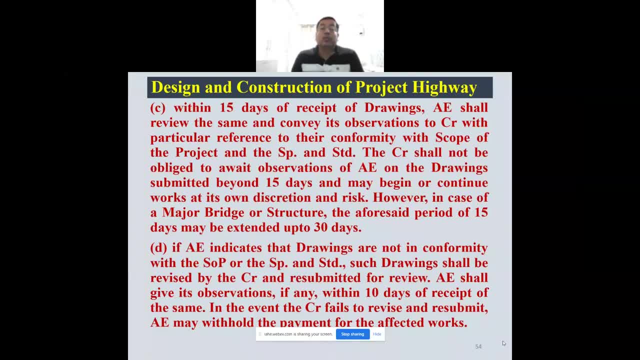 submitted beyond 15 days and may begin or continue works at its own discretionary risk. Suppose your authority engineer could not reply within 15 days. in that case contractor may start the work at its own direction and discretion and risk. however, in case a major bridge or structure, the 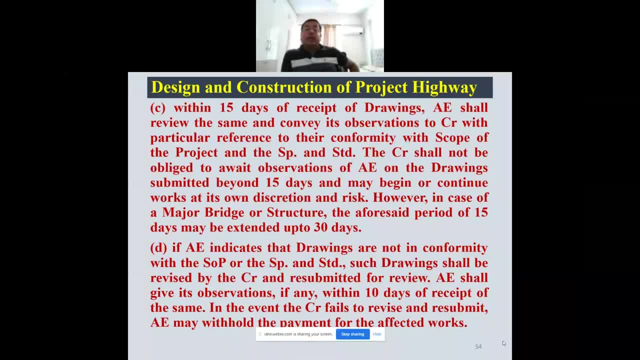 foresight period of 15 days may be extended up to 30 days. in case of a major bridge or a structure, this 15 days is replaced by 30 days. in that case, authority engineer has time of 30 days If authority engineer indicates that drawing are not in conformity with the scope of project. 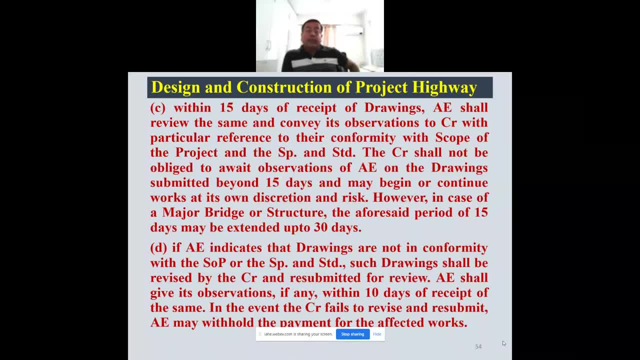 or the specification and standard. such drawing shall be revived by the contractor for review. AE shall give its observation. if any, within 10 days of receipt of the same Conductor, fails to divide and resubmit, AE may withhold the payment for the affected ones. So, 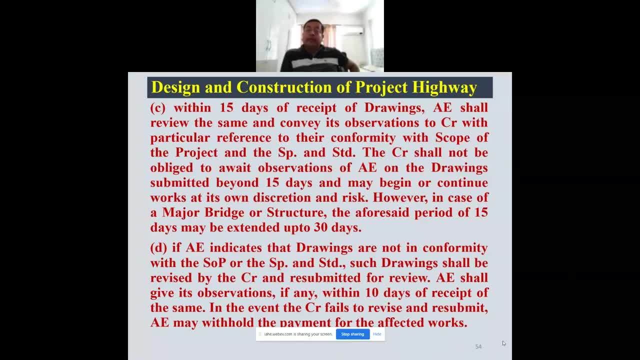 these are the things that the conductor will design. He will give it to the proof consultant. Proof consultant will review it and then it will send to a 30 engineer. A 30 engineer will review and give it, may ask for some additional drawings and within 15 days he will finalize. In case of a, 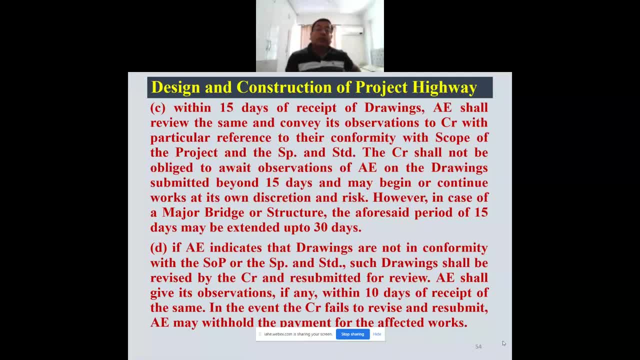 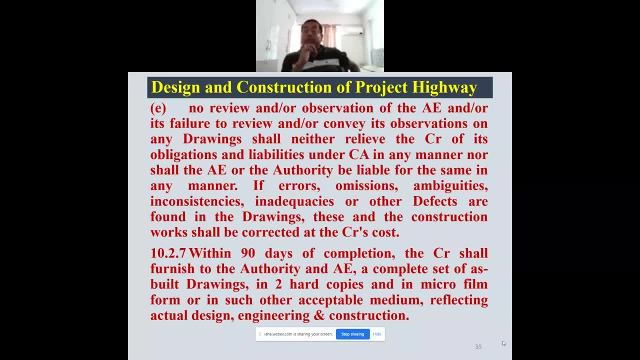 structure 30 days. So these are the mechanism for approval of design of the contractor by the authority engineer. No review and or observation of the authority engineer and or its failure to review and or convey its observation on any drawing shall neither relieve the contractor. 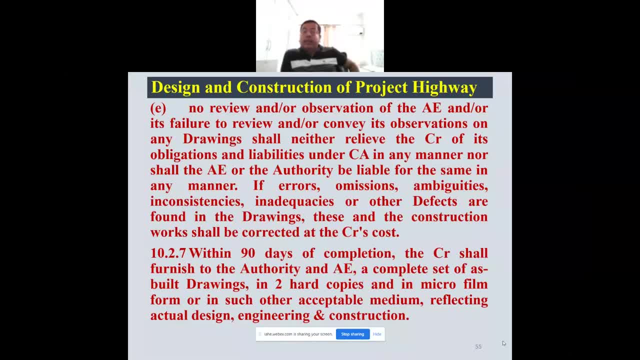 of its obligations and liabilities under the agreement in any manner. nor shall the authority engineer or the authority be liable for the same in any manner. Suppose he has started work, then contractor is solely responsible. He cannot say that I had submitted, but your authority engineer has not approved. I have no mistake, It is full. 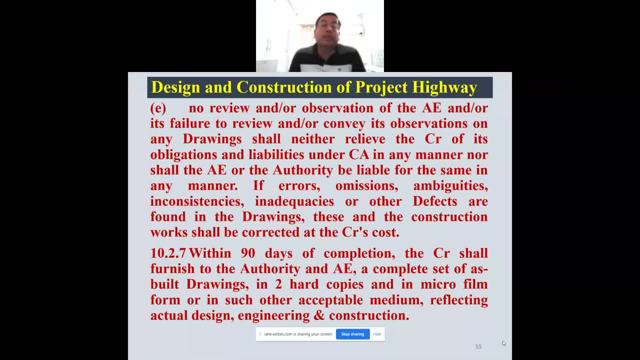 responsibility of the contractor. If errors, omissions, ambiguity, inconsistency, inadequacies or other defects are found in the drawings, these and the construction works shall be corrected at the contractor's cost. Then contractor will have to remedy it, rectify it, at its own cost, at the contractor's cost. 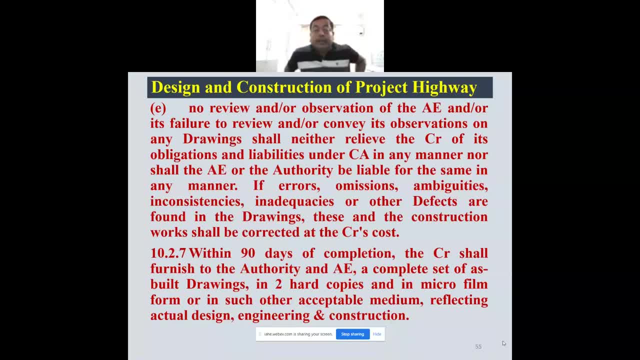 not at the cost of authority. Within 90 days of completion, the contractors have furnished to the authority and authority engineer a complete set of as-built drawings. within 90 days, The contractor shall furnish to the authority and authority engineer a complete set of as-will. 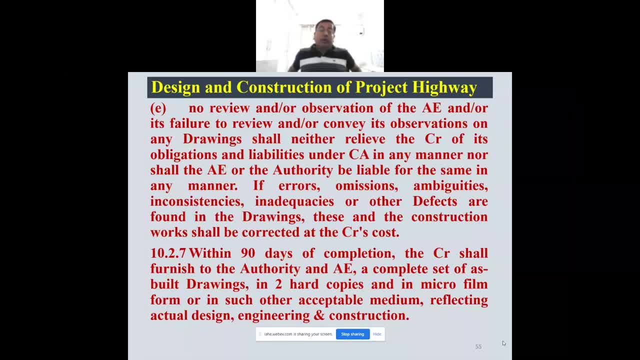 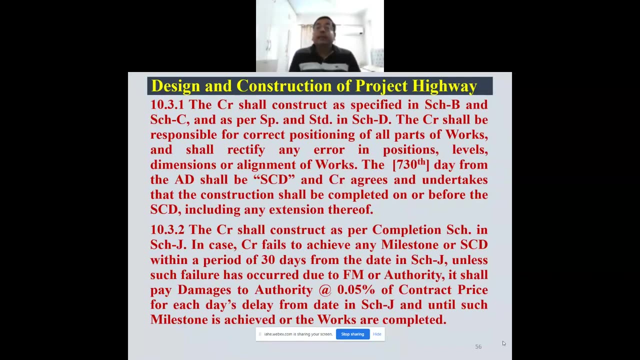 drawings in two hard copies and in microfilm form or in such other acceptable medium, reflecting actual design, engineering and construction. This has to be furnished by the contractor. The contractor shall construct as as specified in Schedule B and Schedule C and as per a specification standard in Schedule D. This I have already explained. 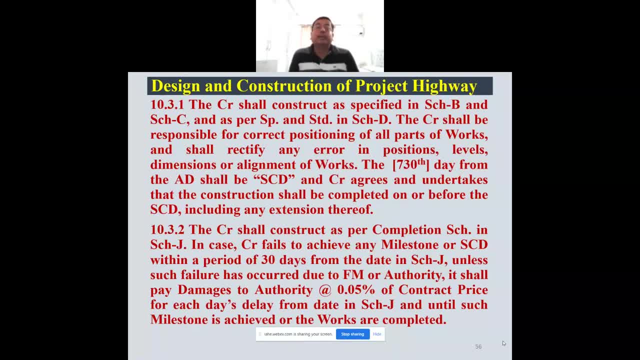 I think it is clear that contractor has to construct as per Schedule B and Schedule C. Schedule B is the modification and Schedule C is facilities and as per a specification standard of the manual and the orange book in Schedule D, The contractor shall be responsible for correct positioning of all parts of works. 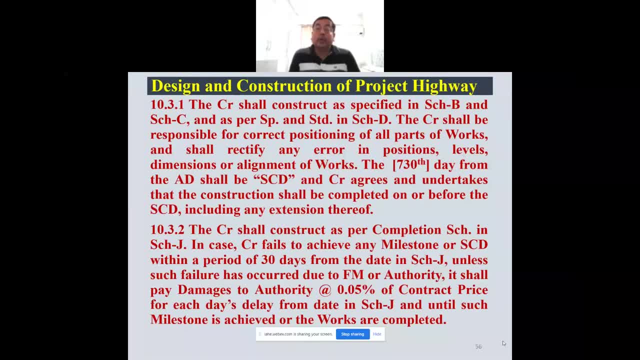 The contractor shall also be responsible for what Correct positioning of all parts of works And shall rectify any error in positions, levels, dimensions or alignment of works. Now the 7.30. it is written in square brackets. You can amend it. 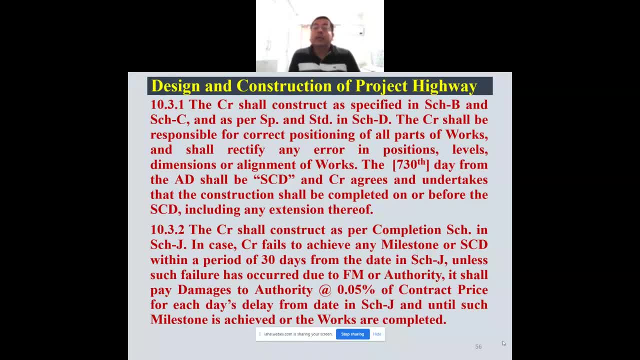 Suppose your work is going to be completed in 800 days, You can replace it with 800.. The 7.30th day from the appointed date shall be Schedule Completion date. And contractor agrees and undertakes that the construction shall be completed on or. 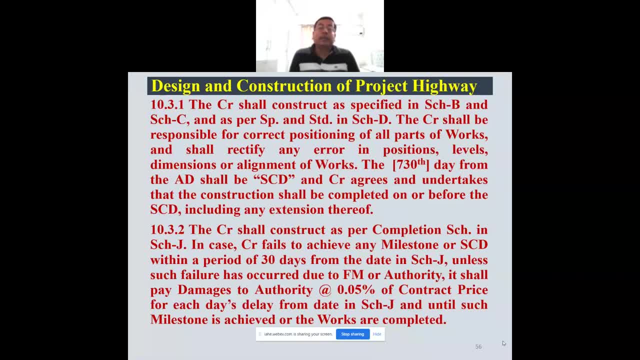 before the Schedule Completion date, Without any extension thereof. Now, 10.3.2. The contractor shall construct as per Completion Schedule in Schedule J. What is Schedule J? Schedule J is milestones which contractor has agreed and furnished to you in a construction. 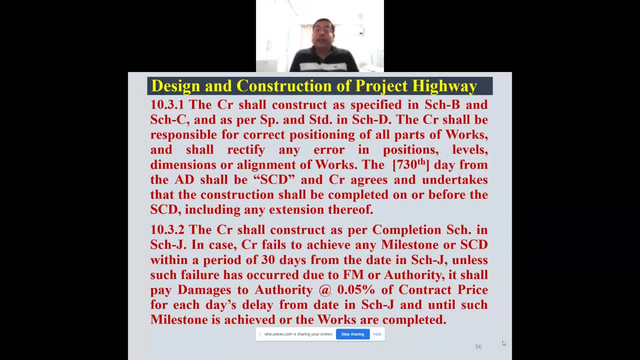 program. In case contractor fails to achieve any milestone or Schedule Completion date 30 days from the date mentioned in Schedule J, The contractor shall construct as per Completion Schedule in Schedule J. What is Schedule J Section Mentioned in Schedule J? Unless such failure as occurred due to force major or authority, it shall pay damages to. 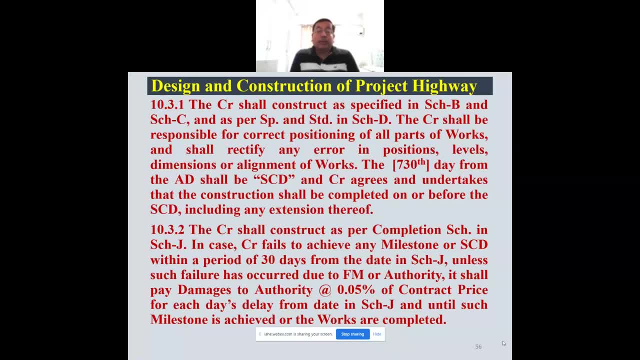 the authority at the rate of 0.05 Percent of contract rate for each day's delay from Date of Schedule J and until such milestone is achieved or works are completed. Slide 10. delivers contractor related results. It means in case of delay, if delay is not due to force major or authority, default he. 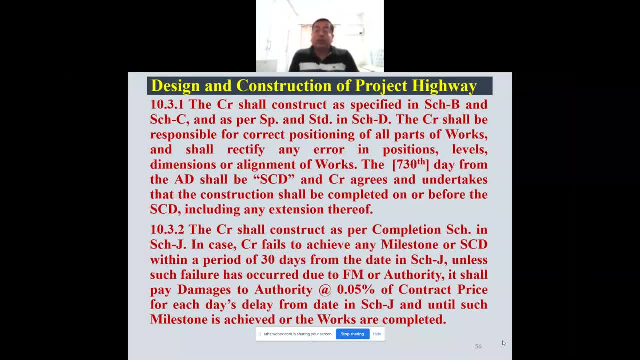 will pay damages to the authority at the FBI reporting. I anticipate 10.24 will be mentioned. Style also reflects premises of contract right on. 1 On between contract offline Ofre period rate of 0.05% of the contract price for each day delay for date in the Schedule J and until. 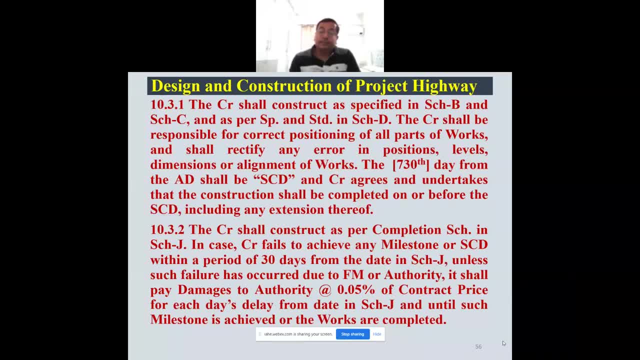 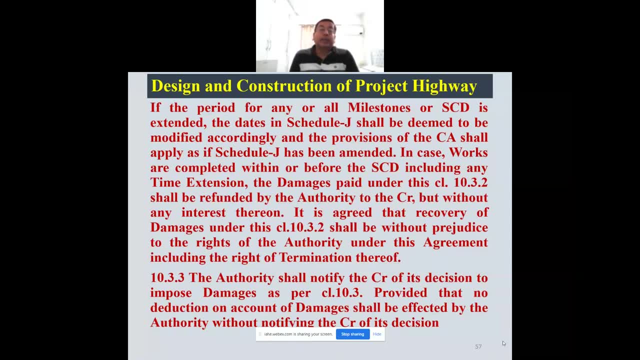 such milestone is achieved or the work are completed, If the period for any or all milestones or schedule completion date is extended. suppose you extended the milestone or schedule completion date. in that case it will be deemed that the Schedule J has been amended and we will accept. suppose you enhance every milestone. 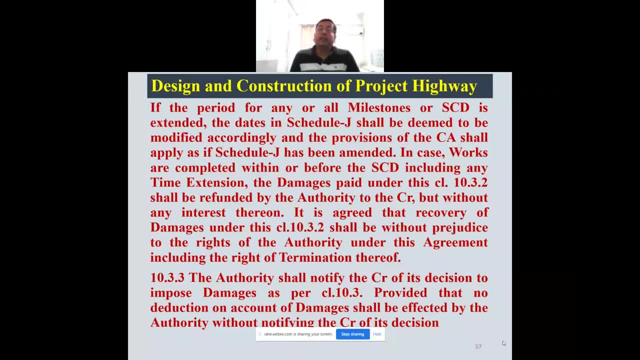 by 60 days and schedule completion date by 60 days, then this will be assumed, that this is the amended Schedule J and we will follow this as agreement In case works are completed within or before the schedule completion date, including any time extension. suppose work was to be completed within two years and you have given the time. 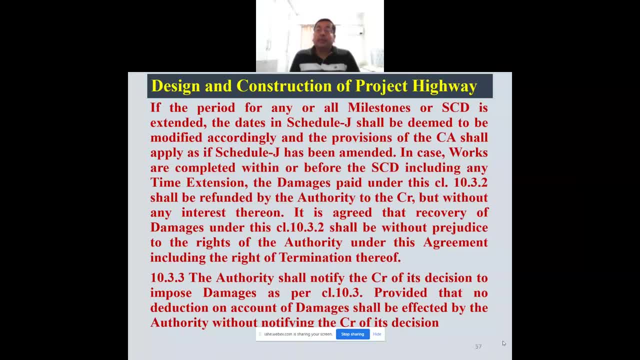 extension, The work has been completed within 60 days. The damages paid under the clause 10.3.2 shall be refunded by the authority to the contractor because he has completed the work within the extended time. that is the time approved by you, but without any interest. 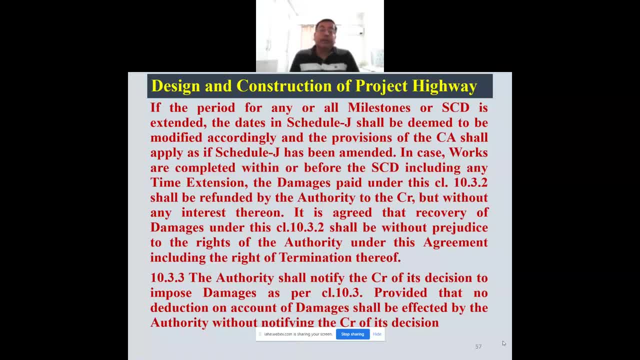 The damages you have deducted will be refunded, but without any interest. It is agreed that recovery of damages under this clause, That is, 10.3.2, shall be without penalty to the right of the authority under this agreement, including the right of termination. 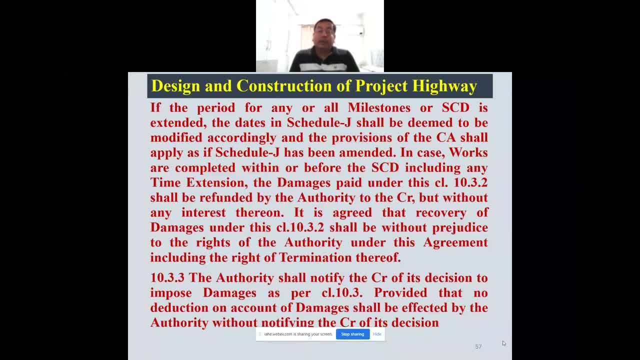 This is not only the damages you have deducted, but you are also having the right, including the right of termination. Suppose he is delaying the milestones, he is not achieving schedule completion date. in that case you can even terminate it. Not only damages is the remedy, but termination is the final remedy and you can go for termination. 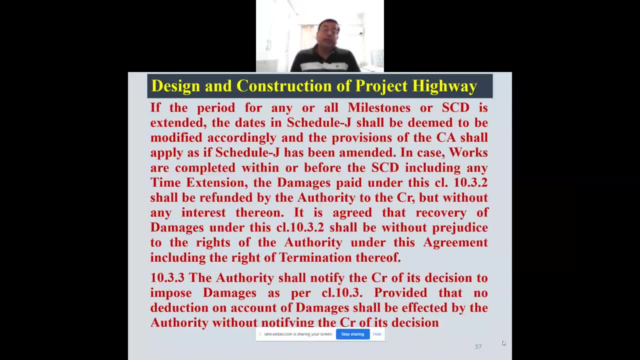 in that case- 10.3.3,- the authority shall notify the contractor of its decision to impose damages as per clause 10.3.. Provided that no deduction on account of damage shall be affected by the authority without notifying the contractor of its decision. 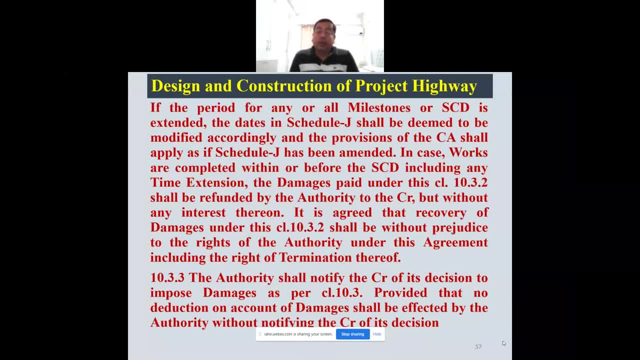 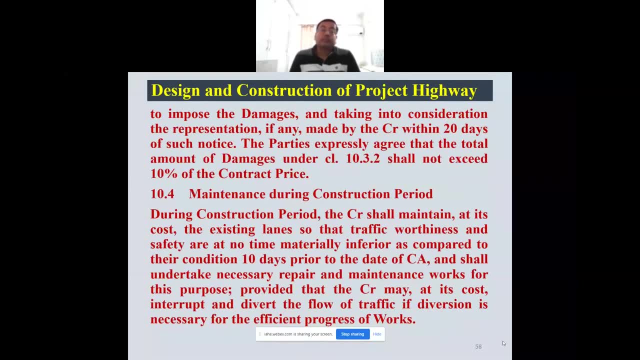 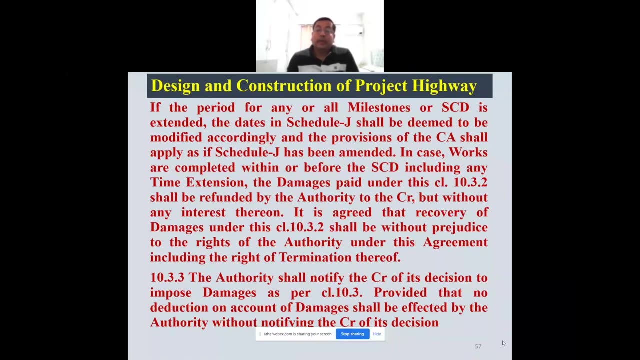 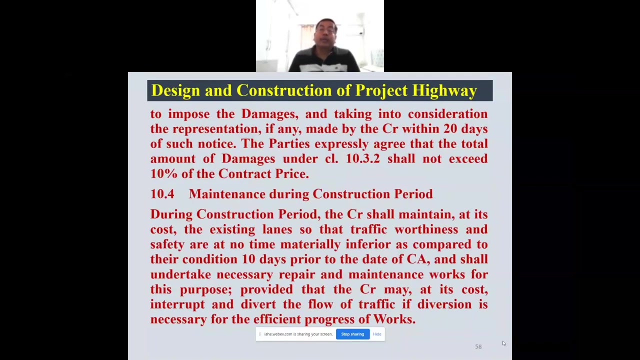 In case of damages, you have to first notify it. If you have not notified it, you cannot charge the damages. Okay, It means authority, without notifying the contractor of its decision, to impose the damages and take into consideration the representation of any made by the contractor within 20 days. 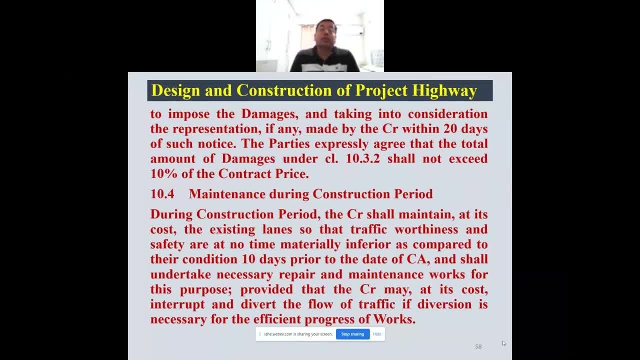 of such notice, The parties expressly agree that the total amount of damages under clause 10.3.2 shall not exceed 10% of the contract price. In any case, the total damages which you are charging to the contractor will not exceed 10% of the contract price. 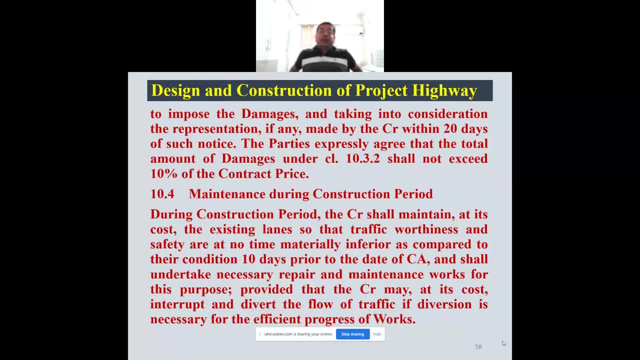 This is very much important that in case of authority you are having only 1%. You have to pay maximum damages to the contractor at the rate of 1%. It has not to exceed 1%. In case of damages by the contractor, it may not exceed 10% of the contract price. 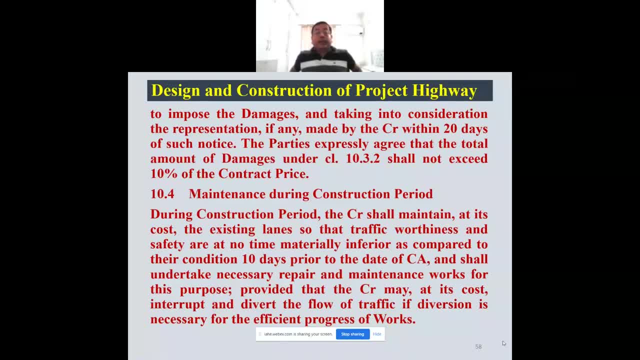 Now maintenance during construction period. I have earlier dealt maintenance during development period. That is again The contractor has not been given a pointed date. Then authority has to maintain the road in traffic worthy and safe condition. Now 10.4: maintenance during construction period. 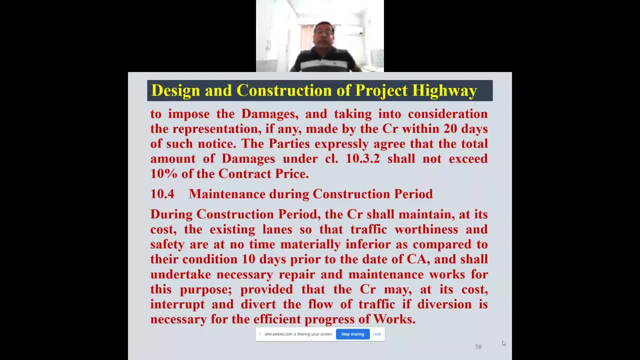 During construction period, the contractor shall maintain, at its cost the existing lanes so that traffic worthiness and safety are at no time materially inferior as compared to their condition 10 days prior to the date of this agreement, and shall undertake necessary repair and maintenance works for this purpose. 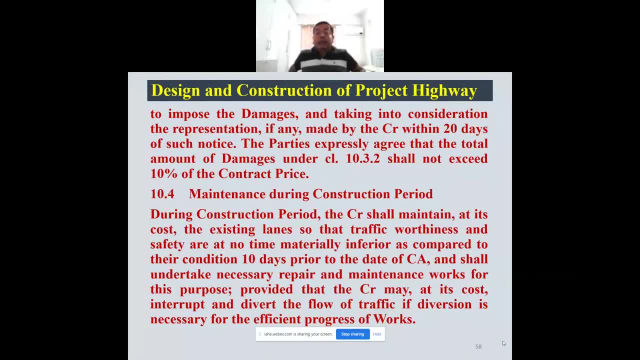 So the contractor will have to keep the road in traffic worthy and safe condition and will not be inferior as compared to their condition 10 days prior to the agreement, and shall undertake necessary repair and maintenance works for this purpose, Provided that the contractor may, at its cost, interrupt and divert the flow of traffic. 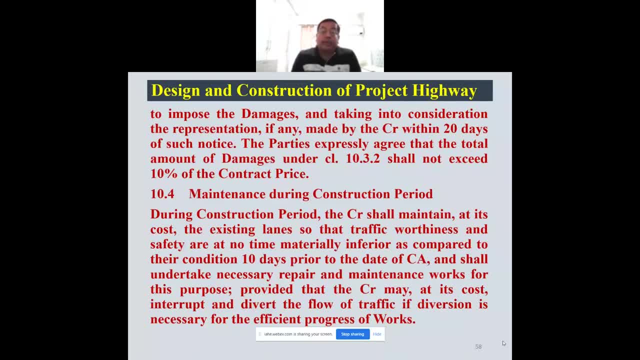 Suppose some diversion is required, he may construct a diversion if necessary for the efficient progress of work. Suppose work Can be expedited by construction of a diversion. he will construct a diversion, but he will not charge it. It is in his scope. 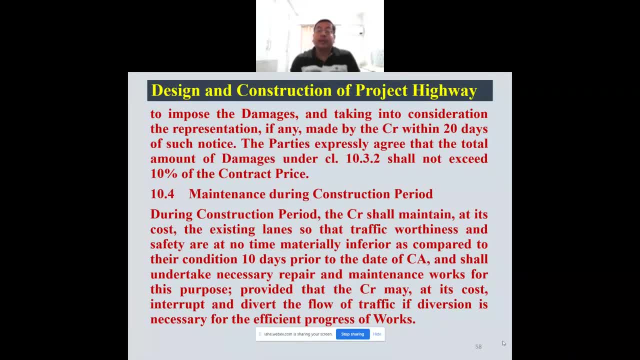 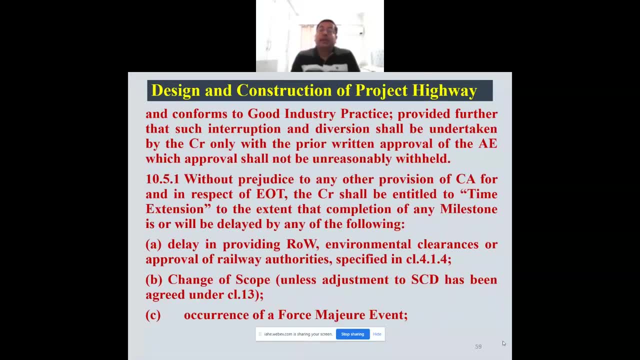 It will be assumed that it is in the scope of the work and a diversion will be constructed by the contractor, Provided further that such interruption and diversion shall be undertaken by the contractor only with prior written approval of the authority engineer To interrupt the traffic or prepare diversion, construct diversion. in that case he will. 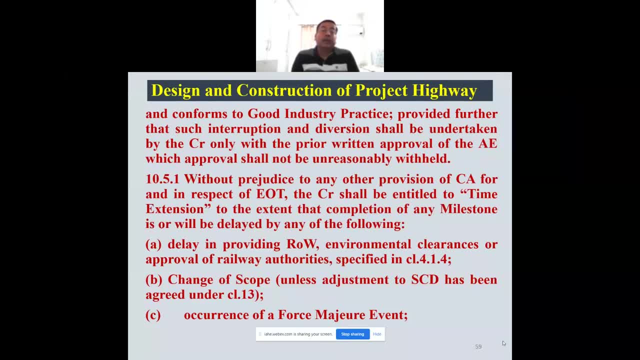 seek prior approval- written approval of the authority engineer and which approval shall not be unreasonably withheld by the authority engineer. Now, 10.5.1.. Without prejudice to any other provisions of the agreement for and in respect of extension of time, the contractor shall be entitled to time extension. 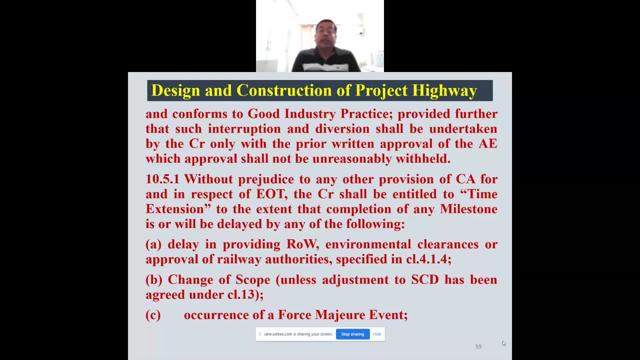 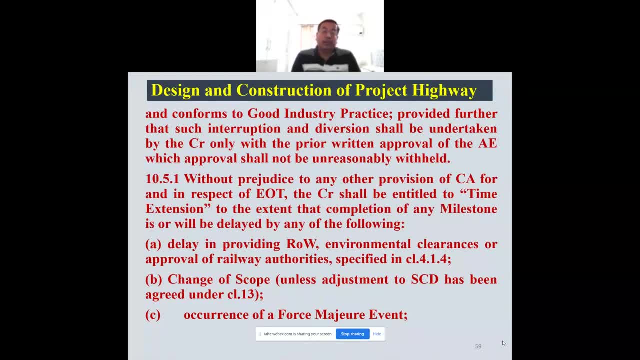 First, delay in providing ROW. Suppose you are, you have delayed in providing ROW. Second, environmental clearances or approval of railway authority as specified in clause 4.14.. This is a clause for EOT. Second is change of scope. 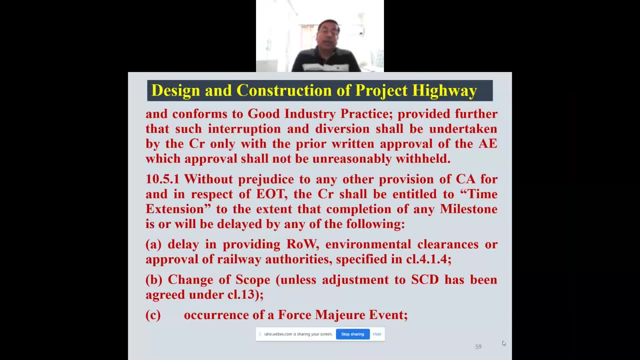 Suppose some change of scope, Suppose some change of scope has been given. Suppose two minor buildings, three culverts are also to be incorporated, also to be constructed, Then this change of scope will have impact on the time extension. So he may seek time extension. 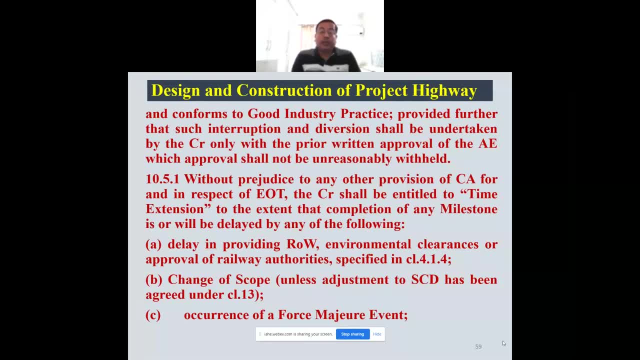 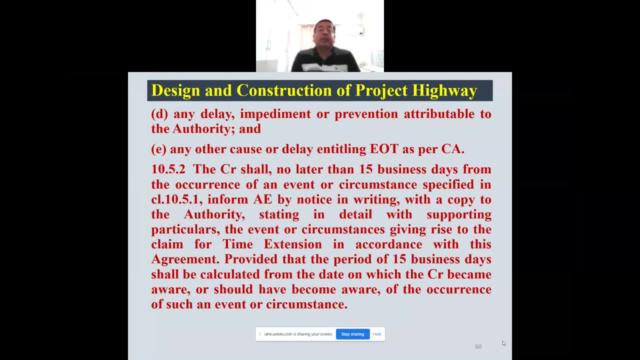 Occurrence of a force major event. Suppose flood has come and flood water remained for 60 days, Then this will also be for a cause for the time extension. Third, Any delay, impediment or prevention attributable to the authority. Suppose you you have not given something which is required by the contractor. 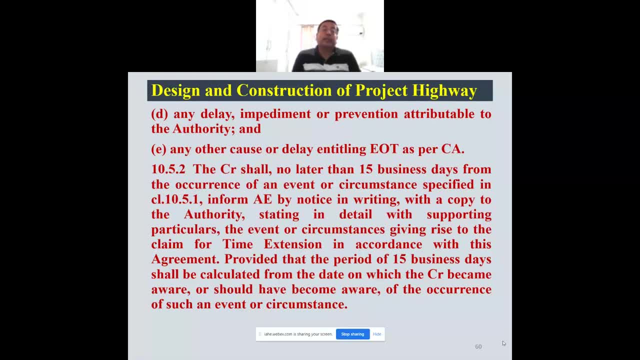 Then this will also be attributable for time extension. Any other cause or delay entitling EOT as per CA, Any other cause or delay may also be part of time extension. 10.5.2.. The contractor shall know later than 15 business days from the occurrence of an event. 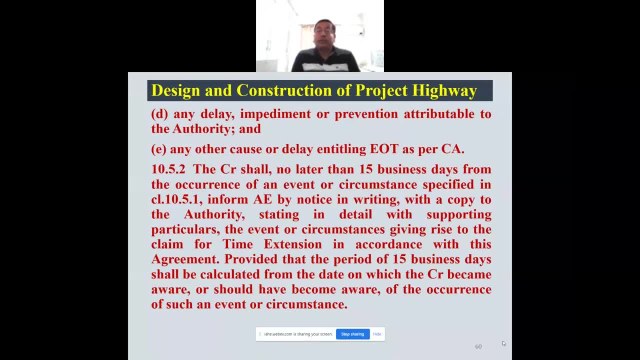 Or 10.5.2.. The contractor shall know later than 15 business days from the occurrence of an event, Or 10.5.2.. The contractor shall know the circumstances as specified in cld 10.5.1.. 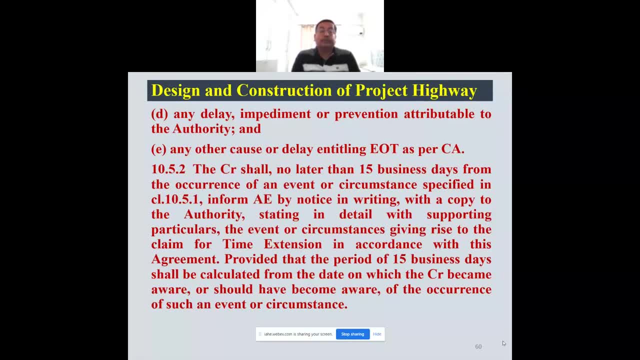 Inform authority engineers by noticing writing, with a copy to the authority, stating in detail, with supporting particulars, the event or circumstances giving rise to the claim for time extension in accordance with this agreement. Within 15 days, he will furnish a detailed time extension proposal as per this agreement. 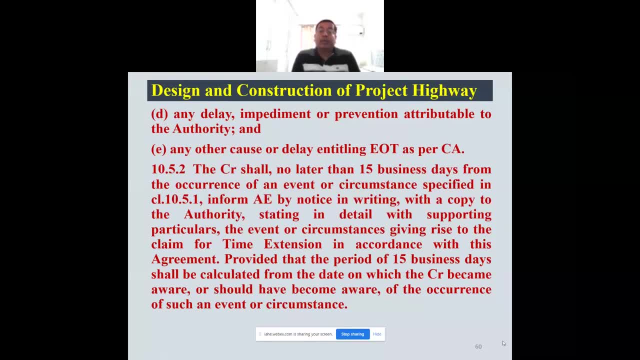 provided that the period of 15 business days disconnects, 15 business days shall be calculated from the date on which the contractor became aware. These 15 business days will be counted from the time contractor became aware, or should have become aware, of the occurrence of such an event or circumstances, not before that. 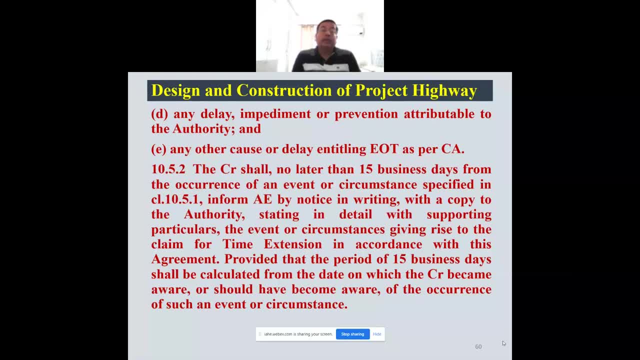 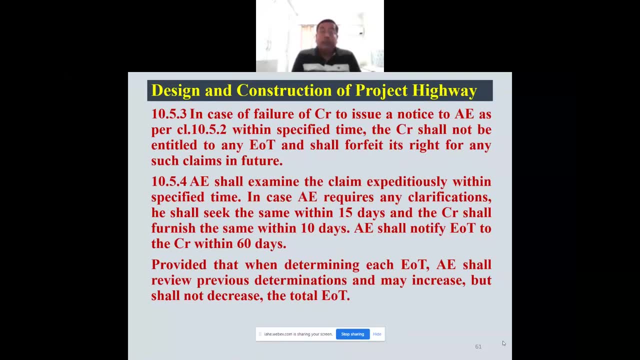 When he becomes aware that this is required, he will seek time extension In case of failure of contractor to issue a notice to the 30th engineer. in case of failure of contractor to issue a notice to the 30th engineer as per clause 10.5.2, within. 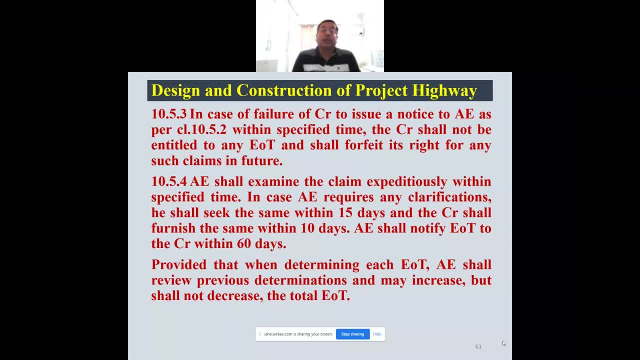 a specified time, the contractor shall not be entitled to an EOT. This is also a very hard clause that if contractor fails within a specified time, he will not be entitled to an EOT and shall forfeit its right for any such claims in future. 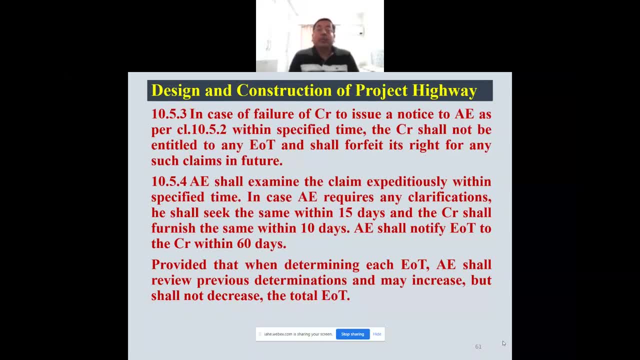 So contractor shall not be entitled to an EOT. The contractor has to be very much prompt and he has to apply for time extension within the time frame, telling which he may lose his opportunity. 10.5.4 A. 30th engineer shall examine the claim expeditiously within a specified time. 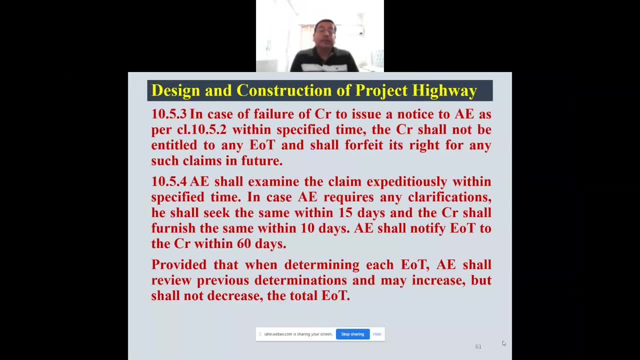 In case a 30th engineer requires any clarifications, he shall seek the same within 15 days and contractor shall furnish the same within 10 days. Here it is defined that a 30th engineer shall examine the claim in a very fast manner, not 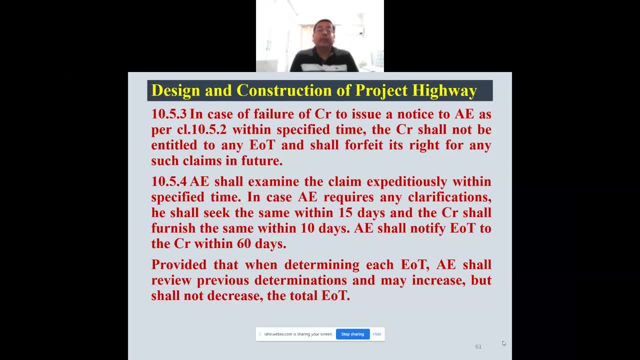 in a very slow manner. In case a requires any clarification, he may seek from the contractor within 15 days and contractor shall furnish the same within 10 days. A shall notify extension of time to the contractor within 60 days. So timelines have been defined in the contract so as to have faster way for time extension. 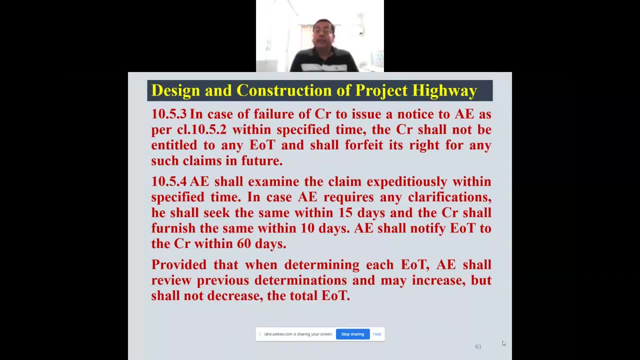 provided that when determining time extension- 10.5.4- A 30th engineer shall examine the claim in a very fast manner, not in a very slow manner. Here it is defined that A 30th engineer shall review the previous determination of each EOT. 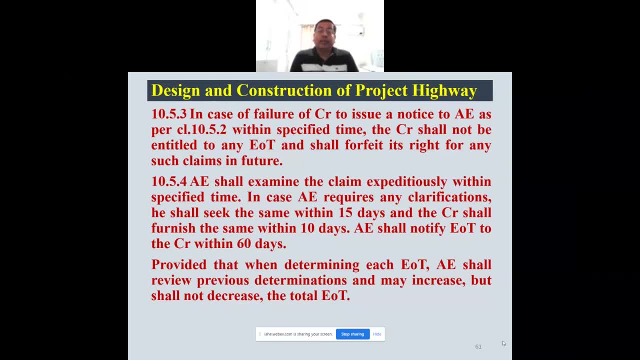 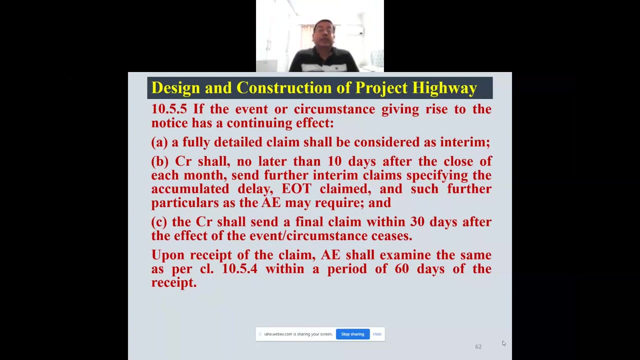 Suppose the 60-day extension of time has already been given and now the contractor is claiming another 90 days, Seeing that the 30th engineer may review and increase the earlier 60 days. clarity on this issue. design and construction of the project highway 10.5.5 if the event or 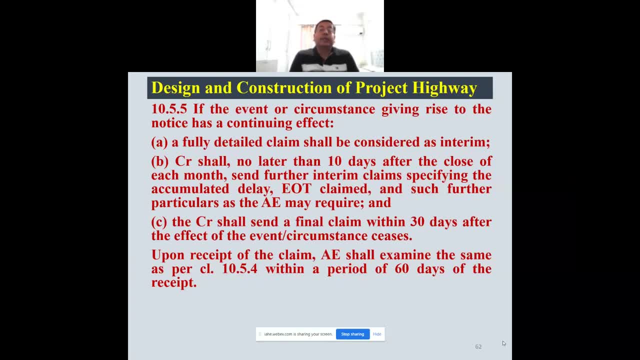 circumstances giving rise to the notice has a continuing effect means the same thing is still continuing. a fully detailed claim shall be considered as. interim contractors shall, no later than 10 days after the close of each month, send further interim claims specifying the accumulated delay, extension of time claimed and such further particulars as the 30 minute may. 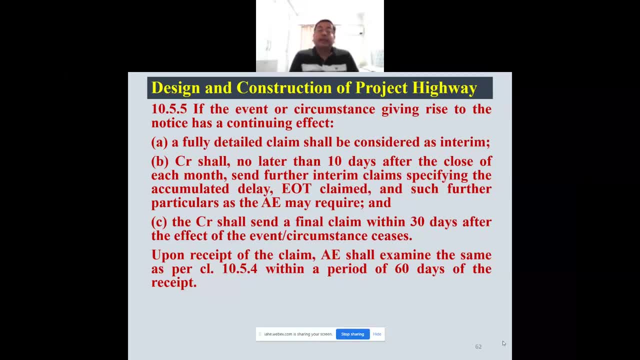 require and the contractor shall send a final claim within 30 days after the effect of the event. circumstances seizes, so he will furnish the final claim within 30 days after which the effect of the circumstances has ceased. suppose it was covid 19 and all the site has been closed and it is still continuing. and after 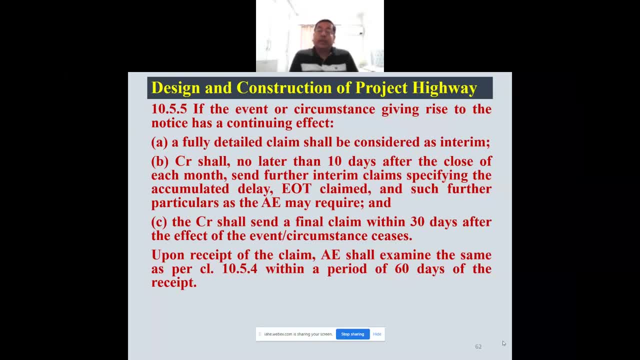 the 45 days this has been closed and now the work has started. then the contractor shall send a final claim within 30 days after the effect of the covid has ceased upon receipt of the claim that the 30 engineers shall examine the same a 13 years. 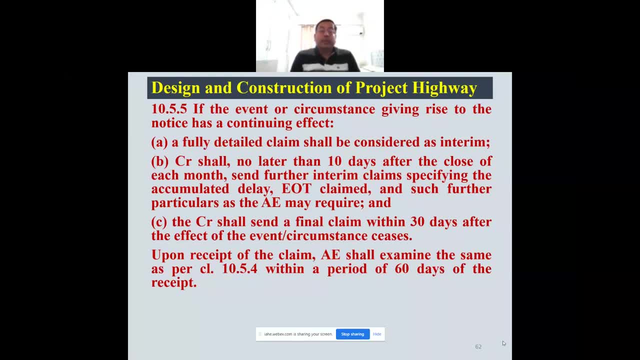 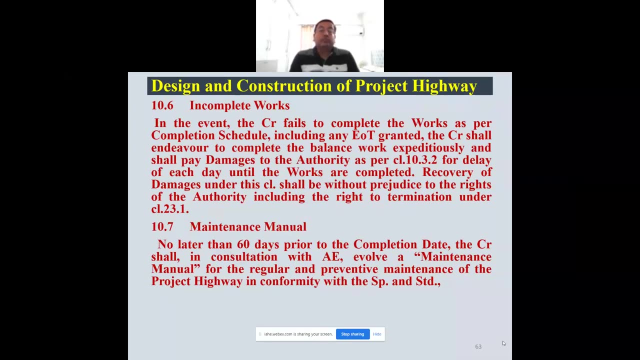 in the eot proposal and the same as per clause 10.5.4: within a period of 60 days of the receipt. within 60 days he has to examine and review and finally he has to give its decision now. incomplete work. in the event, the contractor failed to complete the work. 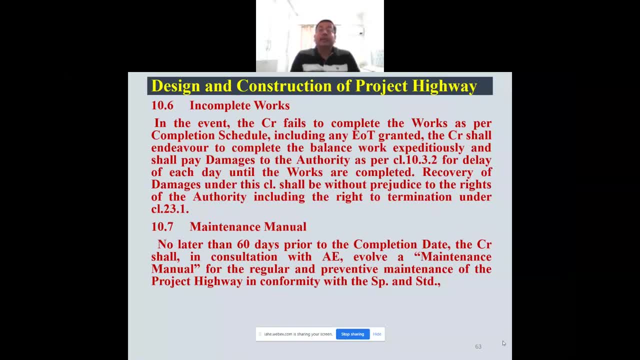 as per completion schedule, including any extension of time granted, the contractor shall endeavor to complete the balance work expeditiously and shall pay damage to the 30 as per clause 10.3.2, for delay of each day until the works are completed. it is already mentioned in 10.3.2 and it is clear that if he fails the milestones or schedule. 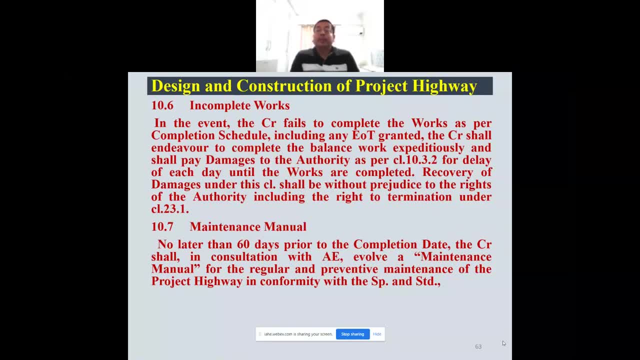 completion date. as procedure, he has to pay compensation damages as per clause 10.3.2. recovery of damages under this clause shall be without prejudice to its right of the authority, including the right of transparency. it means that authority can cannot be satisfied with the damages only. 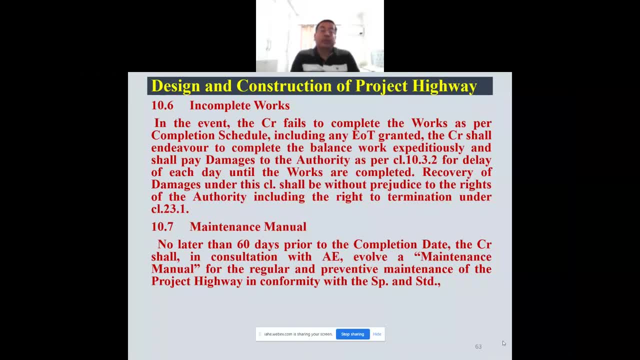 it can terminate the agreement if he fails to complete the work. so incomplete works are to be completed by the contractor expeditiously and in case of failure by the contractor, authority may take very bold decision, very hard decision, to even terminate this agreement. so contractor has to take care of all the things and incomplete works are to be completed. 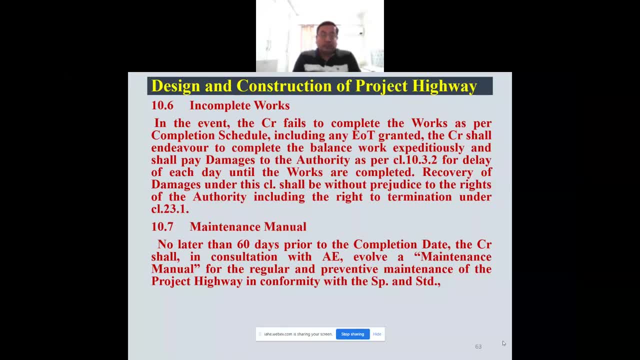 within the defined timelines. maintenance manual. what is maintenance manual? no later than 60 days prior to the completion date. before 60 days of the completion date, the contractor, in consultation with ae, evolve a maintenance manual for the regular and preventing- preventing- regular and preventive maintenance of the project, having conformity with the specification. 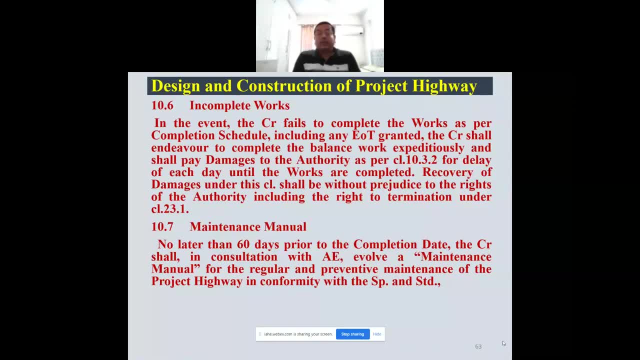 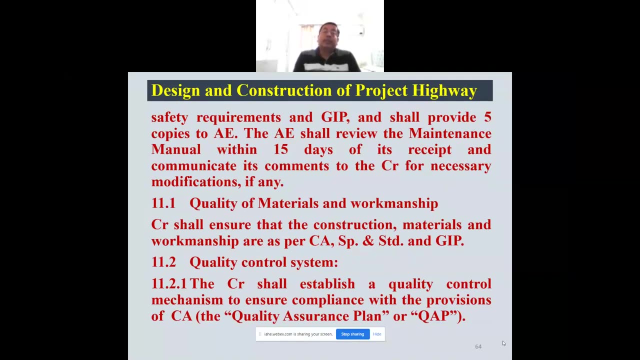 standard. it means the contractor will evolve a maintenance manual 60 days prior to the last date of completion and will submit it to the authority engineer giving details of safety requirement and good as per safety requirements and good industry practice, and shall provide five copy to the authority engineer. 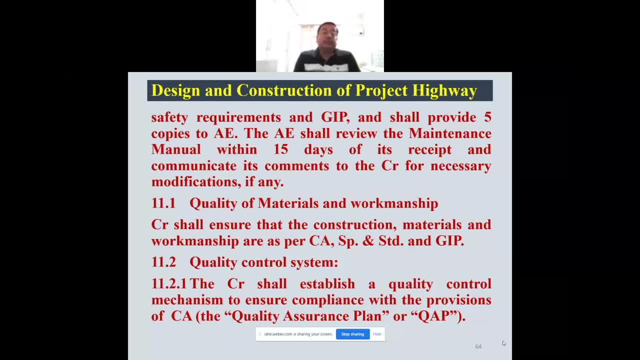 the authority engineer shall review the maintenance manual. the 13 year had to review the maintenance manual within 15 days of its receipt and communicate its coming to the contractor for necessary modification. if any suppose he received he will go through it. what is the maintenance manual? have had it considered all the aspects of maintenance and then he will communicate its. 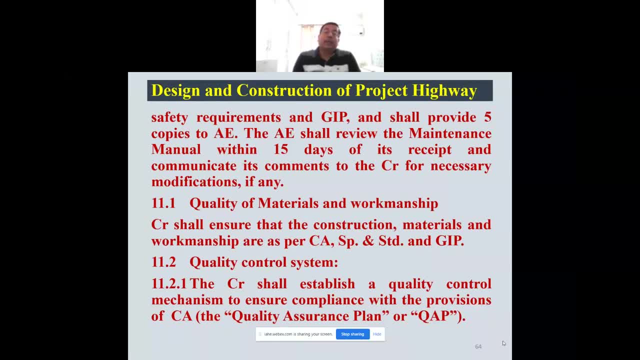 comment to the contractor for necessary modification if required. if it is not required, he will approve it. Quality of material and workmanship: Contractors will ensure that the construction materials and workmanship are, as per contract agreement, specification, standard and good industry practice. See, you want a quality product, so this clause is very much important. that suppose 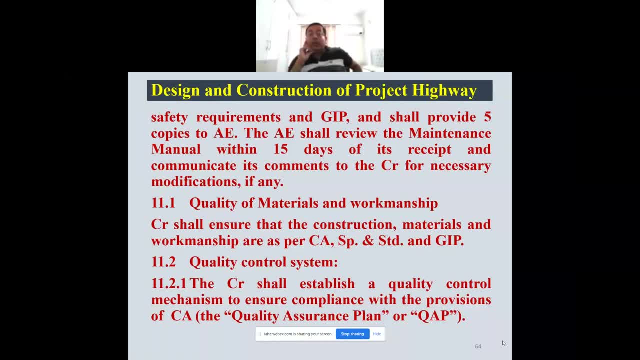 even quality is also given by the contractor, but workmanship will be not there, it is not in line, it is not in line and level. so quality of materials are essential and workmanship is also very much essential. so contractor has to ensure that the construction materials and workmanship. 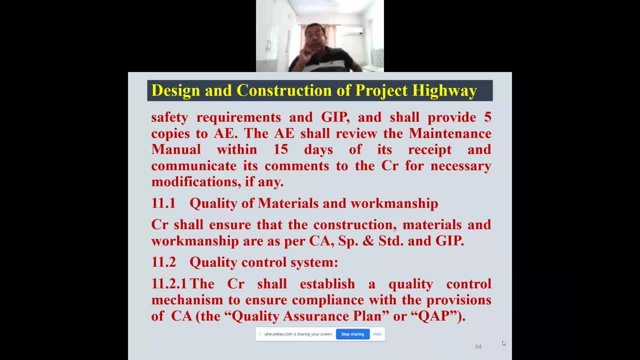 are, as per the provision of the contract agreement, specification and standards and good industry practice. Quality control system: the contractors will establish a quality control working environment. the contractors will establish a quality control operating environment, thatнибудь control mechanism to ensure compliance with the provision of this contract agreement. the quality 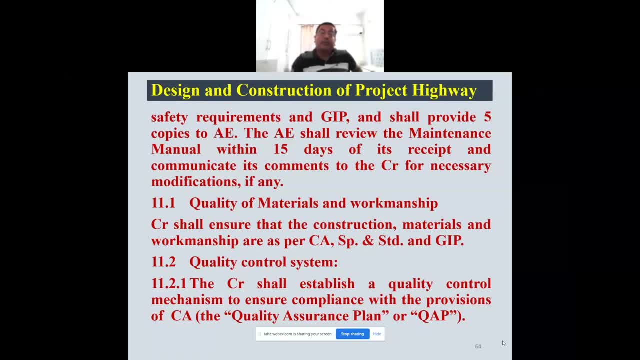 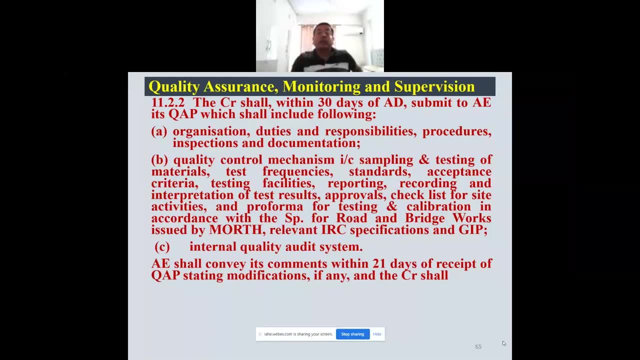 assurance plan, or QAP. What is QAP? The contractors have, within 30 days of appointed date, submit to the 30 days quality assurance plan, which will include following organization: he will give details of its organization, contractors, organization, who is who, and duties and responsibilities of each. 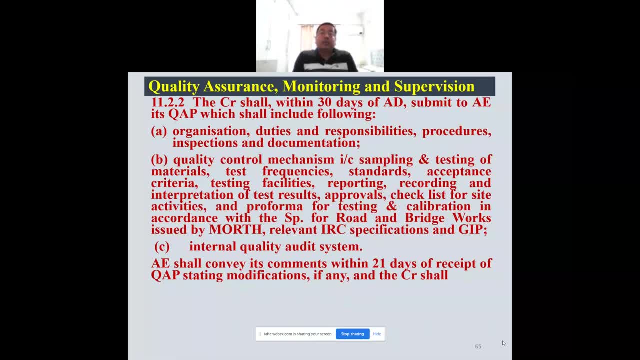 of the person, procedures. what will be the procedures for quality and inspection and documentation, how he will document it. see if you will get it, if you know that he is the quality expert of the contractor. so duties and responsibilities of each of the person should be defined so that 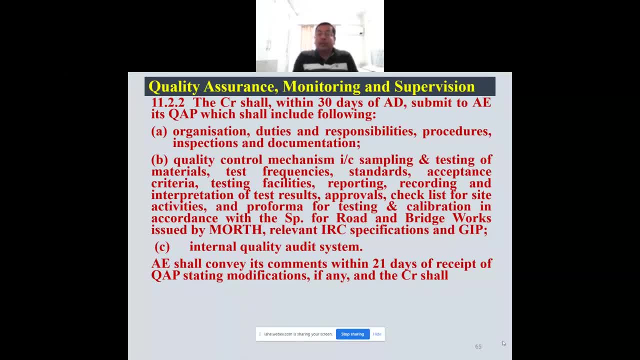 authority, engineer, team leader or authority or thrive representative may know that who is the right person for the quality and who will show you the process. In that case, the quality person of the contractor will show you all the things. so this is why organization, duties and responsibilities, procedure, inspection and documentation has to be furnished. 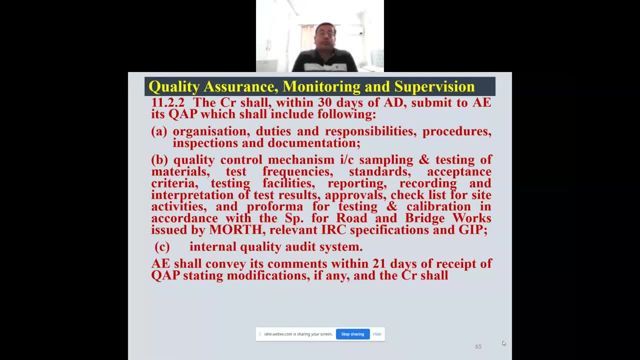 by the contractor to the authority engineer Quality control mechanism including sampling and testing of material he has also to furnish. contractor has to furnish quality control mechanism that is including sampling and testing. how sampling and testing of material has to be done. How testing will be done. 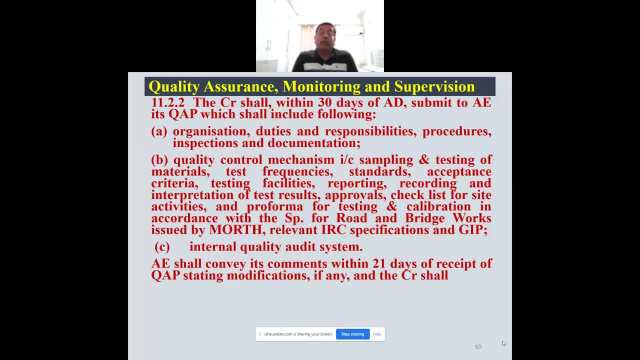 Testing of material will contest frequency. how much test for each quantum of work will be undertaken? a standards: what are the standards? what are the criteria of acceptance, if acceptance criteria must also be mentioned? if it is less than this, this will not be accepted. If it is more than this, then it will be accepted. testing facilities. 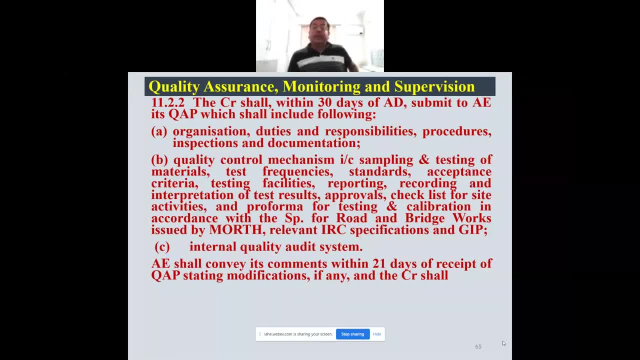 What are the facilities provided for testing, reporting, how it will be reported and recording- all the test results will be recorded- and interpretation of test results. and what is the interpretation of test result? test result has come, but what it interprets that it is good or not good. 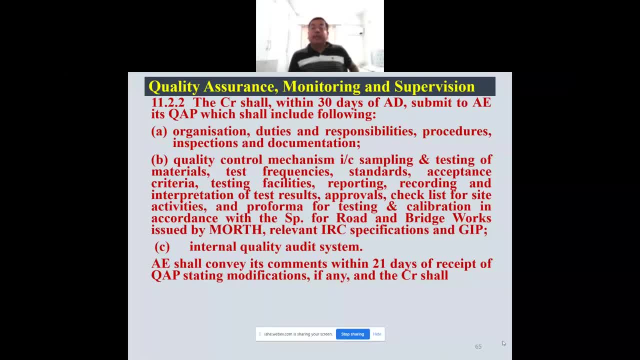 these: interpretation and approvals, checklist of site activity and performer for testing and calibration in accordance with the specification for road and bridge works issued by morth. you have already linked in a schedule d and xl1 of schedule d. still, you are mentioning here that this specification for road and bridge works will have to be followed for the quality. 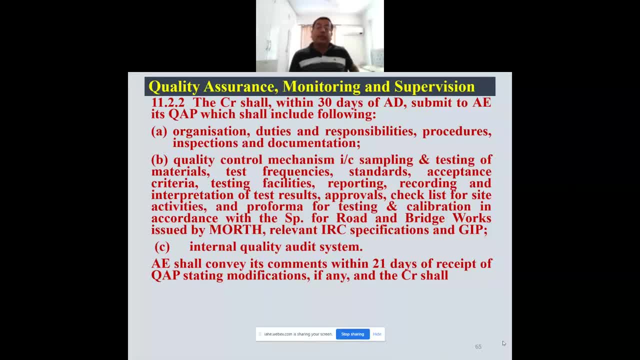 assurance. relevant irc specification and good industry practice is also included. now, internal quality audit system. this has also to be provided by the contractor. a cell convey its comments within 21 days of receipt of quality assurance plan. a stating modification, if any, and the contractor now a 30 engineer will go through the quality assurance plan. 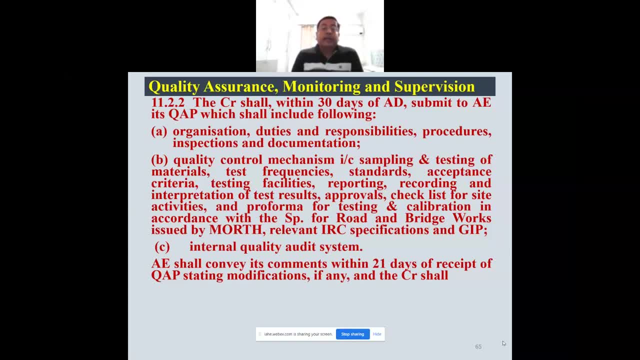 and furnished by the contractor and shall convey its comments within 21 days. within 21 days of receipt of the uap a stating modification that some modification is required, he may ask, he may not ask. if it is not asking it means it is fine light and the contractor cell incorporate those in the 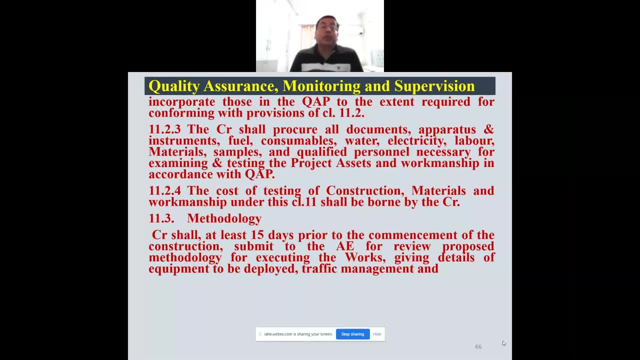 quality assurance plan to the extent required for confirming with the provision of clause ln point. so whatever has been furnished by the contractor will be reviewed by the authority engineer and after awesome told that some modification is required, he will modify and again furnished to the authority engineer and if a certain engineer satisfied then it will be finalized then uap quality. 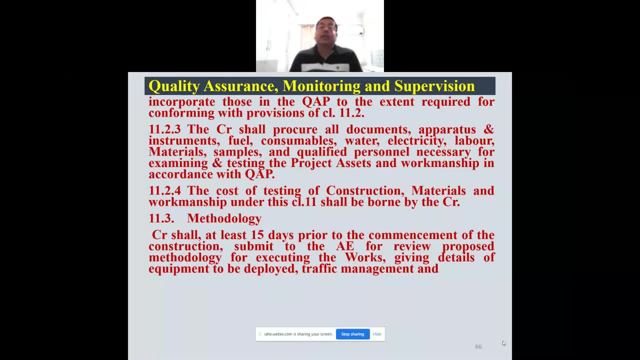 assurance plan will be finalized and accordingly, the quality will be ensured by the contractor, alper uab, which has been a get by the a 13 11.2.3.. The contractor shall procure all documents, apparatus and instruments, fuels, consumables, water, electricity, labor materials, samples and qualified personnel necessary for examining and testing the project assets and workmanship in accordance with quality assurance plan. 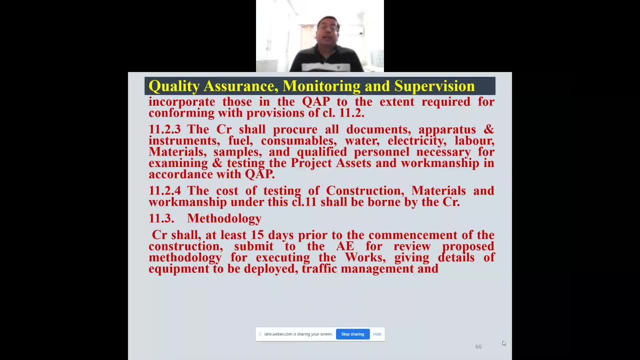 It means contractor has to procure all documents, all type of apparatus and instruments, fuels, consumables like benzene, water, electricity, labor materials, samples and qualified personnel. He must have quality lab and qualified personnel who can test and who can certify, necessary for examining and testing the project assets and workmanship in accordance with the quality assurance plan. 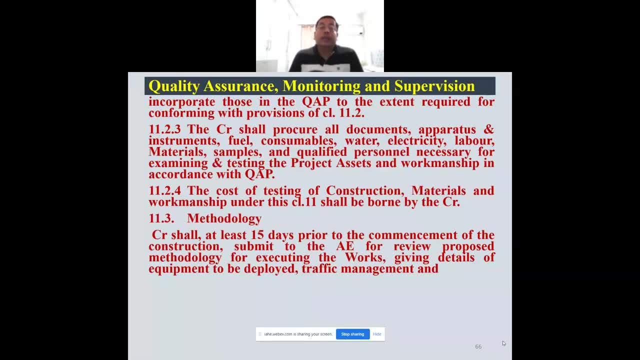 So quality assurance plan is very important. It requires materials, consumables and qualified personnel, and all these things are to be provided by the contractor. as per the QAP, The cost of testing of construction materials and workmanship under this clause 11 shall be borne by the contractor. 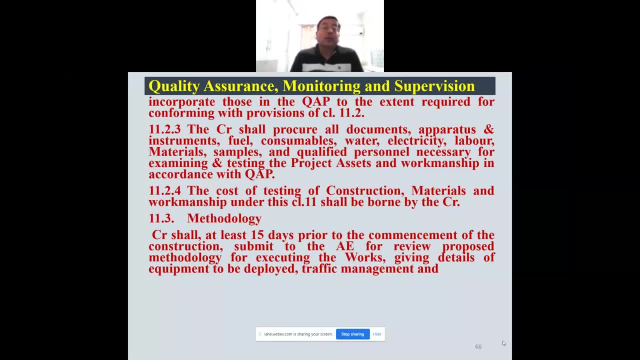 Why it is written. It means the cost is not to be borne by the authority. So it is clearly mentioned that The cost of testing of construction materials and workmanship shall be borne by the contractor. Now coming to methodology 11.3.. 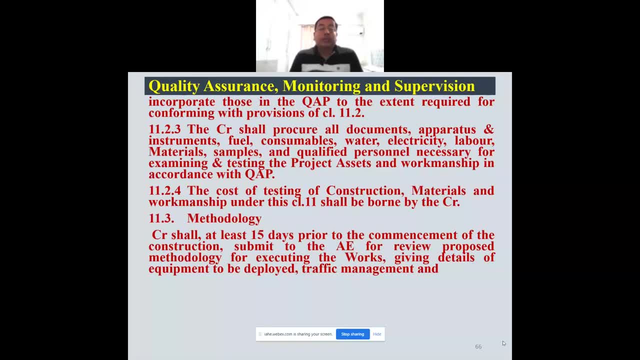 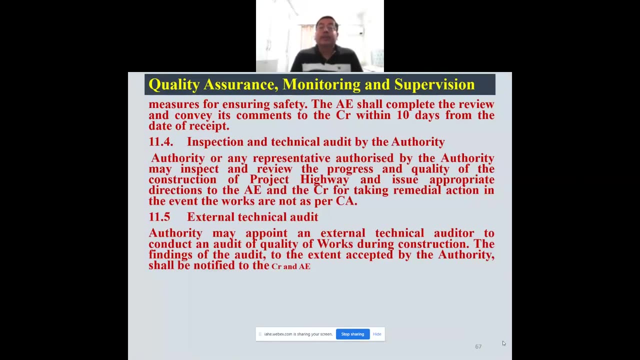 Contractor shall, at least 15 days prior to the commencement of the construction, submit to the authority engineer for review proposed methodology for exuding the works, giving details of equipment to be deployed, traffic management and measures for ensuring safety. The authority engineer shall complete the review and. 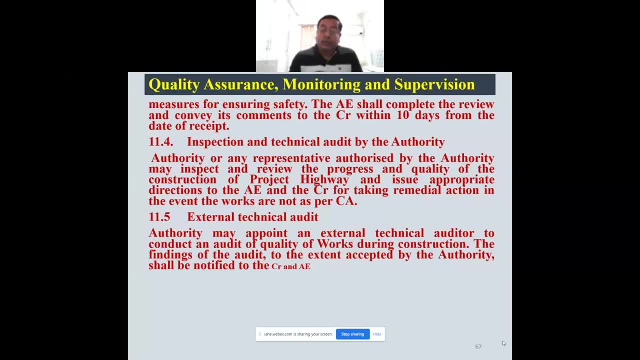 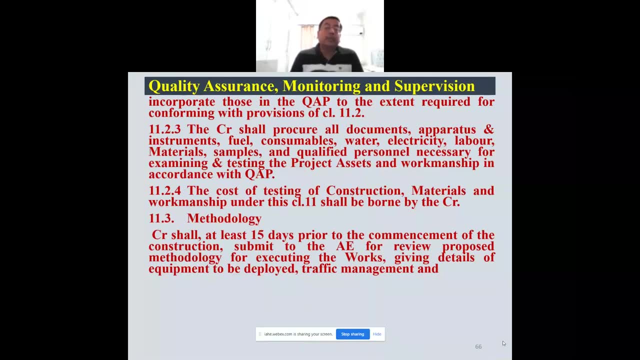 Convey its comment to the contractor within 10 days from the date of receipt. It means methodology, how it will be done. So, for methodology, the contractor shall, at least 15 days prior to the commencement of the construction, submit to the authority engineer for review proposed methodology for exuding the work, giving details of equipment, which type of equipment are being deployed, what are the traffic management plan and measures for ensuring safety. 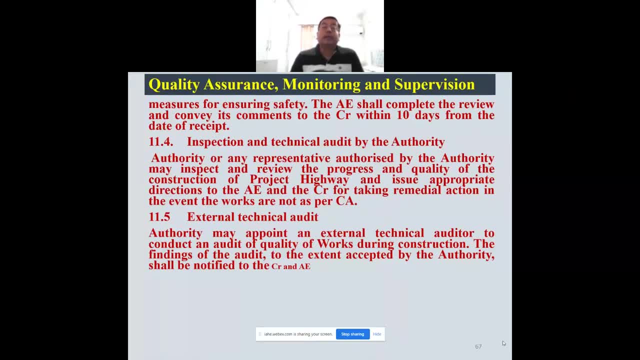 And the authority engineer shall complete the review and Convey its comment to the contractor within 10 days from the date of receipt. The authority engineer shall complete the review and Convey its comment to the contractor within 10 days from the date of receipt. 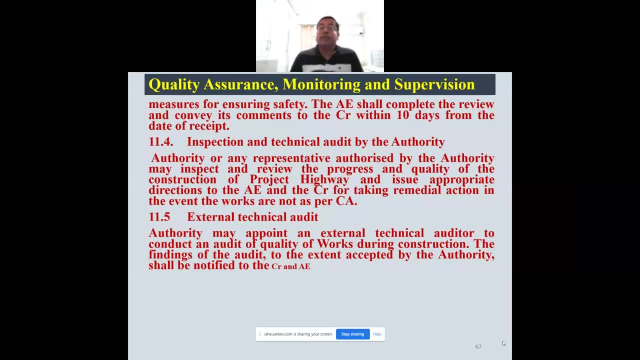 So authority engineer's time limit has also been explained here. defined here It is 10 days from the date of receipt. So this will be finalized within 10 days after receipt of the contractor Inspection and technical audit by the authority. Authority or any representative authorized by the authority may inspect and review the progress. 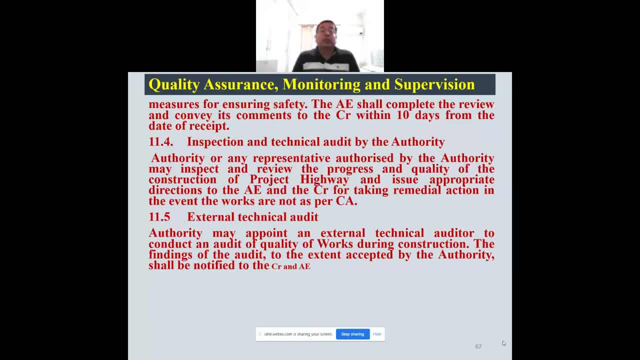 And quality of the construction of the project highway and issue appropriate action to the authority engineer and the contractor for taking remedial action in the event of works are not as per CA See here. this is a very important clause. We are depending upon the authority engineer and he is getting the work done from the contractor. but here authority can also inspect. 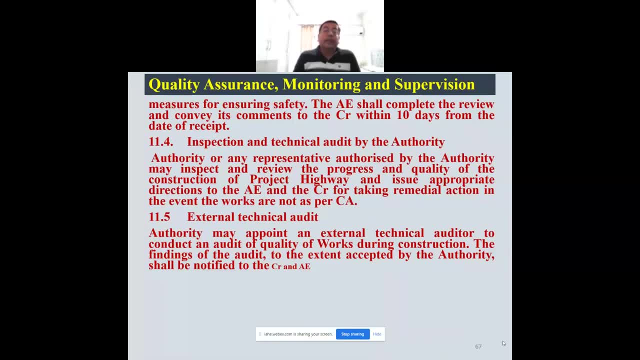 It means authorized representative of the authority may inspect and review the progress and quality of the construction of project highway and issue appropriate action to the authority, engineer and the contractor for taking remedial action Suppose something is not as per the specification standard and project director. 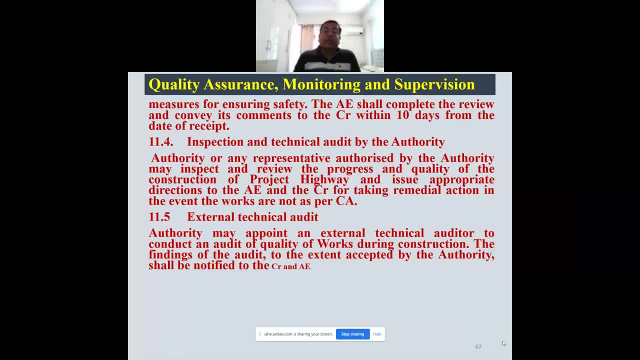 pointed out that this is not as per to the authority engineer, Then authority engineer will have to take immediate remedial action so that the work are as per the provision of the contract agreement, That is, as per the specification standard and as per scope of the project. 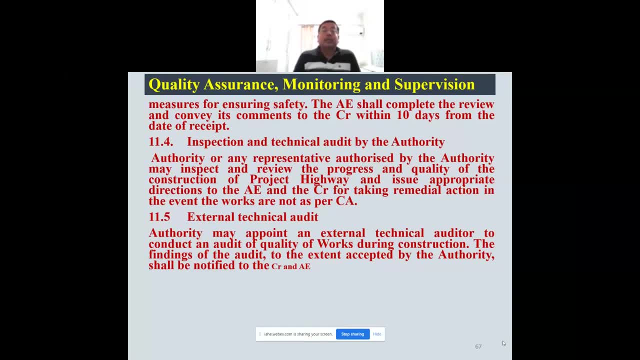 and as per quality it has been constructed. So this is a power to the authority. If this clause is not here, then one can ask that where is the role of authority? How can authority inspect? So it is written Now: authority or authority representative can review the progress. 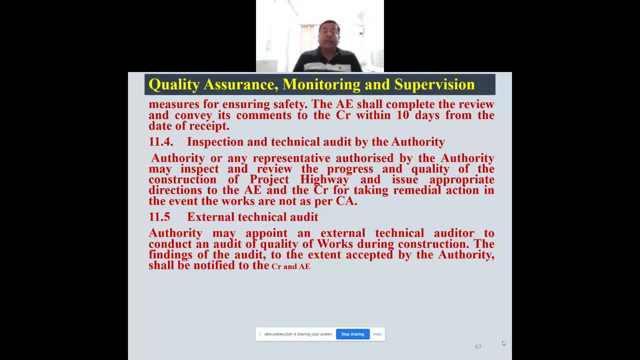 and quality and may ask authority, engineer and contractor for taking remedial action immediately. Now external techniques: Technical audit 11.5.. This is also mentioned. Authority may appoint an external technical auditor to conduct an audit of quality of works during construction. The finding of 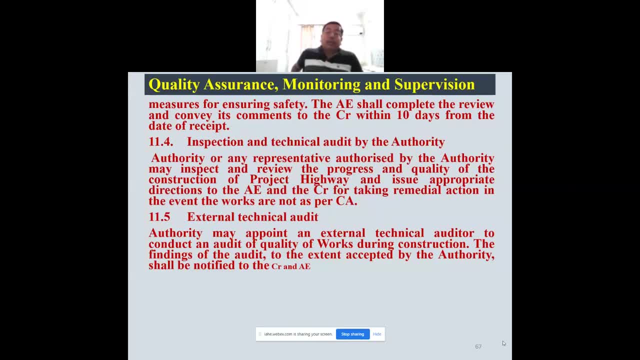 the audit to the extent accepted by the authority shall be notified to the contractor and the authority engineer. This has been mentioned. Suppose sometimes court also interferes or even court is not interfering. Suppose authority want to engage some technical audit of audit by some independent like any engineering college or a different consultant or CRI. 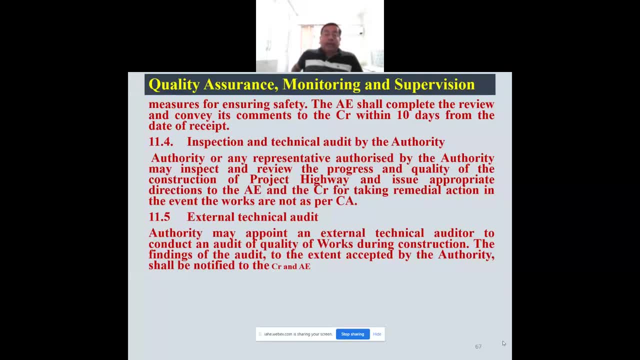 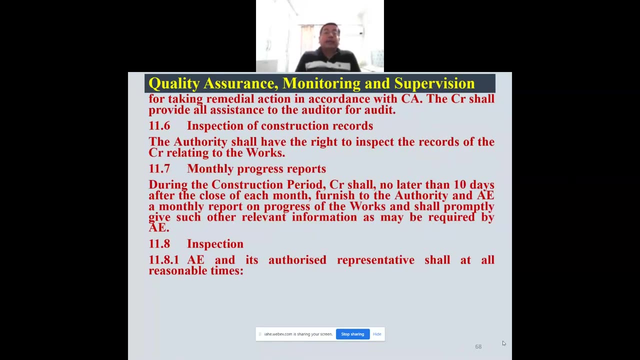 Then whatever findings has been given by the audit and which has been accepted by the authority shall be notified to the contractor and the authority engineer and they will have to incorporate it in the work for taking remedial action. according to CA, the contractor should provide all assistance to the auditor. 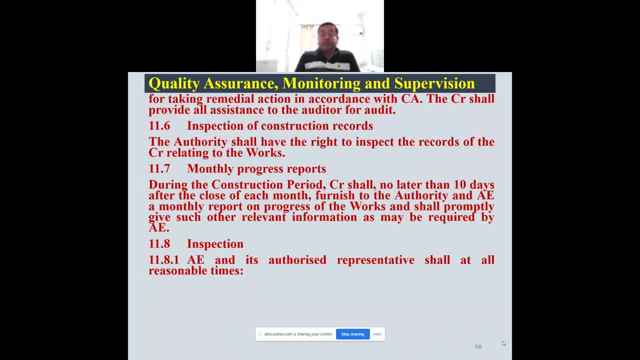 has to provide all assistance to the auditor. suppose your auditor has gone there and the contractor will not provide any assistance, so it is written, it is binding for the contractor as per this agreement that he will have to provide all assistance to the auditor for the audit. so this is also defined. 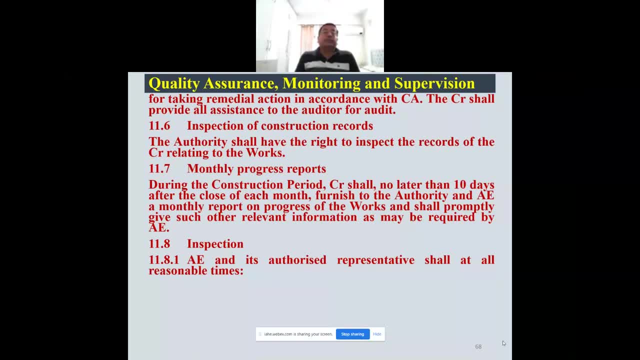 that in case of external audit, the contractor has to cooperate. inspection of construction records: the 30 shall have the right to inspect the records of the contract related to the work. this is also an over riding power that authority, at any time, may send its representative, and who will have the? 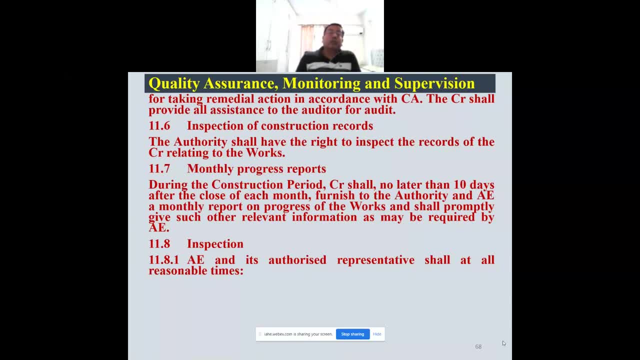 right to inspect the records of the contractor relating to the works. suppose i want to see the WM work in 135th килometre. then they are having documented each, each of the things kilometer wise. he will show you the all the records in the contract or a contractor's record. so that's one of the 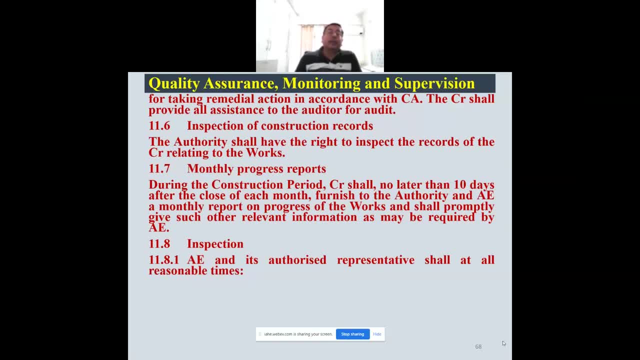 results and you can see the site and also the records and then you can tell it is right or wrong. so this is a power inspection of construction records. construction records had to be shown to the authority by the contractor. now, monthly progress report: 11.7. during the construction period, contractors sell. 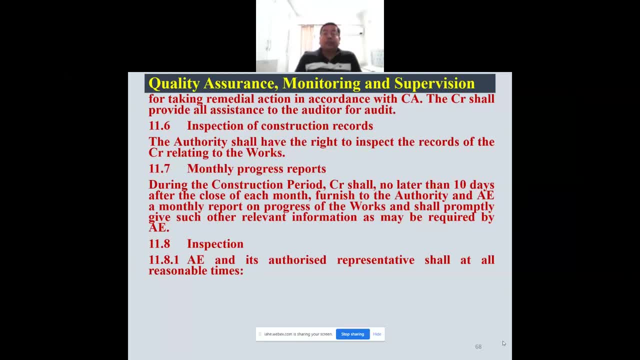 more later than 10 days after the close of each month, furnished to the authority and authority my monthly report on the progress of the works and self promptly gives such other relevant in form so and may be required by a 30 million during costs, and my contract is a little ten days after the. 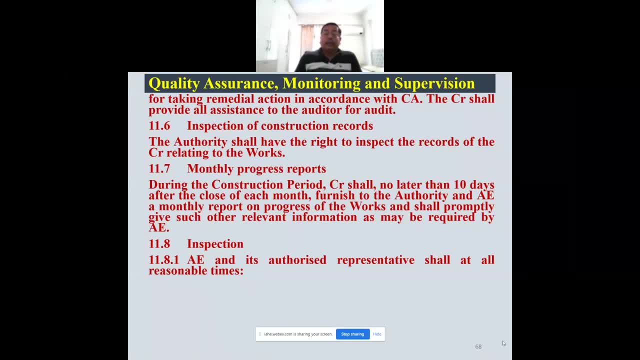 close of each month when whenever a calendar month he has ended within ten days he will furnish to the 30 and a cutterting your monthly report on progress of the gram. he will submit monthly progress report and slightly gives such press on relevant information and may be required by a 13 year inspection. a 13 year and. 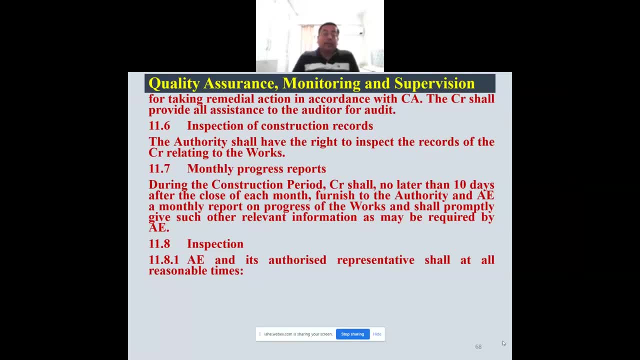 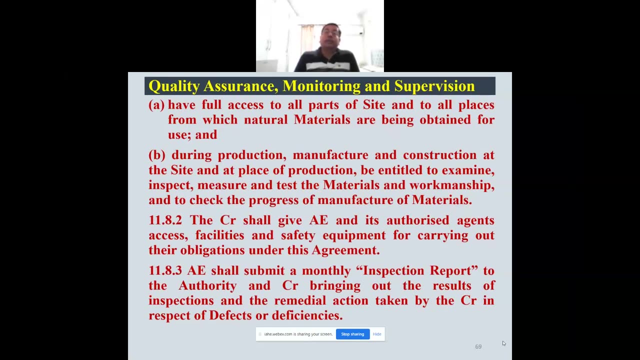 it's authorized representative sell at all reasonable time of inspection. what is the terms under the inspection? what is the provision under inspection? a 13 year and it's authorized representative sell at all reasonable times. have full access to all parts of site and to all places from which natural materials are. 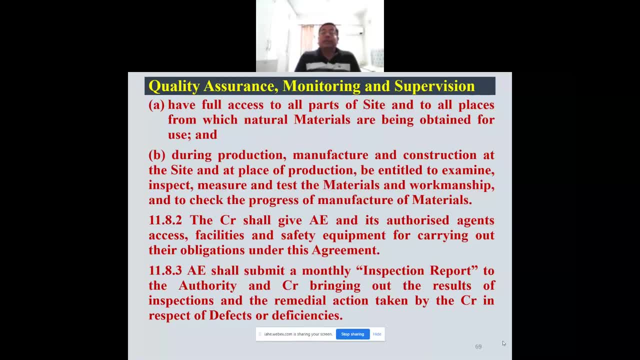 being obtained for you, not only side, he can be it each part of the site and he can also be it a quality side from where is procuring sand or aggregates or anything. so the 13 year or a 30 have full access to all parts of site and all. 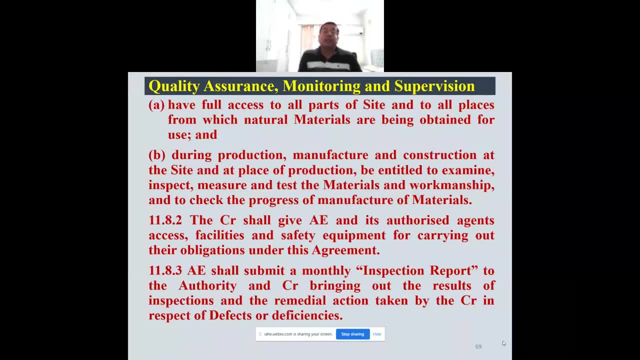 places for which natural materials are being obtained for you and during production, manufacturing, construction and de-semination of the material, and during production, manufacturing, construction and the site and at place of production be entitled to examine, inspect, measure and test the materials and workmanship and to check the progress of manufacture of materials. this has been mentioned. 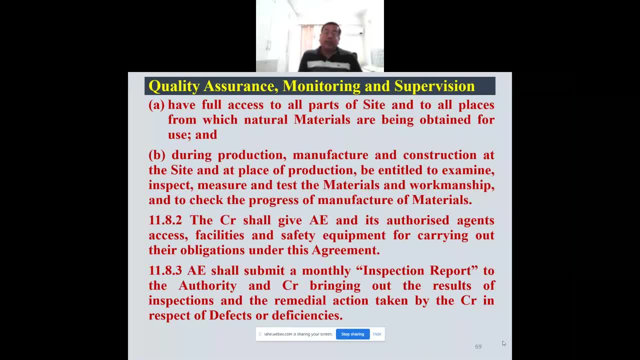 so to authorize authority and authority engineer to test material at site, at the quality site, at the source, and he can tell that this is not a right material and you, you may not use it. in that case they will have to go to the another quality, another place from. 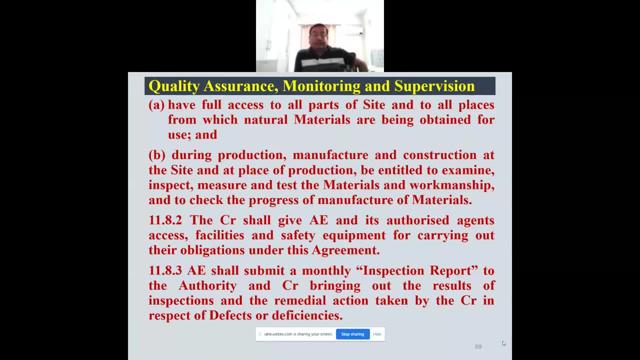 where they will procure the material. so this is written now: 11.8.2. the contractors shall give a 30 engineer and its authorized agents access facilities and safety equipment for carrying out their obligations and disagreement. the contractors shall give a 30 units outside agents. 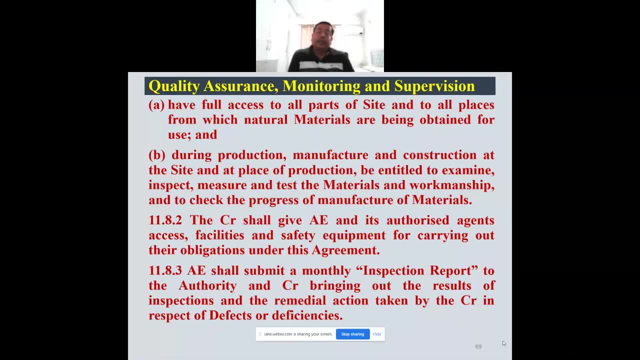 access facilities and safety equipment. safety equipment like helmet, other things, uh- for carrying out their obligations under disagreement. this is also written so so that a 30 engineering or size agent must be safe and they may be given a safety equipment for carrying out their obligations. a 13-year self-submitted monthly inspection report to the 30. now a 30. 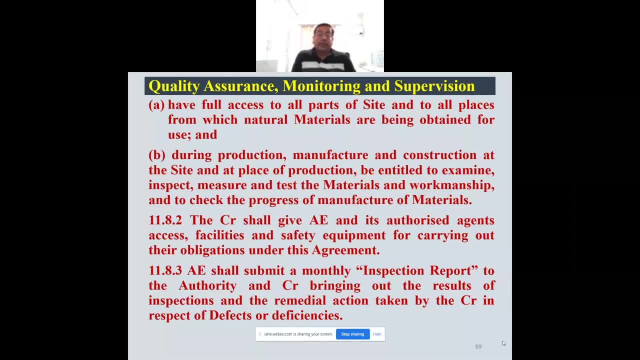 you have given enormous power to a 30 engineer, but a 30 engineer had to report to you, so this is written 11.8.3 is mentioned that a 30 engineer shall submit a monthly inspection report to the authority and the contractor bringing out the results of inspections. 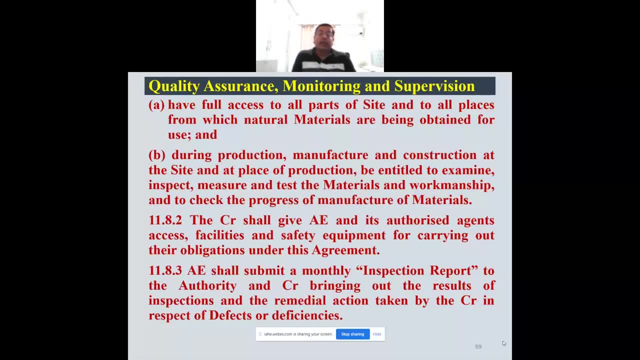 and the remedial actions taken by the contractor in respect of defects or deficiencies. so it is inspection report which has to be furnished by a 13 year to a 30 and contractor bringing out the result of inspection and the remedial action taken by the- suppose a 30- engineer. 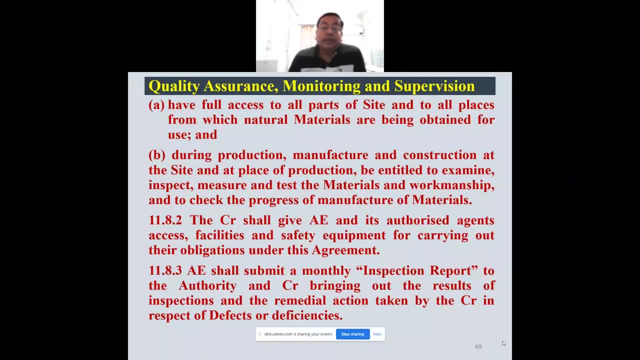 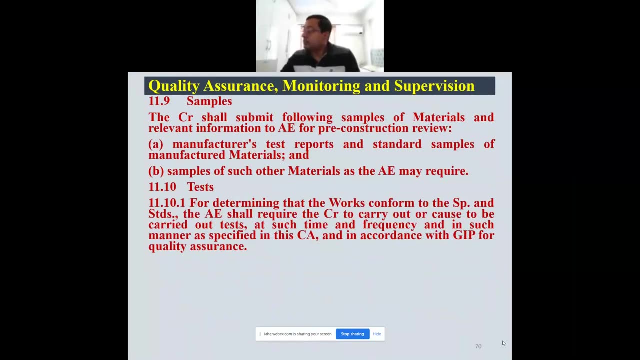 pointed out some mistakes, some some defects, then what remedial action has been taken by the contractor in respect of defects or deficiencies? must also be brought out samples. the contractor shall submit following samples of materials and relevant information to the a 30 engineer for pre-construction review: 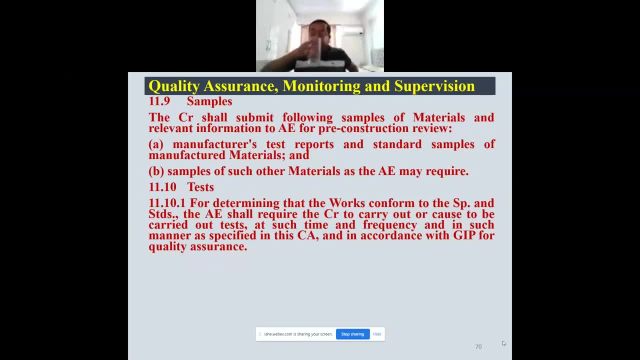 uh, first manufacturer's test reports and a standard samples of manufactured material. what contractor will submit samples of materials and relevant information to the a for pre-construction review: manufacturer's test report and a standard samples of manufactured materials, samples of such other material as the 30 engineer may require? suppose he furnished? 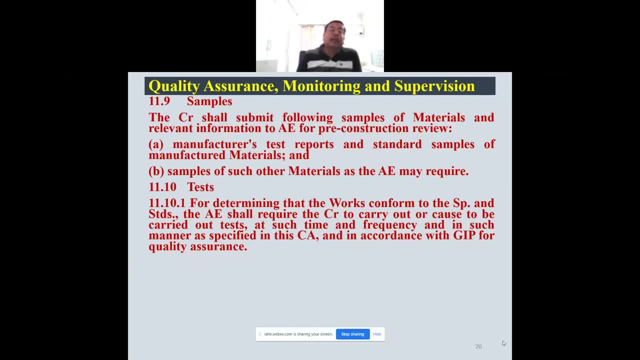 a number of things, but a 30 year may require some more, and then he will have to provide the samples of such other materials as the 13 year may require. now tests 11.10.1 for determining the that the work is conformed to the specifications and the standards the 30 engineer shall require. 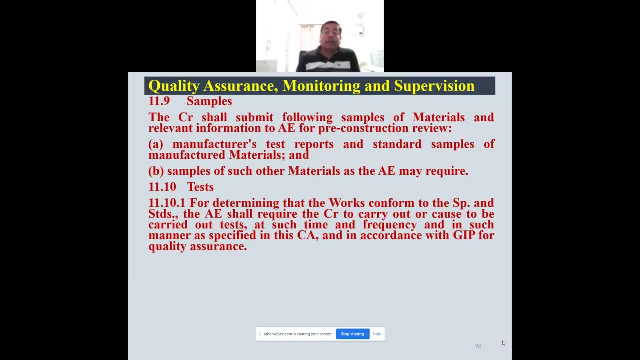 the contractor to carry out or call to be carried out test at such times and frequency and such manner as specified in this agreement and in accordance with the good industry practice for quality. these are 2 steps in which, accordingly, they shall submit a good commercial diagnostics s for a 30 years to carry out or asked to be carried out tests at such times and frequency and in such manner as specified in this agreement and in the new standards. software might be converted to safety. 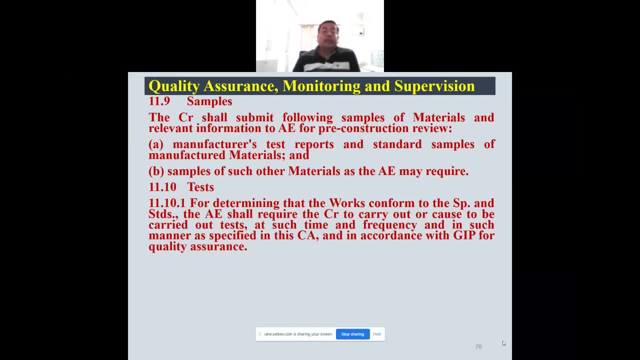 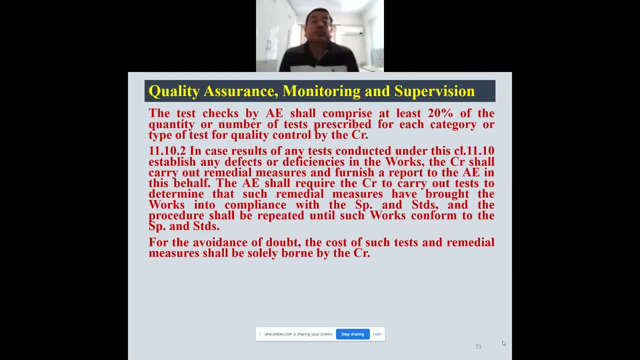 we have accepted 30 years test defined for the test that the contractor has to carry out, all the tests and the frequency as per the agreement and as per this good industry practice for quality assurance. The test checks by the authority engineer. the test checks by the authority engineer. 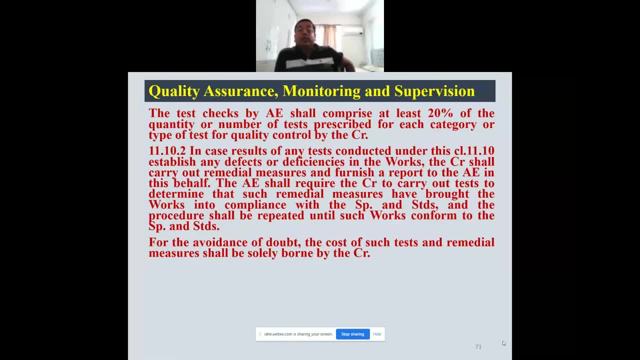 comprise at least 20% of the quantity or number of tests described for each category of type of each category or type of test for quality control by the contractor. It means that suppose 1000 cubic meter of work has been done for M30 concrete, then 20%. 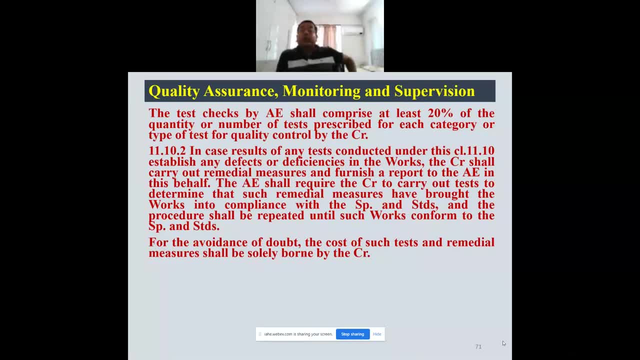 of that, it means 200 cubic meter of that M30 concrete had to be changed. Similarly, out of 100, he has to check at least 20% of each category of type of test for quality control by the contractor, his team leader, his RE, his other person will. 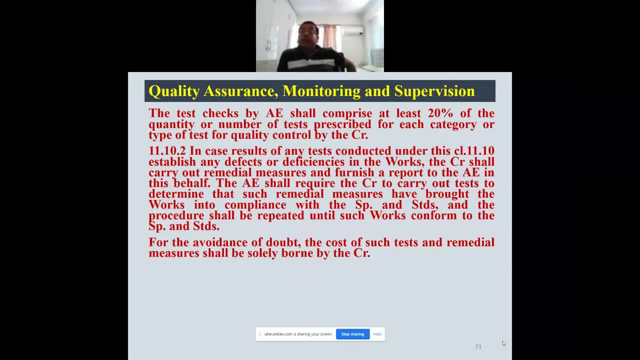 also test, but authority engineer shall test at least 20% of the quantity or number of tests prescribed for each category or type of test for quality control by the contractor. This is the definition of quality control by the contractor. This is the definition of quality control. 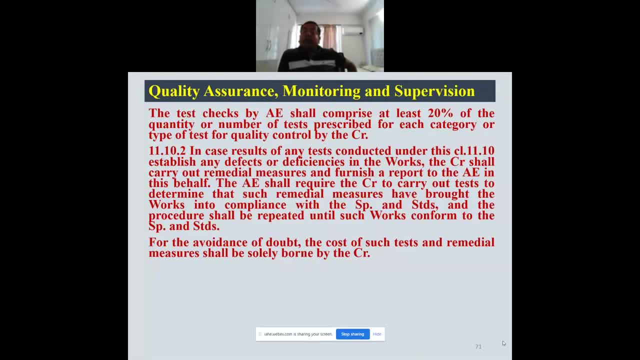 The quality control by the contractor has to be defined because it has to be followed, otherwise authority engineer will not visit and not in case of item rate contracts. it was also defined that at that time there was no consultant, no authority engineer. So PWD personnel like SDO Assistant Engineer and Equity Engineer were defined that they 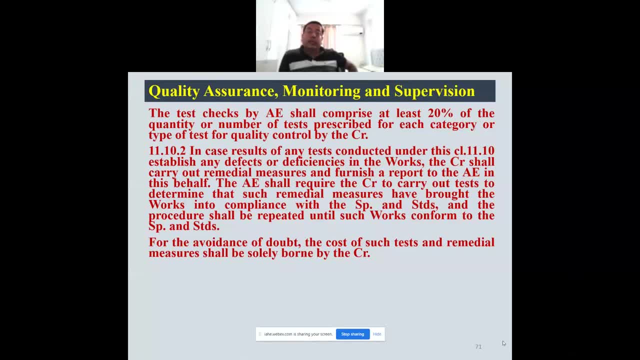 will check 20%, 30%, 50% of which item. Similarly, authority engineer has also been defined that at the time there was no consultant. no authority engineer has also been given a duty that he will test at least 20% of the quantity or number of. 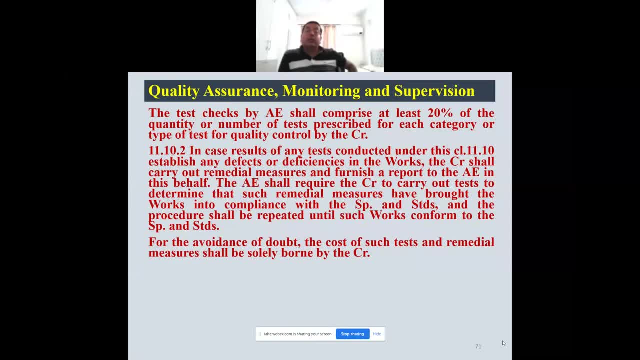 tests prescribed for each category or type of test for quality control by the contractor, so as to ensure quality control at site Now. 11.10.2.. In case results of any tests conducted under this clause 11.10 establish any defects or. 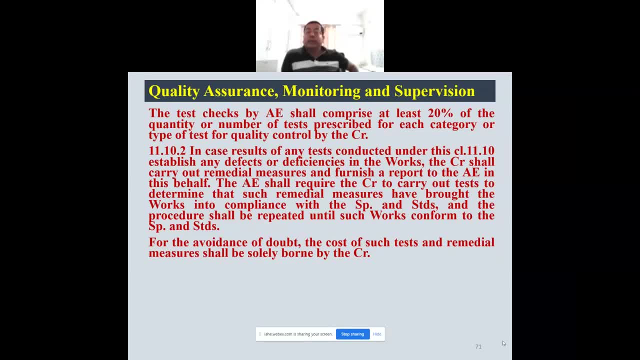 deficiency in the work. Suppose the test was done and some defect or deficiency has been observed, Then the contractor shall carry out remedial measures and furnish a report to the authority engineer in this BR. Then authority engineers shall require the contractor to carry out tests to determine. 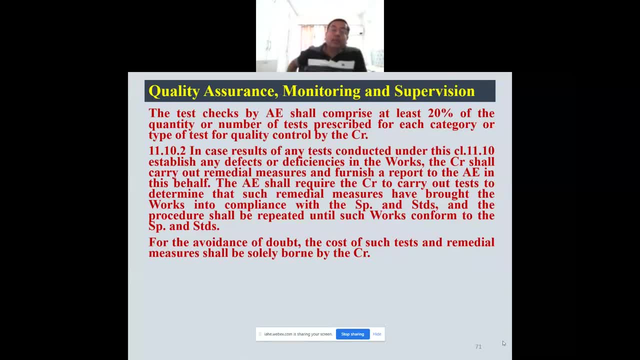 that such remedial measures have brought out the work into compliance with the specification and standard, and the procedures shall be repeated until such work conforms to the specification and standard. The work-wise substandard authority engineer asked to take remedial measures. contractor took remedial measures and furnished a report to the authority engineer. 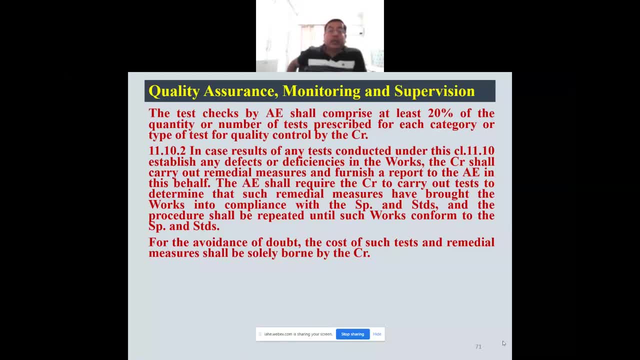 Now authority engineer will ask contractor to carry out tests. Why tests? So as to determine that such remedial measures have brought out the work into compliance with the specification and standard, and the procedures shall be repeated again and again until such work conforms to the specification and standard. 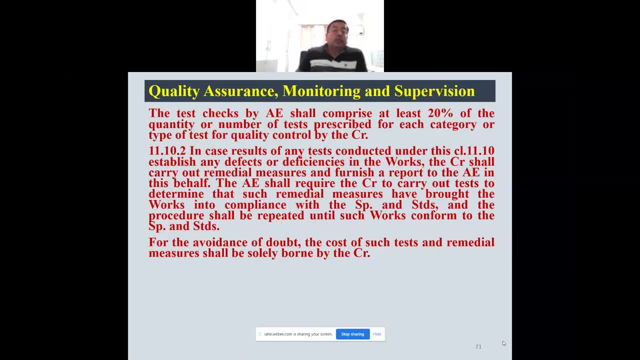 So it is very defined. So contractor, in case of deficiency or remedial measure, will have to retest it till it conforms to the specification and standard. For the avoidance of doubt, the cost of such tests and remedial measures shall be solely. 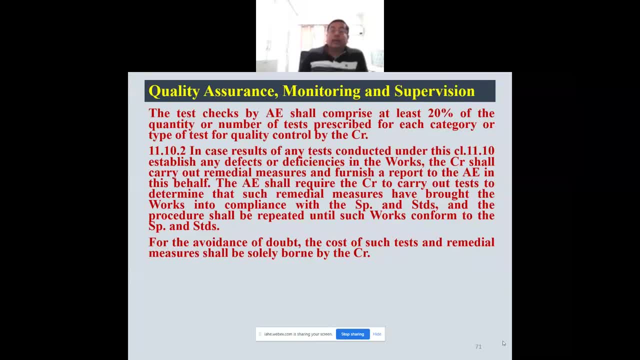 borne by the contractor. This is also written, Otherwise he will ask that I will not pay. Why I will pay for again and again, Why I will pay for again and again. So this is mentioned here for avoiding any dispute in future. 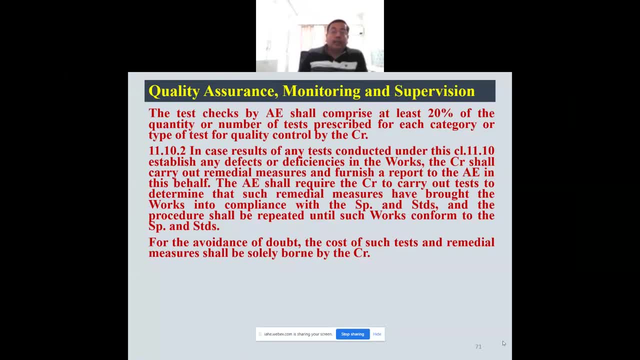 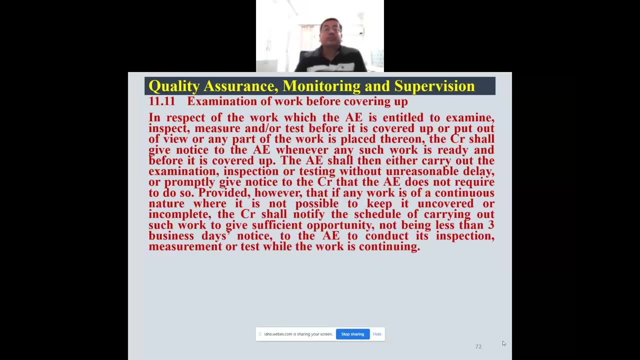 For the avoidance of doubt, the cost of such tests and remedial measures shall be solely borne by the contractor. Now, examination of works before covering up. Suppose your work is going on, GSB is going on and it has to be covered up. 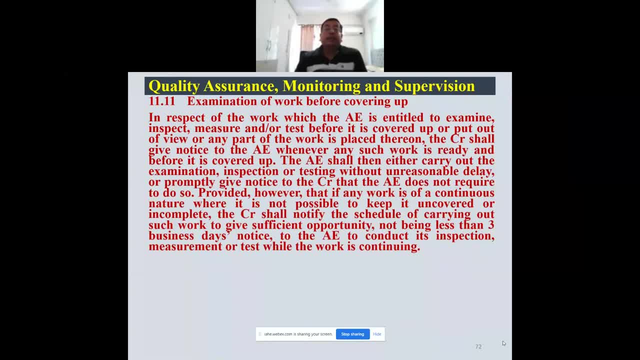 Now WA will be taken up In that case. in respect of work which the AE is entitled to examine, inspect, measure and or test before it is covered up or put out of view, or any part of the work is placed thereon, the contractor shall give notice to the authority engineer whenever any such 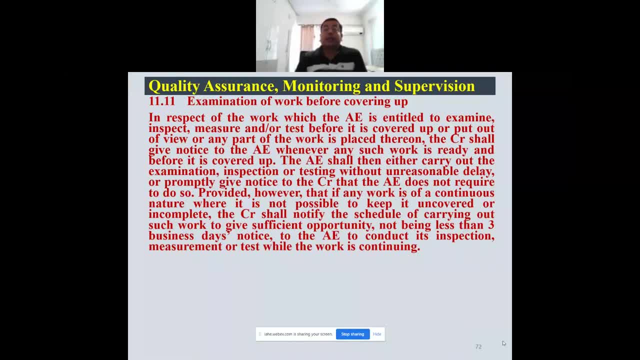 work is ready and before it is covered up, Then contractor has given a notice to the authority engineer that I will cover it up within 3 days or 5 days and authority engineer has to inspect that it is right. it is as per the quality, as per specification and standard. 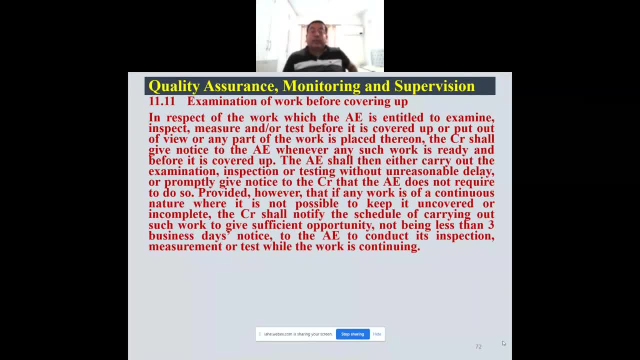 The authority engineer shall then either carry out the examination, inspection or testing without unreliable delay or promptly give notice to the contractor that the AE does not require to do so. Suppose authority engineer knows that the work is all right, there is no need to check. 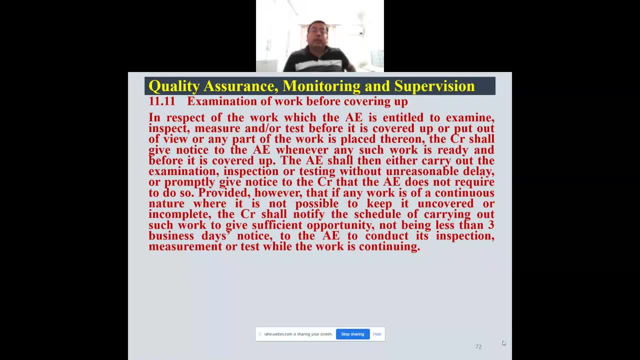 it, then he may write that: okay, go ahead, otherwise he will test, he will be satisfied and only then he will allow. Provided, however, that if any of the work is of a continuous nature where it is not possible to keep it uncovered or incomplete, the contractor shall notify the schedule of 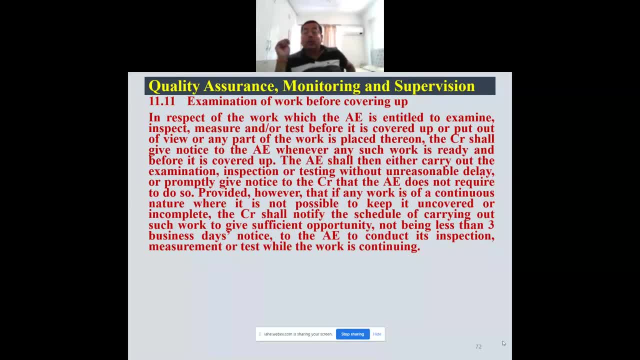 carrying out such work to give sufficient opportunity, not being less than 3 business days notice, to the AE to conduct its inspection, measurement or test while the work is continuing And authority engineer will have to visit the site and conduct its inspection, measurement or test within 3 days. 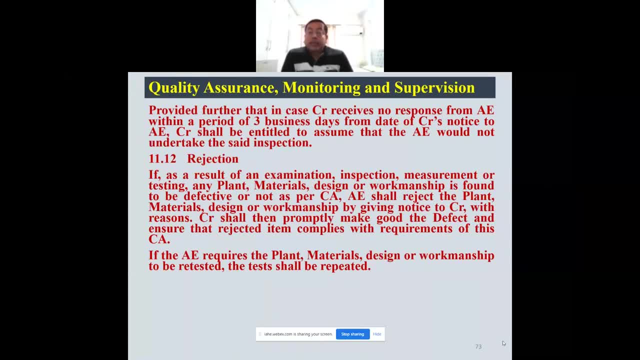 Provided further that in case the contractor receives no response from the authority engineer- suppose after writing by the contractor- and he is not getting any response from the authority engineer within a period of 3 business days from the date of contractor's notice to the authority, contractor shall be entitled to assume. contractor may assume that the AE. 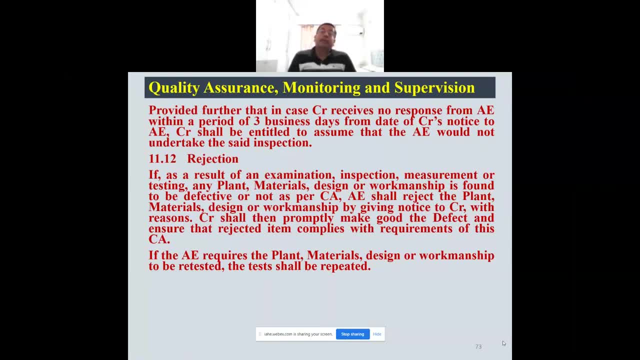 would not undertake the state inspection. After 3 business days He makes a statement He may cover up, cover up the work, assuming that authority engineer would not undertake the state inspection. But 3 business days must be given by the contractor to the authority engineer. 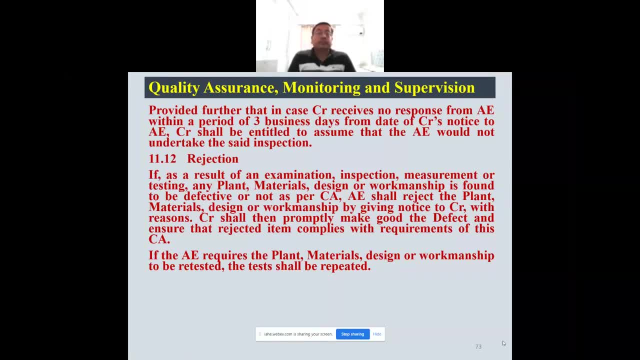 Now coming to rejection. If, as a result of an examination, inspection, measurement or testing, any plant material, design or workmanship is found to be defective or not as per the agreement, A authority engineer shall reject the plant. the plant is not as per the standard it. 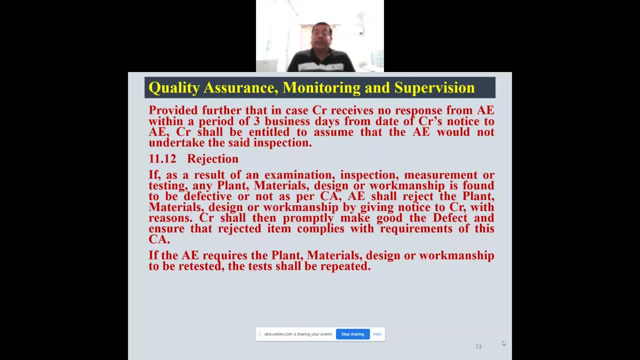 is not computerized. it is not, it will not give proper mixing as per the computerized standard. So if the plant is defective or not, then the contractor will not accept the payment. If the plant is defective or not, then the contractor will not accept the payment. 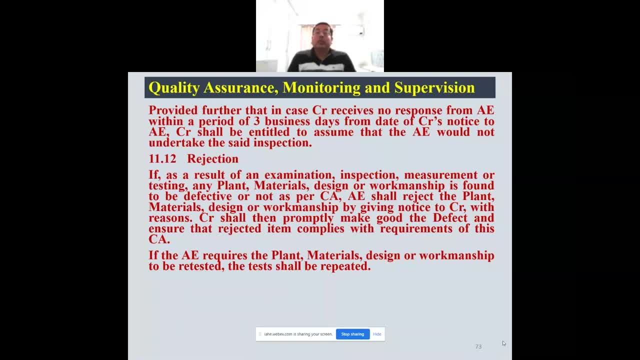 to change it. so a 13 year has to inspect, measure or test any plant material, design or workmanship and in case of any defect or if it is not as per agreement, he shall reject the plant material. suppose material aggregate is not. as for the three, sites are not broken if it is not. 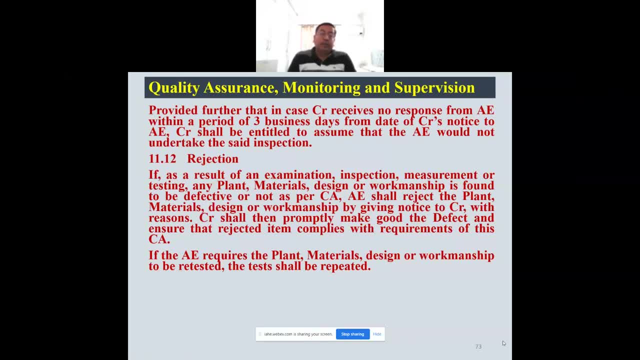 as per the specification standard. it is payables. so he may reject. design or workmanship is not good. your machine is not functioning. it is not in line, it is. alignment is different, it is changed. then he may give notice to the contractor with reasons. contractor shall then promptly make good. 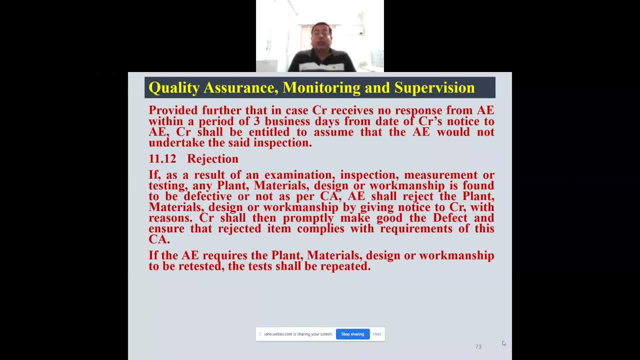 the defects. all the defects will be promptly make good by the contractor and it will be insured by the contractor that rejected items complies with requirement of this agreement. if the 13 year requires the plant material, design or workmanship to be retested- suppose a 30- 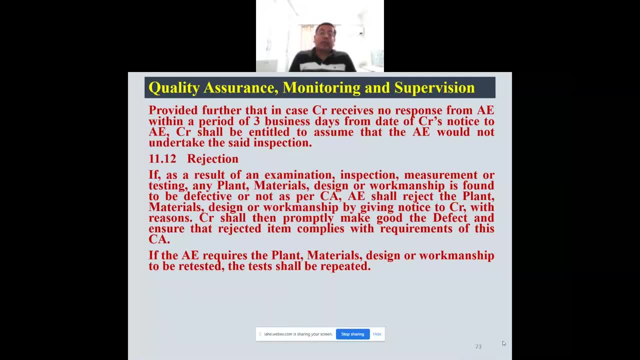 engineer: after hmp was rejected, contractor brought another hmp or if aggregates were rejected, he brought another aggregates. he changed the design or he had again and workmanship he had changed. the machine and workmanship has been improved, settling, centering, everything has been improved and even though after submitting all the things by the contractor初, 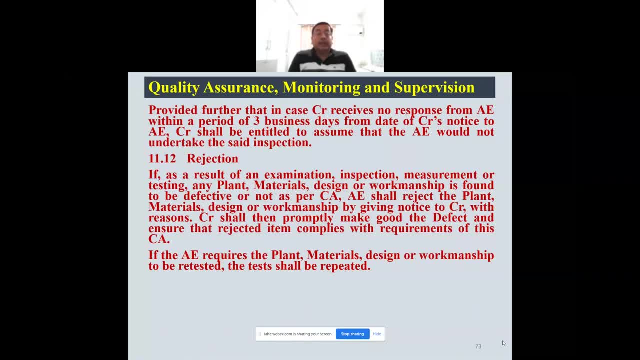 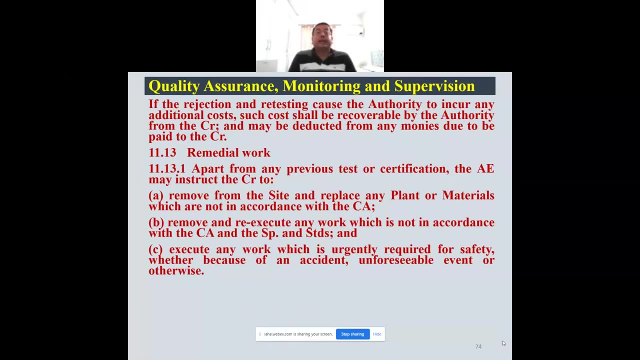 though, after submitting all the things by the contractor authority requires the 13 year requires to be retested, the test has been repeated by the contractor. probe if the rejection and retesting, if the rejection and retesting, if the rejection and retesting cause the 30 to incur any additional cost, Suppose rejection. and 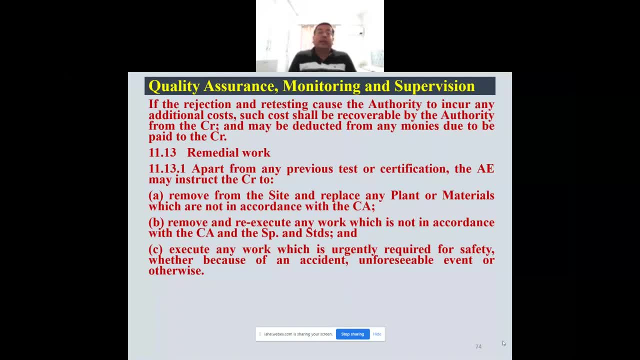 retesting cause about 50 lakh additional cost. Such cost shall be recoverable by the 30 from any money due to be paid to the contractor. HMP and material and all the things were tested by some lab and it took about 5 lakh. 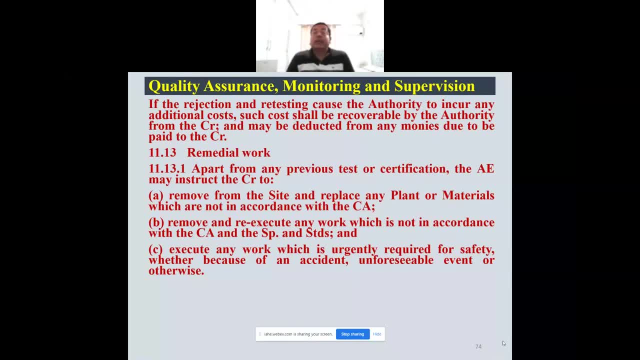 rupees. then this will be paid by contractor and if it is not paid by the contractor, a 30 will deduct from its bill or any money due to be paid to the contractor Remedial work Apart from any previous test or certification. the 30- 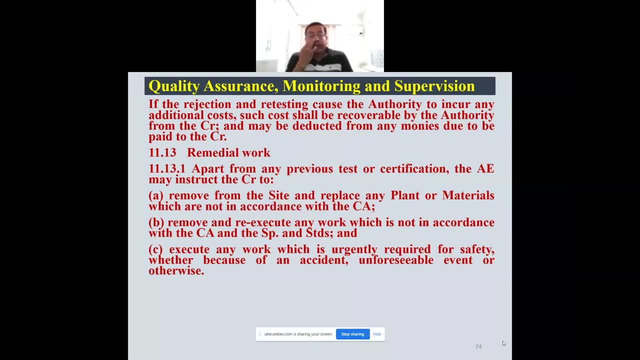 engineer may instruct the contractor to first remove from the site and replace any plant or materials which are not in accordance. site, Not only rejection. suppose HMP has been rejected or aggregates have been rejected, then they will have to be removed from the site and replaced with a good one. So this is 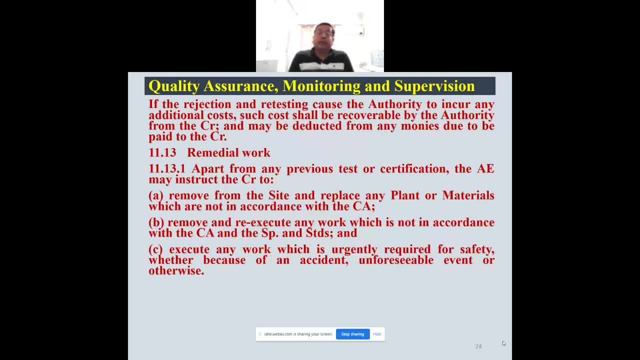 also a duty. Suppose you have rejected the HMP and still it is lying there, He may use it. Similarly, aggregates have been rejected and it is still at site, So all these things are to be removed from the site and replaced with good one. 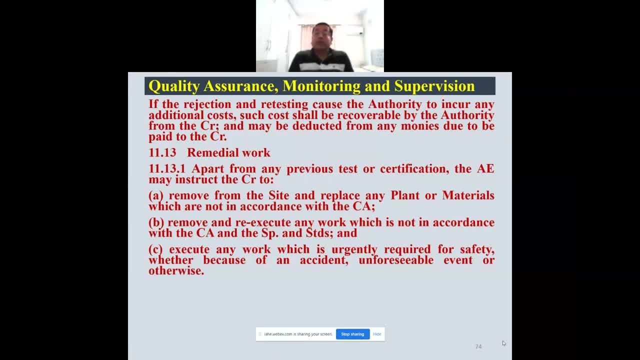 Second, remove and re-execute any work which is not in accordance with the CA and specimen. Suppose some work has been done and it is not as per the agreement and specimen standard, Then he has to remove and re-execute it. He will have to. 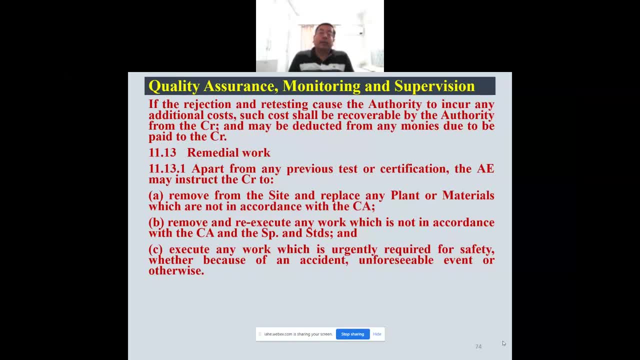 re-execute. Suppose GSB was not up to the mark, then he will have to remove that portion of the GSB and re-execute GSB and then it must fulfill the standard of the agreement and the specification standard. The authority engineer may also instruct to the contractor to re-execute any work which is 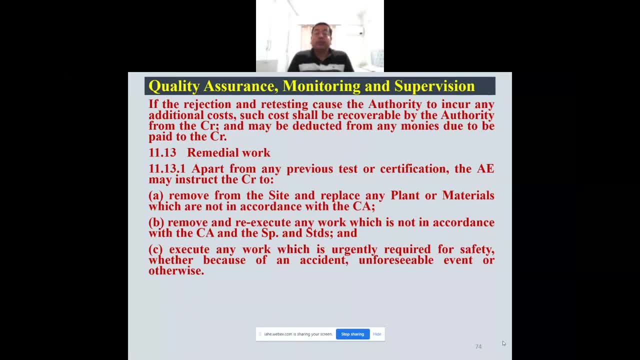 urgently required for safety. Suppose some safety work is urgently required. Authority may ask the contractor to urgently do this work, Whether because of an accident, unforeseeable event or otherwise. Suppose some accident has occurred and this work is essentially and urgently required and this was not known earlier. 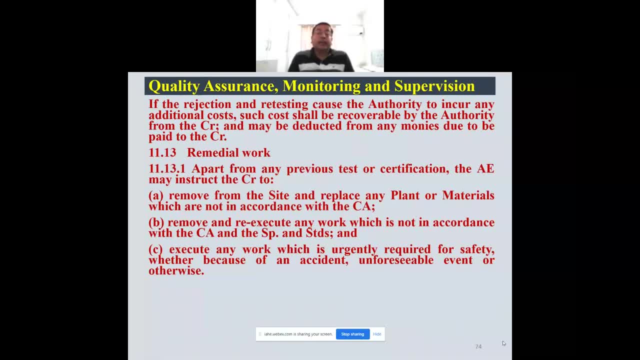 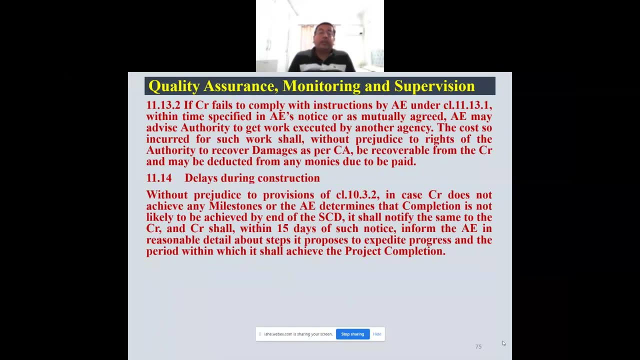 so unforeseeable and in that event the contractor has to do it expeditiously forthwith, as per instruction of the authority engineer. Otherwise it will be default of the contractor. Suppose the contractor fails to comply with instruction by authority engineer. Suppose, after writing by the authority engineer, contractor fails to comply comply. 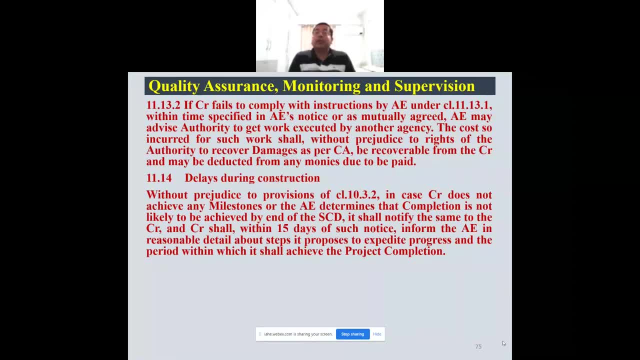 with the instruction by authority engineer under clause 11.13.1, within time specified in authority engineer's notice or as mutually agreed, authority engineer may advise authority to get work executed by another agency. Now, this is a very important clause. Suppose this is. 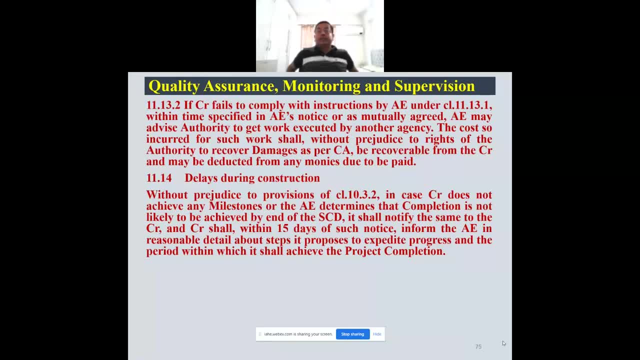 supported by intellectual review for such work, Suppose contractor again fails to comply with AE. special instruction for AE помогation work. Sale without prior right of the authority to recover damages per CA be recoverable from the contractor may be deducted from anyone. 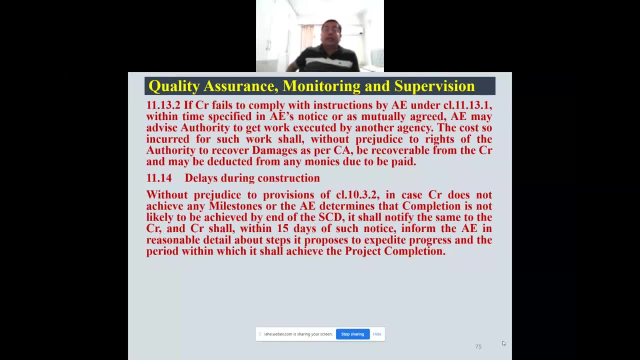 In that case authority will engage another agency and get the work done and will recover as damages from the contractor the amount which has been incurred by the authority for doing that work from the another agency. So it is well defined. In case of failure of the contractor you can get it annulated from another agency and you 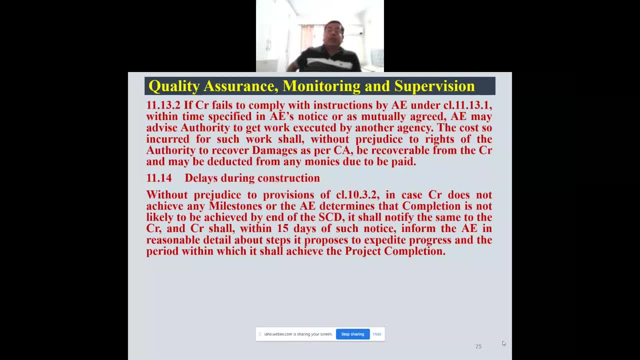 can deduct the money, any money due of the contractor you can deduct from the bill or any money due from the contractor. Delay during construction, Without prejudice to provision of clause 10.3.2, in case contractor does not achieve any milestone or the authority in linear determines that completion is not likely to be achieved. 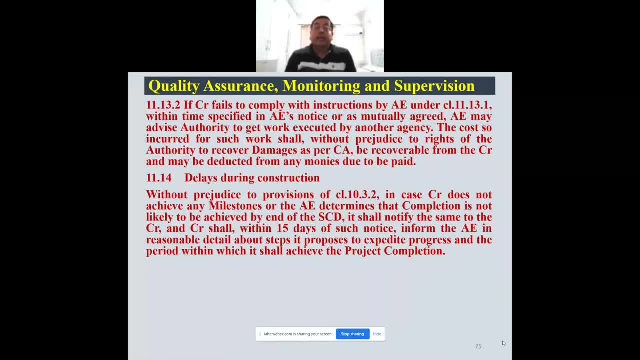 By end of the schedule completion date. it shall notify the same to the contractor. suppose authority engineer understand that he is going very slow and he failed to achieve the milestone and authority engineer becomes sure that the work will not be completed within the defined schedule completion date. 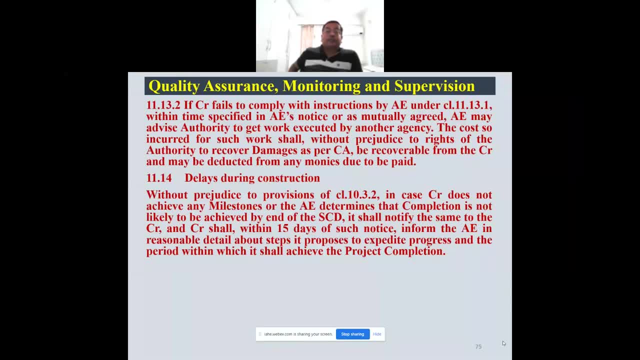 Then it will notify the contractor within 15 days of completion date. Then it will notify the contractor Within 15 days of completion. Then it will notify the contractor and the contractor within 15 days of such notice. inform the authority engineer in reasonable details about the steps it proposes to expedite progress. 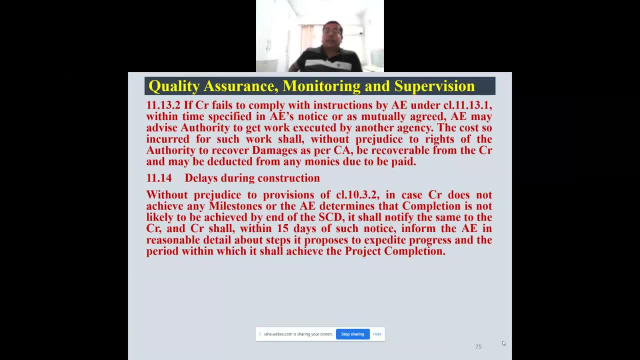 and the period within which it shall achieve the project completion. In that case, contractor will promptly, within 15 days, inform the AE in reasonable details about the steps which contractor is proposed to expedite progress and period within which it shall achieve the project completion. It means that in case of any lag- time lag if it is in the opinion of the authority engineer. 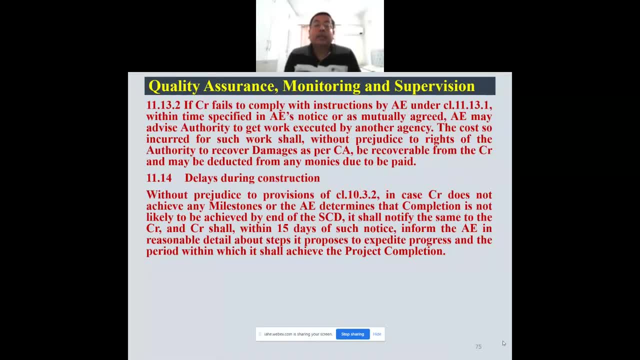 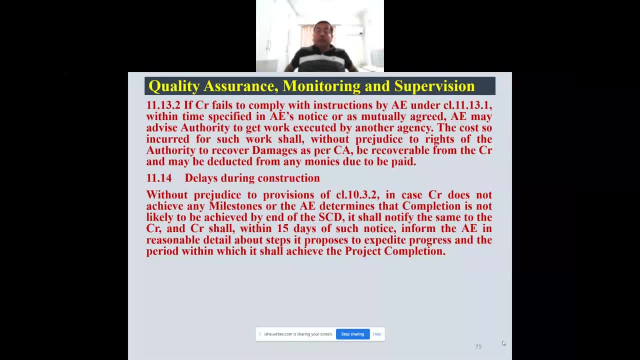 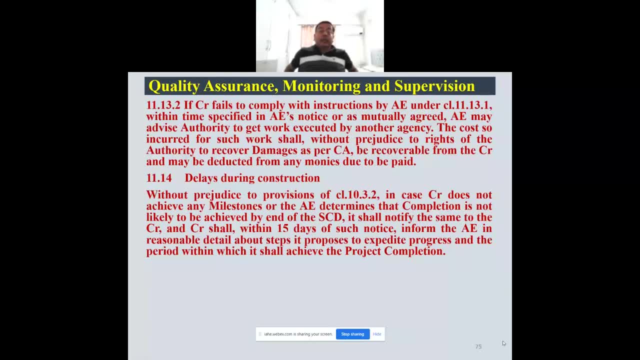 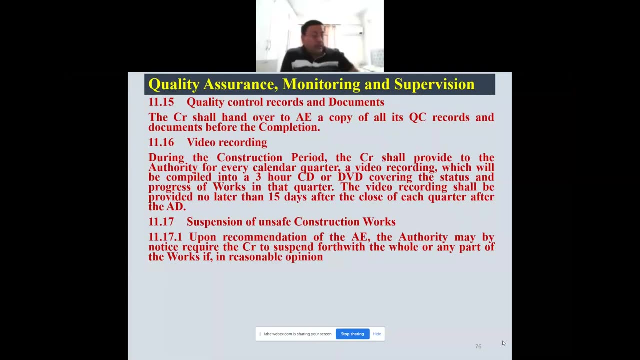 is being done. In that case authority engineer may give notice and contractor has to immediately send its report and its proposal to expedite the progress. Then up to tracking for anyagus impact in anyakali anyakali site and where we have to bring it to the IRCV, SRE, the property tax, as wise to manage私. 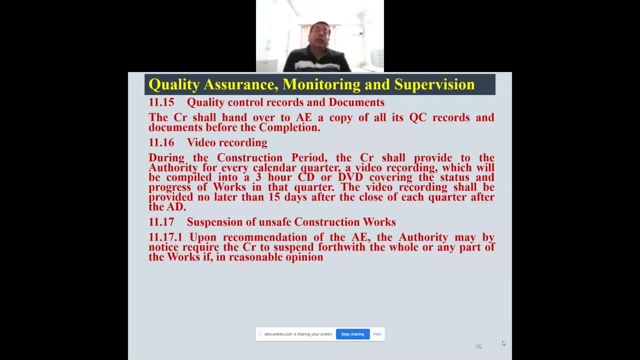 to approve it. This process is also required. So this is the first step. Next step: you must have quality control reports so that if any part is having some problem, distress, then you can see that it is as per a specification or standard and it has been tested and it has. 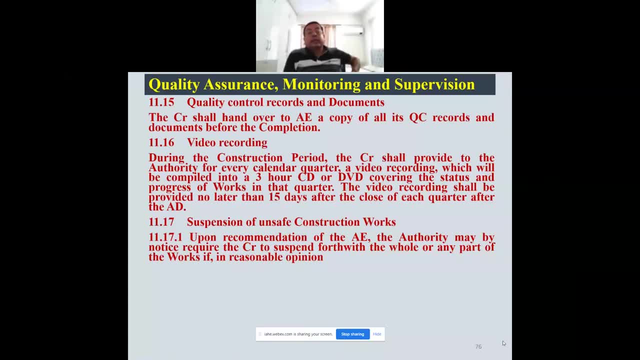 qualified as per a test. it is within the acceptance criteria. it has been accepted as per the acceptance criteria. so all these records of the quality control documents had to be funded by the contractor before completion. to the 30 year now, video recording during the construction period. the contractor shall provide to the 30, for every calendar quarter, a video recording. 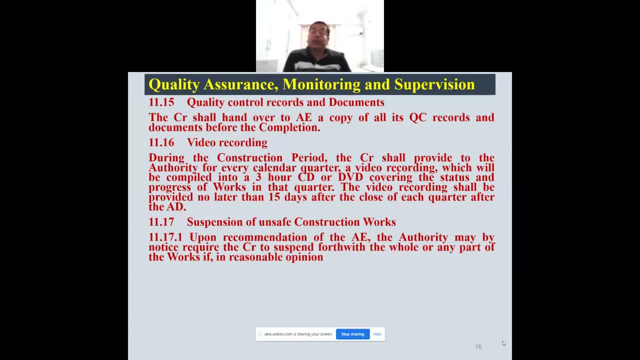 during construction period. every quarter calendar quarter, a video recording which will be compiled to three hour cd or dvd covering the status and progress of works in that quarter. for every quarter of the construction period, contractor has to furnish a cd or dvd of three hours. the video recording shall be provided no later than 15 days after the close of each quarter. 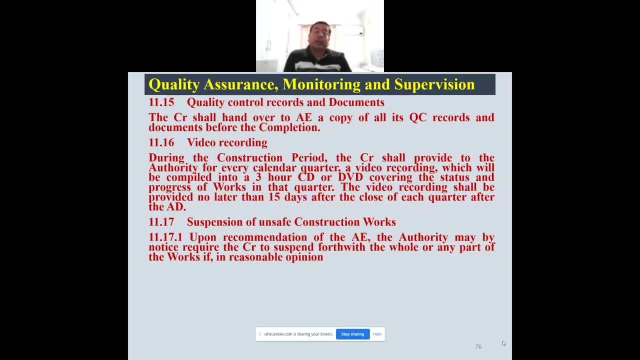 after the appointed date at the end of every quarter. within 15 days they will. the contractor will furnish the video recording to the authority, engineer or authority. suspension of unsafe construction works. suspension of unsafe construction works. suspension of unsafe construction works. this is also mentioned. why it is mentioned? 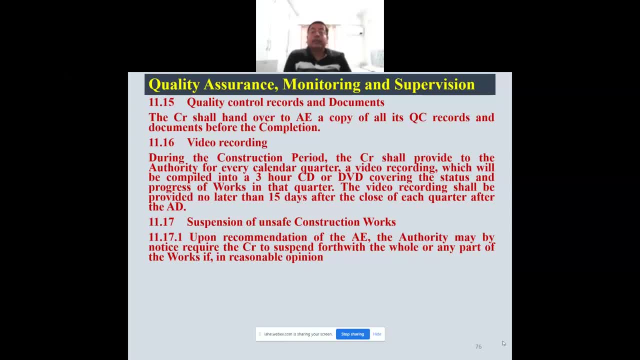 this is also mentioned. why it is mentioned? this is also mentioned. why it is mentioned? because in case of unsafe construction work, it is because, in case of unsafe construction work, it is because, in case of unsafe construction work, it is, uh, dangerous for the user of the road. so it is. 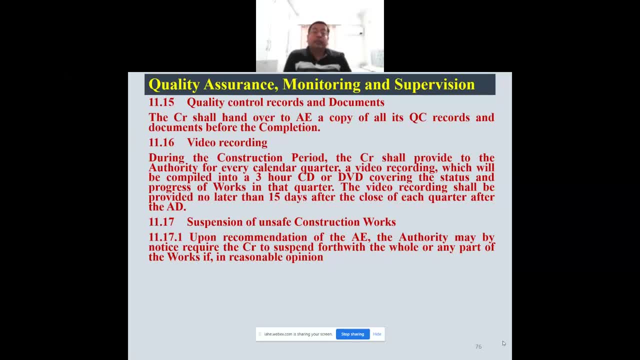 uh dangerous for the user of the road. so it is uh dangerous for the user of the road. so it is your responsibility, and so it has been written. your responsibility, and so it has been written, your responsibility, and so it has been written in the agreement. upon recommendation of the. 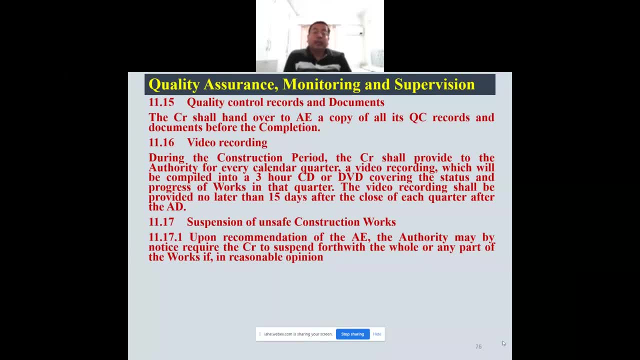 in the agreement upon recommendation of the. in the agreement upon recommendation of the authority engineer the authority may, by authority, engineer the authority may, by authority, engineer the authority may, by notice, require the contractor to suspend notice. require the contractor to suspend notice. require the contractor to suspend force with the whole or any part of the. 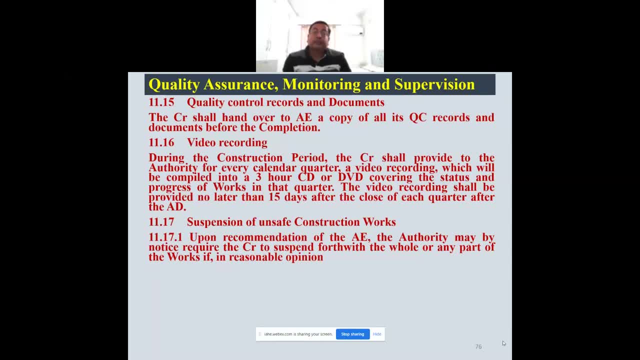 force, with the whole or any part of the force. with the whole or any part of the works, if in reasonable opinion works. if in reasonable opinion works. if in reasonable opinion of the age. such works threaten the of the age. such works threaten the of the age. such works threaten the safety of the users and pedestrian. 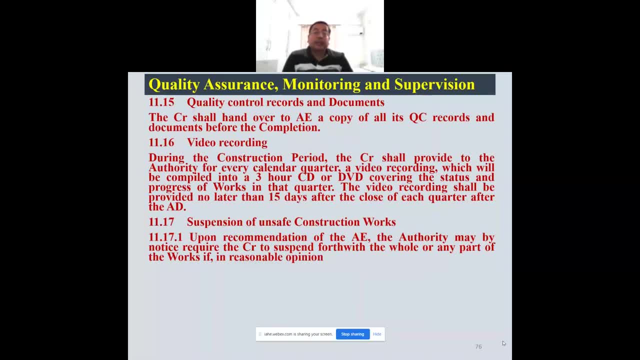 safety of the users and pedestrian: safety of the users and pedestrian. it means upon recommendation of the 30. it means upon recommendation of the 30. it means upon recommendation of the 30: engineer: the authority may engineer, the authority may engineer. the authority may, by notice, require the contractor to. 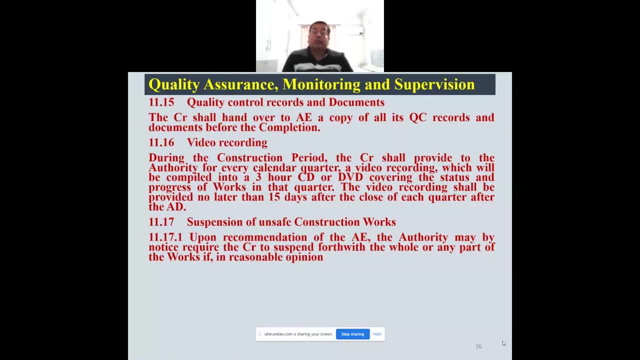 by notice. require the contractor to, by notice, require the contractor to suspend force with the whole or any part. suspend force with the whole or any part. suspend force with the whole or any part of the work, of the work, of the work which part of the work which is unsafe. 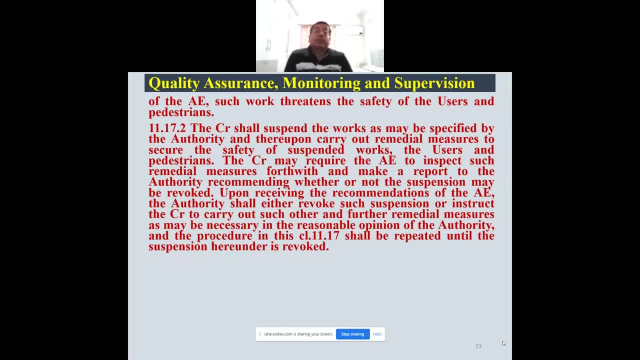 which part of the work which is unsafe, which part of the work which is unsafe as per a. as per a. as per a. such work threatens the safety of the such work, threatens the safety of the such work, threatens the safety of the users and pedestrians. users and pedestrians. 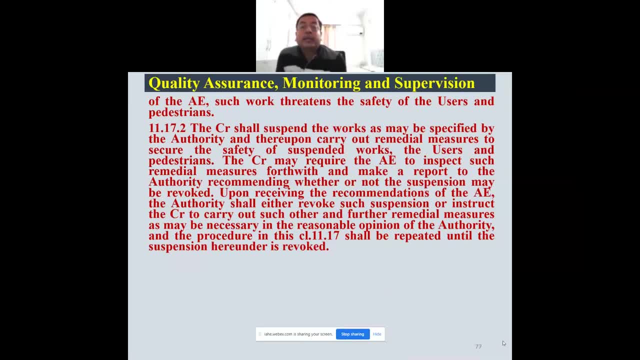 users and pedestrians, so you can ask the contractor not to do so. you can ask the contractor not to do so. you can ask the contractor not to do and it is unsafe. you rectify it and it is unsafe. you rectify it and it is unsafe. you rectify it and stop the work until safety measures. 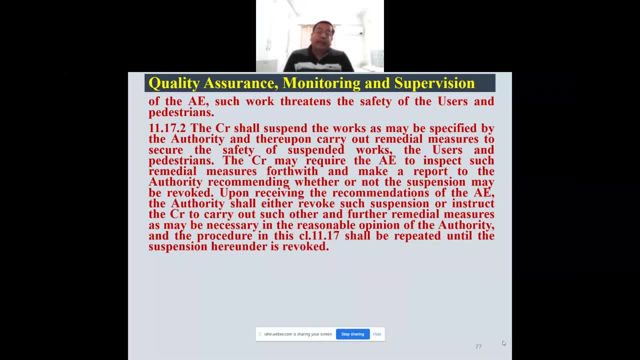 and stop the work until safety measures and stop the work until safety measures are being taken. 11.17.2. the contractor shall suspend the works. the contractor shall suspend the works. the contractor shall suspend the works as may be specified by the authority and as may be specified by the authority. and. 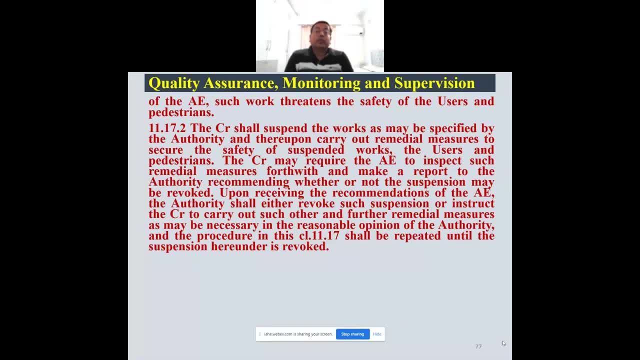 as may be specified by the authority and thereupon carry out remedial measures. to thereupon carry out remedial measures. to thereupon carry out remedial measures to secure the safety of suspended works. secure the safety of suspended works. secure the safety of suspended works, the contractor shall suspend the works. 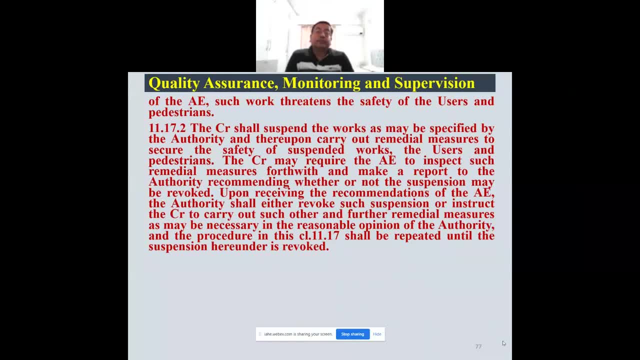 the contractor shall suspend the works. the contractor shall suspend the works as may be specified by the authority. the contractor will immediately suspend. the contractor will immediately suspend. the contractor will immediately suspend the work as may be specified by the. the work as may be specified by the. the work as may be specified by the, and thereupon carry out remedial measures. 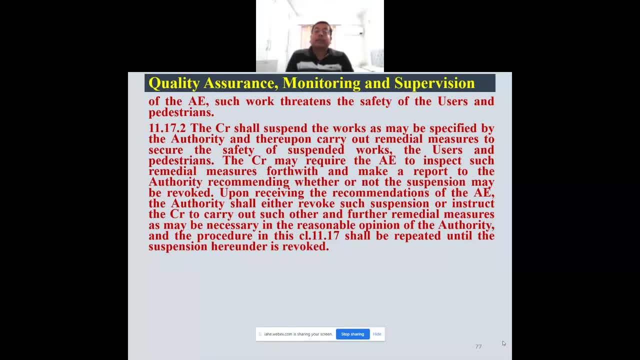 and thereupon carry out remedial measures. and thereupon carry out remedial measures to secure the safety of suspended, to secure the safety of suspended, to secure the safety of suspended works, works, works. he will say: take remedial measures to. he will say: take remedial measures to. 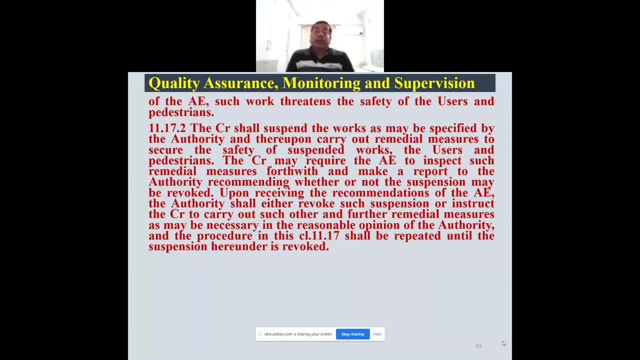 he will say, take remedial measures to secure the safety of suspended works. secure the safety of suspended works. secure the safety of suspended works, the users and pedestrians. the contractor. the users and pedestrians. the contractor. the users and pedestrians. the contractor may require the authority engineer to. may require the authority engineer to: 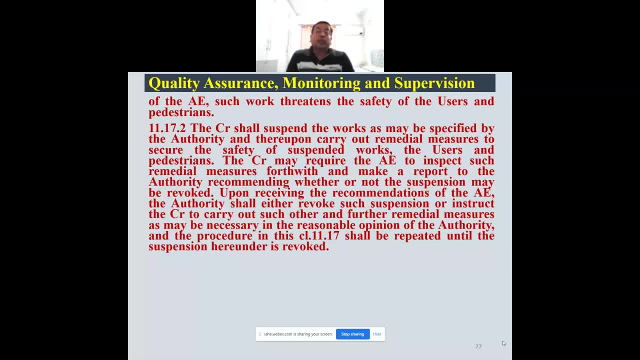 may require the authority engineer to inspect such remedial measures forthwith. inspect such remedial measures forthwith. inspect such remedial measures forthwith and make a report to the authority. and make a report to the authority. and make a report to the authority recommending whether or not the suspend. 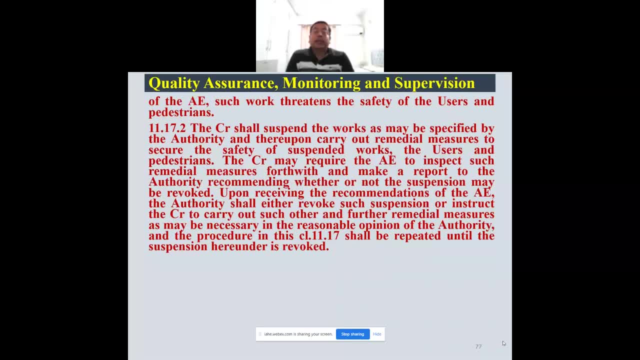 recommending whether or not the suspend. recommending whether or not the suspend suspension may be revoked. suspension may be revoked. suspension may be revoked. suppose such thing has happened in that. suppose such thing has happened in that. suppose such thing has happened in that contractor will contractor will contractor will ask the authority to inspect such. 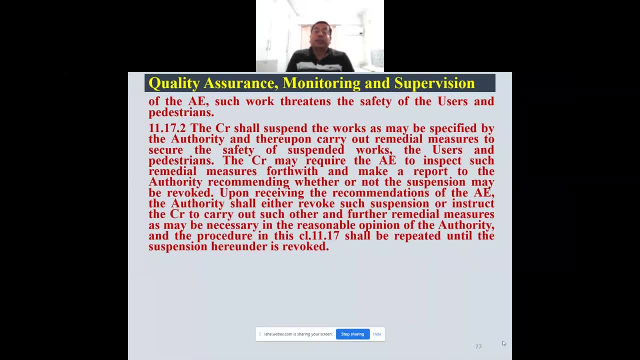 ask the authority to inspect such. ask the authority to inspect such remedial measures done by contractor. remedial measures done by contractor. ask the authority to inspect such remedial measures done by contractor, and forth with make a report to and forth with make a report to and forth with make a report to the authority recommending whether or not. 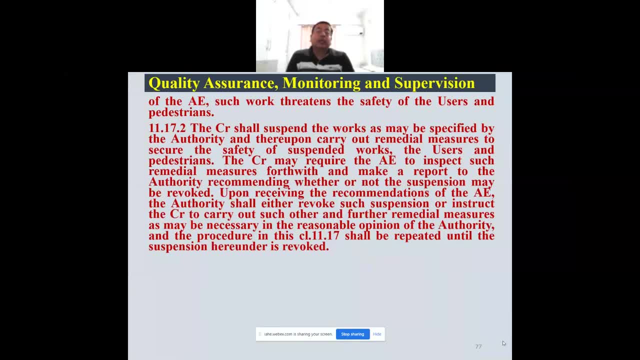 the authority recommending whether or not the authority recommending whether or not the suspended work may be revoked. the suspended work may be revoked, the suspended work may be revoked. so this is also written because. so this is also written, because so this is also written because contractor has done the work, but 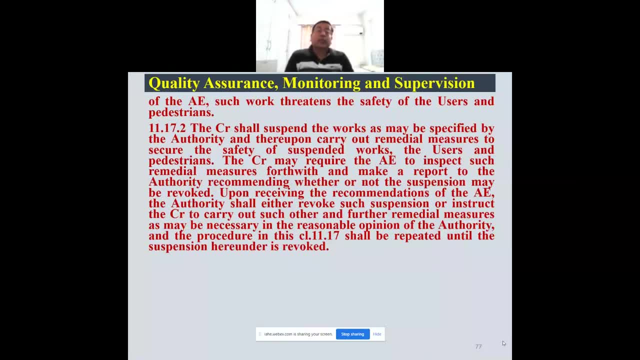 contractor has done the work. but contractor has done the work, but 13, you know, is not taking action. so 13, you know, is not taking action. so 13, you know, is not taking action. so this is written so that a 13 year may. this is written so that a 13 year may. 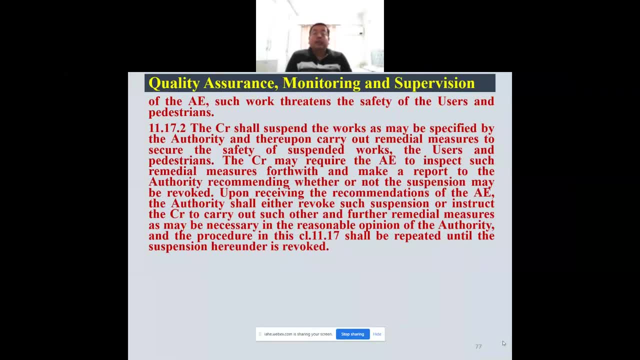 this is written so that a 13 year may take quick action. take quick action. take quick action. upon receiving the recommendation of the. upon receiving the recommendation of the. upon receiving the recommendation of the 13 year, the 30 cell. either revoke such 13 year, the 30 cell, either revoke such. 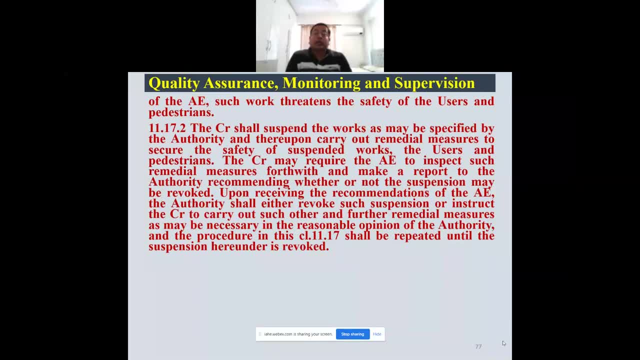 13 year, the 30 cell, either revoke such a suspension or instruct the contractor a suspension, or instruct the contractor a suspension or instruct the contractor to carry out such other and further. to carry out such other and further. to carry out such other and further remedial measures as may be necessary in 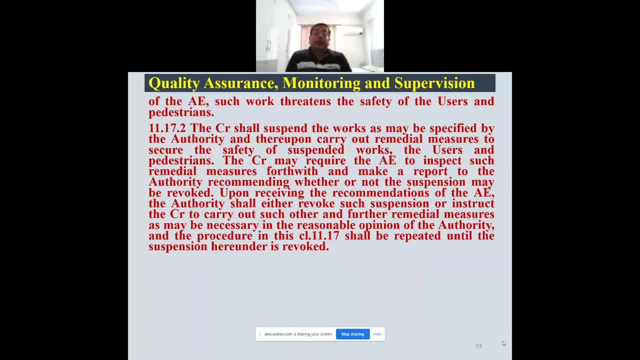 remedial measures, as may be necessary in remedial measures, as may be necessary in the reasonable opinion of the 30. what a the reasonable opinion of the 30? what a the reasonable opinion of the 30? what a 13 year will do after recommendation? 13 year will do after recommendation. 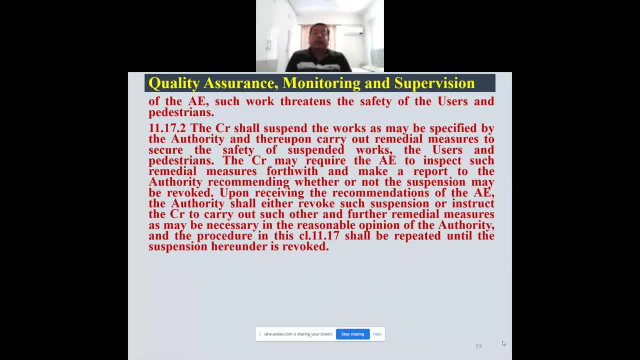 13 year will do. after recommendation 30, you will recommend that this work is 30. you will recommend that this work is 30. you will recommend that this work is remedied and it is now safe. and a 30- remedied and it is now safe. and a 30. 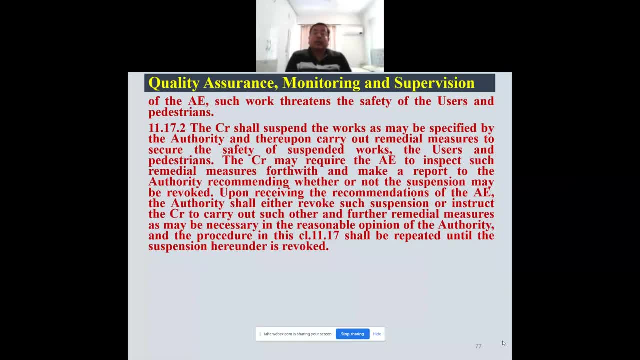 remedied and it is now safe and a 30 may remove such suspension or instruct. may remove such suspension or instruct. may remove such suspension or instruct the contractor to carry out such other the contractor to carry out such other the contractor to carry out such other works and further remedial measures as: 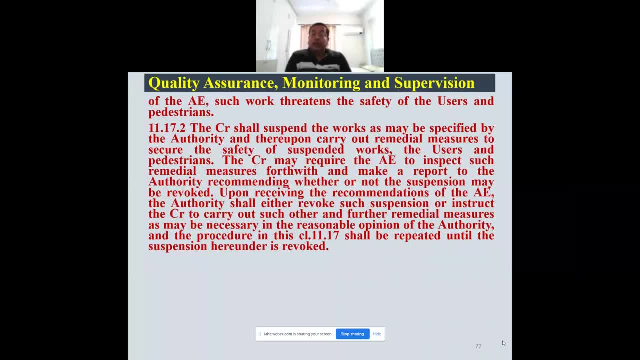 works and further remedial measures as works and further remedial measures as may be necessary in the reasonable, may be necessary in the reasonable, may be necessary in the reasonable opinion. suppose you have asked 13 year a opinion. suppose you have asked 13 year a opinion. suppose you have asked 13 year. a 13 year is saying that it is safe still. 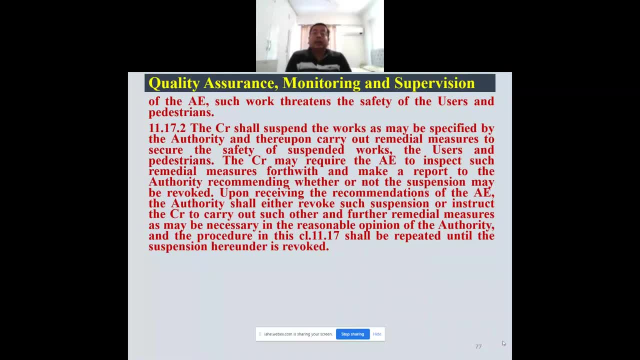 13 year is saying that it is safe still. 13 year is saying that it is safe still. you can go to the site and see, and you, you can go to the site and see, and you, you can go to the site and see, and you can ask the contractor to do something. 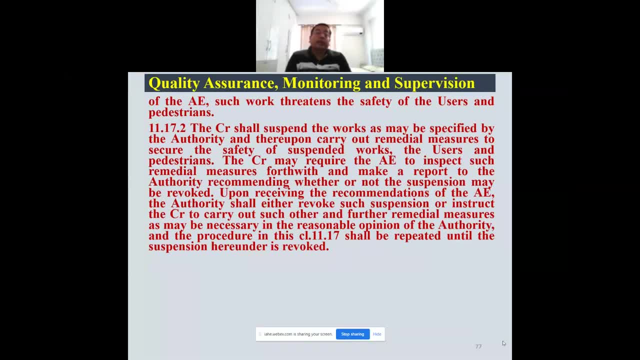 can ask the contractor to do something, can ask the contractor to do something else so that the work may be very much else, so that the work may be very much else, so that the work may be very much safe for the engine and the procedure of safe for the engine and the procedure of. 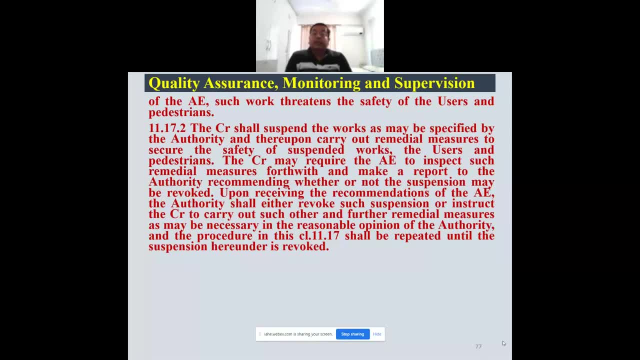 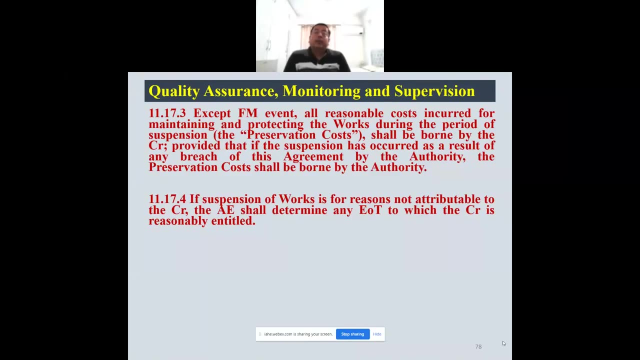 safe for the engine and the procedure of this clause shall be repeated until the this clause shall be repeated until the this clause shall be repeated until the suspension is revoked, except force suspension is revoked. except force suspension is revoked except force. measure event: all reasonable costs. measure event: all reasonable costs. 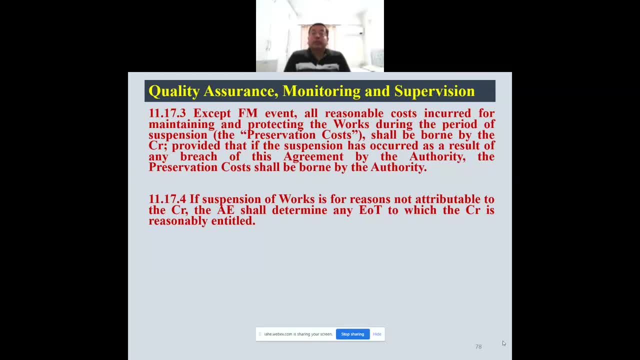 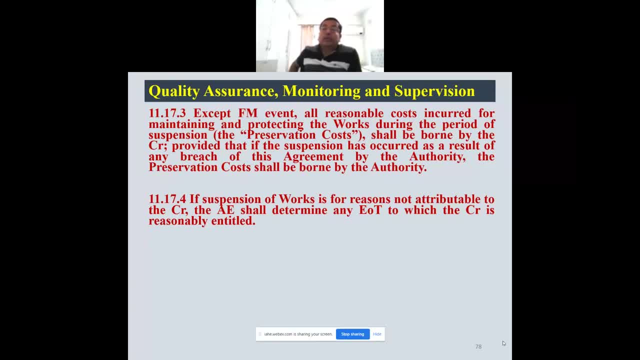 cost incurred for maintaining and cost incurred for maintaining and protecting the works during the period. protecting the works during the period. protecting the works during the period of suspension. the preservation cost shall of suspension. the preservation cost shall of suspension. the preservation cost shall be borne by the contractor, provided that 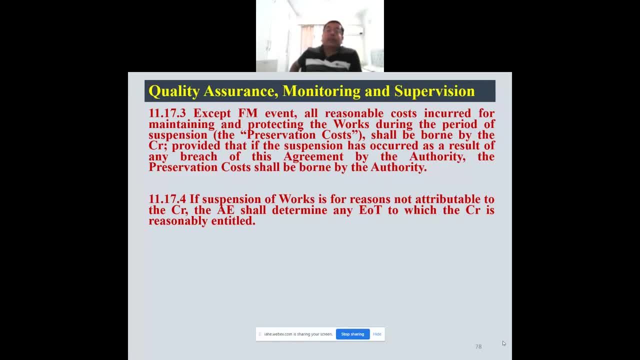 be borne by the contractor. provided that be borne by the contractor. provided that if suspension has occurred as a result, if suspension has occurred as a result, if suspension has occurred as a result of any breach of this agreement by the, of any breach of this agreement by the. 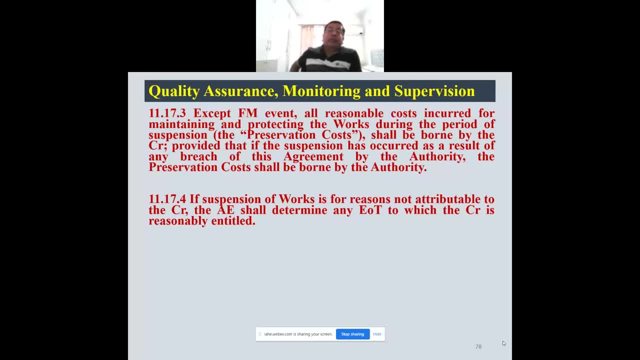 of any breach of this agreement by the authority, the present the preservation authority, the present the preservation authority, the present the preservation cost shall be borne by the authority. it cost shall be borne by the authority. it cost shall be borne by the authority. it has been clearly defined that this in: 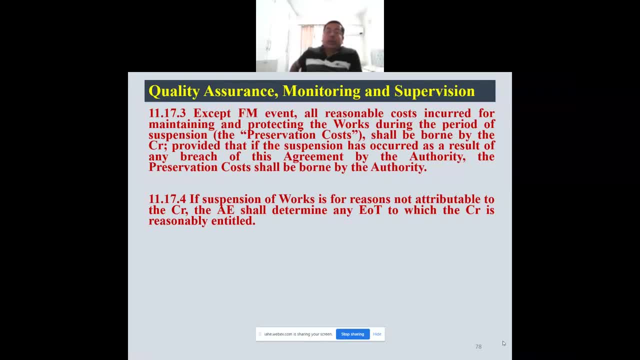 has been clearly defined that this in has been clearly defined that this: in case it is not force measure event or a case it is not force measure event or a case it is not force measure event or a 30 default. all these things are to be 30 default. all these things are to be: 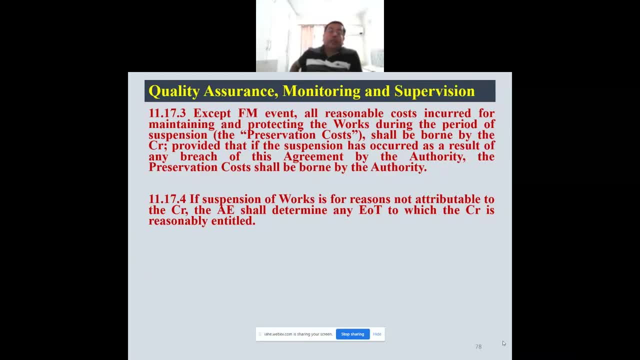 30. default. all these things are to be borne by the contractor. but in case it borne by the contractor, but in case it borne by the contractor, but in case it is force measure event or default by the. is force measure event or default by the? is force measure event or default by the authority, the preservation cost shall be. 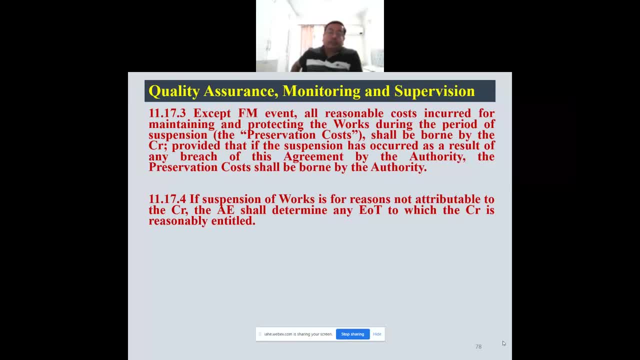 authority. the preservation cost shall be authority. the preservation cost shall be borne by the authority. if suspension of borne by the authority. if suspension of borne by the authority. if suspension of works is for regions not attributable to works is for regions not attributable to works is for regions not attributable to the contractor. suppose suspension of. 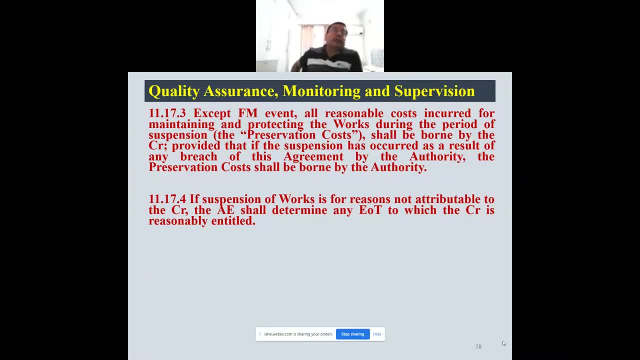 the contractor. suppose suspension of the contractor. suppose suspension of working for region not attributable to working for region not attributable to working for region not attributable to the contract contractor has not made any. the contract contractor has not made any. the contract contractor has not made any mistake, he has not made any default. why? 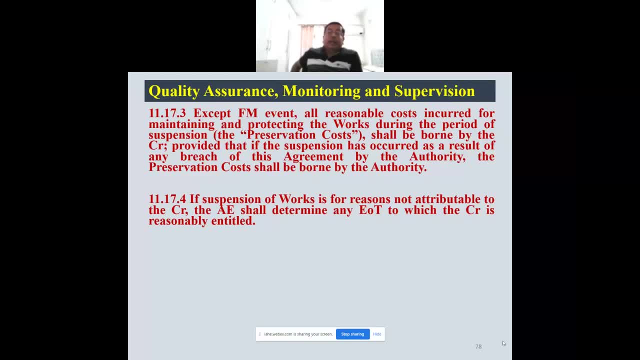 mistake? he has not made any default. why mistake he has not made any default? why he should rectify, in that case the 30, he should rectify, in that case the 30, he should rectify, in that case the 30. engineers shall determine any EOT to. 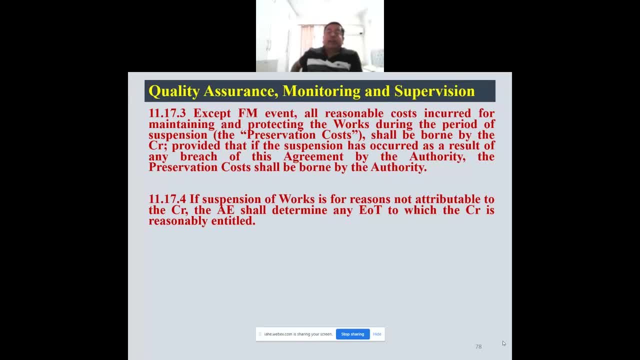 engineers shall determine any EOT to. engineers shall determine any EOT to which the contractor is reasonably, which the contractor is reasonably, which the contractor is reasonably entitled. in that case he will get time entitled. in that case he will get time entitled. in that case he will get time extension. extension of time will be. 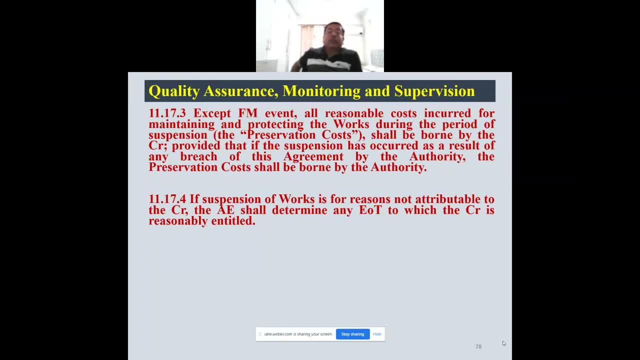 extension of time will be provided to the contractor for this. because it is provided to the contractor for this, because it is provided to the contractor for this, because it is not his default, and why it not his default and why it not his default and why it should be suspended in this case, a. 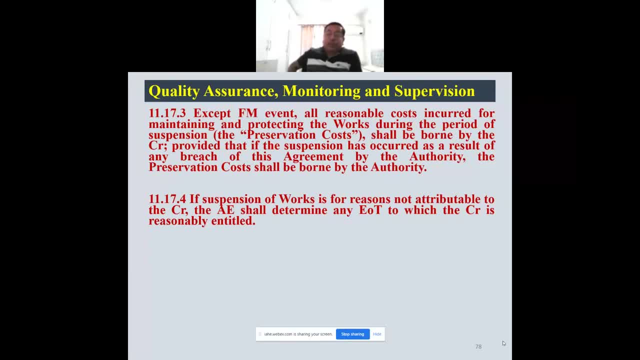 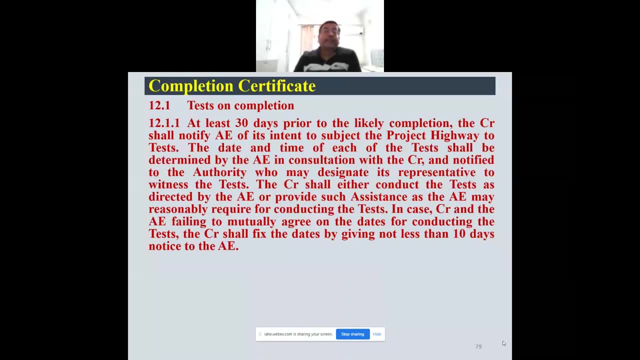 should be suspended. in this case, a should be suspended. in this case, a contractor will get time extension from contractor, will get time extension from contractor, will get time extension from the authority. now, I think, sir, we can the authority now. I think, sir, we can the authority now. I think, sir, we can take questions. sir, please ask me, we can. 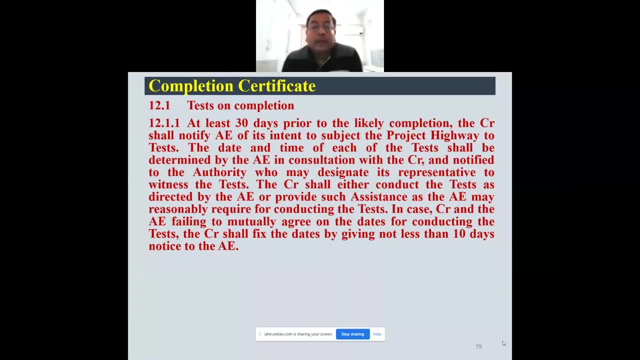 take questions, sir, please ask me. we can take questions, sir, please ask me. we can take questions. we will continue in take questions. we will continue in take questions. we will continue in second officer. okay, okay, second officer. okay, okay, second officer. okay, okay, any query? yes, sir, I do have one query, sir. 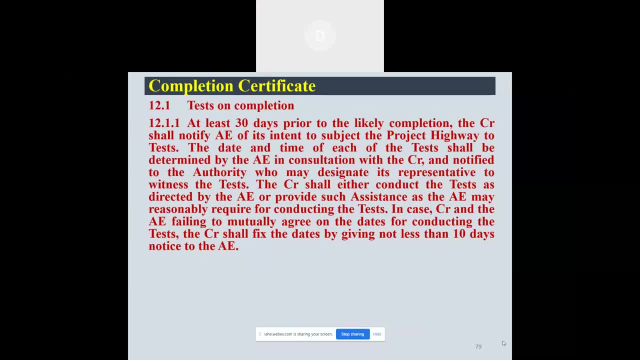 any query? yes, sir, I do have one query, sir, any query. yes, sir, I do have one query, sir, yes, yes, yes, suppose in schedule be number of. suppose in schedule be number of. suppose in schedule be number of straight-light poles are given. okay, so, straight-light poles are given, okay so. 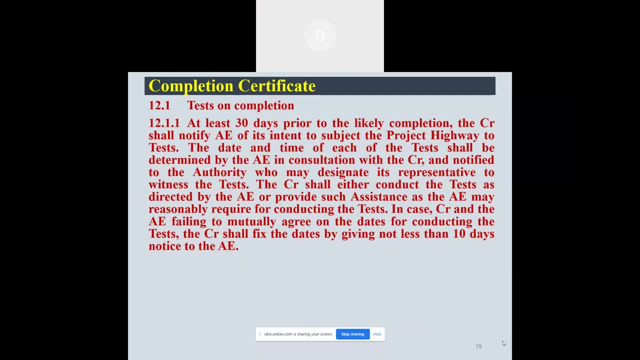 straight-light poles are given, okay. so number is mentioned there. suppose 40 number is mentioned there. suppose 40 number is mentioned there. suppose 40 numbers or 60 like that, okay. but when we numbers or 60 like that, okay. but when we numbers or 60 like that, okay. but when we go by the codal norms it comes on a. 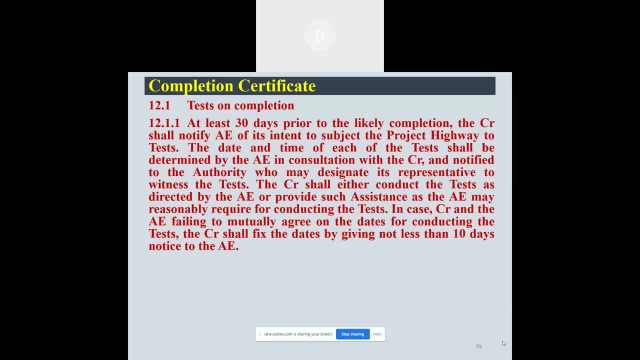 go by the codal norms. it comes on a go by the codal norms. it comes on a higher side. okay, but that schedule B is higher side. okay, but that schedule B is higher side. okay, but that schedule B is clearly delineated. so is there is. 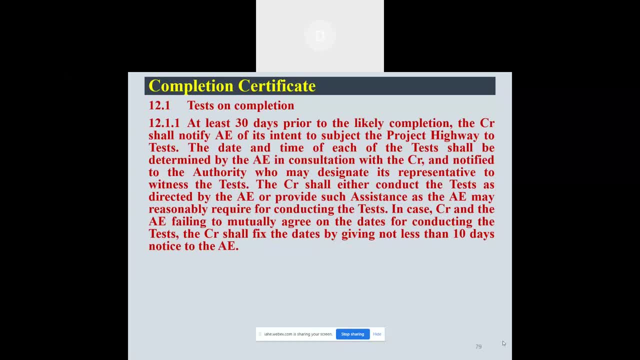 clearly delineated, so is there is clearly delineated, so is there is conflict between schedules B and schedule. conflict between schedules B and schedule, conflict between schedules B and schedule C. and contractor obviously will stick to C and contractor obviously will stick to C and contractor obviously will stick to the whatever is profitable to him. that 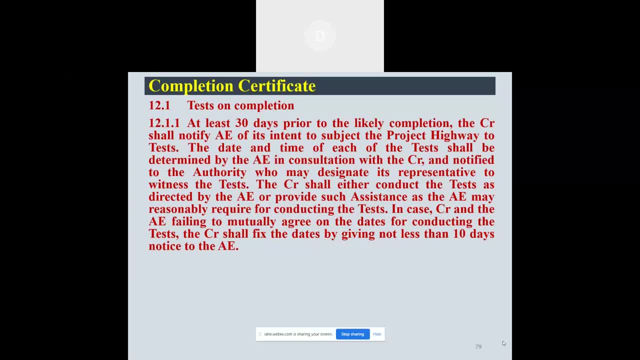 the whatever is profitable to him, that the whatever is profitable to him. that schedule only if you have defined the 60 schedule, only if you have defined the 60 schedule, only if you have defined the 60, poles in your seat will be and see to poles in your seat will be and see to. 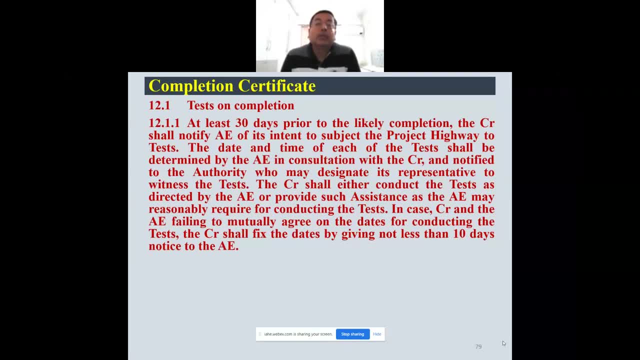 poles in your seat will be and see to see. to see, then he had to a dude. if you see to see, then he had to a dude. if you see to see, then he had to a dude. if you have not defined it, it will be followed. have not defined it, it will be followed. 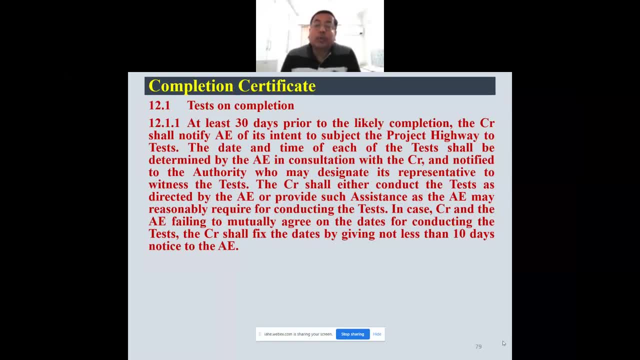 have not defined it. it will be followed as per manual. so yes, the polls have been as per manual. so yes, the polls have been as per manual. so yes, the polls have been defined by you in C to B and C. then he defined by you in C to B and C. then he: 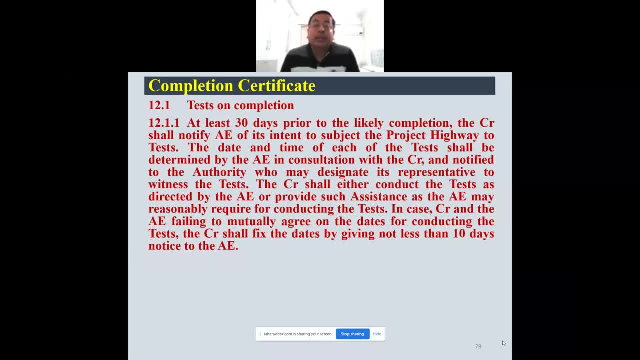 defined by you in C to B and C, then he will add you to without getting any, will add you to without getting any, will add you to without getting any additional money. but if we not mention additional money, but if we not mention additional money, but if we not mention, then, as per manual, if it is 40, he will. 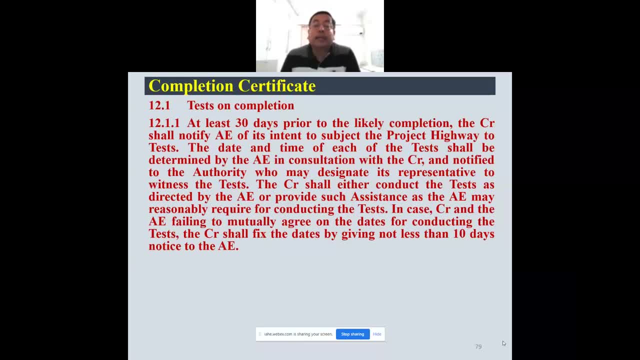 then as per manual. if it is 40, he will. then as per manual, if it is 40, he will provide only 40, and if he will provide provide only 40, and if he will provide provide only 40 and if he will provide 60, he will get additional payment for 20. 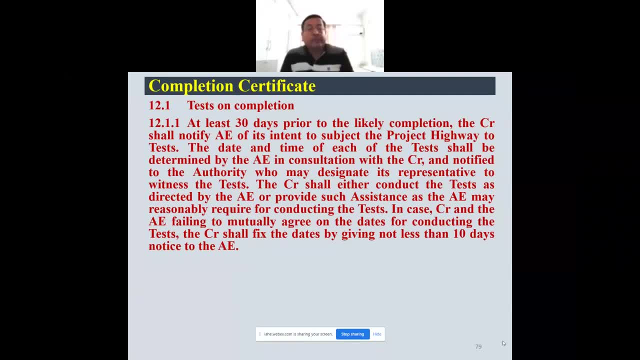 60. he will get additional payment for 20- 60. he will get additional payment for 20 because, as per manual, only 40 was, because, as per manual, only 40 was, because, as per manual, only 40 was required. yes, sir, it may be 30 or 35, so 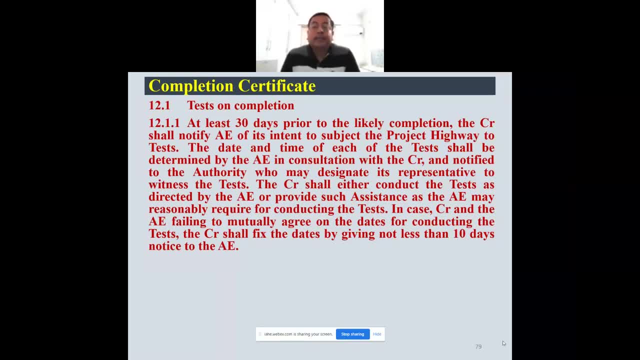 required: yes, sir, it may be 30 or 35. so required. yes, sir, it may be 30 or 35. so whatever is additional will have to be. whatever is additional will have to be. whatever is additional will have to be paid by the authority to the conductor. 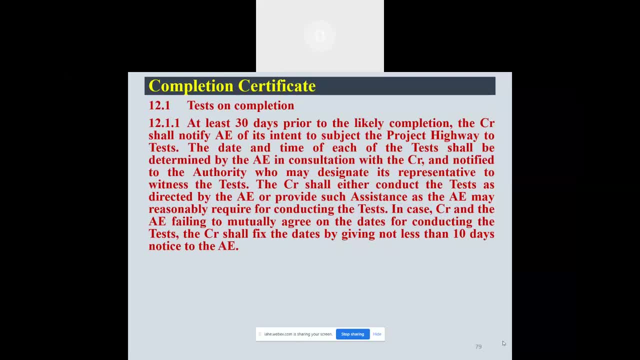 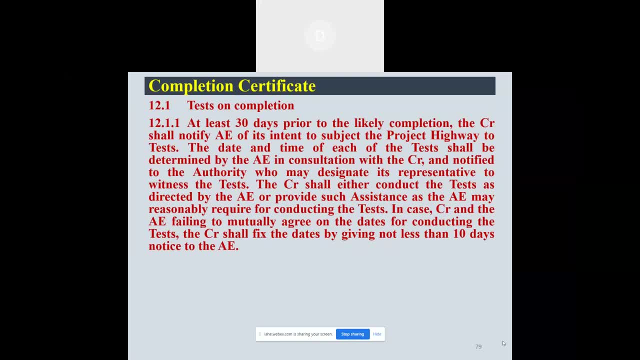 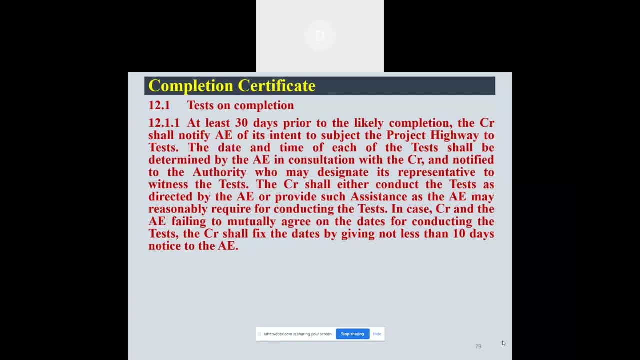 yeah, yes, sir, just I will know the. yeah, yes, sir, just I will know the officer in charge of the authority in officer in charge of the authority in officer in charge of the authority in bracket, it is pretty obligatory. oblig bracket, it is pretty obligatory. oblig bracket, it is pretty obligatory. oblig cgm, yeah. or in case of mark different, 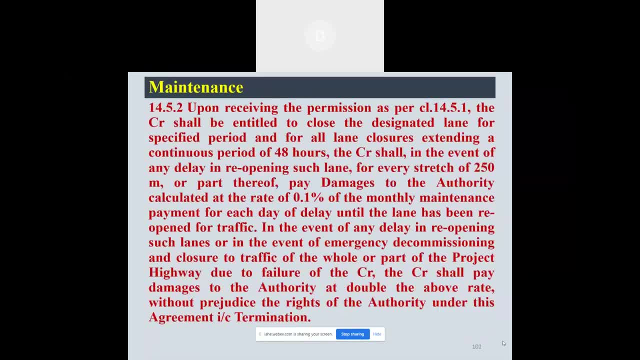 cgm- yeah, or in case of mark, different cgm- yeah. or in case of mark, different education are given. so is responsible education are given. so is responsible education are given. so is responsible for overall supervision and monitoring of. for overall supervision and monitoring of. for overall supervision and monitoring of the execution of the project. as the 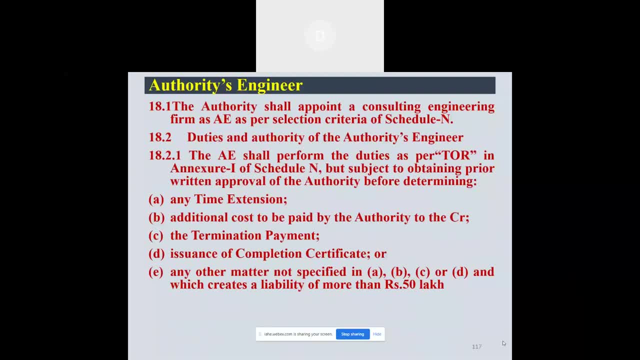 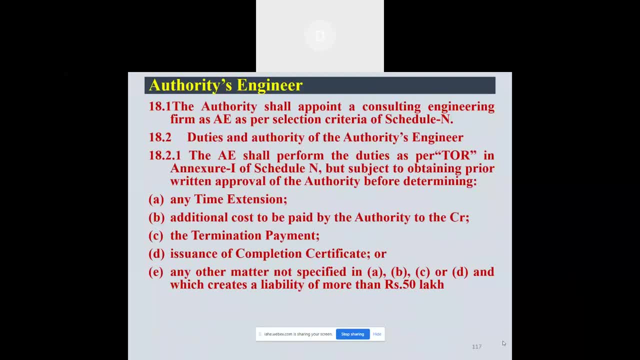 owner of the project. the authorities engineer is appointed to authorities engineer is appointed to authorities engineer is appointed to assist the authority for carrying out the assist. the authority for carrying out the assist, the authority for carrying out the function as detail under clause 18.2, as: 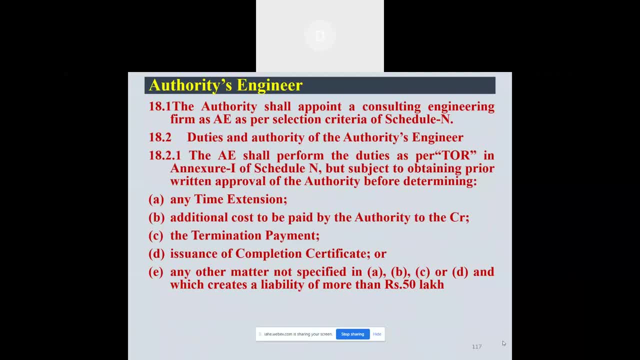 function as detail under clause 18.2. as function as detail under clause 18.2, as such an officer of the authority is such an officer of the authority is such an officer of the authority is vested with all such powers and vested with all such powers. and. 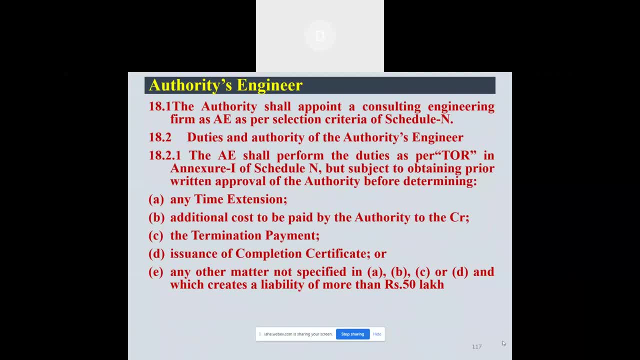 vested with all such powers and responsibilities as, or enjoined upon the responsibilities as, or enjoined upon the responsibilities as, or enjoined upon the authorities. engineer is fully competent authorities. engineer is fully competent authorities. engineer is fully competent to issue instruction of our proper. to issue instruction of our proper. 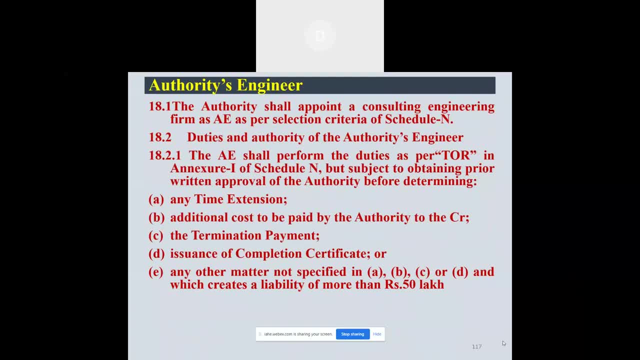 to issue instruction of our proper monitoring and supervision of the monitoring and supervision of the monitoring and supervision of the project, either by himself or through a hello. what is the question? so so so, sir, this type of clause was not, sir, this type of clause was not, sir, this type of clause was not there in our earlier. 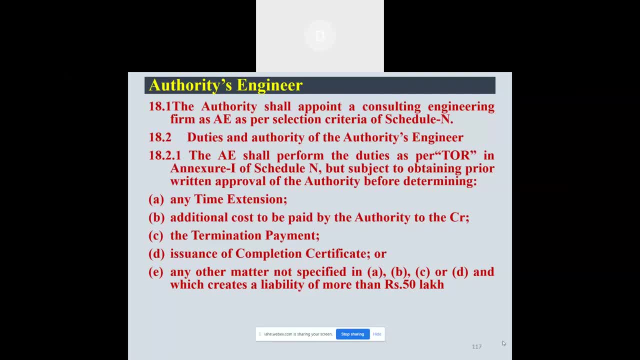 there in our earlier there in our earlier documents. now it is documents. now it is documents. now it is coming to the picture. so my question was coming to the picture, so my question was coming to the picture. so my question was: is there any kind of conflict between? 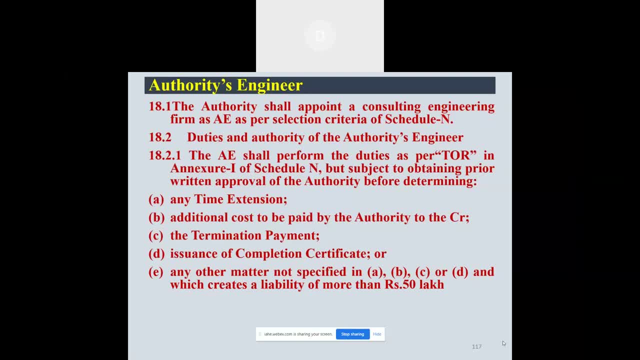 is there any kind of conflict between? is there any kind of conflict between, authorities role, because he is overall authorities role, because he is overall authorities role, because he is overall responsible. client is overall responsible, responsible client is overall responsible responsible. client is overall responsible for the quality and all these things. 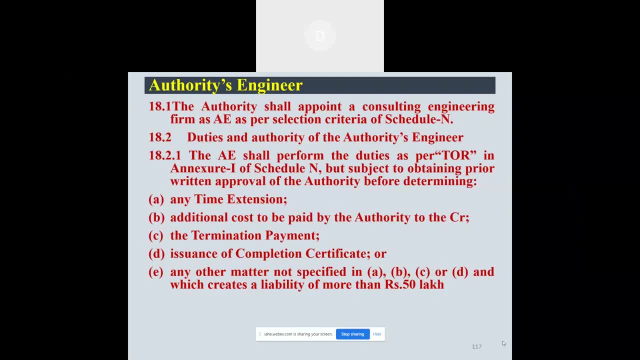 And then AE is there, he is having his own set of obligations and Why AE has been authorized for these things. Your question is why AE has been authorized for all these things. Yes, sir, Because see, as per international best practices, a 13-year-old is a third-party expert. 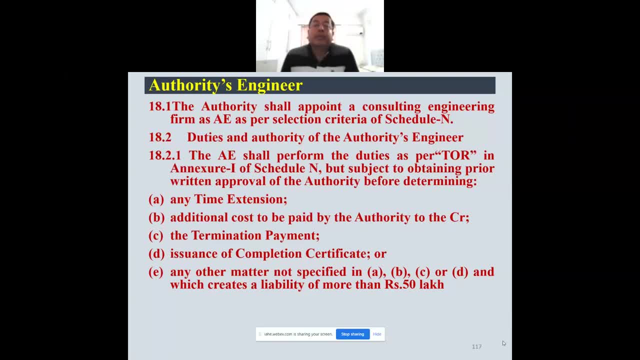 Yeah, And what he has to done as per Schedule N, in TERM of reference. everything is well defined, what work has to be done by the 13-year-old, And we want that. we should not interfere. We are not third party, You are the first party. 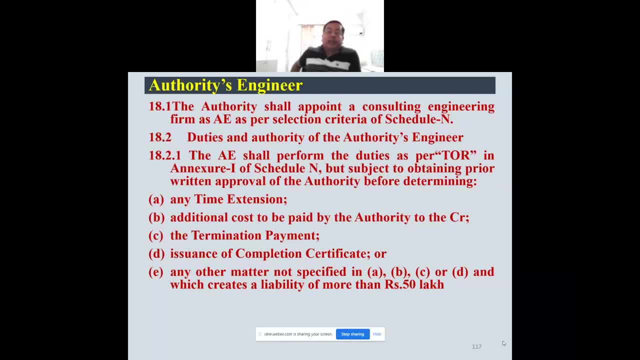 So whatever has to be done should be done by a 13-year-old. However, you can ask your 13-year-old that this is not as per the specification standard and as per the safety norms, And so you get it done. So authority engineer has been given every power. 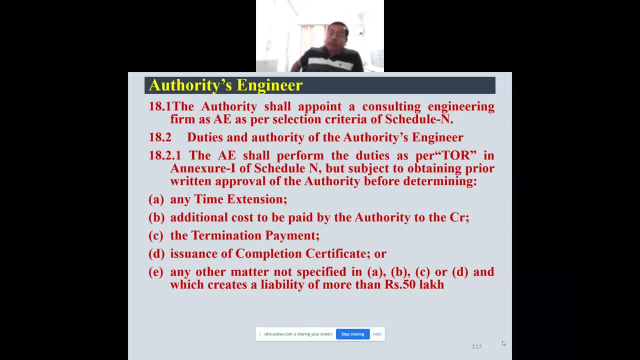 But some of the powers has been kept with the authority and he had to seek permission of the authority before taking any decision. So this is the international best practice Authority. engineer has been given enormous power but still he cannot decide time extension, COS termination, payment and issuance of completion certificate. For all these things he has to. 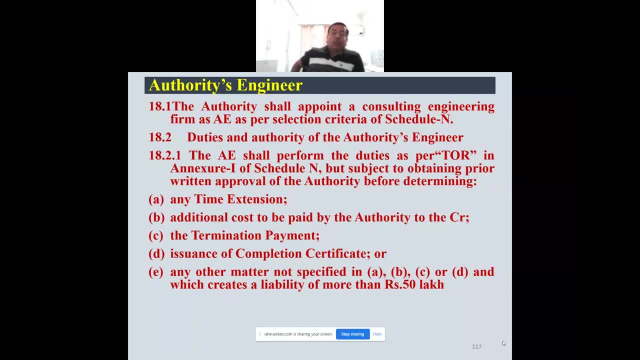 go to the authority for seeking permission. So this is a balancing that all the powers are not vested with authority engineer, But authority engineer is the main person who has to get the work executed through contractor. And authority engineer is not alone. Authority engineer is a team. 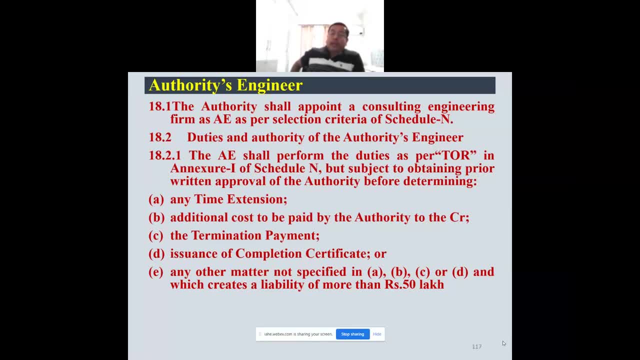 a firm, a firm with a number of key person, And each and every person, like team leader, RE, quality expert or quantity surveyor, and all the highway engineer, bridge engineer, all type of key person, are there and they are performing their duties and they have to follow this agreement and 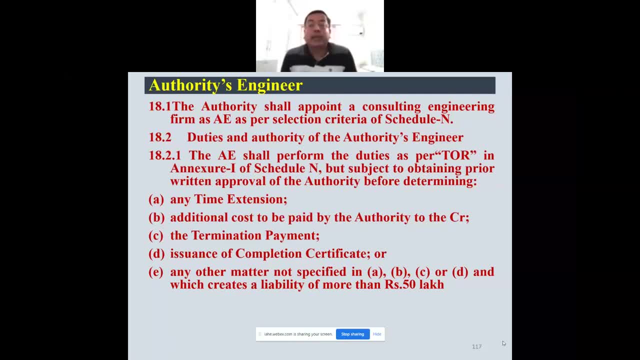 get the work done from the contractor as per quality assurance plan and as per safety norms and as per a specification standard of the contract agreement. So this is a very balanced document and you must also see that internationally it is a best practice that third parties should. 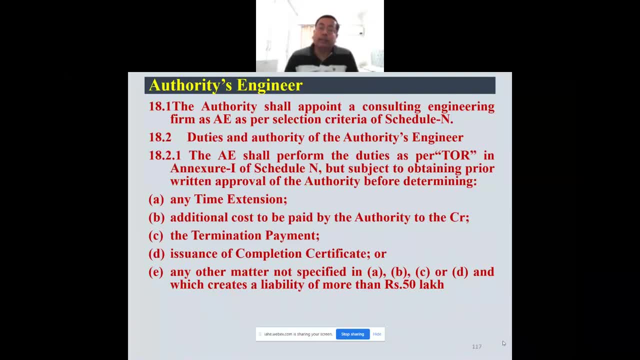 get the work done and third parties should have the expert. If you will tell, it will be a conflict. So instead of doing directly, it should be done through authority engineer. So this has been done, Okay. Yes sir, Yes sir, Thank you sir. 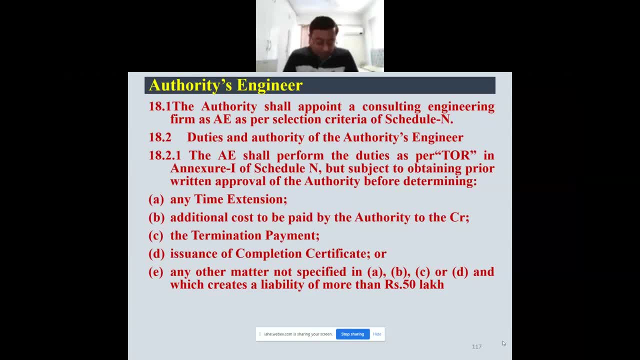 Okay. Any other query? Hello, sir. Yes, Sir, I'm from West Bengal, PWD, PWD, West Bengal. Yes, sir, Okay, So my question is, as per contract agreement, any change or the change of the scope? 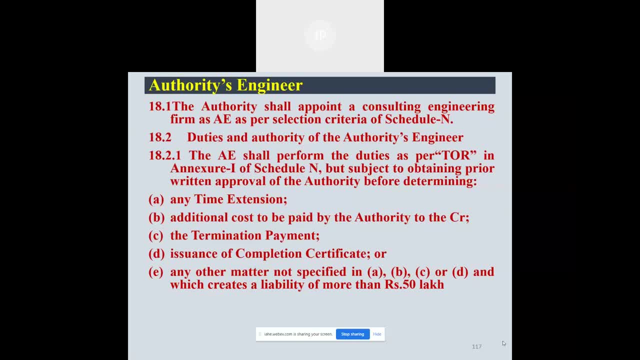 valuation should be calculated as per SOR- current SOR, Okay, And if there is any deletion of work, Okay, Then whether that should also be calculated from the current SOR or it should be calculated on pro-rata basis, as mentioned in the schedule H. 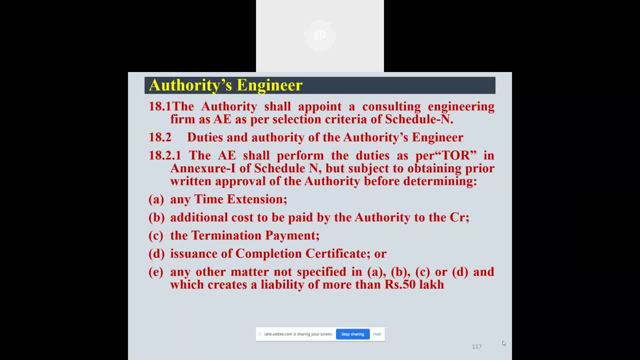 It should be as per schedule H. In case of negative COS, it should be as per schedule H, Because schedule H, how schedule H, has been finalized, Once contractor has designed, contractor has furnished you all the things, including schedule H and the schedule H has been examined by the 30 engineer or you. 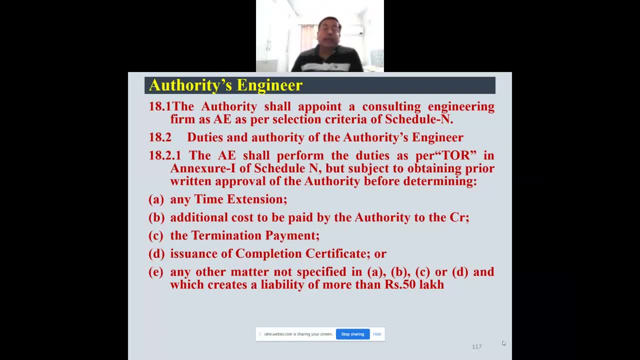 and you have approved it. Now suppose a culvert or 10 culvert is there which are to be deleted, The cost of the culverts can be derived from the schedule H which is in the contract agreement. So the cost of the culverts can be derived from that schedule H which is in the contract agreement. the connection. suppose 100 crore is the total quantum and five percent is the cost of work of that culvert and it is having 20 culverts, then for 10 culvert it will be half of that and that amount will have to be deducted as change of scope in case of negative cus. yes, 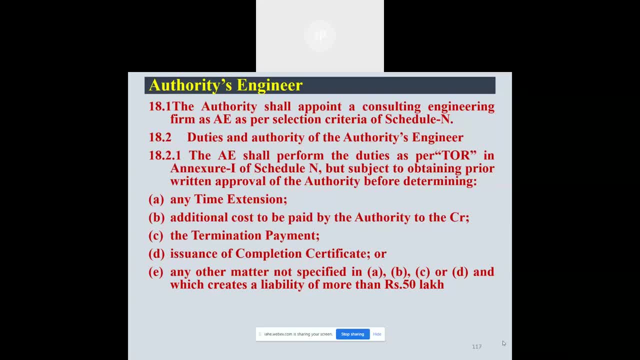 but in in one case my authority engineer has deducted by calculating the amount as per current sor. this is not correct for positive cos. it is mentioned. i will come later on on the cos and i will explain it. change of a scope for new change of a scope, sor rates are to be taken, but 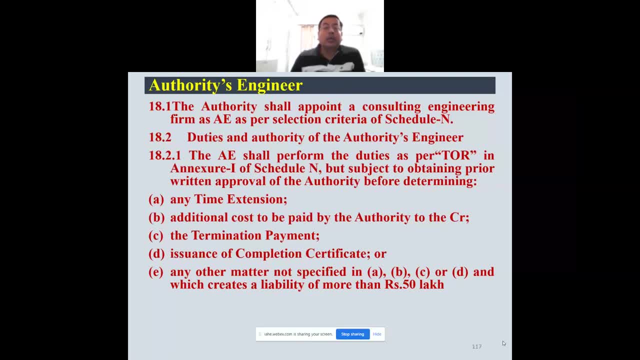 for reduction. schedule h is better because schedule h is already defined. everything is defined. now, if you are calculating a negative cus on the sor, you will have to pay something more to the contractor to be benefited. but in case of schedule h it is balanced because schedule h has been provided by the 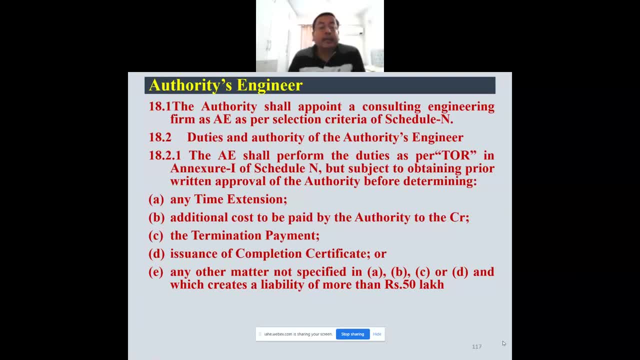 schedule h has been provided by the contractor and accepted by the authority engineer, and on that quantum only we are issuing negative cos. so there is no problem. so negative should be done as per schedule h. okay, thank you. any other questions? any other questions, sir one, i want just one more clarification. yes, sir, please. 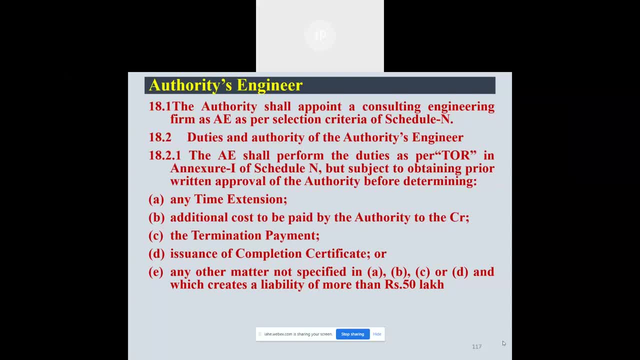 yes, sir, as per agreement, it is a return. 90 percent of rw should be provided to the contractor at the time of declaration of appointed date. okay, Then, whether it should be ROW or it should be 90%. length of working front: See when you will prepare appendix. I have explained earlier that they require working front including embankment and 3 meter parallel string. 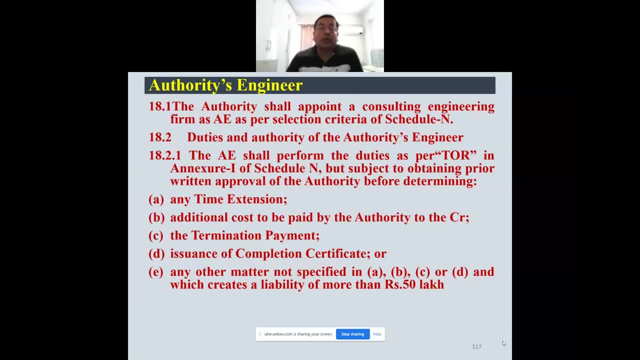 That is the thing which is required, not entire ROW. Suppose your ROW is 45 meter but you are constructing 2 length paired soldier And suppose embankment height is 2 meter, then 10 meter plus 2 meter earthen soldier. 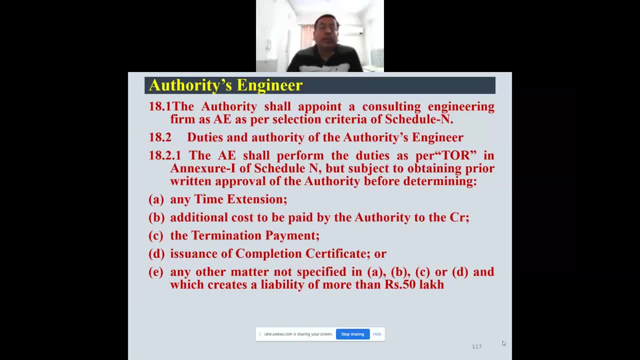 Suppose only 1.5 meter, but you assume 2 meter. 2 is then 12, 10 plus 14,, 14 plus 4.. 4. 3 meter on both sides, 14 and 8,, 22,, 22 up and plus 3,. only 25 meter is required. 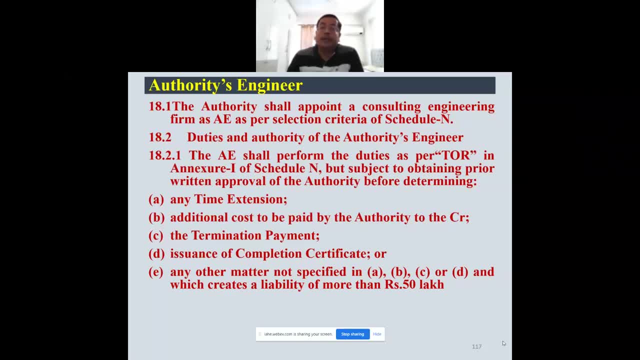 In that case only 25 meter working front if available. he cannot claim because it is written in the document That entire ROW is not required Working front including embankment and 3 meter parallel string. So it comes to 25 meter in this case. 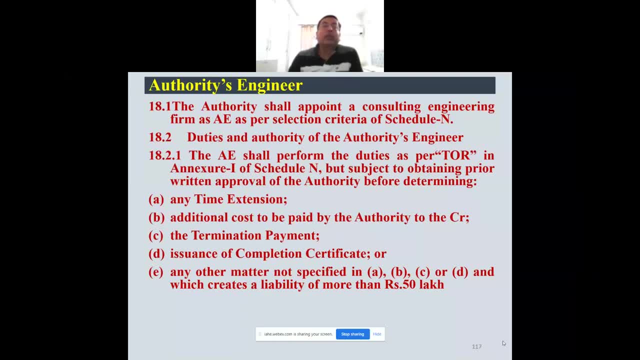 If the embankment height is 2 meter, So only 25 meter should be available, Because in that case he will be able to construct the ROW. So this has been defined in the agreement. And one thing is very much important: 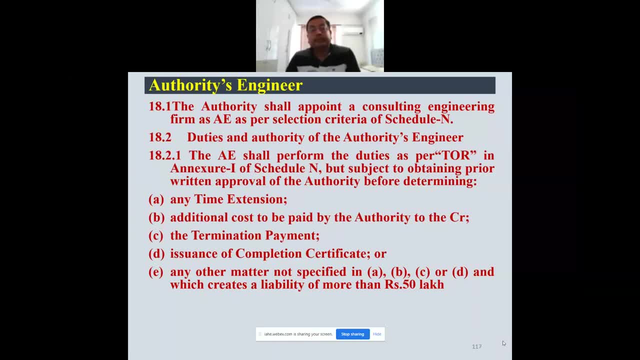 You can amend anything before bidding. Before bidding, you go through your site and, depending upon your site, you modify the agreement, the draft contract agreement, And prepare a table. Suppose you have amended 10 clauses. You mention all the clauses, what is written in the clause and what modification you have done. 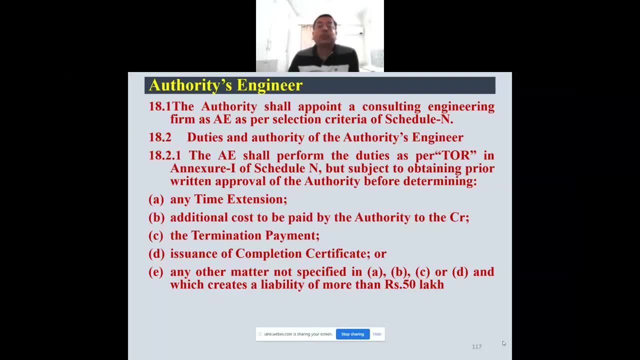 And remarks why you are modifying And take approval of the completed 30. And then only float the bid, RFP and the DCA. Suppose all the things are in the DCA. nobody can challenge you. Because, Sir, it is not better that we can define the definition of ROW? 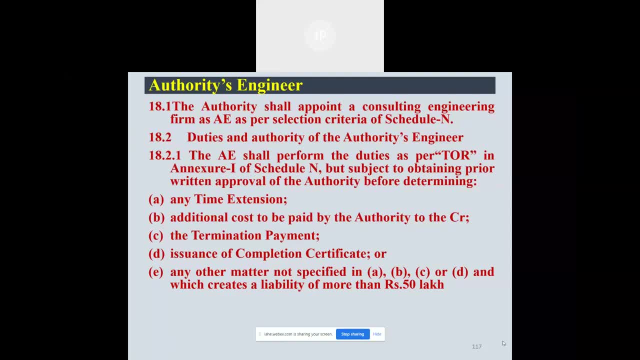 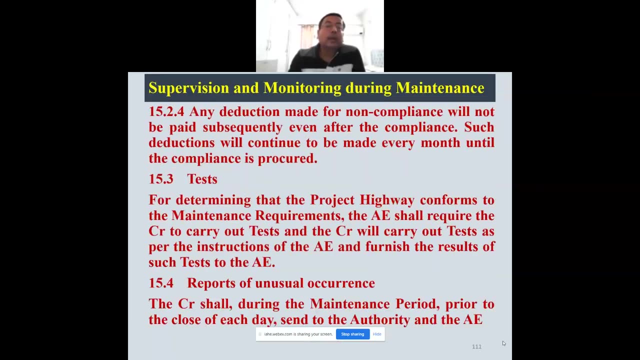 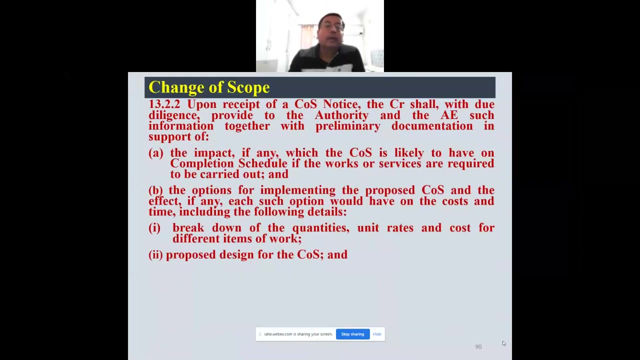 Yes, ROW is In general. ROW means. ROW means right of way, But it is written in that way. In that slide I have mentioned, I am going to show you. The ROW in the DLM format is look like this: 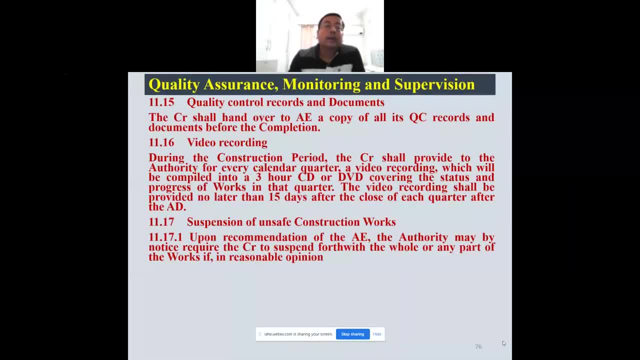 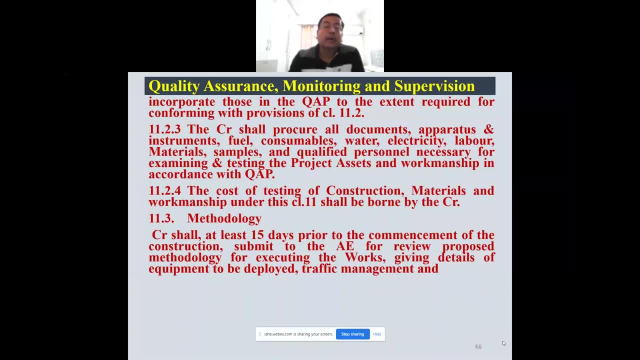 And if you want to see the ROWs look like this In the ROW you have to write this, So you copy the ROW. And then you have to write the ROW And it is written in the DLM format, So you do that. 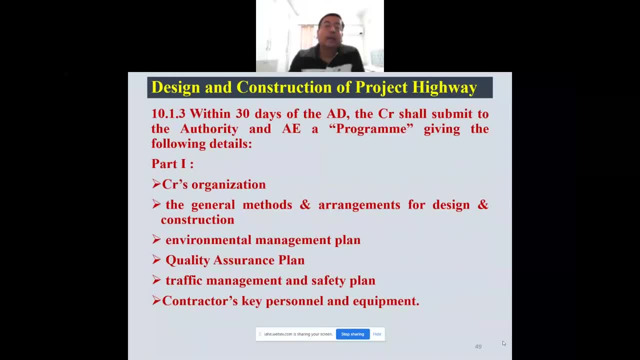 The board is covered with the ROWs, And then you have to look at the default, Then you have to look at the ROW. In this case, you say this is ROW, This is ROW, And then you have to add ROWS to this.